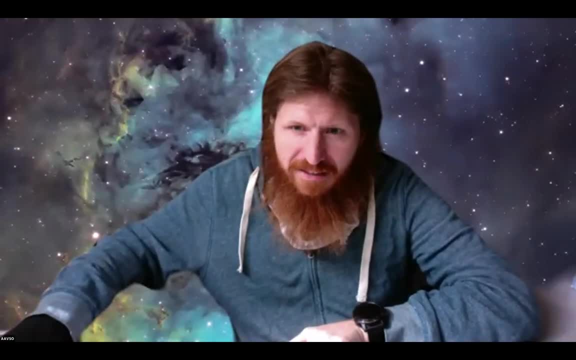 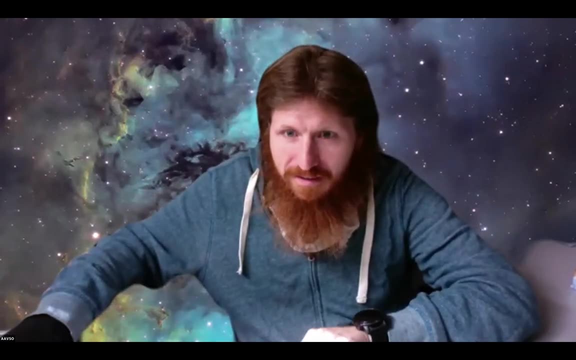 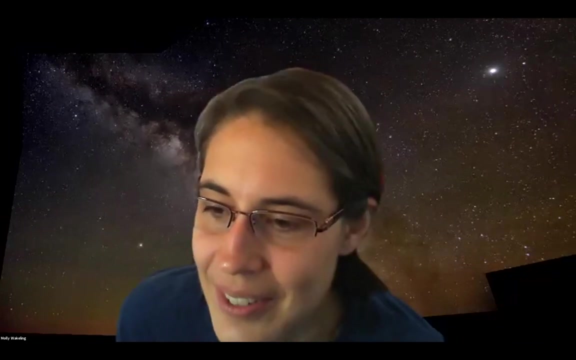 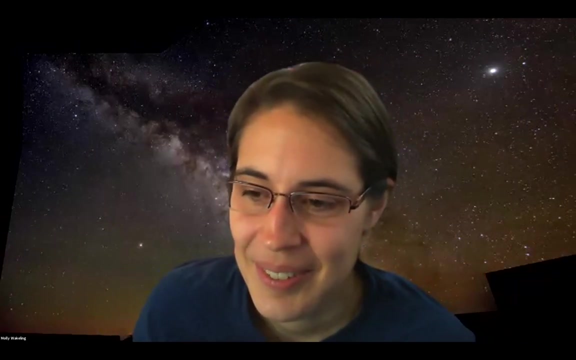 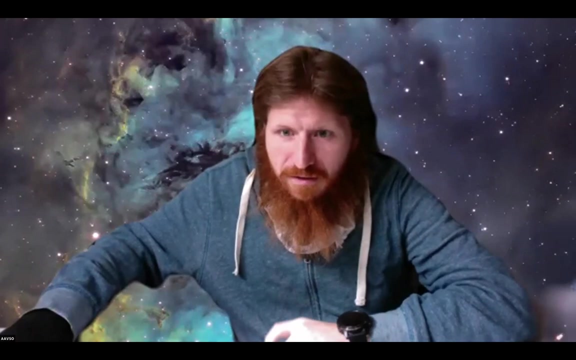 Southwest Missouri, Finland, and oh, SLU is the group I remember now, Yeah, yeah, India, All right, Spain, UK, Ohio, Abacoikee, San Clemente, Central Florida, Wow, Sorry, So many, I can't keep track. 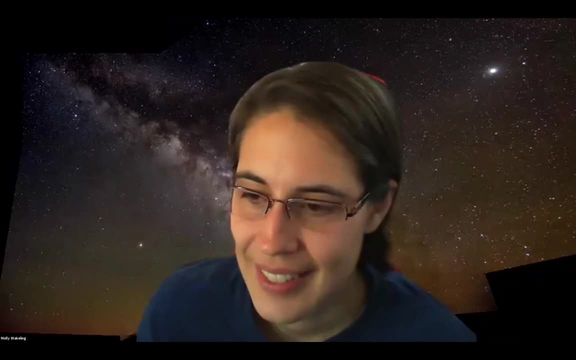 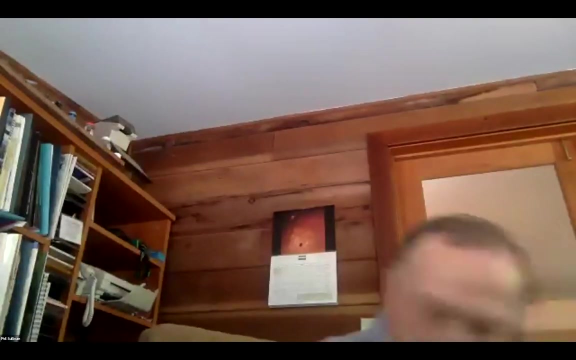 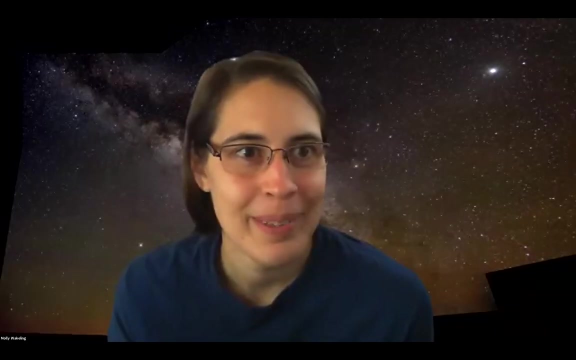 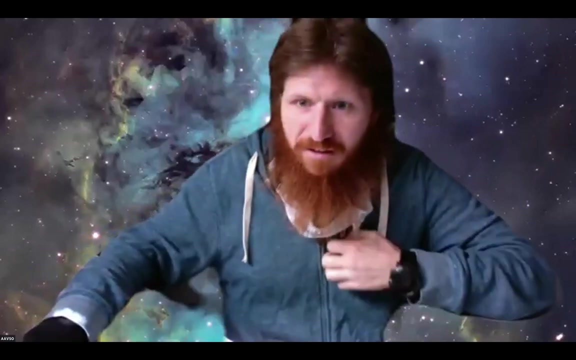 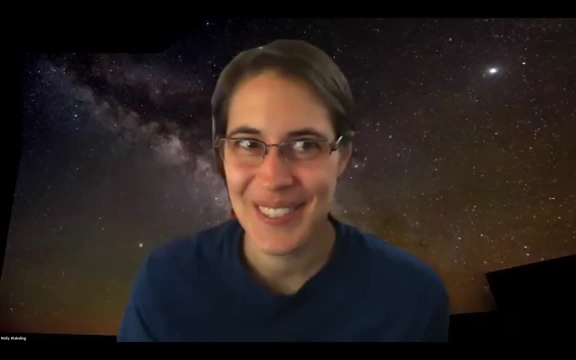 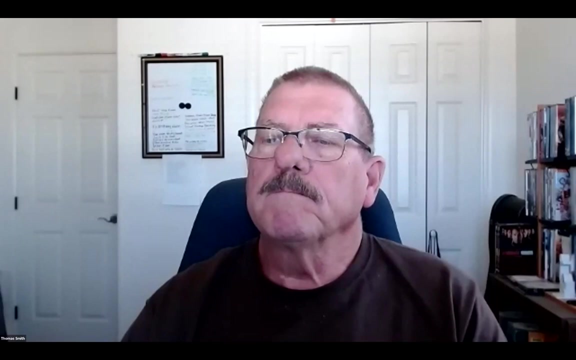 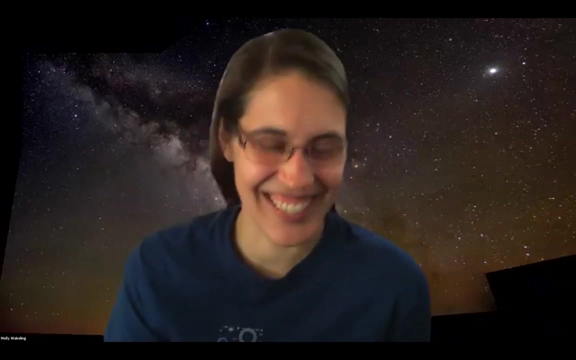 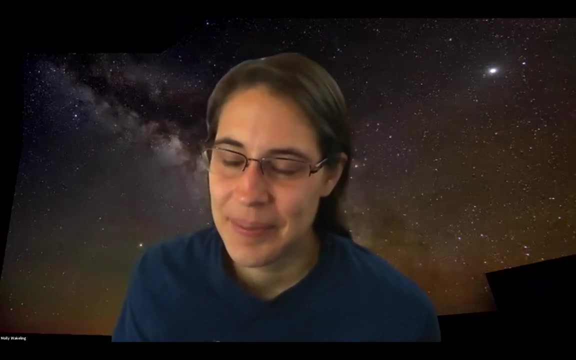 Okay, Oh, Barbados. Cool SLUvian sounds very Dr Seuss-esque. Yes, it does. I was just thinking the same thing. That's my favorite, All right. Well, it is 11 o'clock. 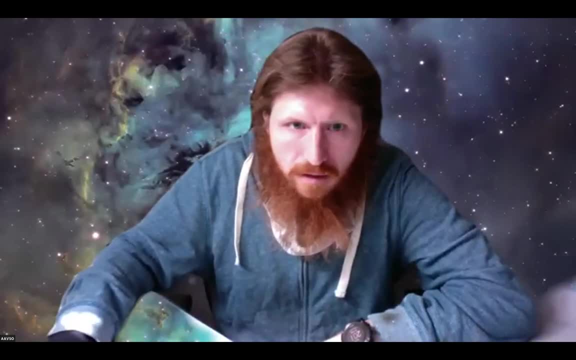 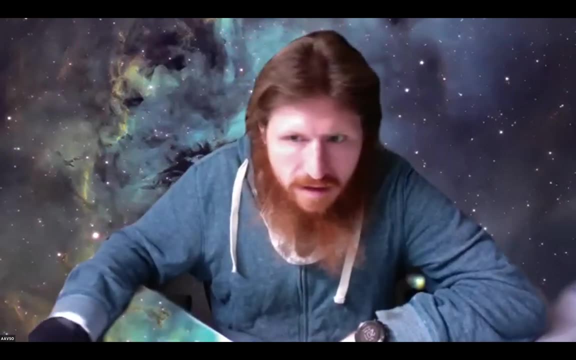 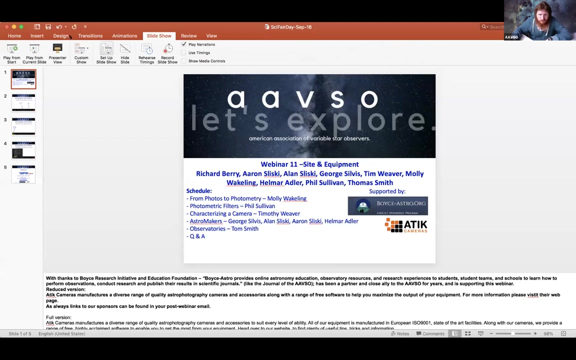 Yep, Let me go ahead and share my screen real quick And we can get started. I'm going to have to make this into a slideshow view. Oops, I have the webinar over the top of it, so we can't actually. There we go, Hello everybody, and welcome to the first. 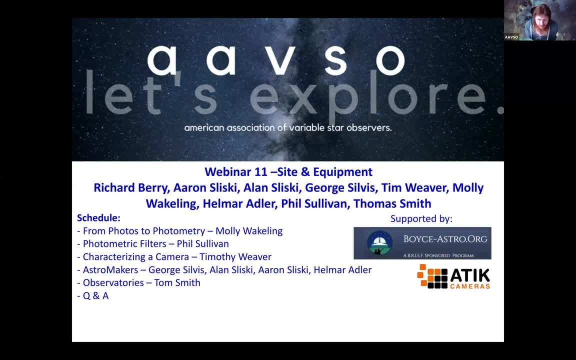 of two site and equipment webinars that we will be having to close out our very successful observing section webinar series. This one will focus on- Well, it won't really focus. It's going to tell you as many things as you can possibly want to know about the intricacies. 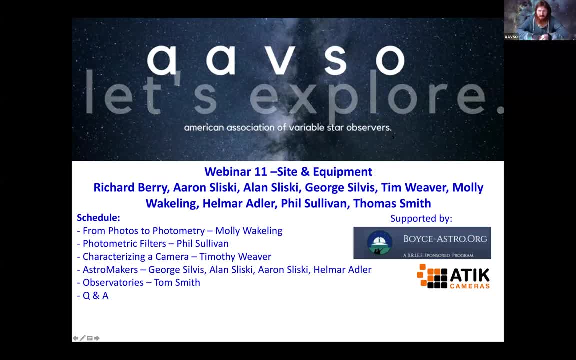 of the different ways that you can get involved with the, with site and equipment, and all of the different possibilities that exist there. Obviously, it won't be all of the different possibilities, but it will at least cover quite a few of the highlights. The first thing that I'd like to do is 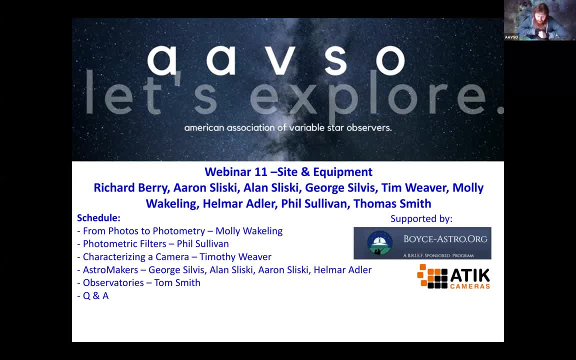 You know. Okay, I'd like to give a big thanks to our sponsors, Boyce Astro and their Initiative, and Education Foundation. Boyce Astro provides online education, astronomy education, observatory resources and research experience to students, student teams and schools to learn how to perform observations. 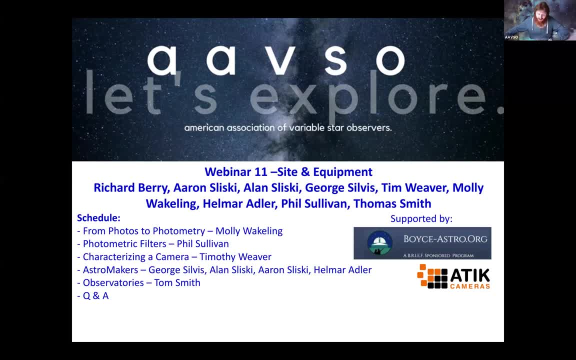 conduct research and publish their results in scientific journals, And they have been a close partner and ally of the AAVSO for several years. at this point, We would also like to thank ADEC Cameras. They manufacture a diverse range of quality astrophotography cameras and accessories. 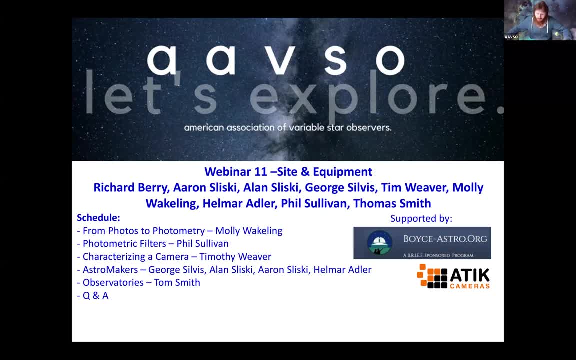 along with a free range of software to help you maximize the output of your equipment. For more information, you can visit their web pages. As always, there will be links to those in the post webinar email that you will receive. Just a few highlights about the webinar series itself. 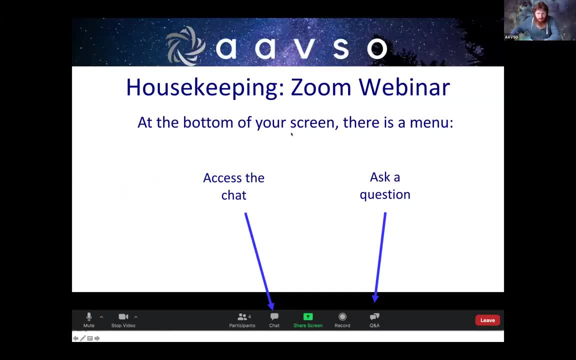 Okay, All right. So a quick reminder. the chat will be located here. Most of you have already found it. You can ask a question through Q&A. Please ask your questions here, as we can easily scroll through them. Sometimes they are very difficult to find in the chat. 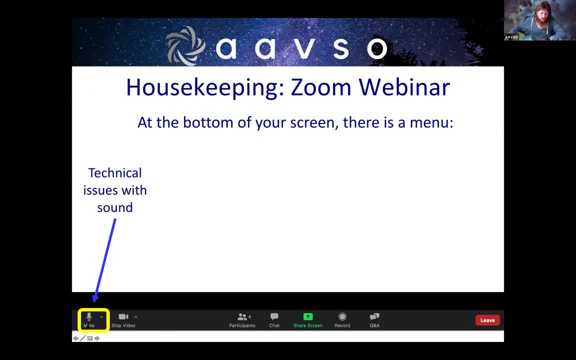 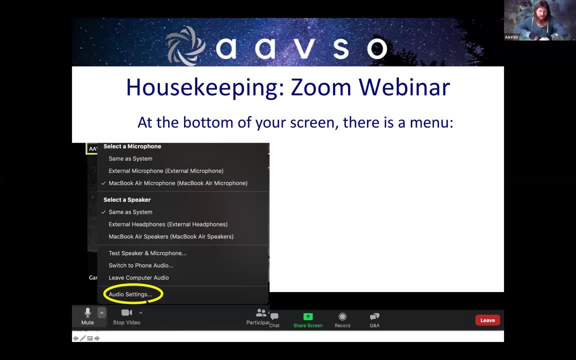 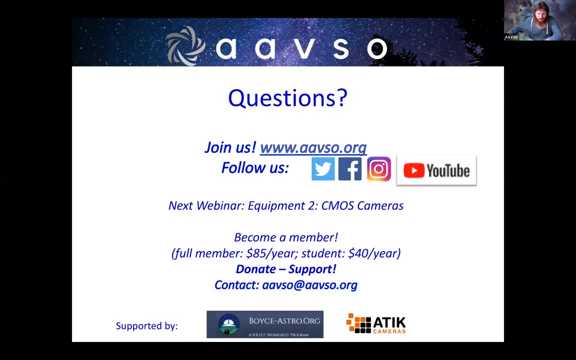 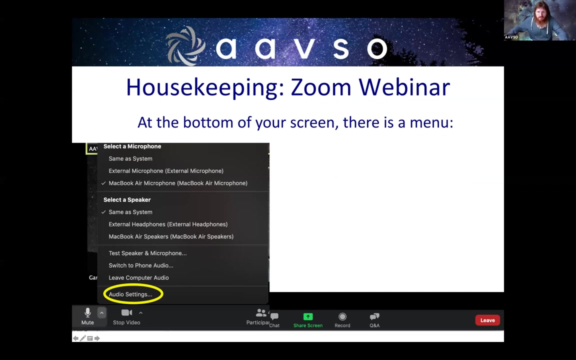 If you have any sound issues, your best bet is to go here. Hopefully there will be something here that will help you with your audio session. There isn't much that we can control on our end, So hopefully you can figure that out And, without further ado, I will send it off to Richard Berry to introduce the Site and 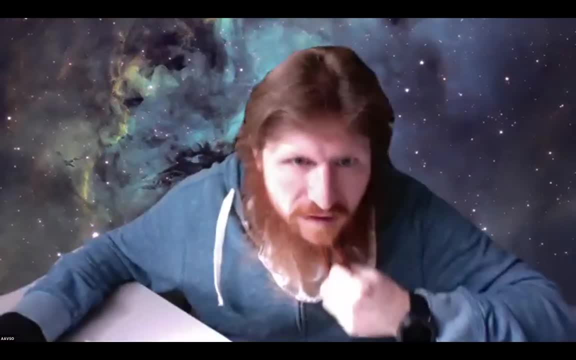 Equipment Observing section: RICHARD BERY. Thank you, Bert. The sections for many, many years did not introduce the site and equipment observing section. I think it's important to note that there are a number of different sections. One of them is the Site and Equipment Observing section. 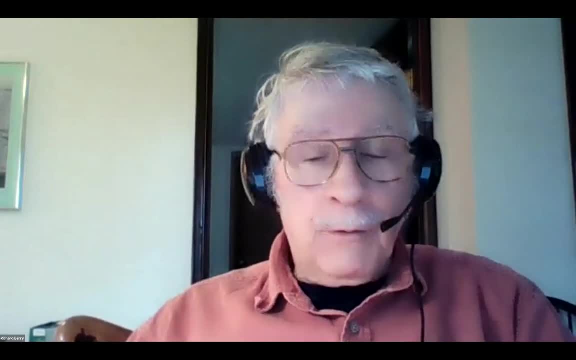 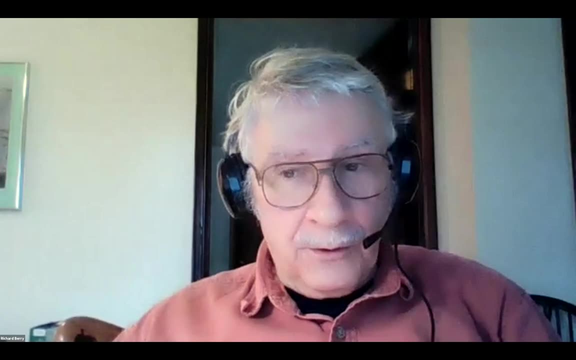 The other is the Site and Equipment Observing section. So the site and equipment observing section is a section that includes the instruments and equipment that we use. They were focused almost entirely on the objects we observed, And yet there was a continuous and ongoing need to talk about instrumentation and to 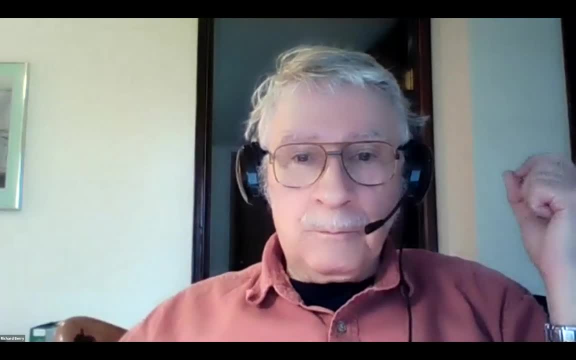 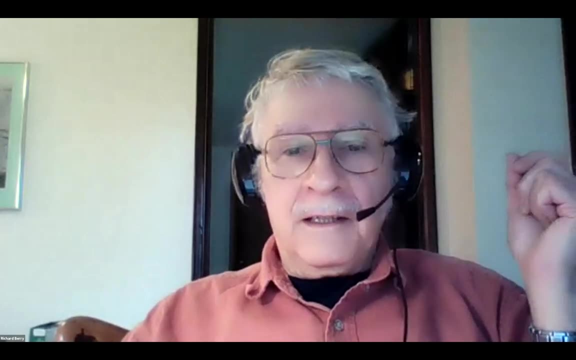 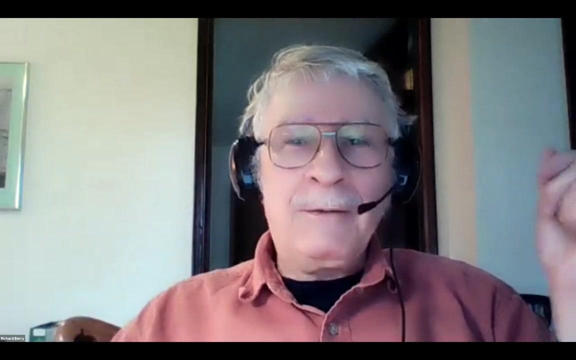 talk about the equipment. So I think sometime earlier this year they said we need somebody to take that over. So we did. I finally said okay, I'll do it, having no idea what I was getting into but thinking you know it might be fun. 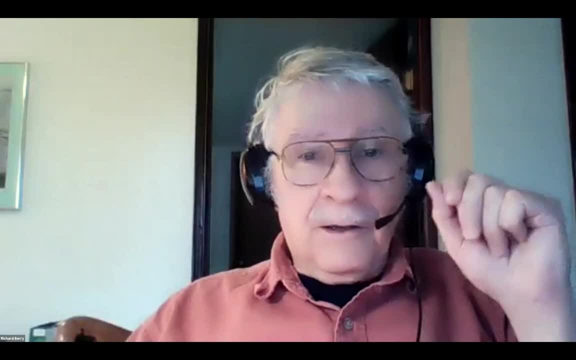 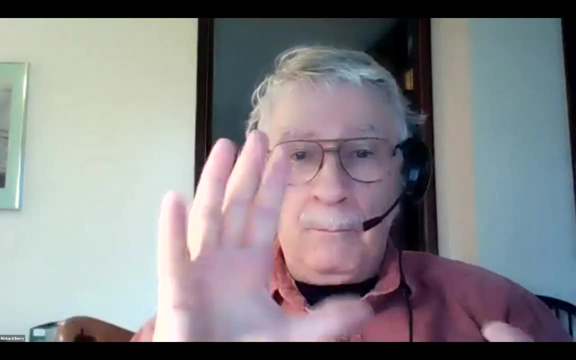 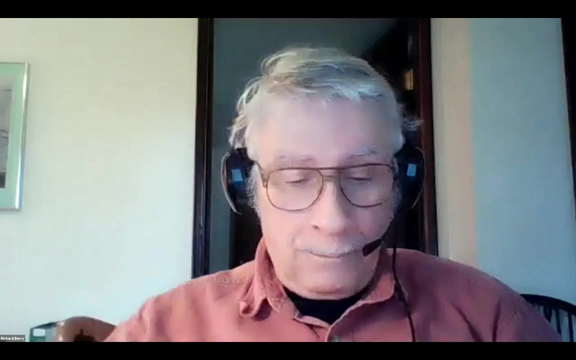 And it has been fun- Our section now covers- we called it instrumentation, because I'm now talking about things that measure stuff, and equipment, which is things that do stuff like telescope mounts, whereas instruments will be more like cameras and stuff like that. 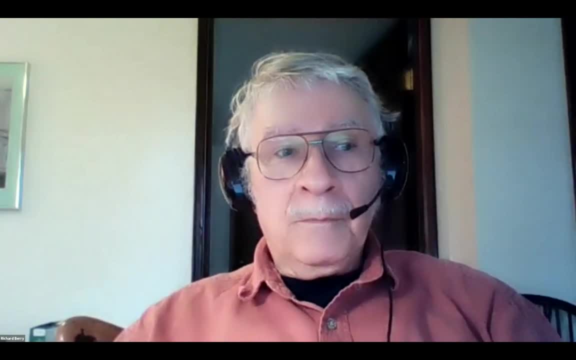 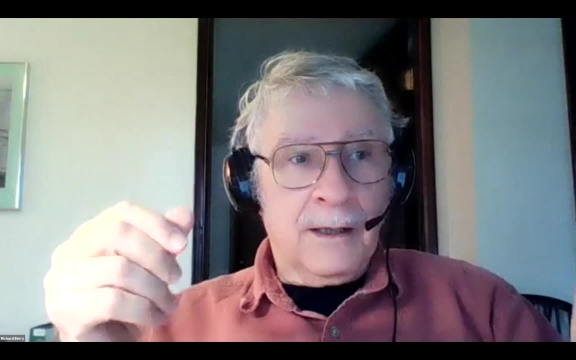 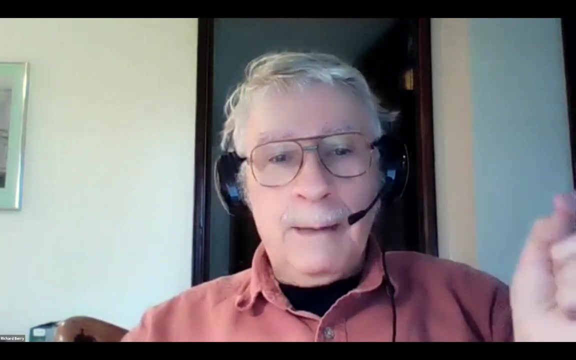 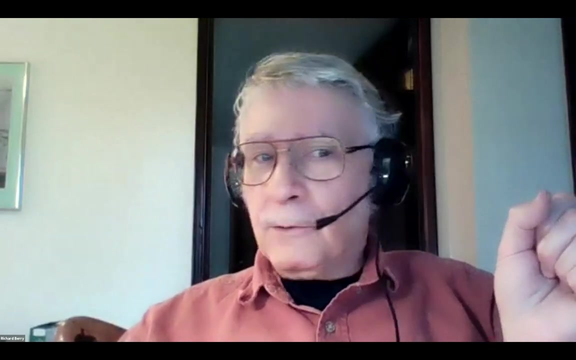 Today's group we put together to present a diverse picture of what the section is all about. We'll begin with Molly Wakeling talking about how a photographer became a photometrist. Okay, and I think there's probably a lot of beginners out there who are thinking I don't know if I can do that- 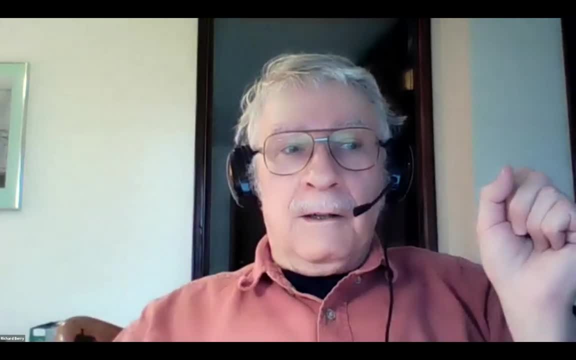 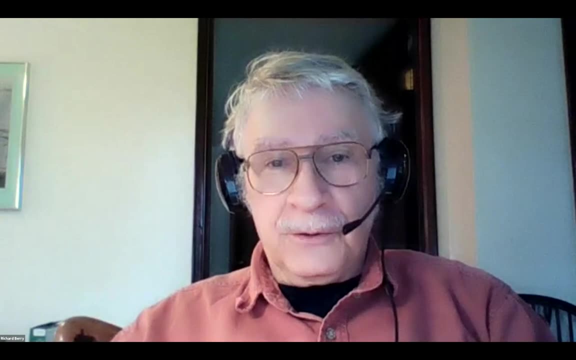 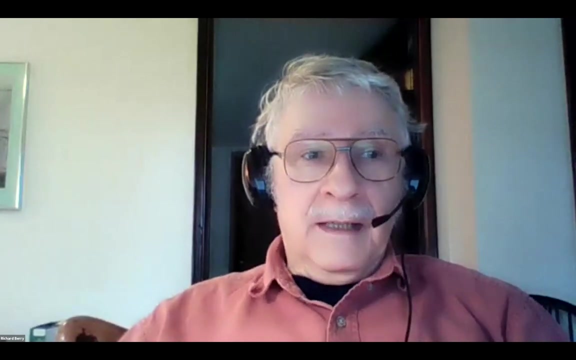 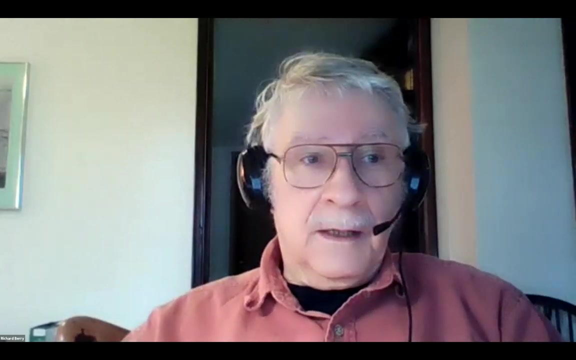 Well, Molly will talk about how to do that. Photography Photometric filters by Phil Sullivan. Astronomers like to use filters so that they know what wavelengths we're looking at. Phil will fill you in on that. One of the fundamentals in understanding how your camera works, whether it's CCD or CMOS, is characterizing. 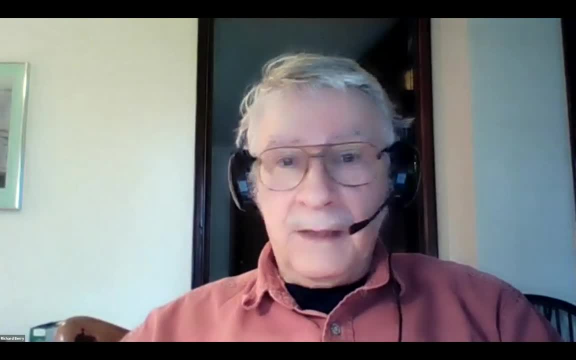 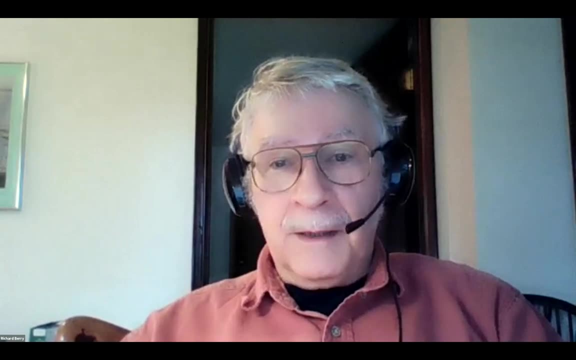 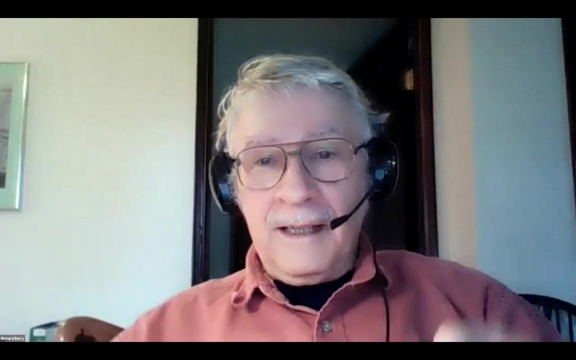 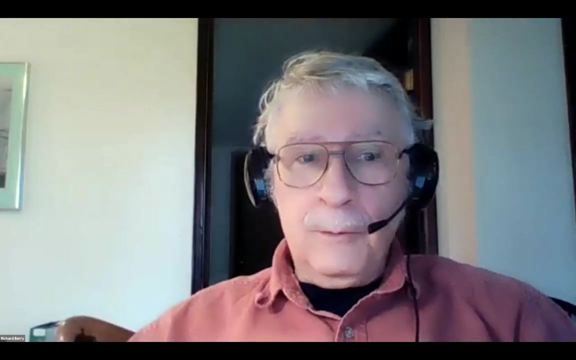 What's the gain? So forth. Is it linear? Timothy Wakeling will be talking about that, And the most fascinating areas is astromakers. you can build your own equipment like a really, really great flatfielder. So George Allen, Aaron and Helmer will be talking about that. 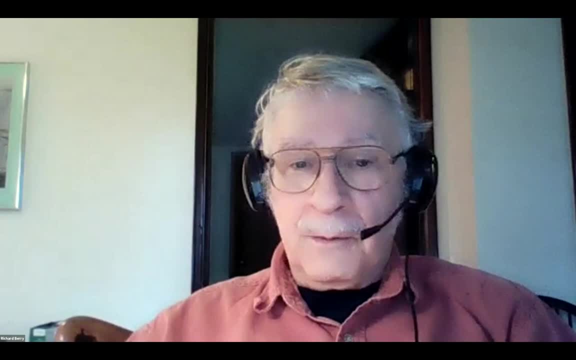 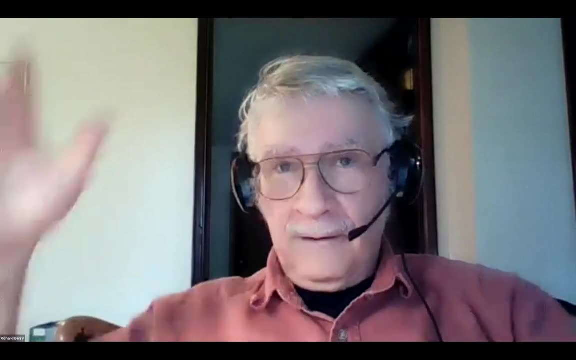 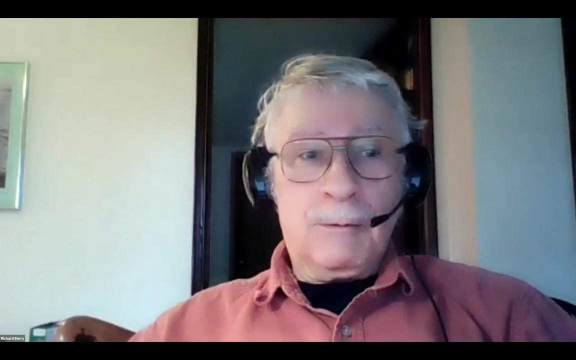 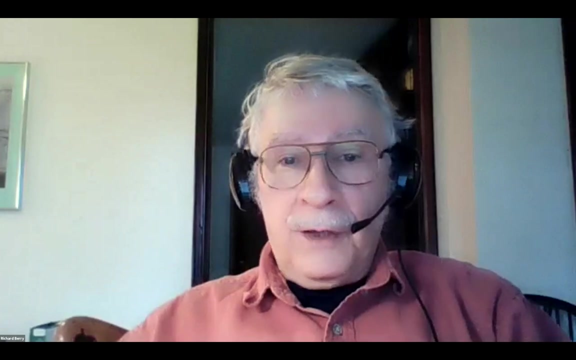 And we'll be wrapping up with Tom Smith talking about observatories- Hopefully everything from the very simple thing you can put in your backyard- a tarp over a pile of 2x4 frame- all the way through to something really, really fancy, And then there will be a question and answer at the end. So, without further, 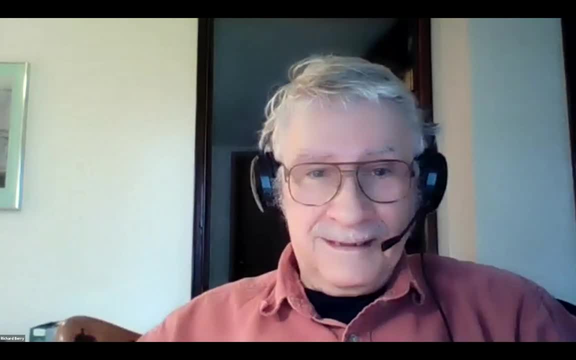 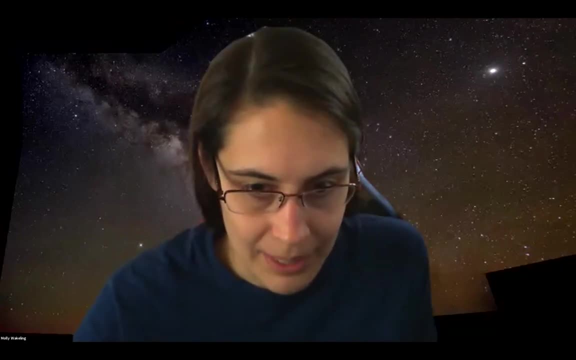 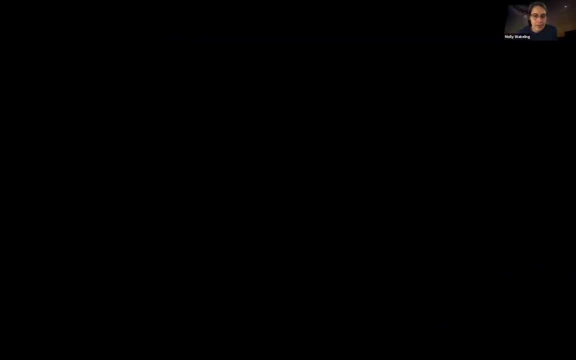 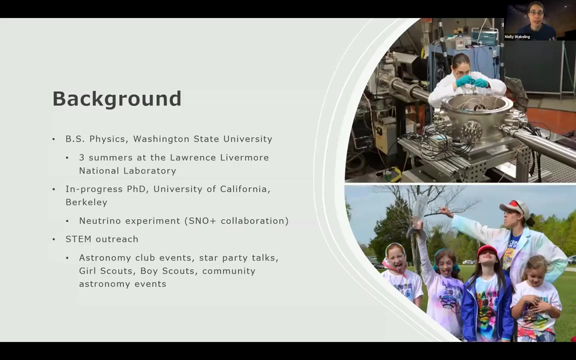 ado, I will turn it over to Molly. Good morning everyone. So I'm just gonna go ahead and hop into my presentation here, because that's where I have my introduction and whatnot. All right, there we go. Okay, So I am an astro. I've been doing astrophotography for about the last. 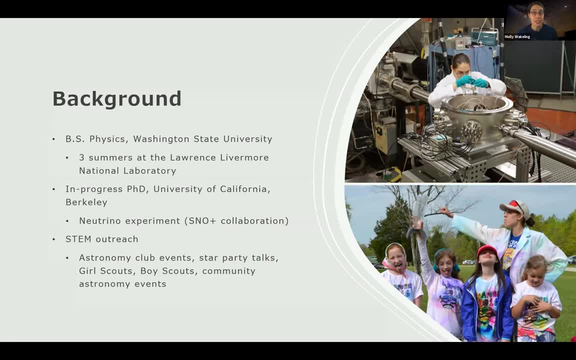 five years and I have been wanting to do scientific observing for a while, So I'm gonna talk about in this presentation how I've been, how I used equipment that I already had and the similarities between the two- The similarities and differences between doing astrophotography and scientific data. 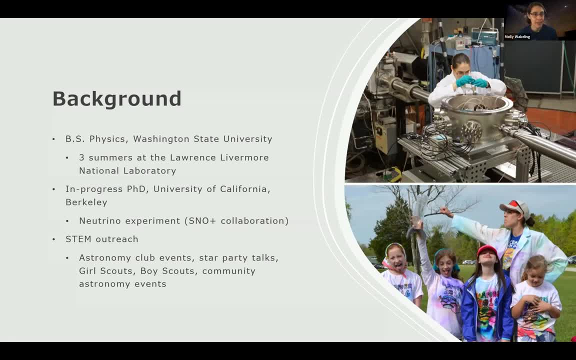 taking. So first a little background on me. I have my bachelor's in physics from Washington State University and I got to spend three summers working at the Lawrence Livermore National Lab where I got to do a lot of hands-on experiments and stuff like that. So I love. 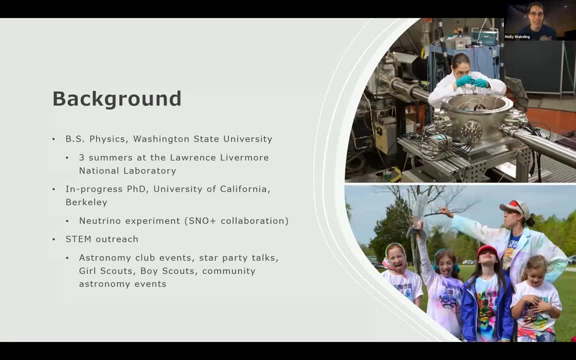 messing around with hardware and learned a lot about sensors and detectors and stuff like that. So it's It's It's. It got me a lot into working on the hardware side of things, Currently working on my PhD at UC Berkeley doing neutrino experiment stuff, and I do a lot of STEM outreach as well. 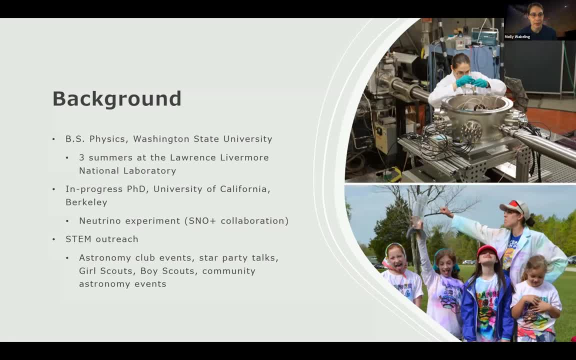 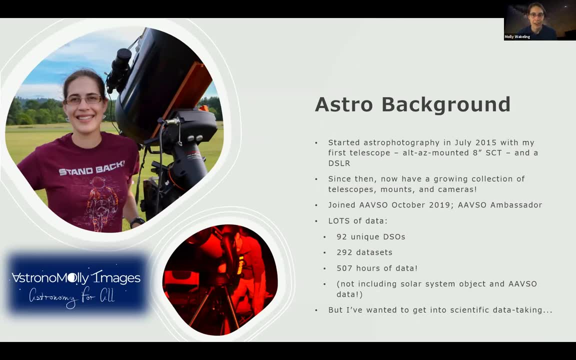 I like to do a lot of stuff with scouts and star parties and astronomy club events and things like that. On the astrophotography front, I started out with an eight-inch Schmidt-Cassegrain on the Altaz mount with the DSLR and have 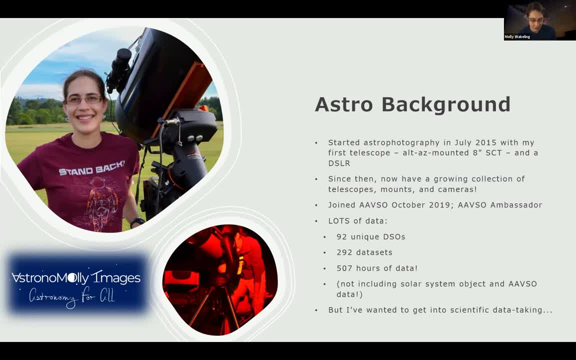 My equipment and knowledge base Have grown quite a lot since then, and I've been able to do all kinds of different astrophotography and get really into it. I just joined the AAVSO back in October after meeting Stella Kafka through a mutual friend, and so that's kind of how I learned about how I can do some. 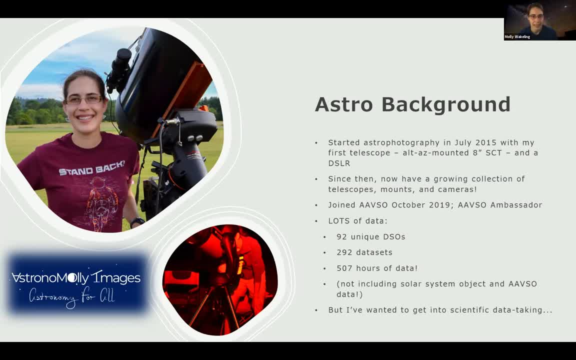 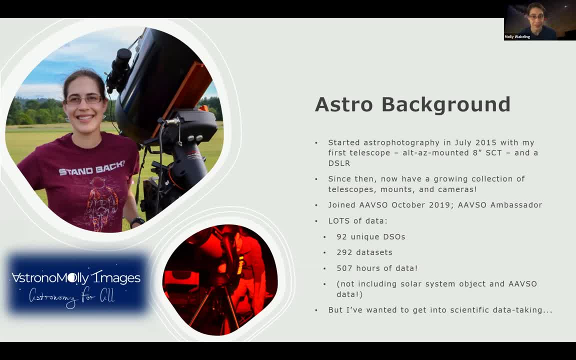 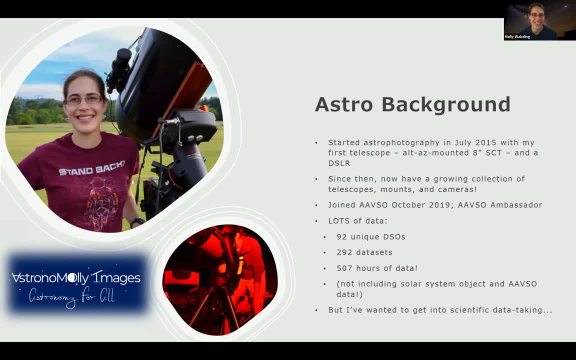 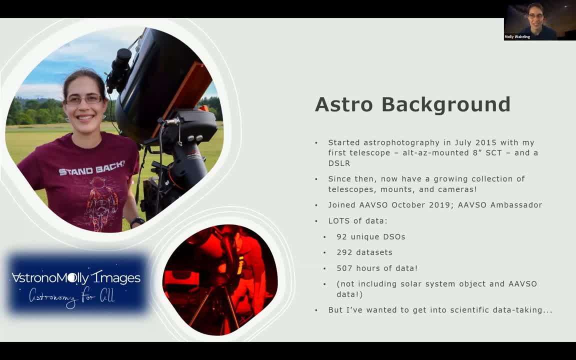 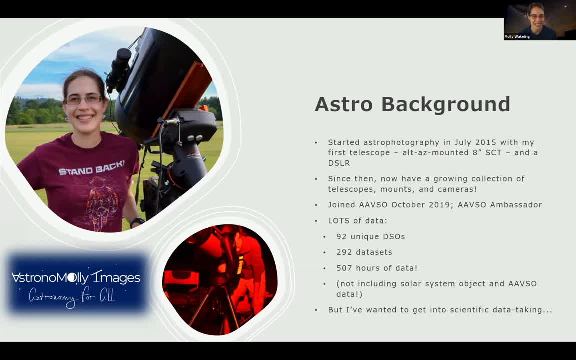 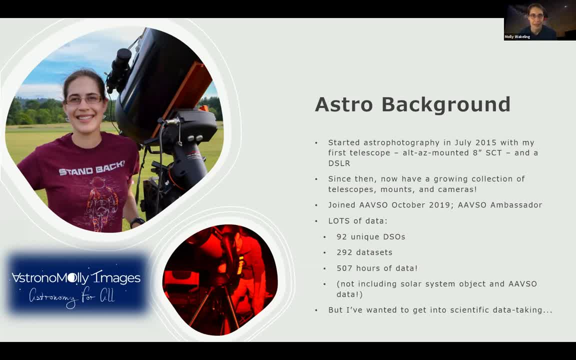 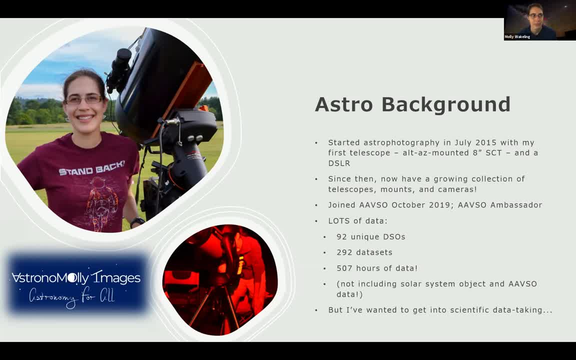 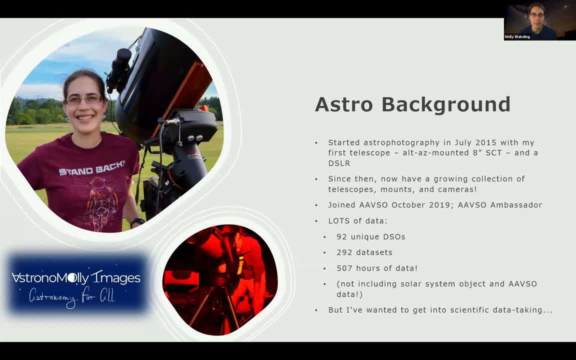 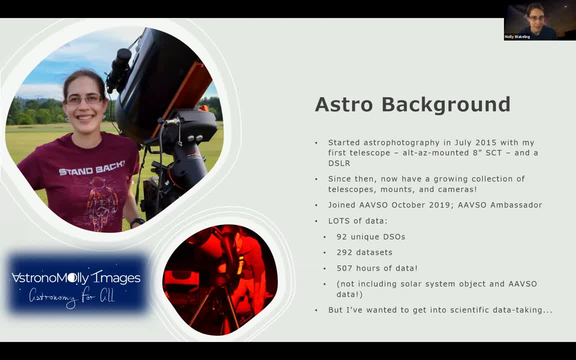 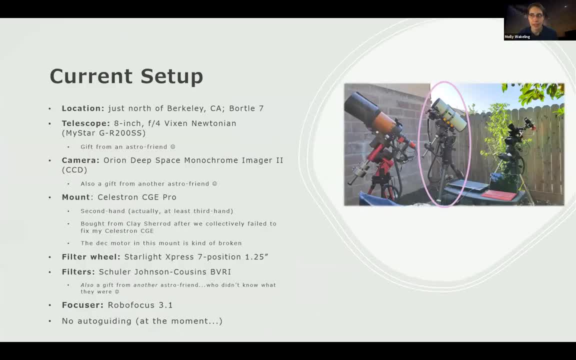 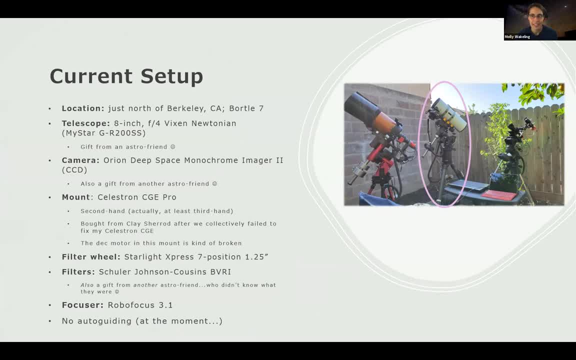 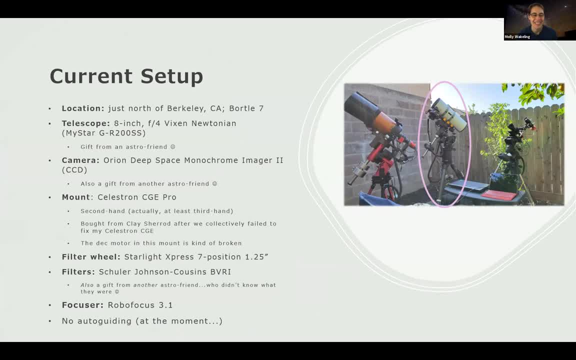 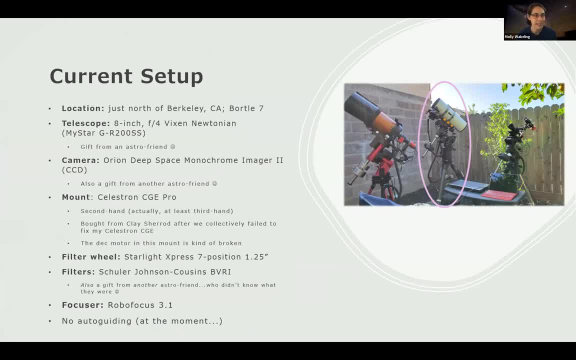 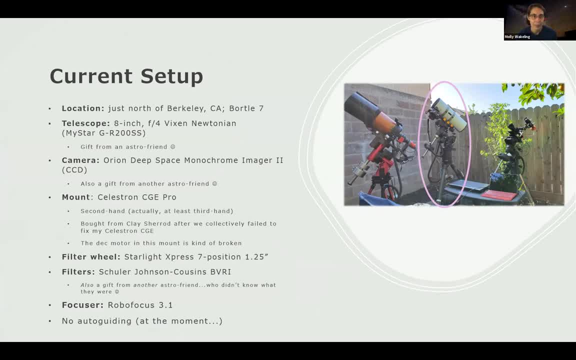 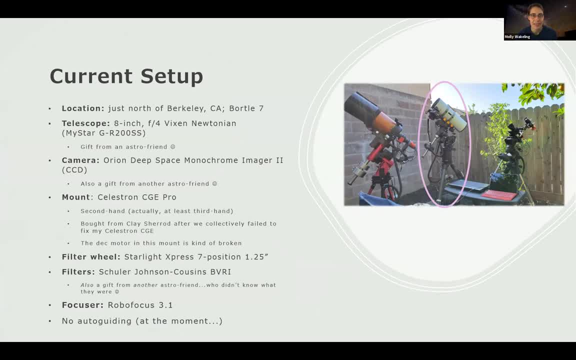 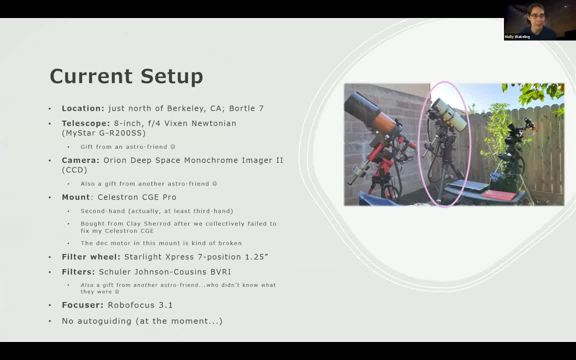 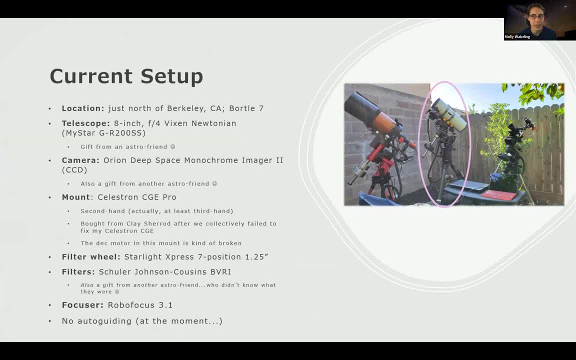 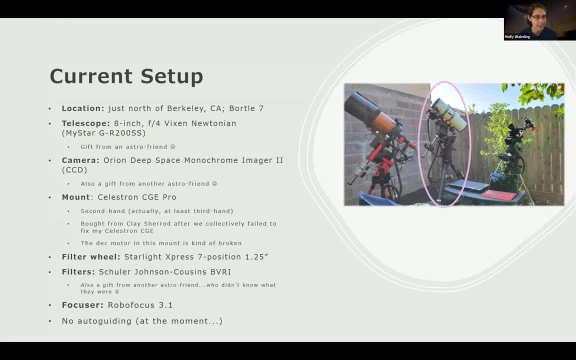 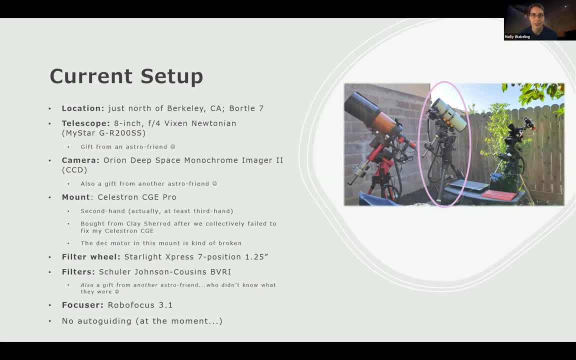 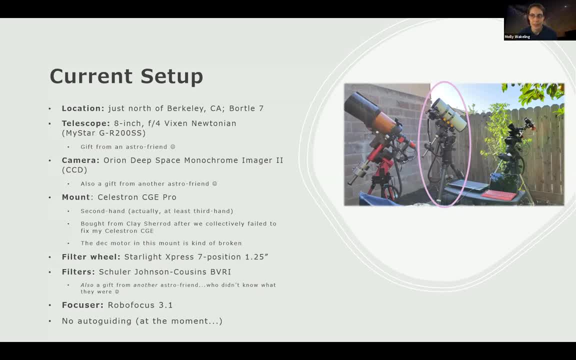 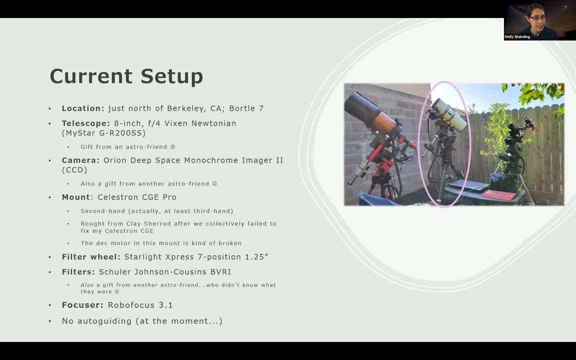 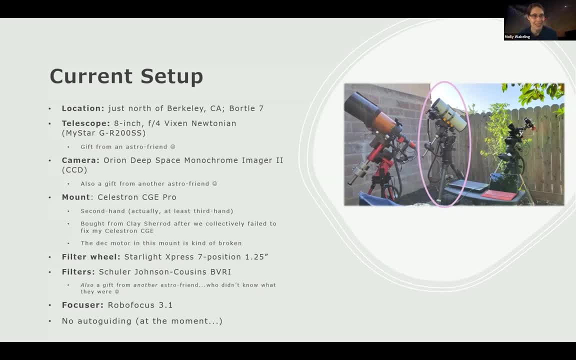 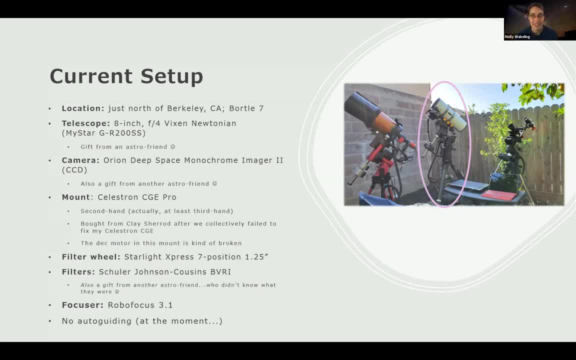 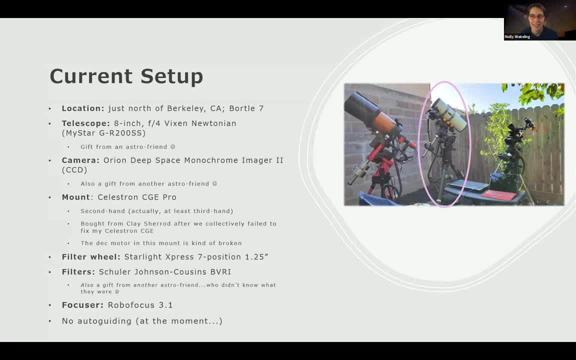 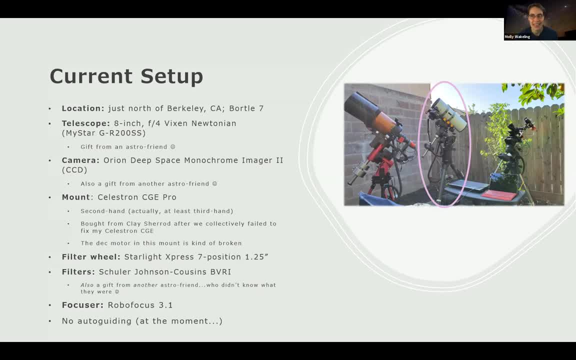 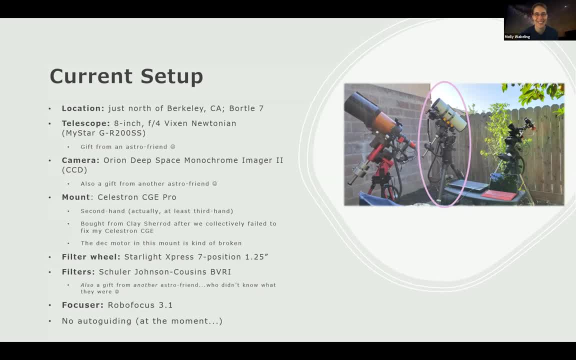 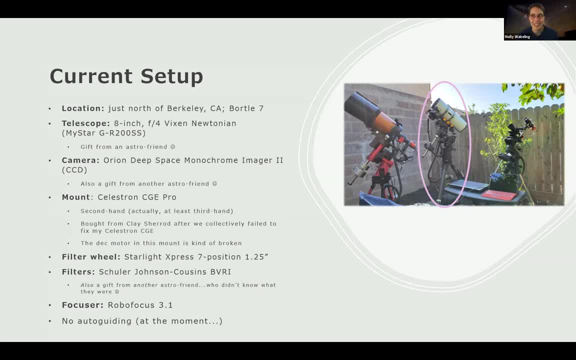 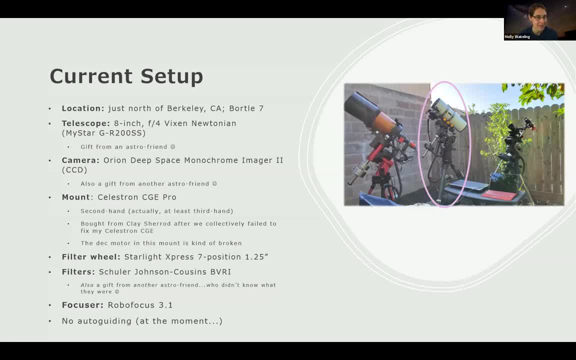 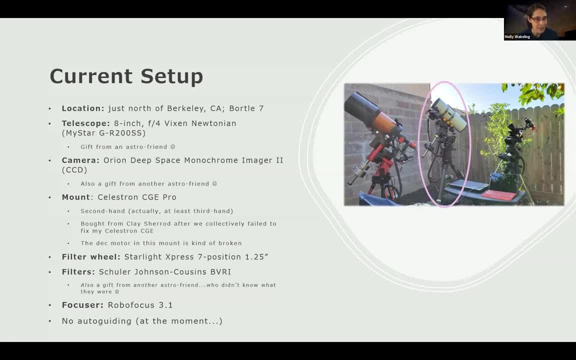 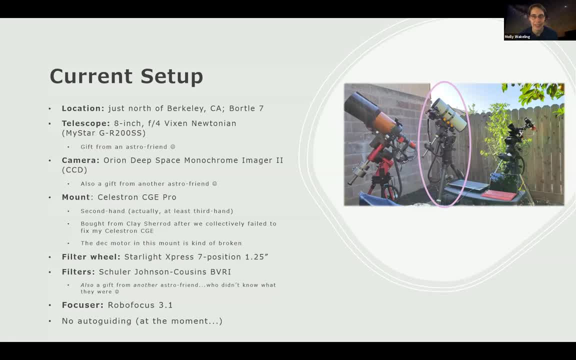 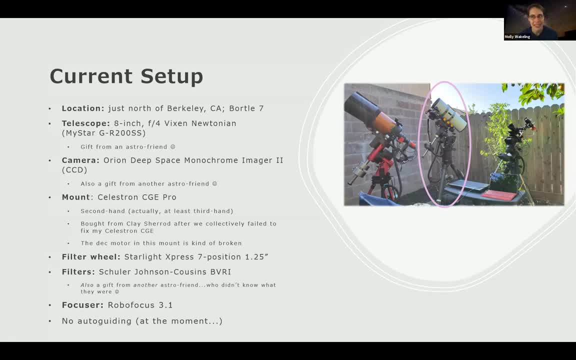 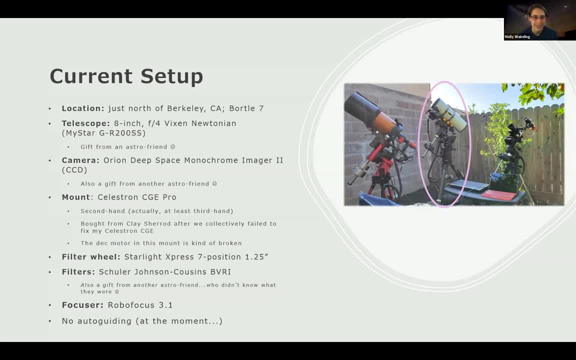 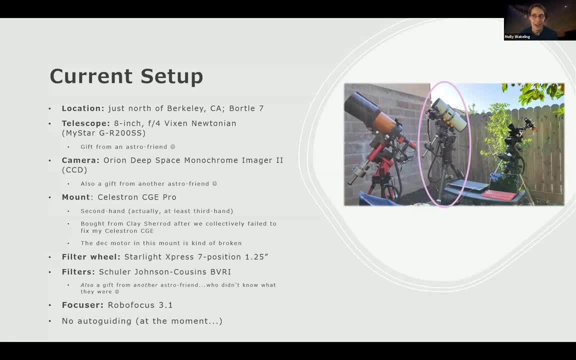 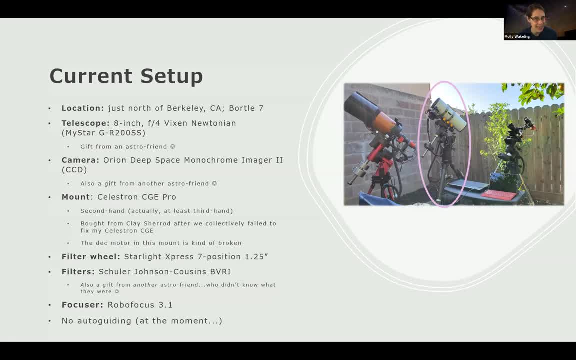 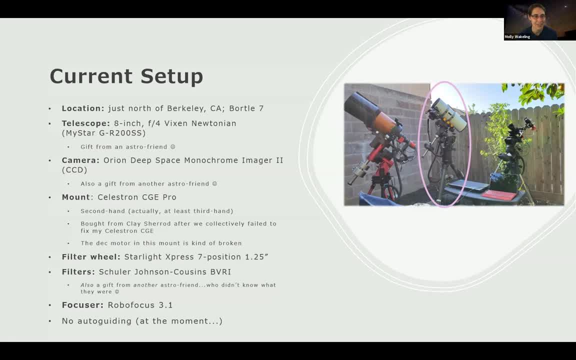 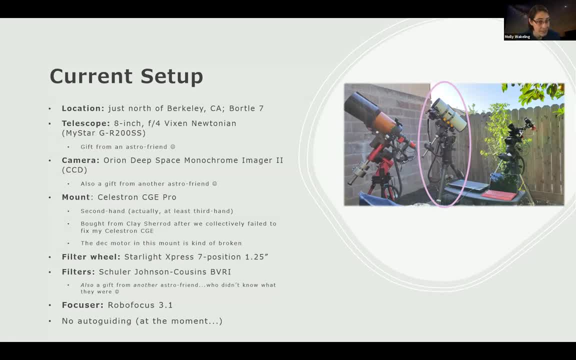 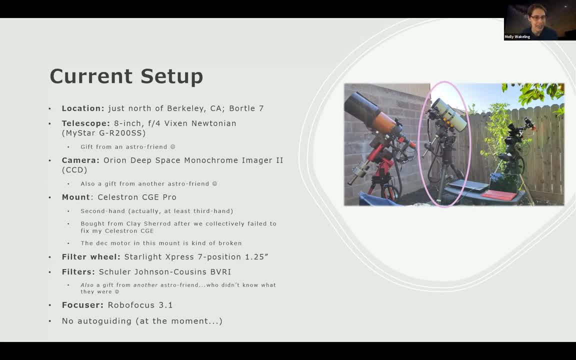 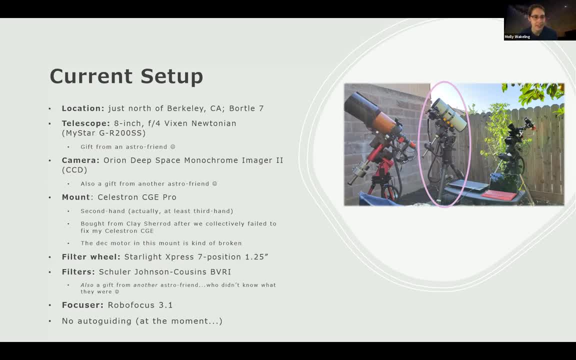 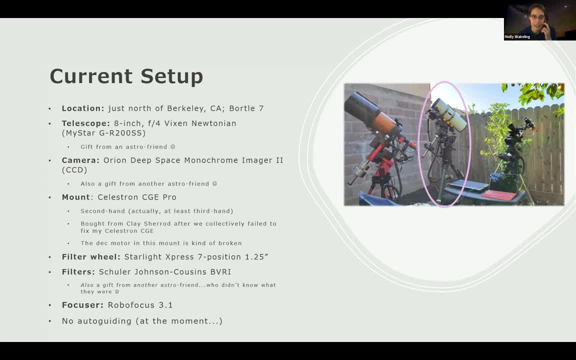 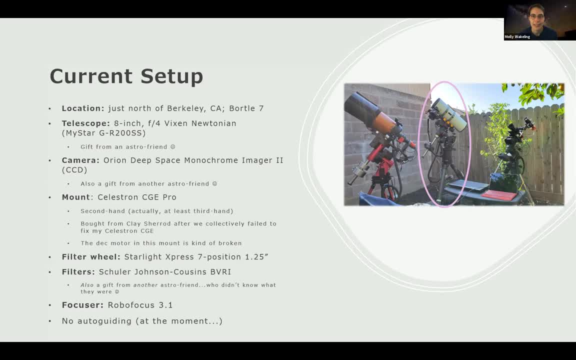 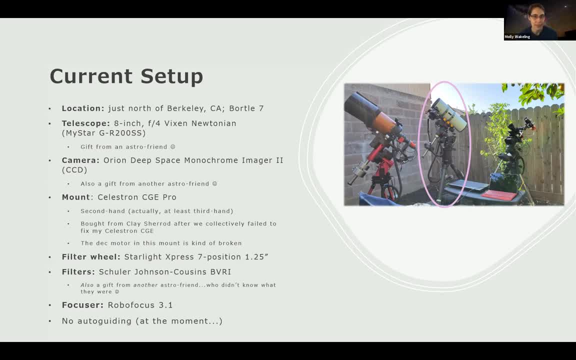 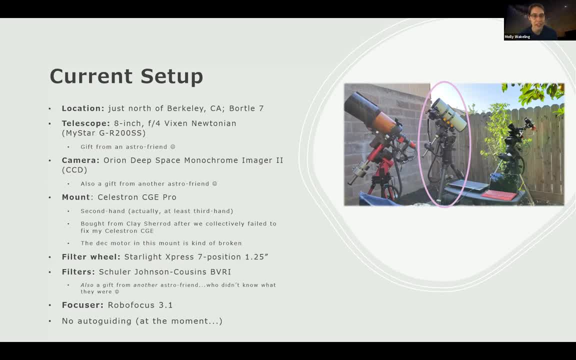 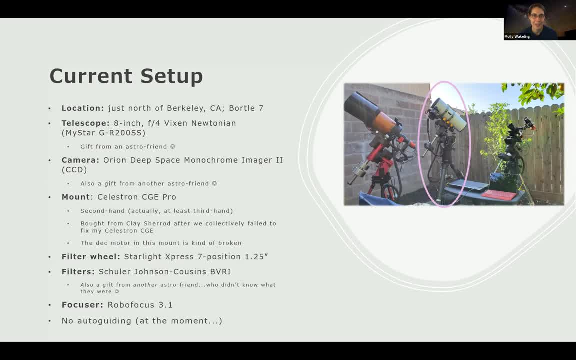 they were. i posted on claudia nights about them and somebody was like, oh, those are photometric filters, you want to sell them to me. i'm like, no, those sound really cool, i'm gonna hold on to those. and now i've been able to use them. so that's been really neat. uh, i know astrodon sells some as well. 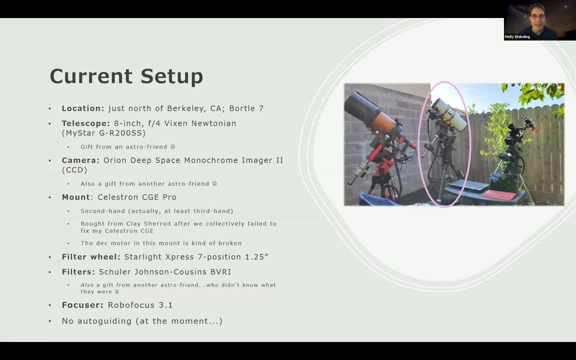 um, but yeah, that they'll be coming up later in the webinar about what these filters are, and i have an electronic focuser so that i can have good focus between the different filters and with temperature changes and whatnot, and i'm not auto guiding at the moment. uh, my deck axis. 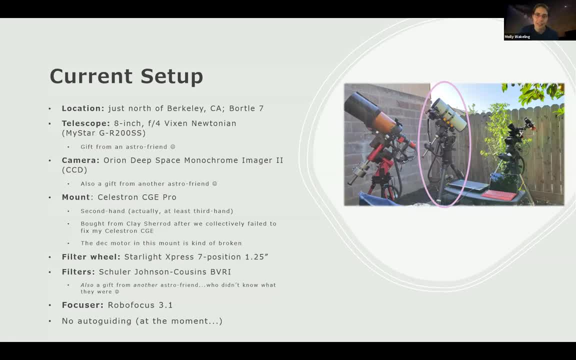 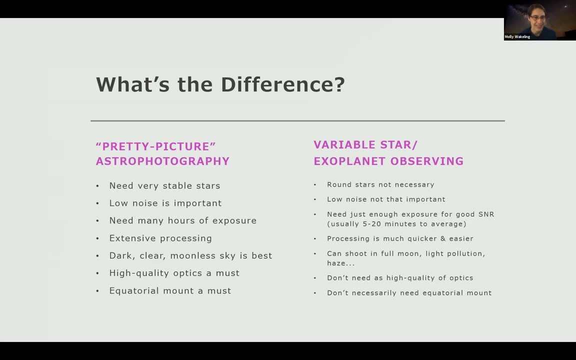 won't auto guide, but i could at least guide the ra axis. but now it's having trouble too, so i might just not guide this one. we'll see, okay. so what is the difference between what i call pretty picture astrophotography and variable star slash, exoplanet observing? 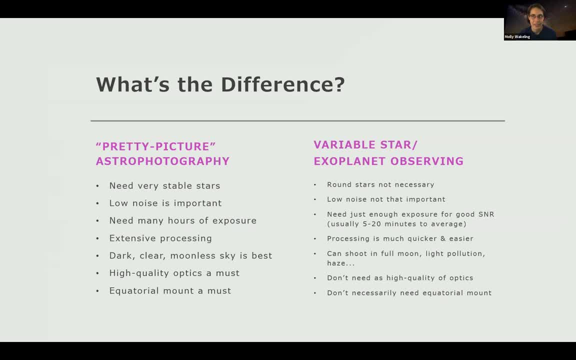 you So for pretty picture as photography. there's a lot of things that you need in order to make a picture look nice. You want nice round stars. If your stars kind of start to streak out a little bit, become elongated, it makes your image look messy. 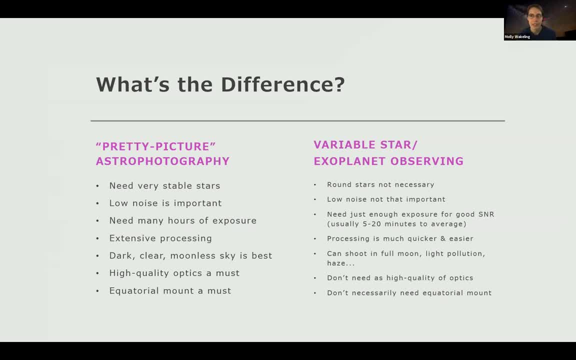 And usually I throw those frames out. You want to have as low noise as possible And we use cooled cameras and lots of processing to process out that noise, And one of the things to help reduce that noise is taking many hours of exposures. A lot of post-processing is involved, getting good at using pics in sight and tools like that. 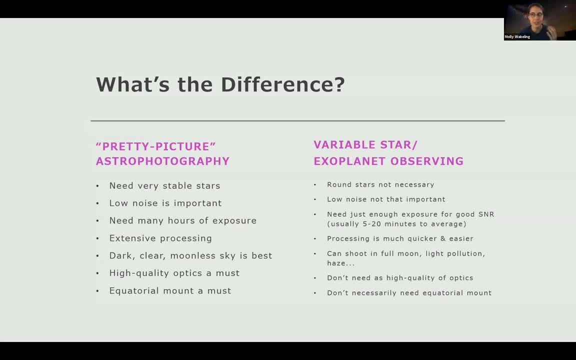 Having dark, clear, transparent, moonless skies are really what you want to use for astrophotography. High quality optics, a mount that works really well, But in my experience so far with doing variable star observing, pretty much none of that is necessary to be able to take reasonable observations. 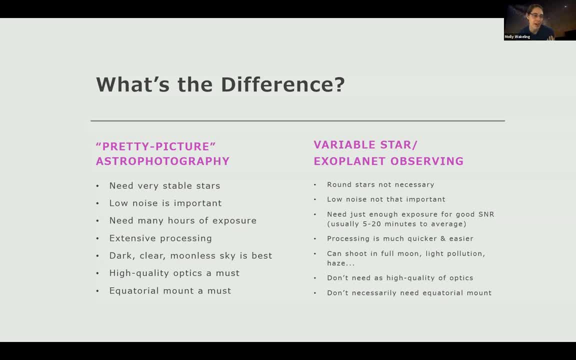 So your stars don't have to be so high, They don't have to be round, They just need to be round enough to be able to plate solve. You know, if they're really streaked out, the plate solver is not going to be able to figure out what part of the sky you're looking at. 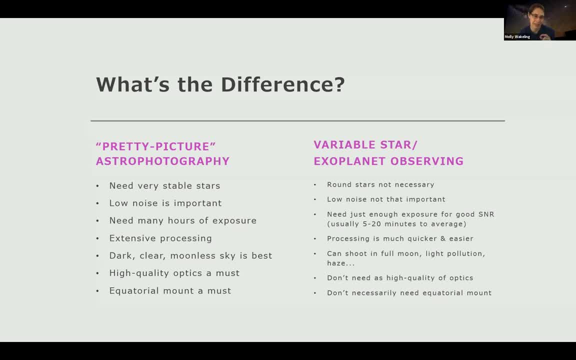 And it can cause some difficulty in processing, but they don't have to be really round. Having low noise is not super important, because you stack a couple of frames and you're still able to integrate over the size of that star and get a brightness measurement. 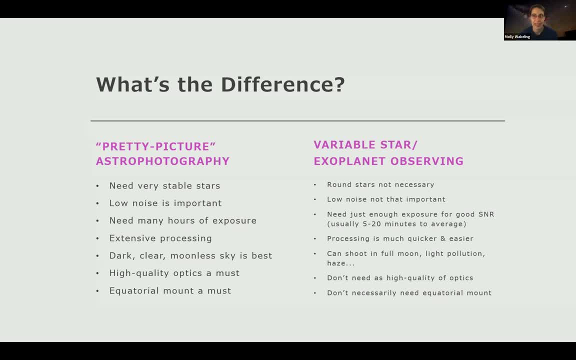 With that noise present, Instead of spending hours on a target, I spend a couple of minutes on a target, especially for one. that's not like a time series over the course of the night. If I'm just taking one observation that night, I'll take. 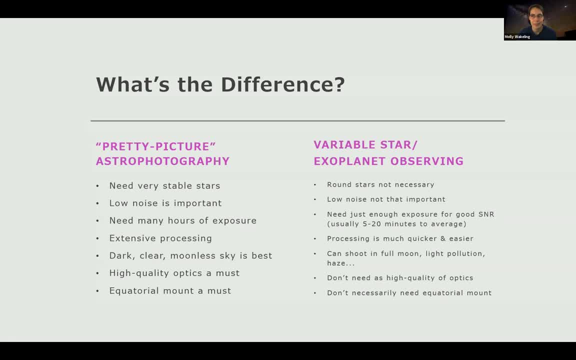 five frames in each filter and that takes about 5-10 minutes. and that's about it, And then I move on to the next target. So you don't need a ton of data on a given target to submit that. data Processing is much quicker and easier. 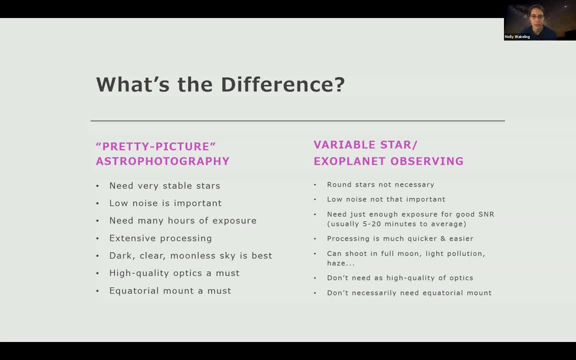 There's not a hard that you have to do. you can shoot through a full moon, through light pollution, through haze, because whatever effects like- like haze or extra light and stuff like that- are on your target star are also on your comparison stars. so The, the, the, the level relative to each other are still the same, which is the important bit. So you can imagine less than ideal conditions maybe, And if you only have one rig, you can spend the. 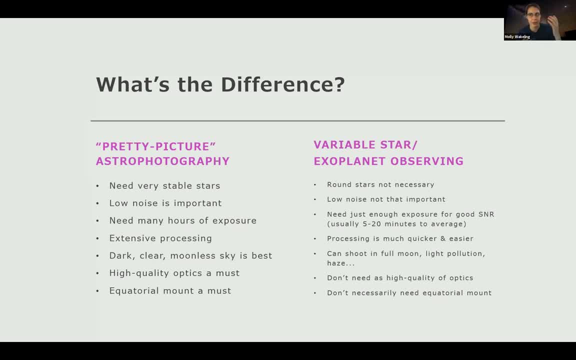 Less ideal conditions than ideal conditions: nights doing variable star observing and the more ideal nights doing pretty picture astrophotography. You don't need as high quality of optics. That Vixen Newtonian, like many Newtonians, has some pretty severe coma, and I'm not even. 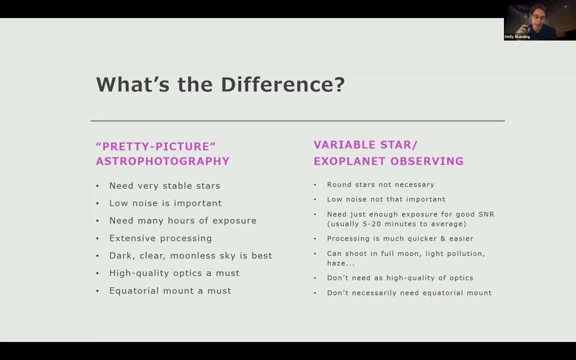 using a coma corrector. I can't quite get the spacing figured out, but the camera I have has a very small chip so I don't even see the coma. but even if I did, having the stars be a little bit elongated is not a problem And you don't. 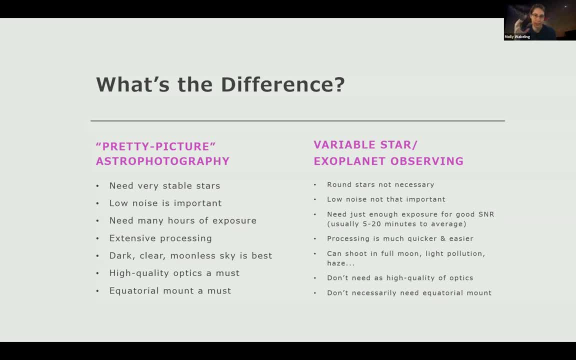 necessarily need an equatorial mount either, because if you're using, if you're only doing five or ten minutes on a target, you're not going to get a whole lot of field rotation and if your star that you're interested in is in the middle, then you don't have to worry about it being cut out by the field. 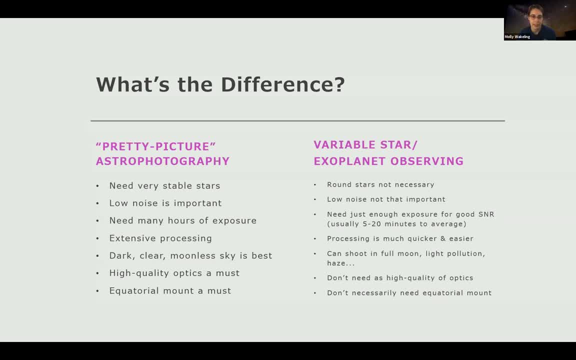 rotation So, and you don't need a mount that tracks super duper well, You can use lesser equipment and be able to get good measurements still. So to kind of see the differences in what those data points are, I'm going to show you a little bit of a 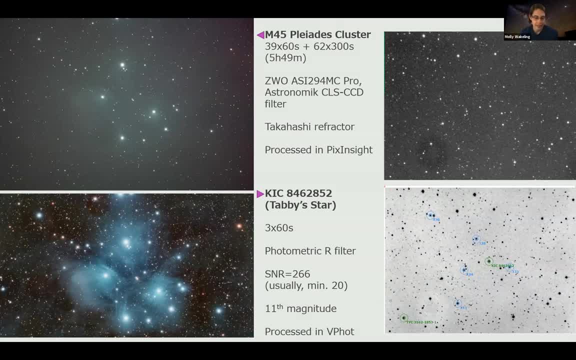 picture of what the data sets look like between astrophotography and variable star observing. Here's just a quick example. On the left is a single frame on the top and then a fully processed image of the Pleiades cluster, and that's almost. 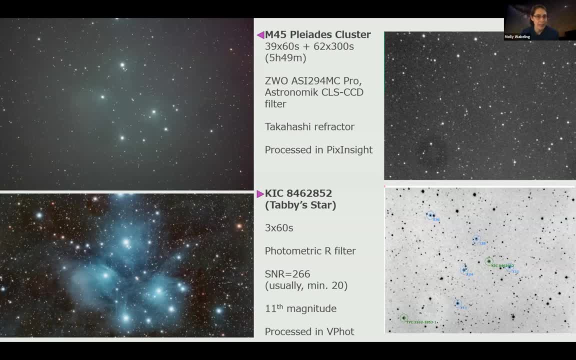 six hours of data with a really nice refractor and lots of processing, And over on the right, the top is a single frame, the bottom is a stacked and inverted frame in the VFOTE software And this is a three minute exposure time using a photometric filter and it's on. 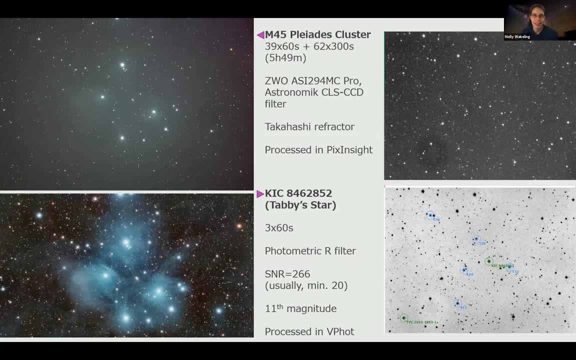 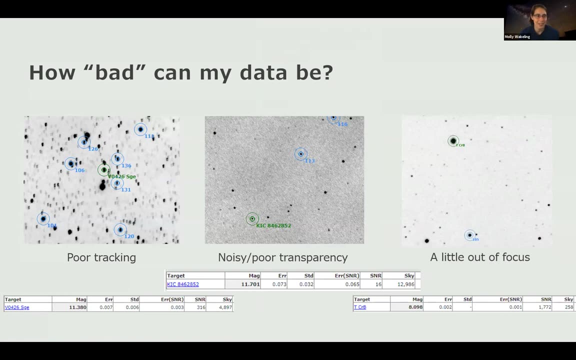 eleventh magnitude star with a really high SNR, even though this camera is relatively noisy. So just to give a visual on what the difference between those two images looks like. So how bad can your data be and still give a reasonable result? These are some less-than-ideal. 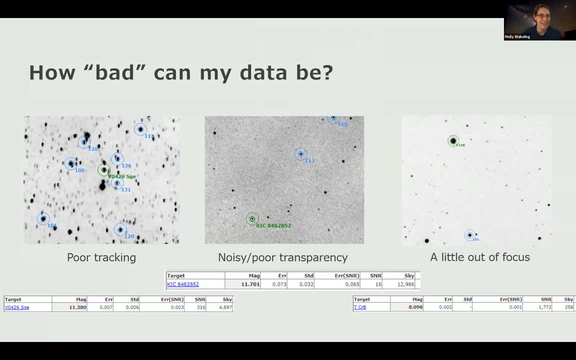 that I still processed and submitted data for. So the one on the left is bad tracking. You can see my stars are elongated. Maybe not the most precise of measurements, as far as the fact that the annulus, the annuli, are circular, doesn't quite match the star. 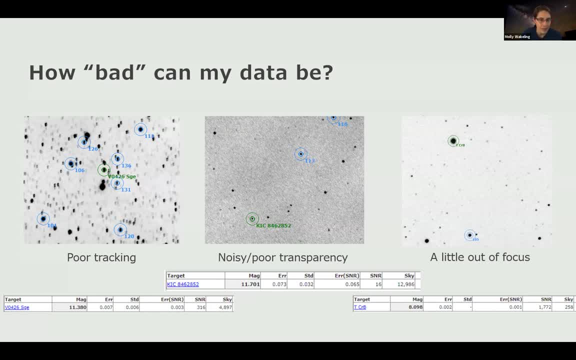 but the error was still pretty low on that one, The middle one. it was a it's a noisy image, The transparency was poor, but despite that it was still. I could still see that 11th magnitude star, that one's tabby star, right there. 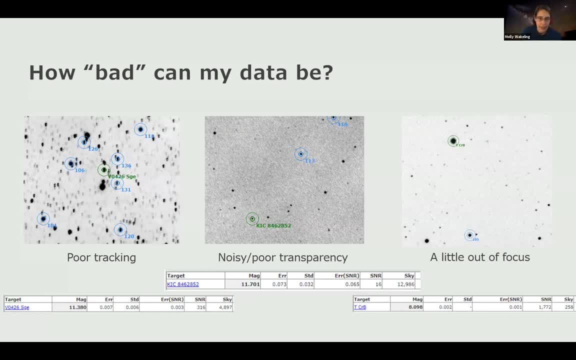 And the comp star is well enough to get a measurement, And if you're actually might wanna be a little bit out of focus from what people tell me, like the one on the right cause, then you have more pixels over which that star is. 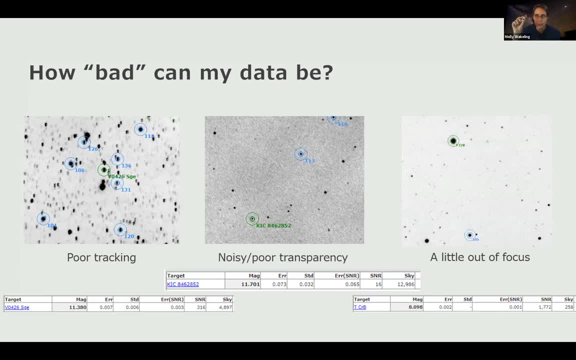 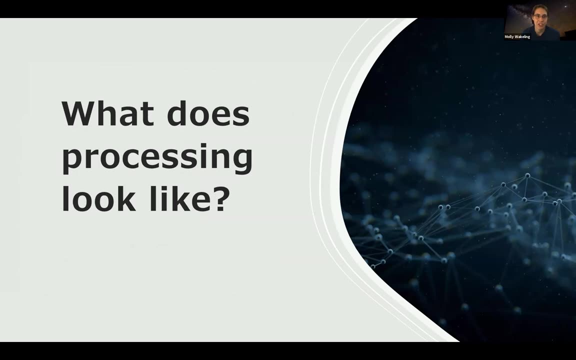 and you can not be as susceptible to individual pixel difference in levels and stuff like that, So it's a little bit out of focus and that actually probably helped make that a better measurement. Okay, so to kind of when we had a, we had Stella Kafka on the Astro Imaging Channel recently. 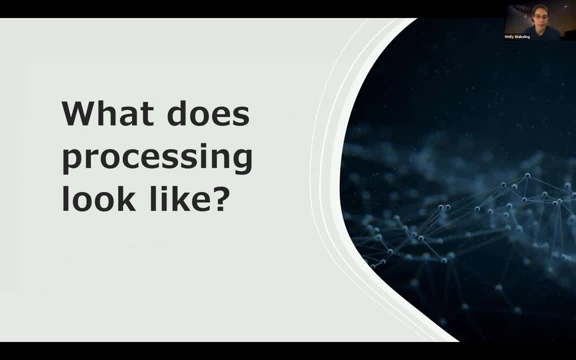 talking about AAVSO and how to submit data, And I think a lot of people were pretty mystified by how you actually process the data and what that whole process looks like. So I'm not gonna go into detail on how to use VFOT. 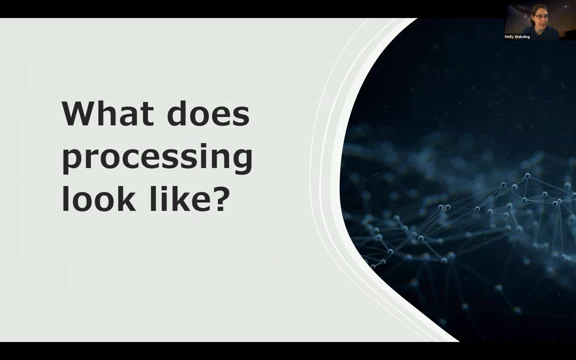 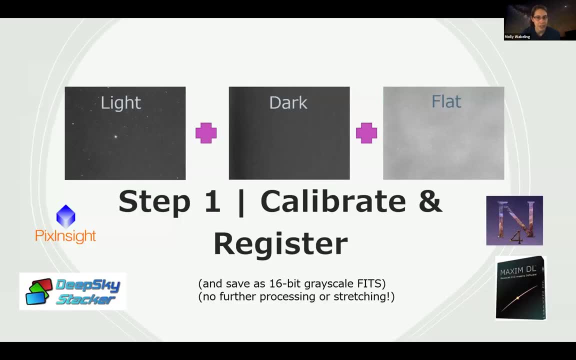 because of time limitations And there's manuals out there for that, But I just wanna kind of do an overview of what that process looks like, just to kind of demystify what all is involved. So, just like regular astrophotography, you still wanna take darks? 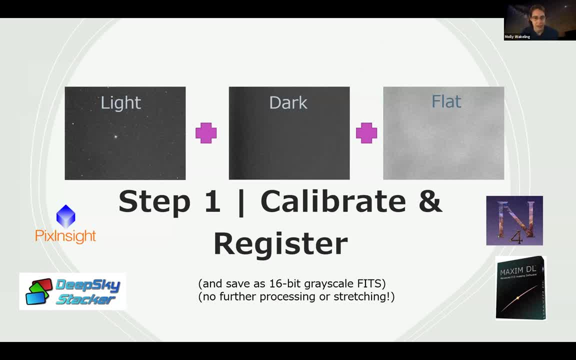 you still need to take darks and you need to take flats in order to have a more accurate measurement, And I calibrate my light frames in PixInsight. still, You can use whatever software you already use for doing the calibration And you need to save it out as a standard. 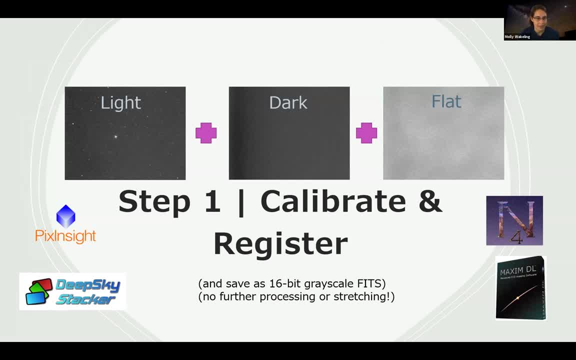 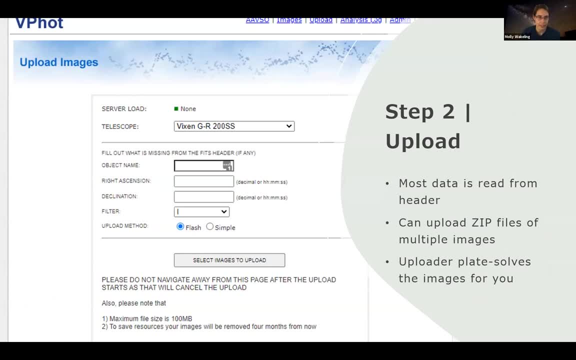 You can save it out as a 16-bit FITS file, because VFOT doesn't like 32-bit for some reason. But you don't even wanna do any other processing on it, Just calibrate And then upload those FITS files to VFOT. 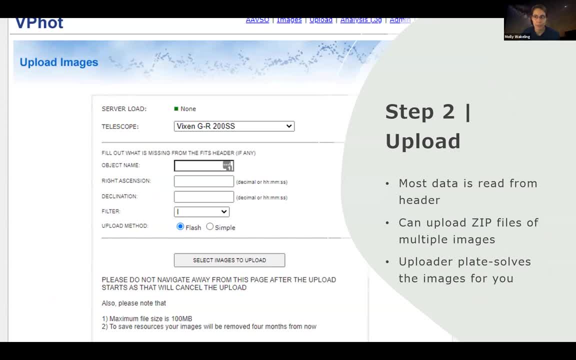 And you can actually do that as a single zip file, And it pulls all the relevant information out of the header. I have to specify which filter it is, because I call them different names than their standard names. But yeah, that's all the information I have to provide. 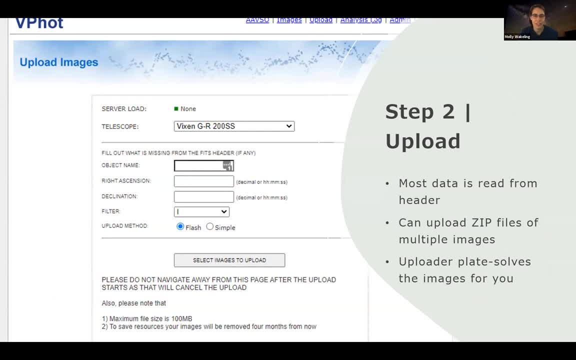 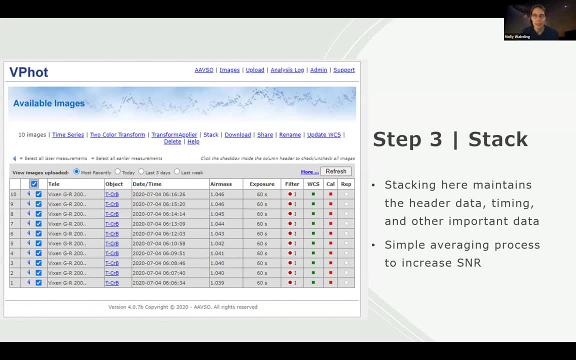 It is what telescope I used and the filter I used, Because all the rest of the information is in the header. Then I stack the images in VFOT, because that way it preserves the timing information, which is important for knowing the air mass and some other things that it uses. 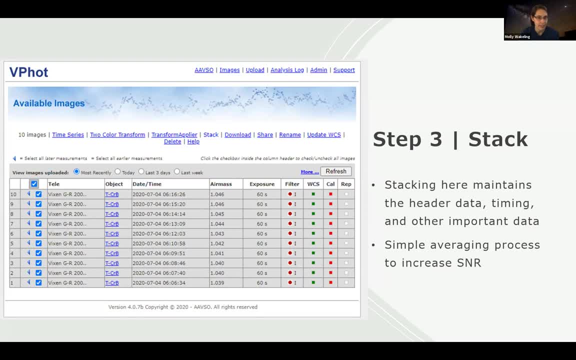 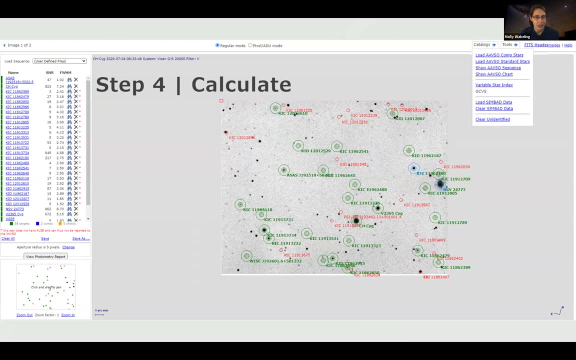 to calculate the magnitude of the star. So here I have several IR filter images on TCRB and I stack them in VFOT, which is really just an average. It just averages them And then the next is the calculation steps. So you click on that stacked image. 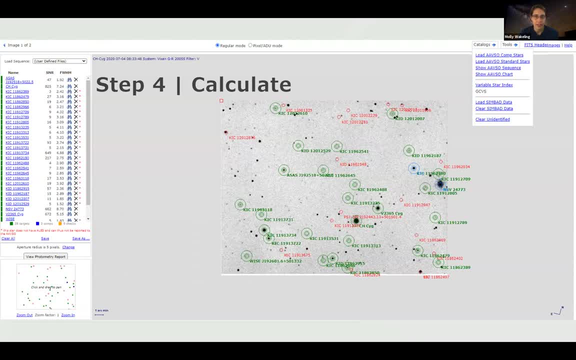 and you click on a variable star index, or GCVS, And it's already plate solved your images, So it goes through and highlights those stars for you And then you delete all the stars that you're not currently interested in making a measurement on. 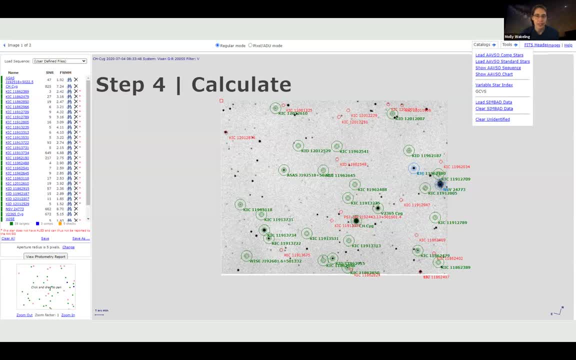 And then also have it. it's got a list of comparison stars for all the variable stars that are in the database, So it will find those for you. You don't have to go through and identify what star is which or anything like that. 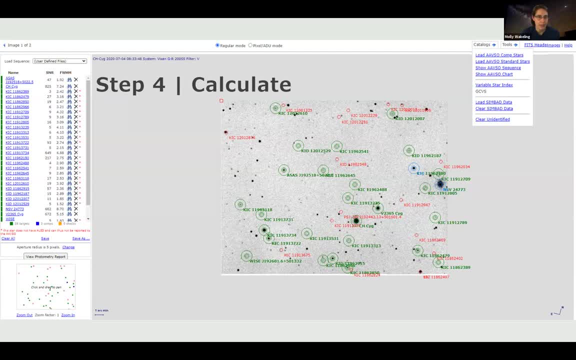 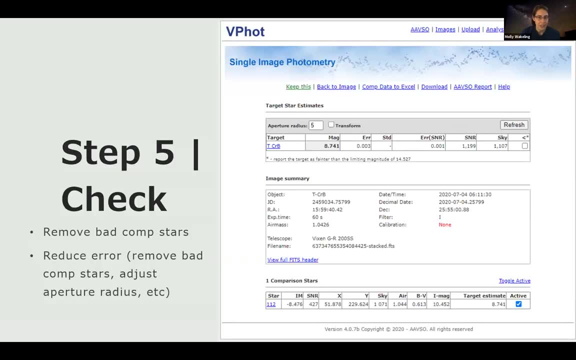 And then you just a couple of other parameters to get a good measurement on the size of the annuli and things like that. There's details on that in the manual. And then you check to make sure that the error is low and none of the comp stars are far away. 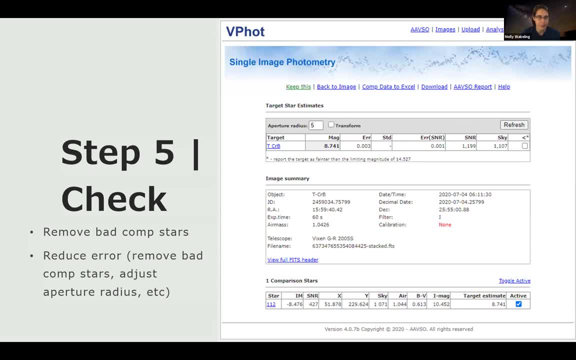 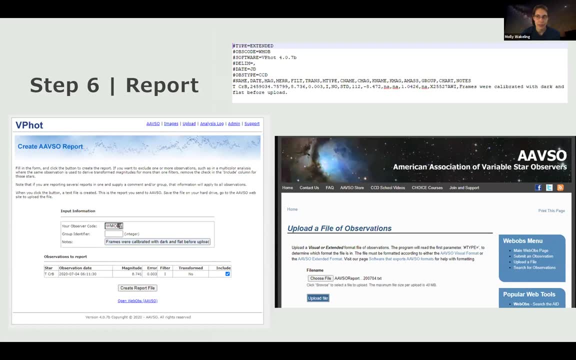 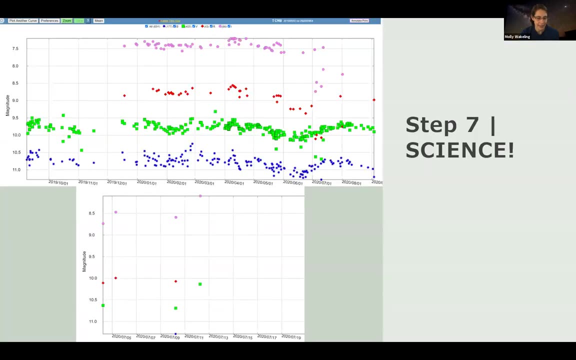 from their true values, so that you know you have a good measurement. And then you hit the generate report button and it spits out a text file that you then upload And that's the whole thing. Probably takes about 20 minutes And that's your submitted observation. 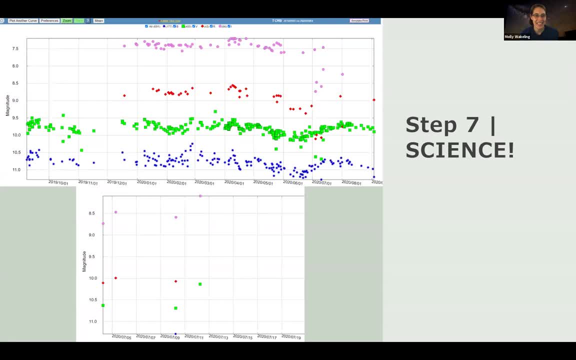 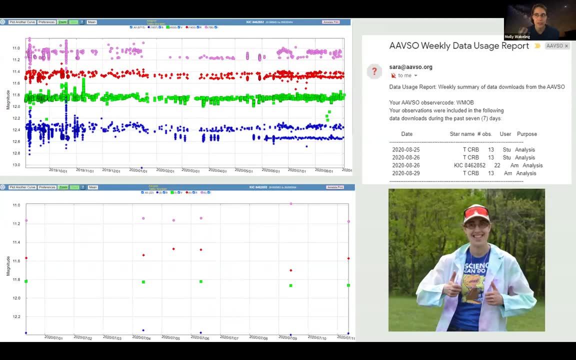 And you have done science. You have contributed to the scientific community. Your data shows up in the light curve generator on AAVSO And people who are doing research on variable stars can download those data sets and your data is a part of it. 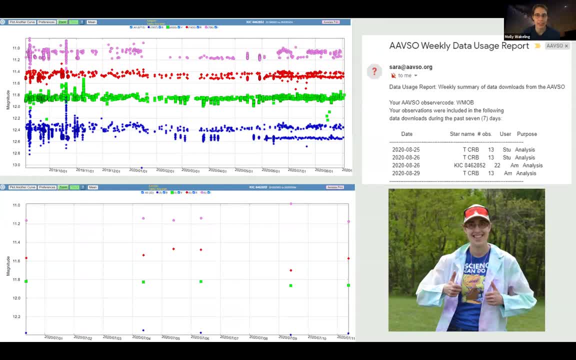 And every week you get a summary email on which of your data sets have been downloaded. So it's really cool to know that you've participated in the advancement of science and getting to participate in that. I get to do it in both a professional and an amateur capacity. 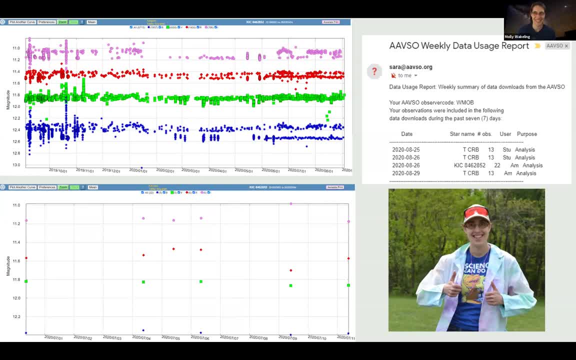 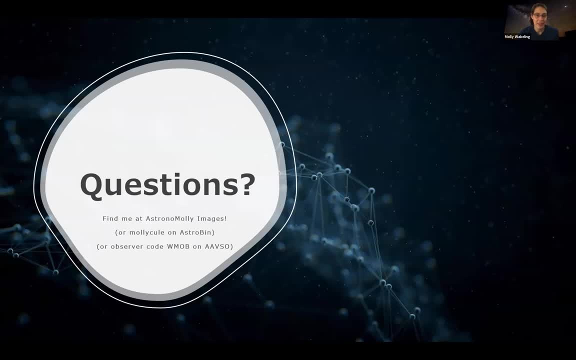 doing two different kinds of things, But yes, you have contributed to the doing of science And I guess we're gonna do questions at the end, So you can go ahead and throw the questions in the Q&A so that you don't forget them. 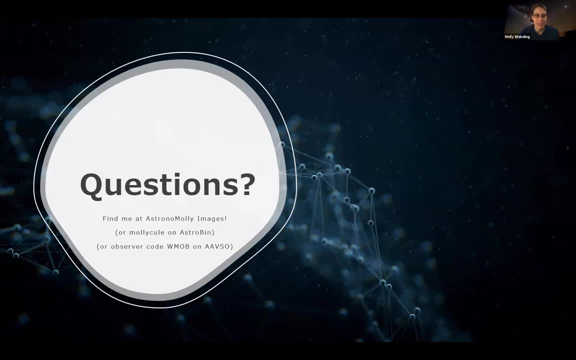 And if you wanna follow my adventures and misadventures, I am on social media as Astronomolly Images and I'm on Astrobin as Molycule, or my observer code is WMOV And yep, thank you, Thanks, Moly. 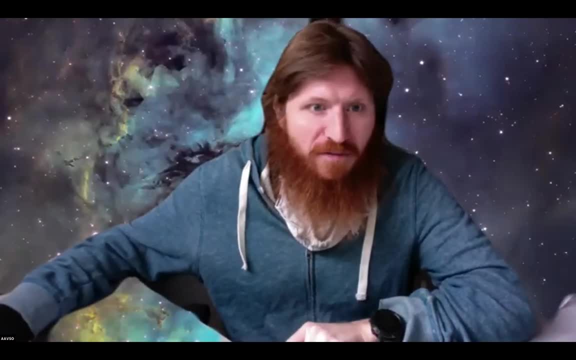 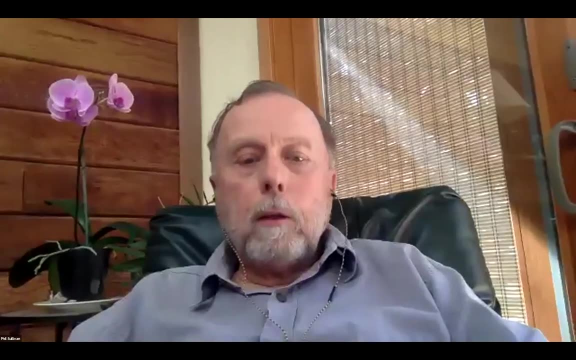 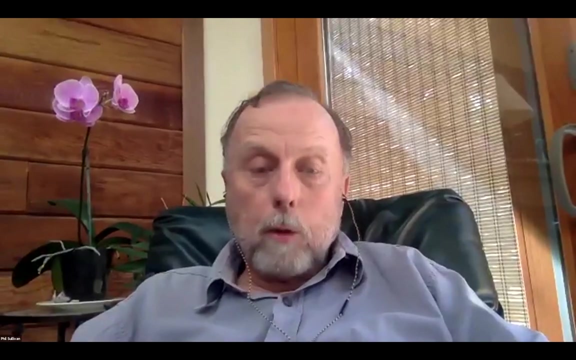 Next up we have Phil, who's going to be talking about photometric filters. Okay, my name is Phil Sullivan. I've been a member of the AAVSO for quite a while. I do observations From my own observatory and I also use the AAVSO network telescopes. 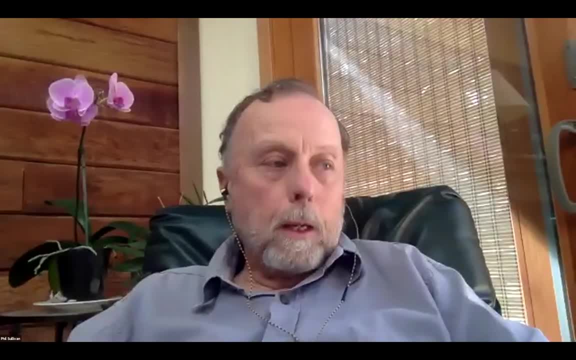 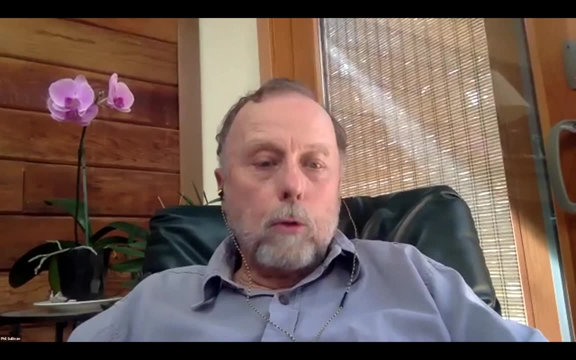 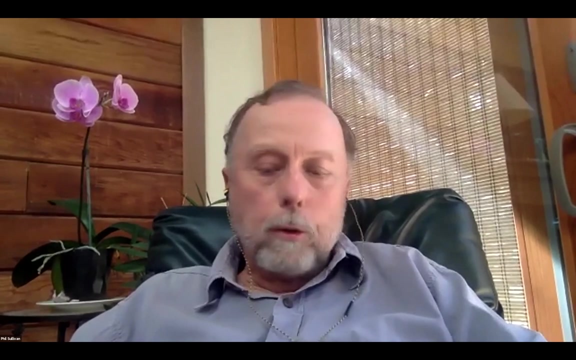 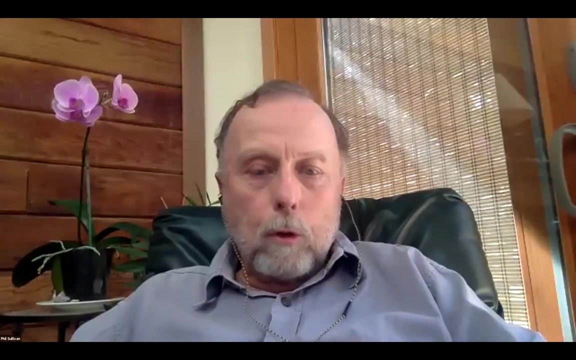 And I also teach photometry in the choice courses. My discussion is gonna be primarily directed at people who are transitioning from astrophotography to photometry, and also for beginners. I don't have time to do everything I wanna do, so I'm gonna refer you to a spot. 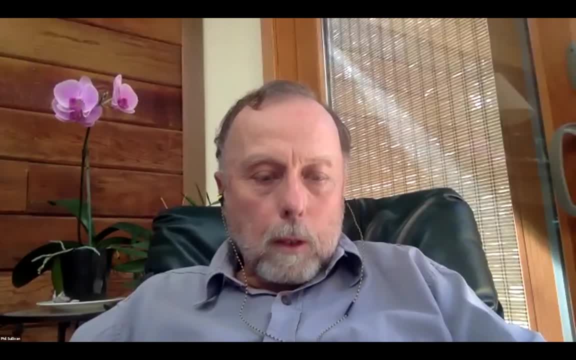 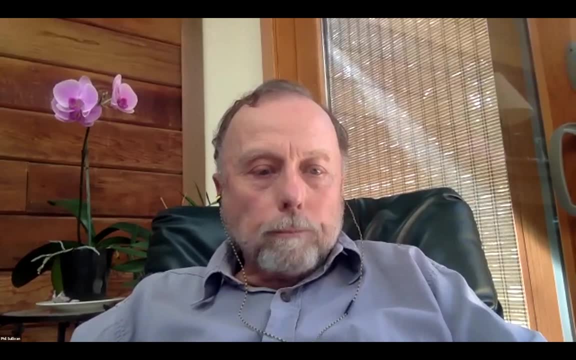 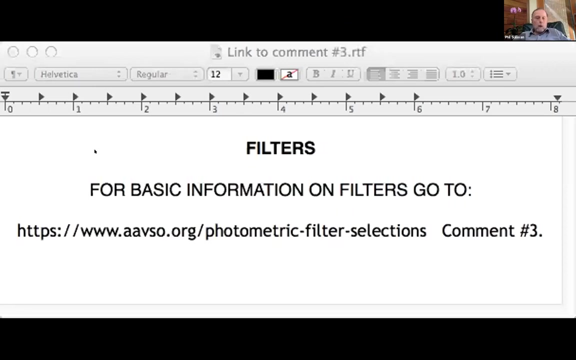 where I had an extension post. See if I can find that slide. There we go. If you want the basics, go here. I'm gonna leave this up. I'll put my notes there. I'm not really familiar with all the technicalities here. 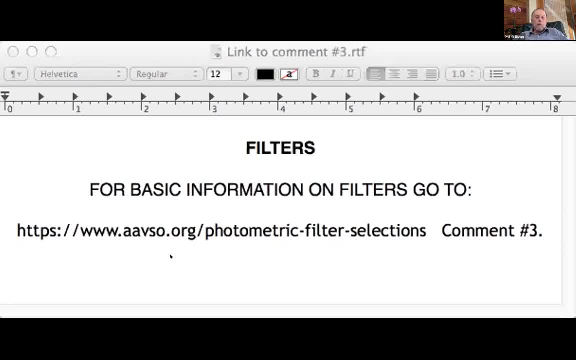 This is a link to a forum post where I kind of condensed all the things I thought were important for really beginners And I'll leave that up for a while. I really wanna get to three basic issues with filters. There's been a lot of going on with filters recently. 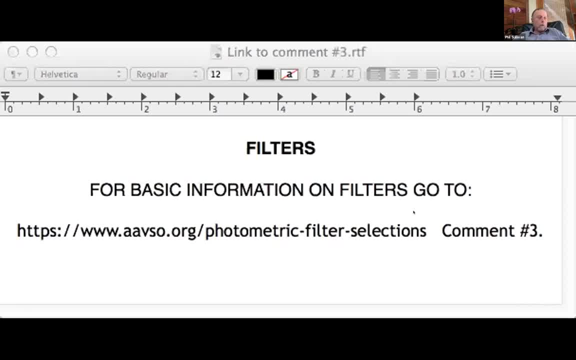 and not all of it is good. The first question is: do you really need to buy these filters? And for a lot of people, I think the answer is no, at least for beginners, As you get more serious and you get more experience. 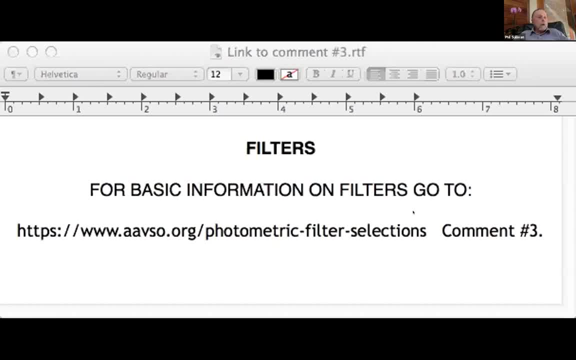 you're eventually gonna wanna get photometric filters, But for starters, if you have a RGB set, you can use the green. Green works very well as a substitute for the photometric V If you look at the transmission curves for V and G. 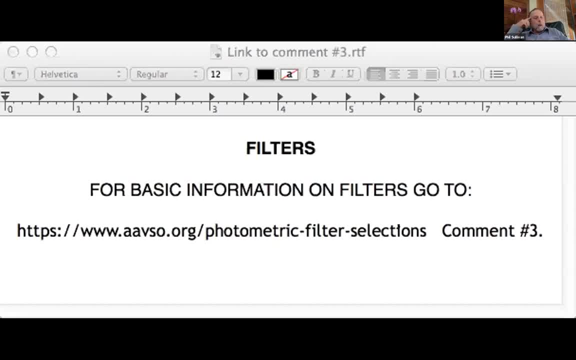 they're very, very close Now, so you can get your experience and get started using the G filter and you can do good quality of photometry with the G filter. The only problem with using a G filter: you have to limit your targets to what is called non-red. 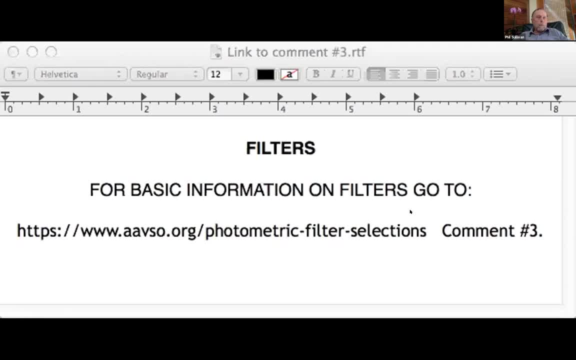 which is probably something with a B minus V of one or less. If you should use non-red stars, you'd do very well. Eventually, there's a process you can do called transforming your G filter to V filter, but that's something that's more advanced. 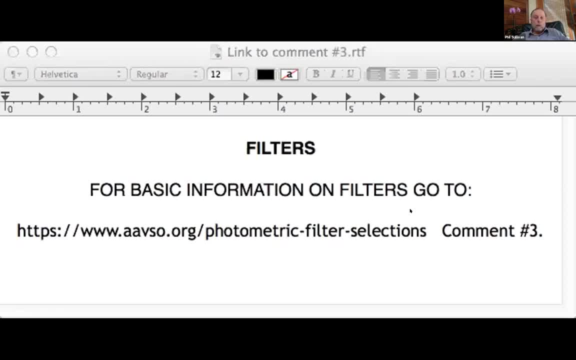 and I don't think I really wanna get into that, but there may be more discussions about that in the forums. The real goal is just get started. Start using your G filter as if it were a V filter. Start getting practice. Submit your measurements to the AVSO. 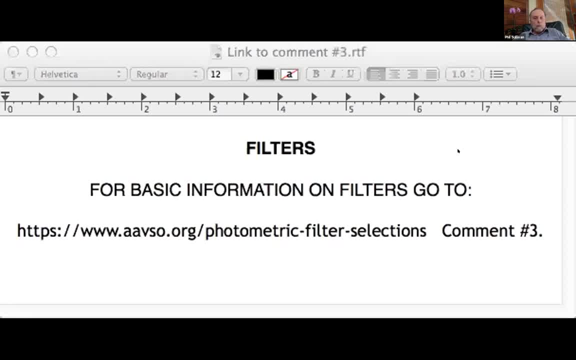 You're only gonna know how well you're doing when you can compare your own measurements with other people's measurements. So submit your data. If you're using a G filter, you have to submit your data, Identify your filter as TG and then see how you're doing. 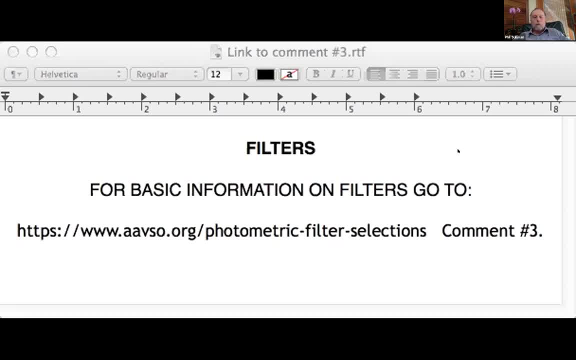 And don't be worried about it if you submit something that doesn't look quite right or looks really, really bad, because it's very easy to remove what you think is a bad data point without any fuss. Okay, so there are also a few things you can do. 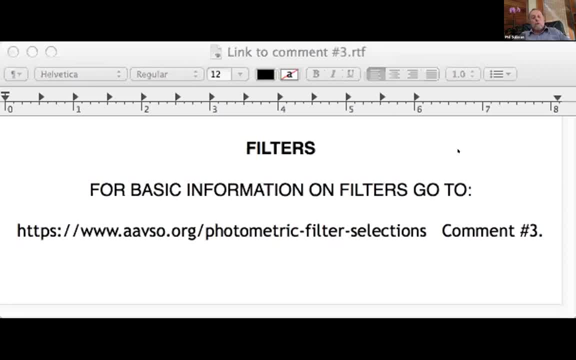 Okay, so there are also a few things you can do. Okay, so there are also a few things you can do. There are a few things you can do without using a filter at all, but I don't have time to get into that. 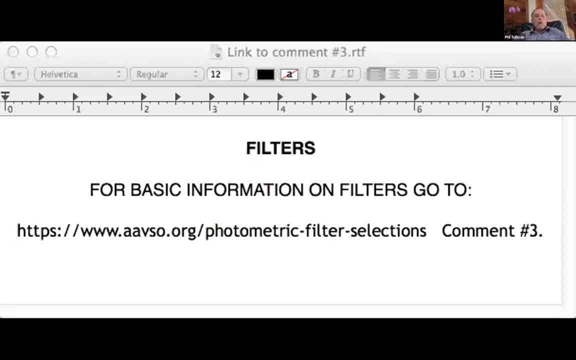 What I wanna cover next is what you need to know to make an intelligent decision about buying filters. There's two basic ways to make these photometric filters. I'm gonna be referring only to the Johnson-Cousins photometric filters. There's two ways to do it. 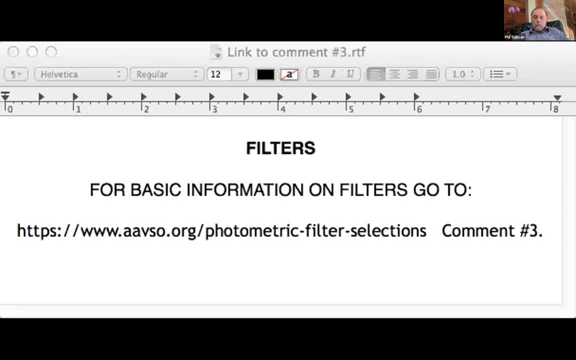 You can make them out of colored glass, where the photons you don't want it to come through are absorbed by the light, or you can do it by multiple optical coatings, where the interference effect causes gives you the filter effect. This is: can everybody be able to see this? 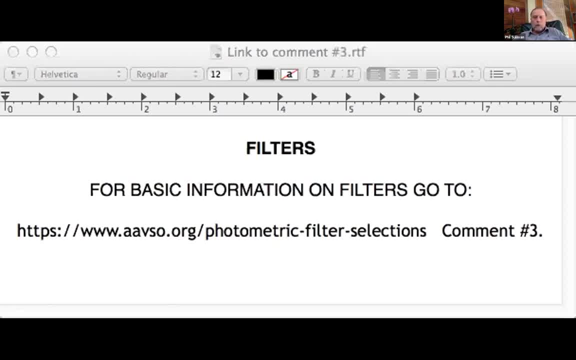 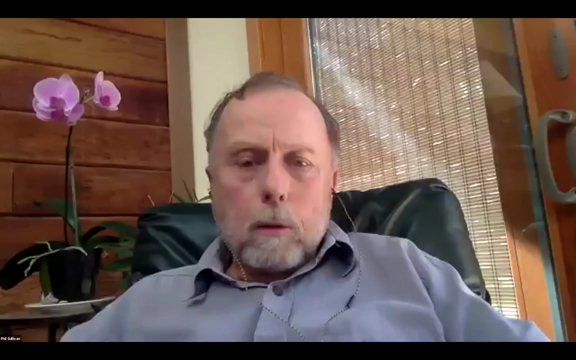 Johnson-Cousins filter. Okay, I'm gonna screen share here. That's showing up. You'll need to stop your screen share and do the thing where you select your desktop instead of the single window. Oh, stop screen share. Okay, here I am again. 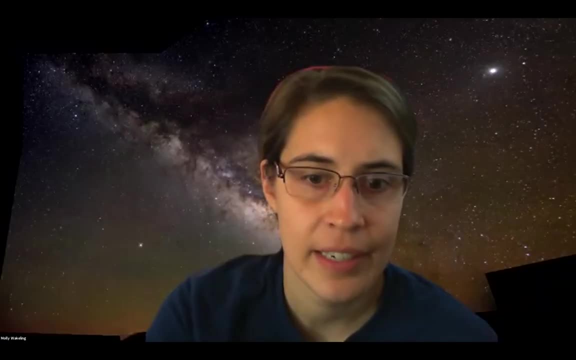 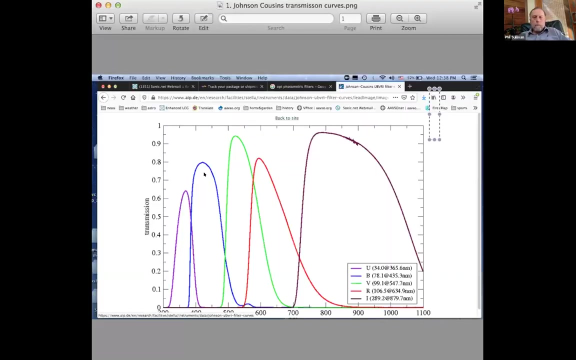 Now let's go screen share again, Yeah, and then hit that first icon. It says desktop. Okay, Here's what I wanna show. Is it there now? Yeah, Okay. Okay, these are the transmission curves for the Johnson-Cousins filters. 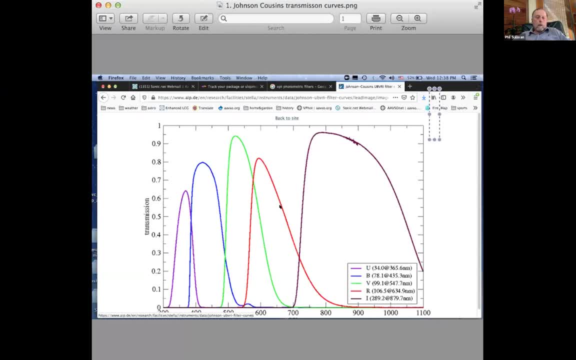 U B V R and I Notice a couple of things with this. Notice how close And how much overlap there is between the V and the R. Also, the peak transmission is pretty close in the B and V. There's less overlap. 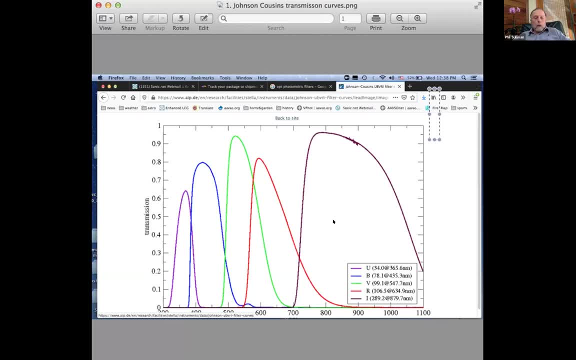 and there's more distance between the peak. This is I. the maximum response to most silicon detectors, CMOS and CCD is in the R. Notice this little bump down here. This is the blue filter And a little bit of sensitivity all the way into R. 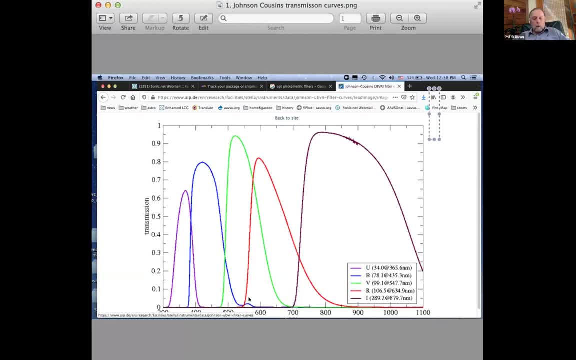 We may end up having to talk about that a little bit later. That's could be an important thing. Okay, So in the, in the, in the, There's another kind of filter, a series of filters that you need to see. 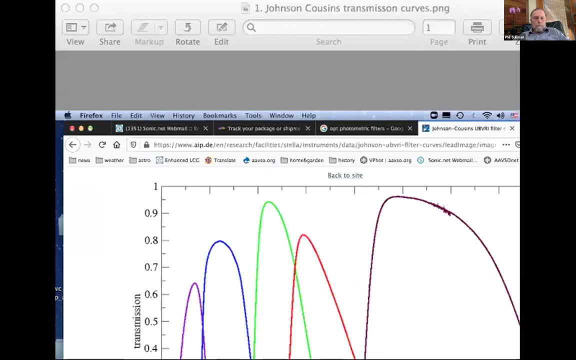 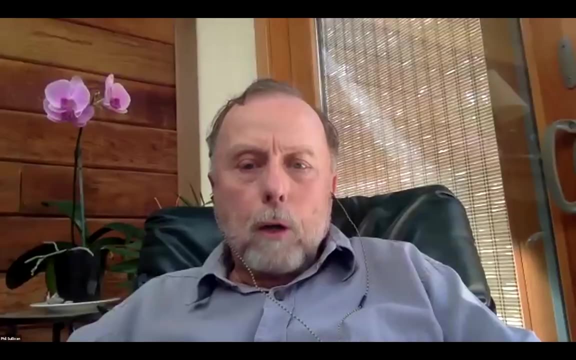 Is it showing up? So I think when you shared your screen this time, you clicked on this particular image, So you'll have to stop sharing again and switch over. Okay, good, Thank you. Stop sharing. Okay, Screen share again. 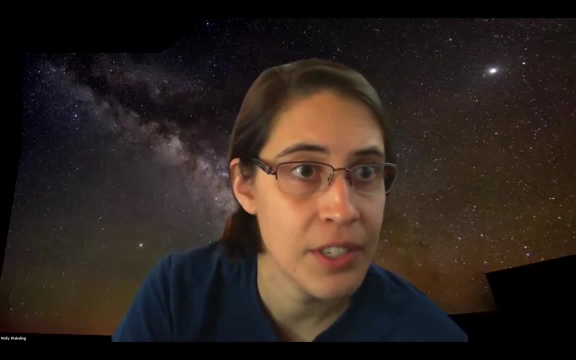 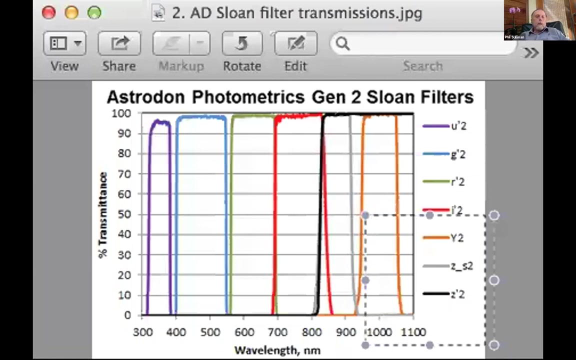 Or just pick your whole desktop, Then you don't have to do the start-stop thing, or that. Is this showing up? Yes, Okay, So these are the Astrodon Sloan filters. These are mostly used by professionals, But you should notice that they have a very different. 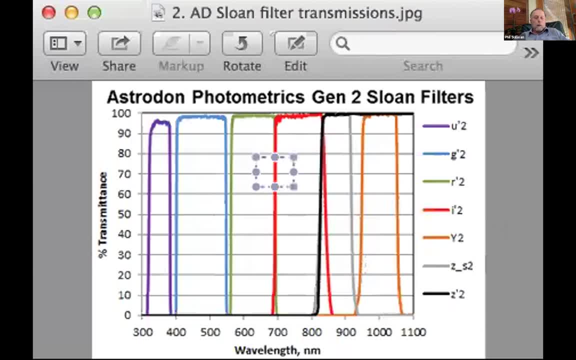 Pattern than the Johnson-Cussin filters. They have these vertical Sides and a very flat top. This is a hallmark of the Sloan filters and also of a. You can only do this with interference filters. Okay, Now I'm going to have to tell you a make. a very bold statement is that I think that the Astrodon filters are the best, and these are the ones that have been used the most in a for a long period of time in the AAVSO, and I've done some testing recently. 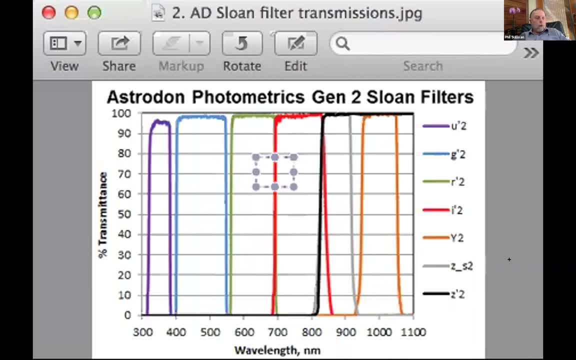 The Astrodons still are Okay- In my opinion, the best. Recently, however, actually about three years ago, the Astrodon was bought out by another company and called Optical Structures and also bought out a bunch of other small Amateur astronomy sites like LumiCon, JMI, Farpoint. 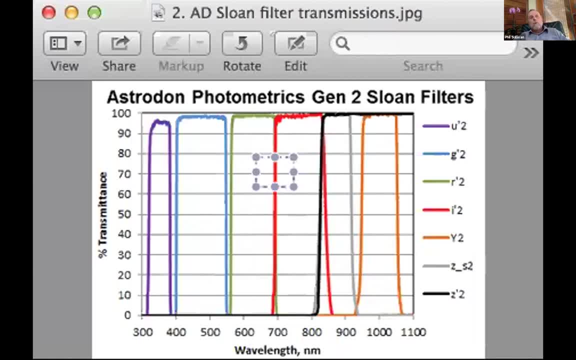 After this happened, the Astrodon filter started drying up, The access was getting difficult And actually at one point Astrodon stopped producing filters completely. There was no production from Astrodon. Now recently they're starting to come back again And this is very promising, because a lot of people thought that Astrodon was the best filter maker was going to go under. 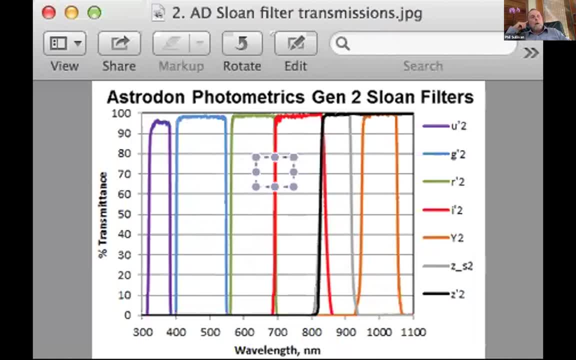 But now people are starting to get them again. But you have to understand that if you're going to order Ashton filters, you're going to have a long wait, measured in months. I'm going to talk a little bit about the Bader. 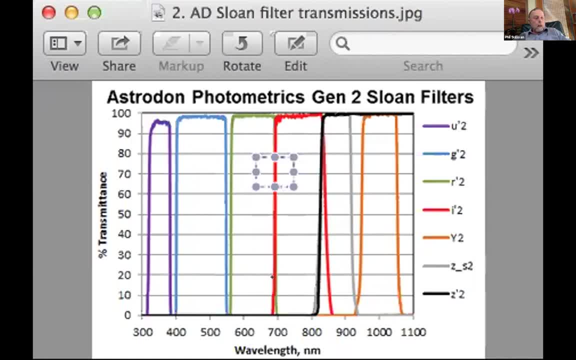 filters. These are made in Germany. They have a good reputation. They are actually made as a combination of the glass, colored glass filters and coatings. But the problem with the Bader's now is that they're going to stop making them. They put it on their site that they're no longer going to be. 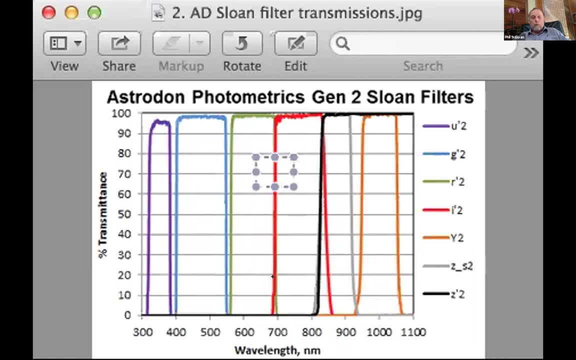 making Johnson colored filters. They're going to switch over to the Sloan filters, So this is a certain. this is a consideration. If you want to get the Bader filters, you better buy them soon, because when the stocks are gone, they're. 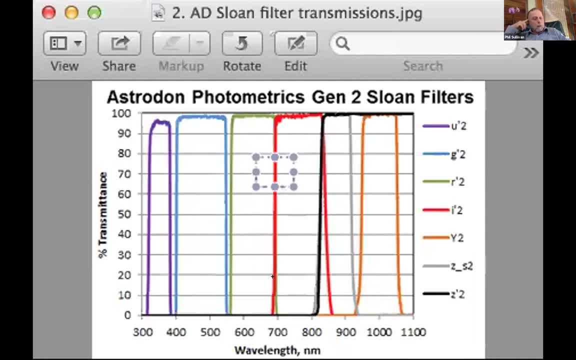 not making any more. The Bader filters are five millimeters thick. This is pretty unusual. Most Bessel filters are the glass. the colored glass filters are called Bessel filters And they're generally four millimeters thick, and the interference filters are three. 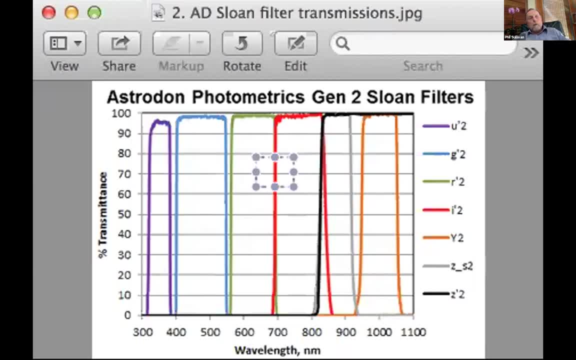 millimeters most of the time. It'd be very nice if you had your filters all the same thickness, because then you don't have to refocus between the filters. Recently, some so-called Bessel filters- that is, Bessel means colored glass filters. 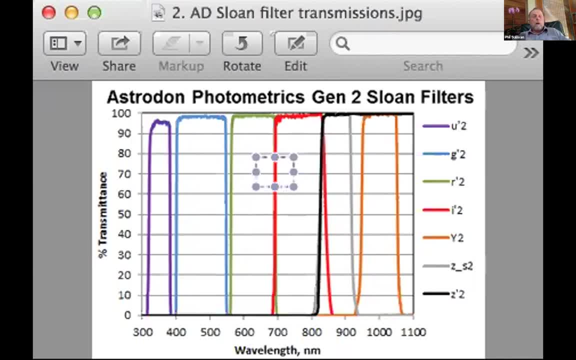 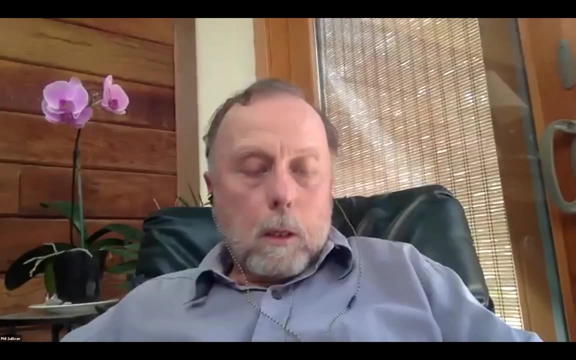 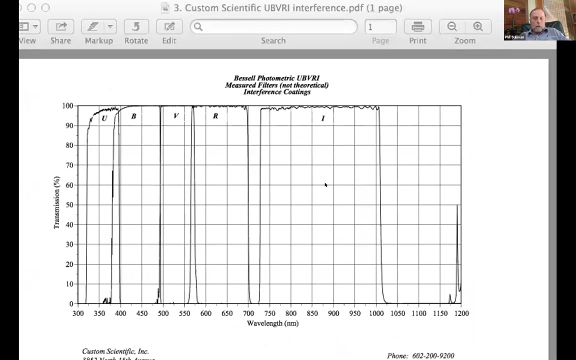 started showing up under a couple of different brand names. But the problem is, if you look at the transmission curves, they're not. I'm going to stop and start again here. Okay, Now there is. are we seeing this? Okay, These, this is the transmission curves of these. 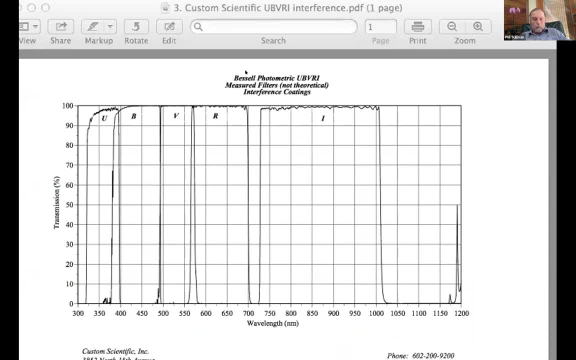 new so-called Bessel filters Here. it says right here: Bessel phonometric UBVRI interference coatings. This is an oxymoron. Bessel filters are colored glass filters, But these have shown up under a couple of different names recently. 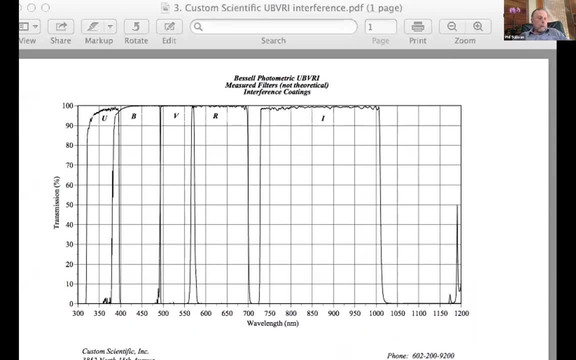 Okay, Okay. So I'm going to say more about this a little bit later. The new- also new- are the Optolongs. Optolongs, I think, have been around for a while for astrophotographers, And I know that there are filters that are used by people who do exoplanet observing. 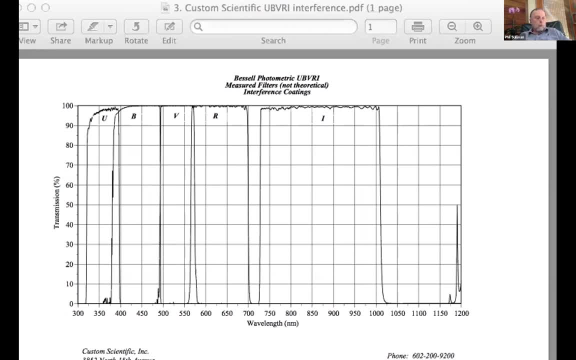 But they're just, they're new into the you know the, you know the, you know the photometry market. So I did some testing on these filters myself. I tested my own Astrodons versus the Optolongs and the Chromas, which are some of these new so-called Bessel filters. 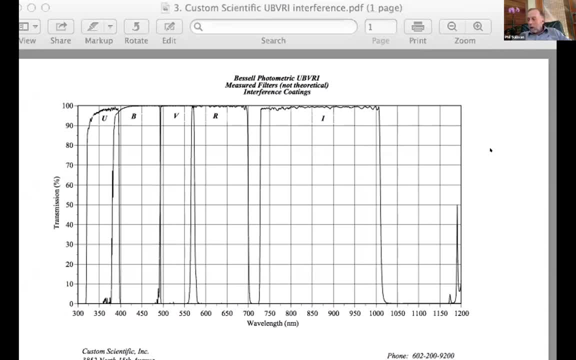 And based on my testing, the Astrodons were superior, The Chromas were average, And then you know more studies from NASA. but you know so on and so forth survived And you know the own-on лет have been a good test. their results you know, at a level very. 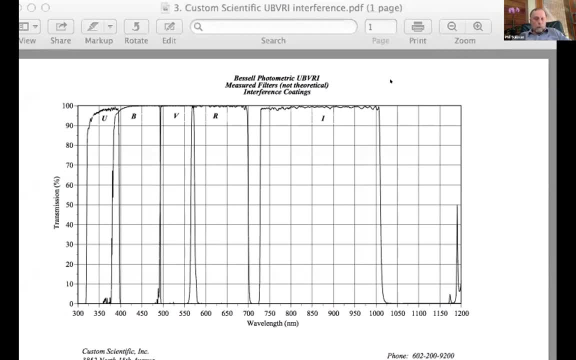 high. so I thought you know both theids were good To me. you know, Tom a过 ved – I just have to say basically I'd like to explore that one more time. These so-called Bessel filters didn't do very well. 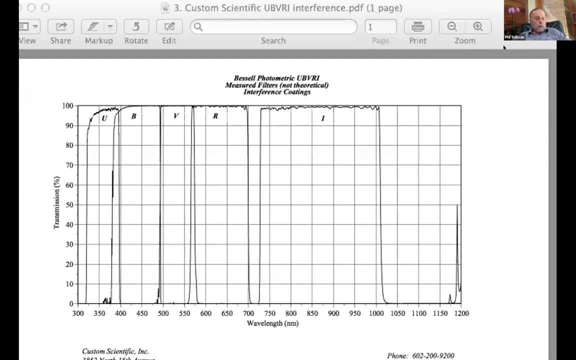 And the OptoLungs did pretty well, So I think OptoLungs are a good option. I think these Bessel filters- so-called Bessel filters- need some more work And I don't think they should be called this. These should be called Bessel filters. 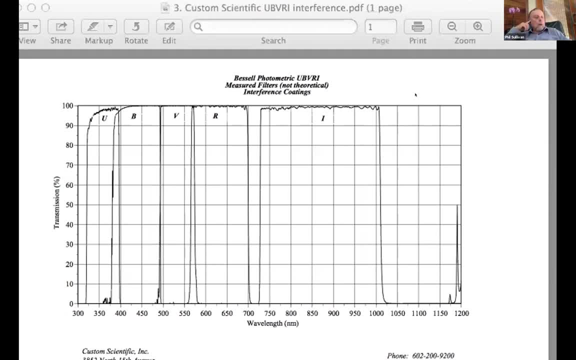 So next thing I wanted to cover is if you go buy filters now, which ones should you consider? And I think it depends on your situation- If you don't have any filters at all and you really want to get into photometry with photometric filters. 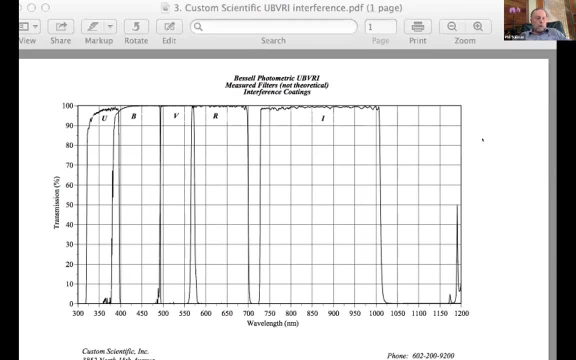 then I'd recommend the OptoLungs. They seem to be decent filters and they're much cheaper than the other filters. Look around, though. the retailers are selling these at different prices. Most retailers will give you the lowest price that they can. 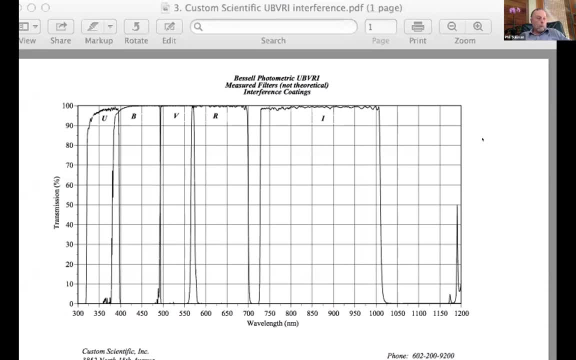 if you've improved that. the other at the low price came from a reputable dealer. When you buy the OptoLungs, you can only buy full sets. This includes a U filter. That's probably not a great idea because you don't. 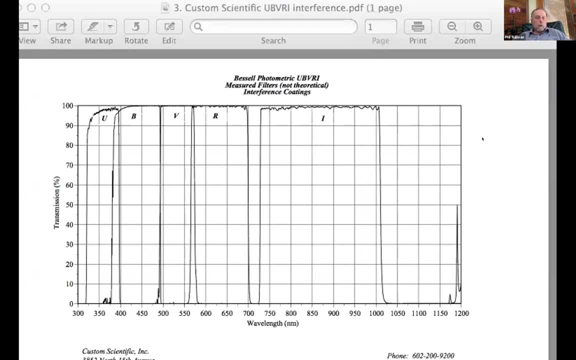 as Molly said, you're really not going to use the U filter. The atmosphere and glass absorbs the U signal, And the only thing that you can use it for actually is, I think, observing Venus. That's the only thing that's bright enough. 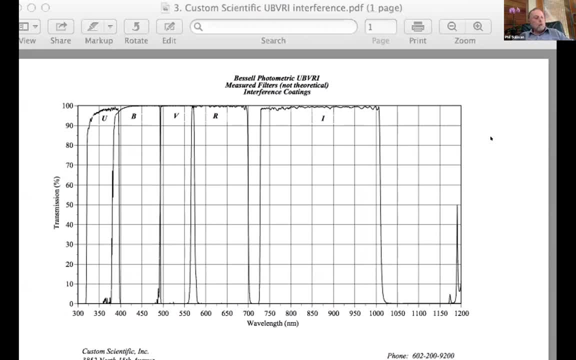 to use a U filter for, And one of these retailers I talked to said that yeah, if you buy the OptoLungs, get the U filter, you can actually sell the U filter, The U filter To the pretty picture people. 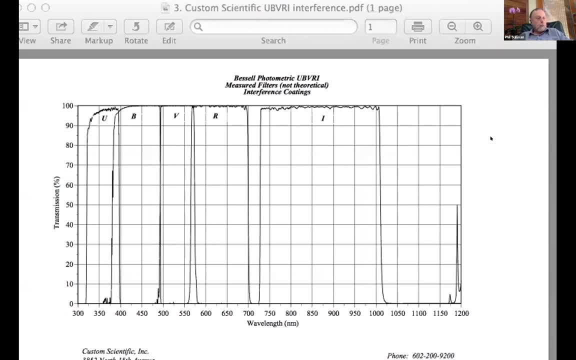 who want to take pictures of Venus. Now, if your situation is that you have the red, green, blue filters, I suggest you just use the green filter for a while, Get your experience there And let the dust settle, because there's a lot of strange things happening. 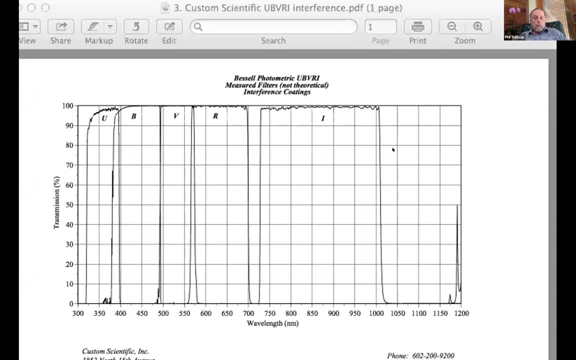 in this market now. But if you think you're going to really use them for the green filter, really be serious about photometry- you might consider putting in an order for the astrogons, At least one in B and maybe an. I Just realize you're going to be waiting a couple of months. at least You got about two minutes left, Okay, But if you don't order direct- but I wouldn't- I would recommend that you don't order from a dealer which is who's going to charge your credit card to keep your place. 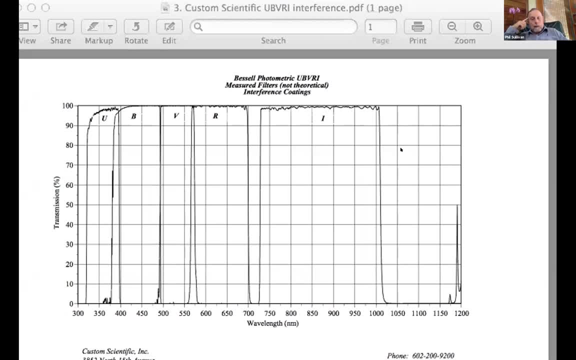 in line. One of them is going to do that And you might be taking a risk because it's not for sure that the astrodon is going to survive, But I really want the astrodon to survive. So I want people to order the astrodons because 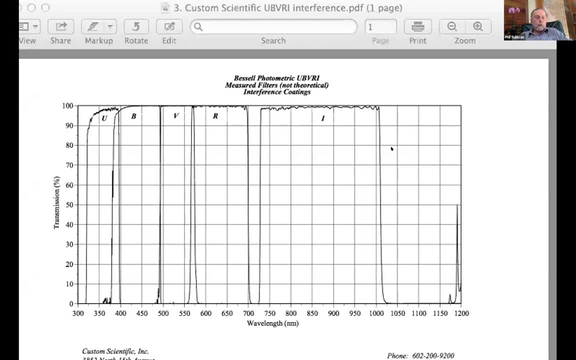 they make the best filters, And if we don't have astrodon, it could be a very sad case. So if you have the batter filter, if you have a batter V, you better start scrambling to get a batter V and maybe an I, because batter is also going out of the filter business. 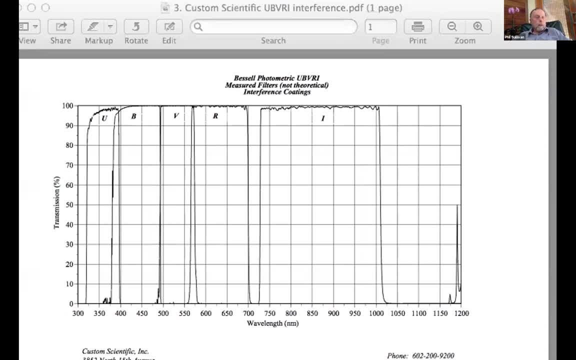 the photometric filter business They're going to. you can, if you can still get them- batters are good filters, I think, And you'll have a better filter. You'll have a fine set, but you might lose your opportunity. 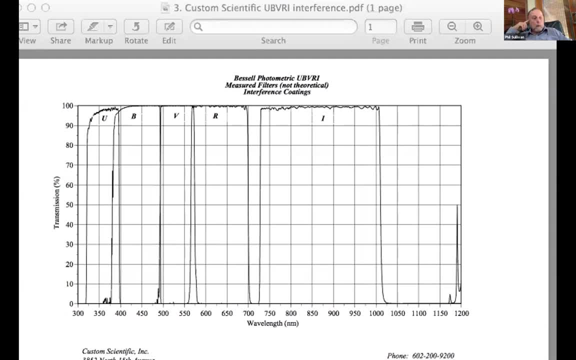 So the cautions: I would avoid the mislabeled Bessel filters. Be careful of anything that's sold as a UBVRI filter as Bessel. you have to check the transmission curves. If it looks like this, I'd get. I'd keep away from it. 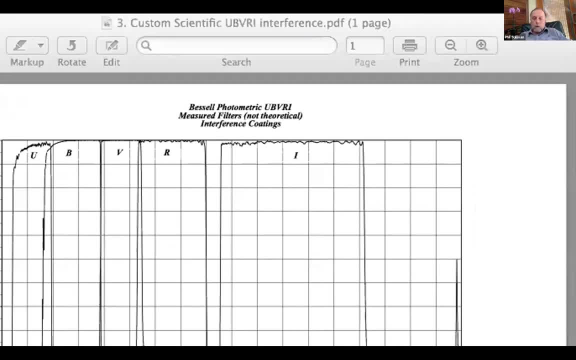 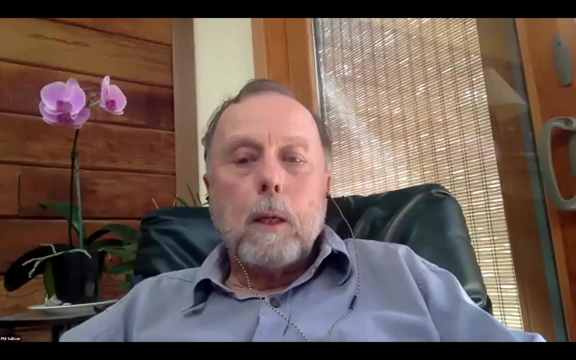 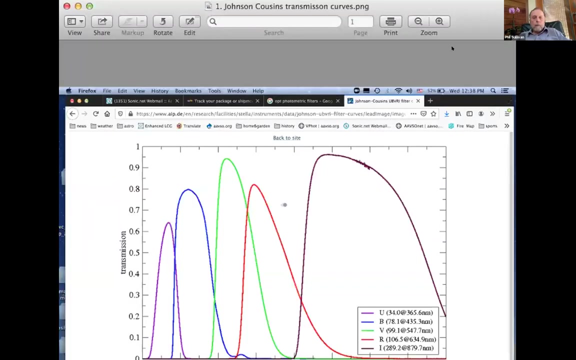 If it looks like this, this one over here, anybody see that, Can't see that. We're still seeing your Bessel photometric slide. Let me, let me start this again here. See that, Yeah, If you have these typical Johnson Cousins filters and they say it's a curves and they 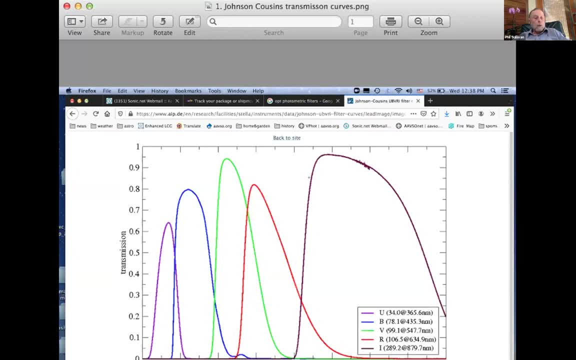 say it's a photometric Bessel filter, you're probably wrong. So if you have these typical Johnson Cousins filters and they say it's a curves and they say it's a photometric Bessel filter, you're probably wrong. Ok, So that's an intuitively fine. 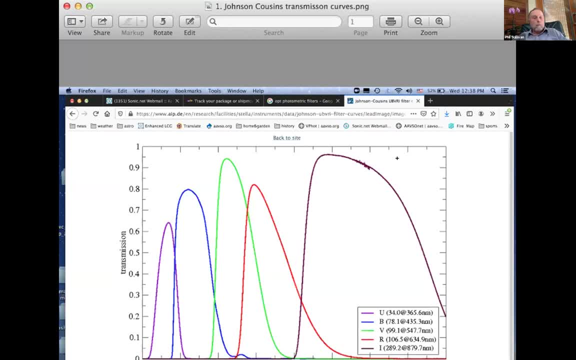 That is a true Bessel filter. If it's got those flat tops and steep vertical sides, it's not. It's one of these pseudo Bessel filters. The problem with those is that in my testing they don't do it very well. 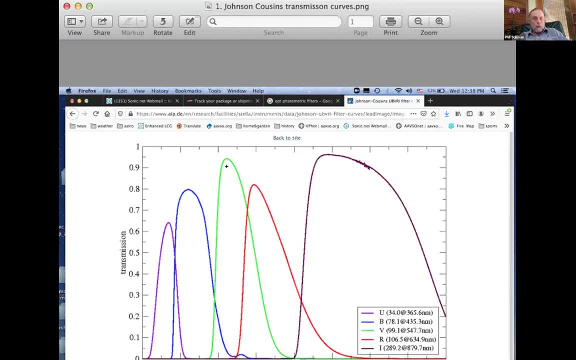 And they're the most expensive filters out there, even more than the Astrodot's Okay, So I hope that's helped. A lot of people have been asking questions about what the filters are, what filters to get, and this market is in influx in chaos. 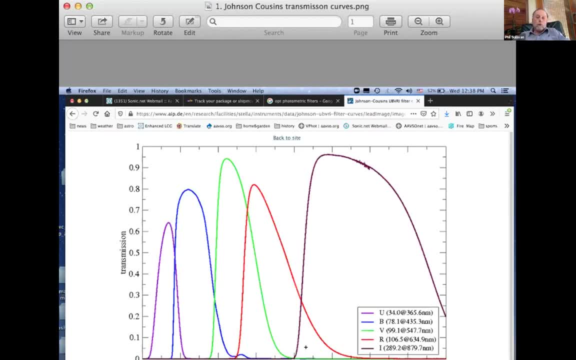 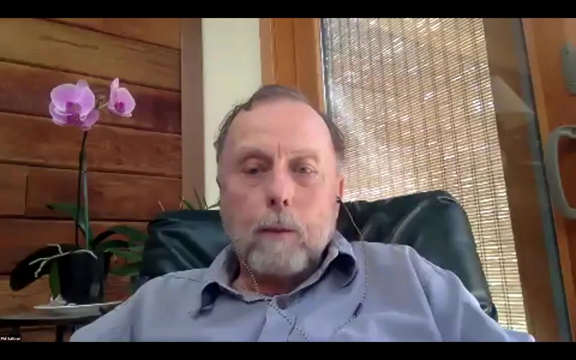 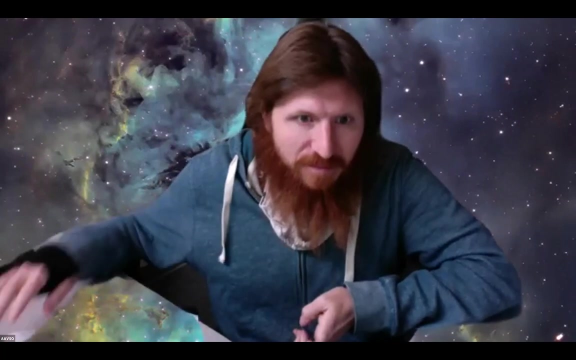 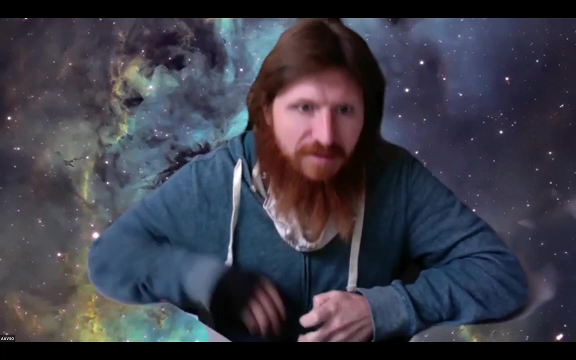 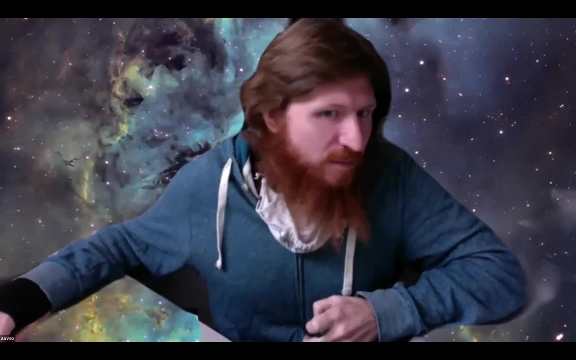 really, but hope to hope to make some decisions. okay, that's it. thank you, Phil. next up we have Timothy Tim Weaver talking about camera characterization, and if you don't mind stopping your screen sharing, Phil, oh, I'm sorry. there we go. no worries, take it away, Tim. I think you're muted. you are unmuted, but I cannot. 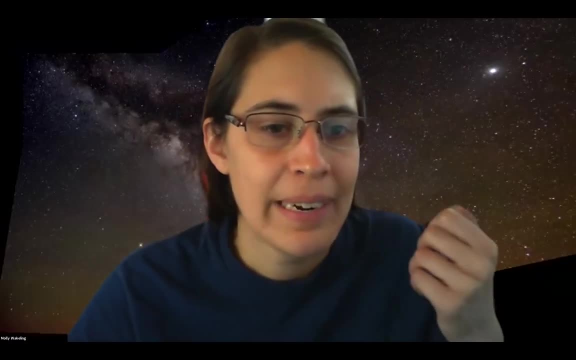 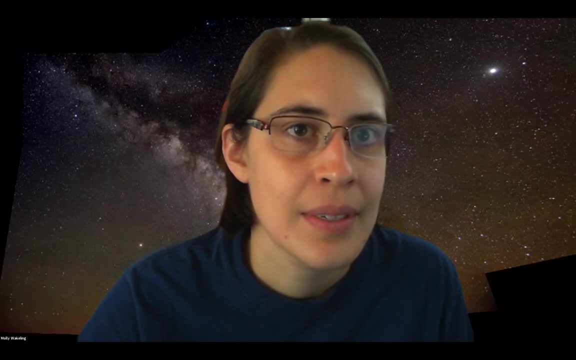 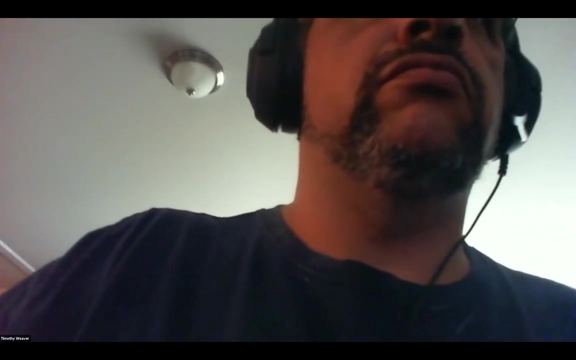 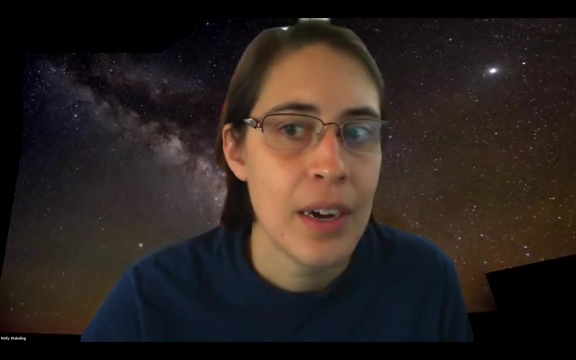 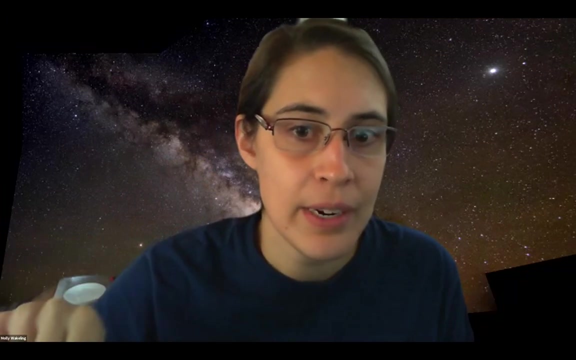 hear you microphone might have might be muted, separate from zoom he looks like he's looking at. I know we still don't have you what. make sure that it's not. there's not a hardware switch on your mic and also make sure that it's not muted in in on your 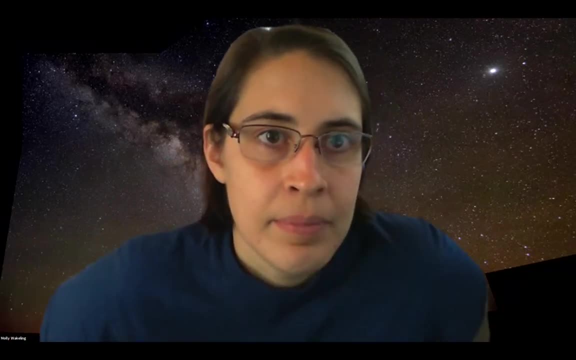 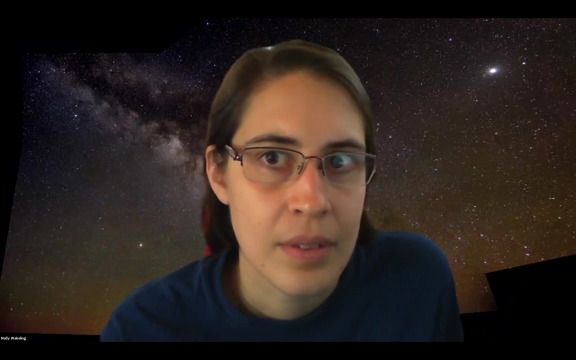 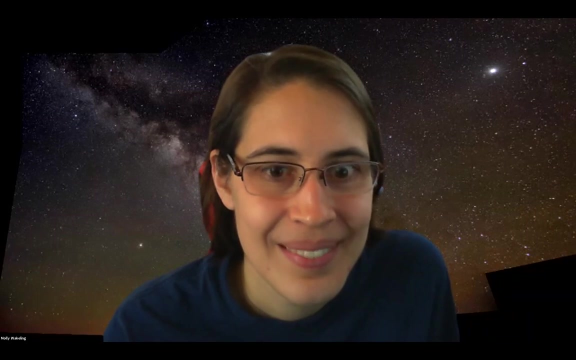 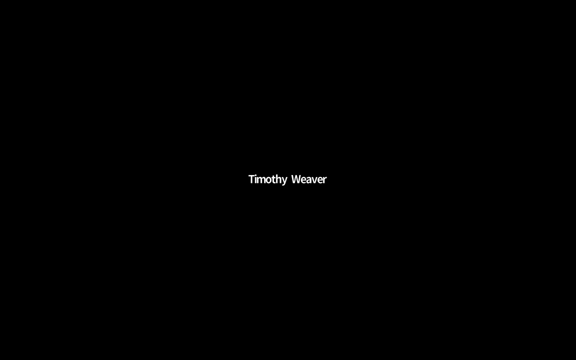 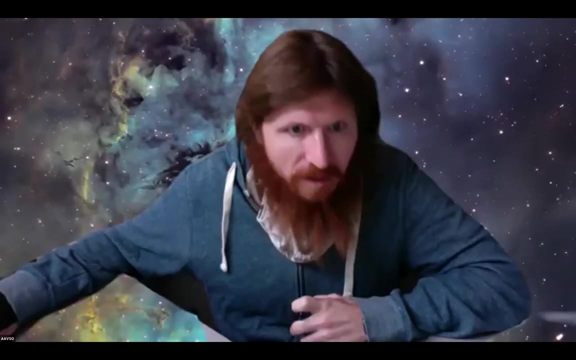 computer, like if you're on Windows or yeah, no, we still don't have you. you could also in zoom make sure you have that microphone selected. he's gonna go out and come back, I think. okay, I heard some sound. I'll give him one more minute and if not, then we'll. 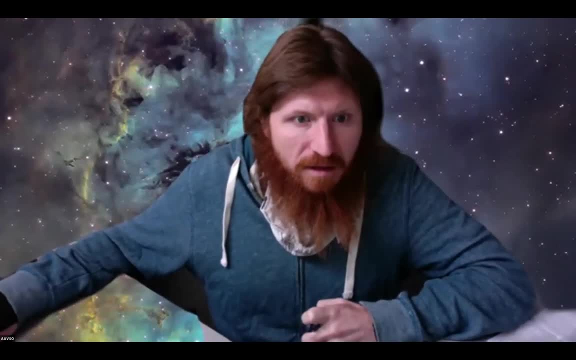 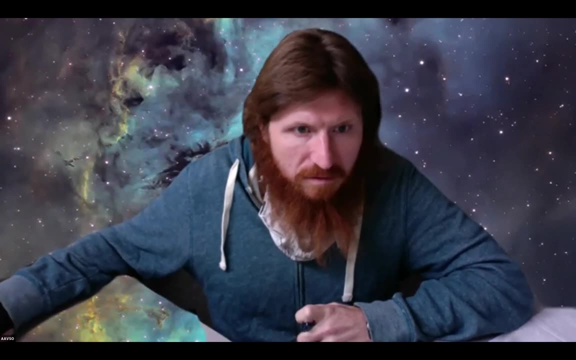 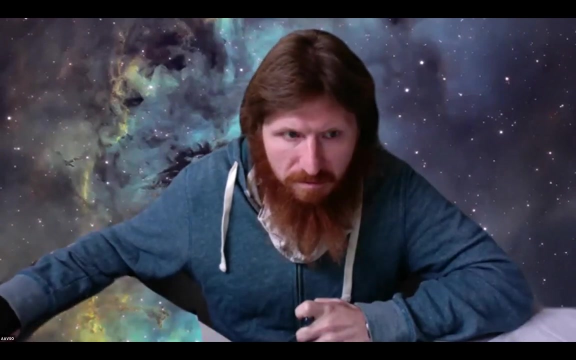 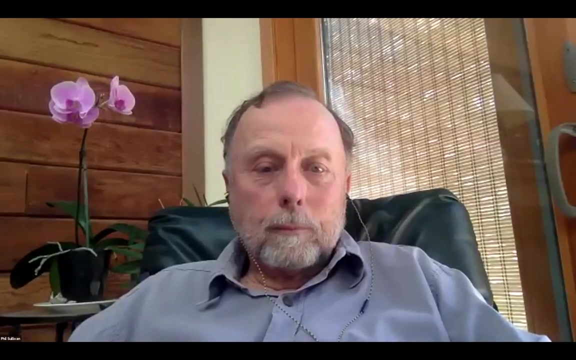 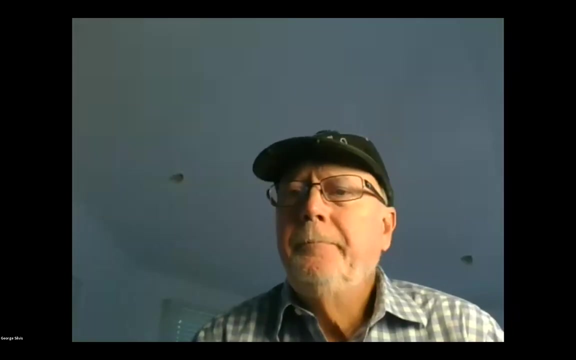 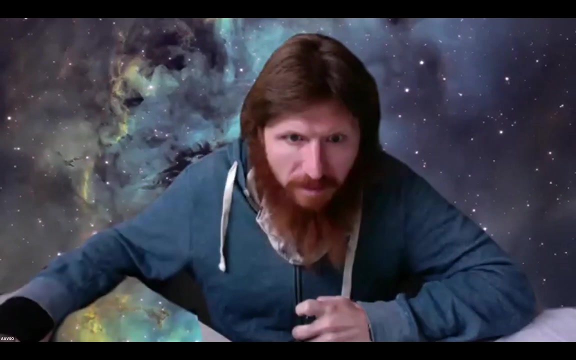 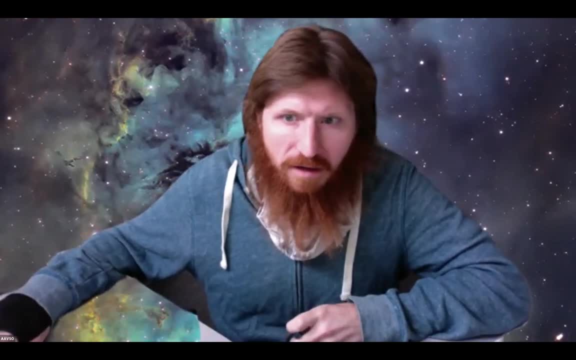 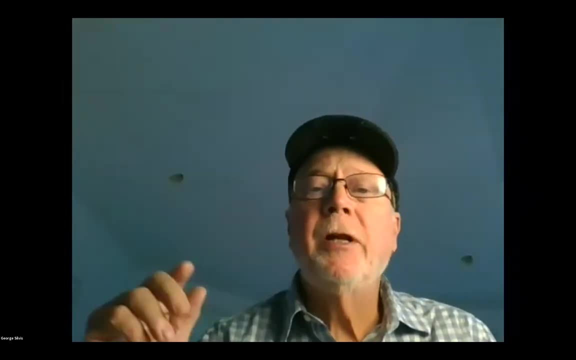 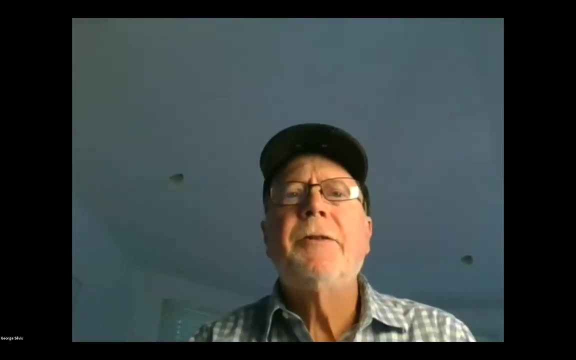 sure what's up with them. Why don't we give them a couple minutes to figure it out? Alan, do you mind starting up the AstroMakers presentation? Let me start. I wasn't quite sure who was going first. Okay, so let's see. I'm shared and on screen. Excellent. So AstroMakers, what are they? 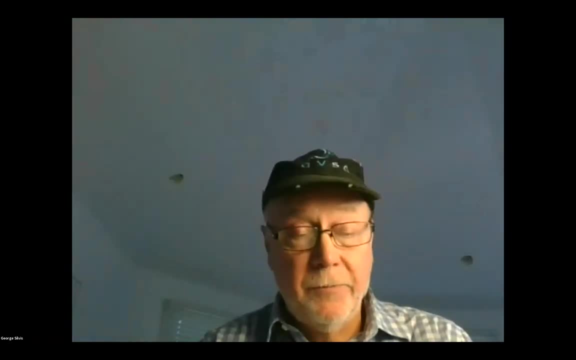 The AstroMakers is the part of the instrumentation focus group which is focused on making things. This builds from the whole maker movement, which you may be familiar with, which is the umbrella term for independent inventors and designers and tinkerers. 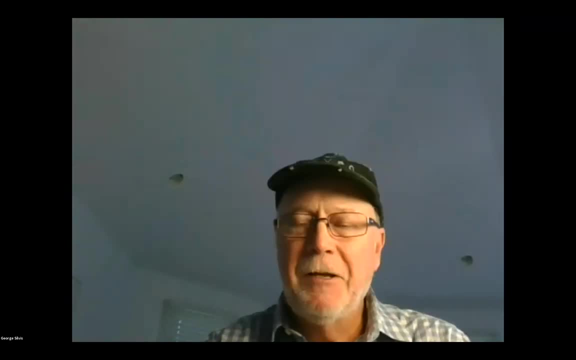 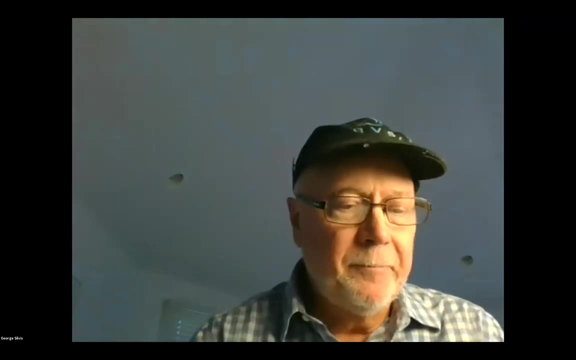 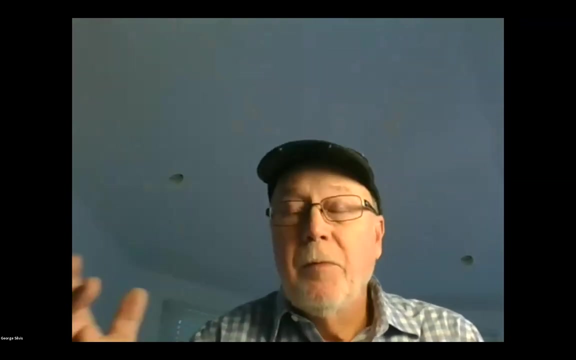 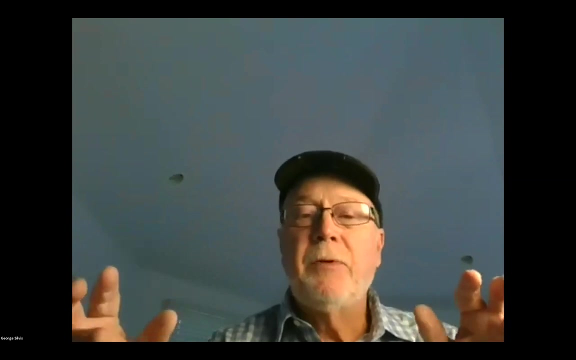 a convergence of computer hackers and traditional artisans. Remember Heathkit and the Radio Shack kits? Well, this is nowadays. we have things like Adafruit and Sparkfun and all these other places for buying parts and building projects. So our goal in the AstroMakers is to really bring projects forward all the way to the point of 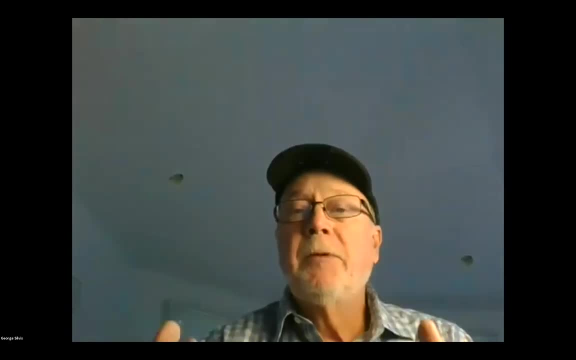 where other people can build them. If it's a hardware project, we're going to publish schematics and build materials and instructions on how to build, And if it's software, the software is going to end up in a repo So everybody can take a look at it. 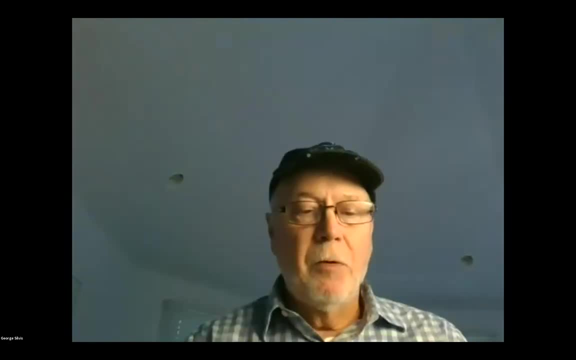 modify it and tweak it. But rather than doing a more general talk, let me turn it over to Alan Slisky, who's actually building some projects, And after that we're going to hear from Helen Edler, who's also building a real project. Let's take a look at what 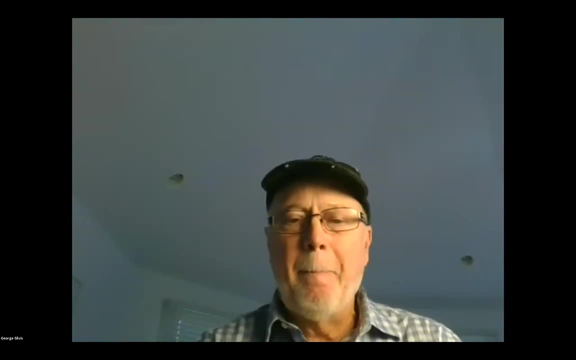 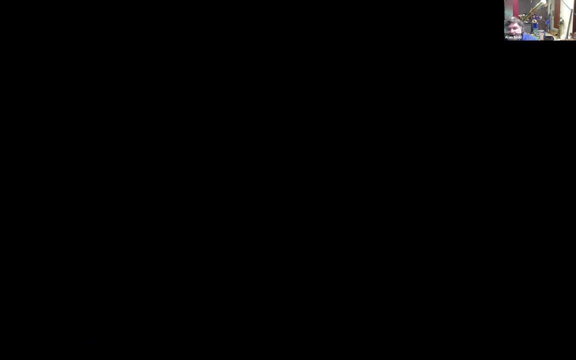 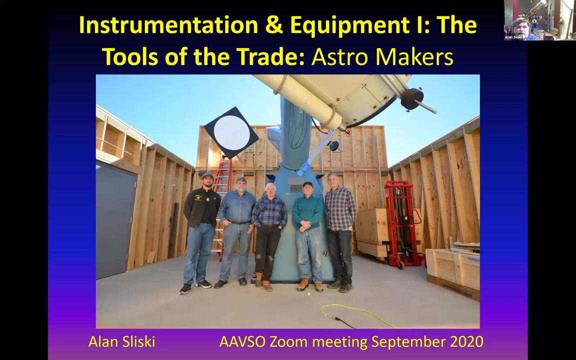 they're doing. Alan, let me jump in there. Sure, I'm an AstroMaker since before it was called that. I've been making astronomy gear since I was in high school or before to chase eclipses and stuff, And I'm getting much more back into it lately, helping some friends. 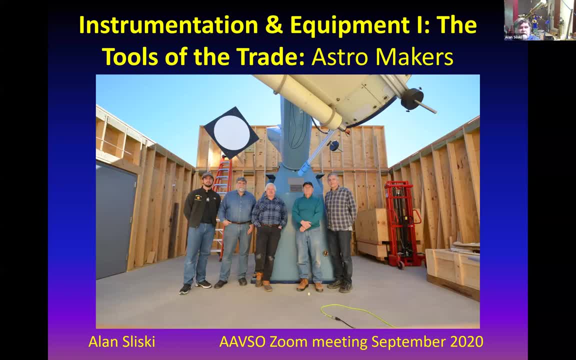 and colleagues build equipment for observatories, large and small, And it occurred to me that a lot of the development effort is common to what other people need and there's no reason to not share it all. So, with Richard Berry's help and Arnie Hendon's help and George's help, we're trying to 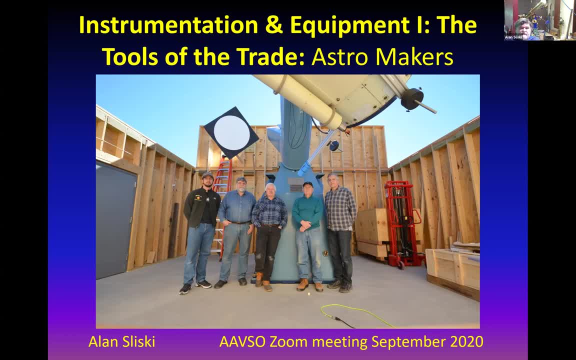 disseminate some of this information so that other people can bootstrap off of it. So we have a lot of the underlying technology in pretty reasonable shape, And if other people want to take on some of this work and build some stuff for their own observatory, that's a good thing. 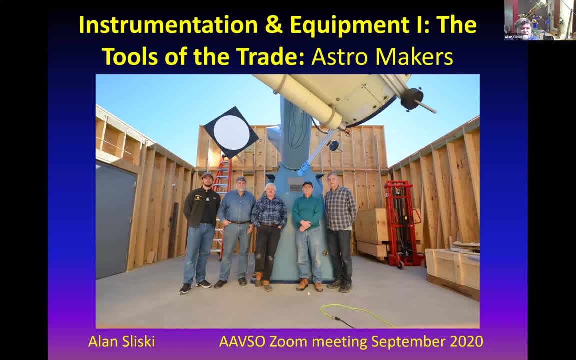 We have more people doing it. Several of these gadgets for a while have common application And many times there are good commercial solutions and sometimes there are not. And people can build this stuff, either because they're interested in building their own stuff, stuff because they want to save money, or because they want to customize it somehow to their own. 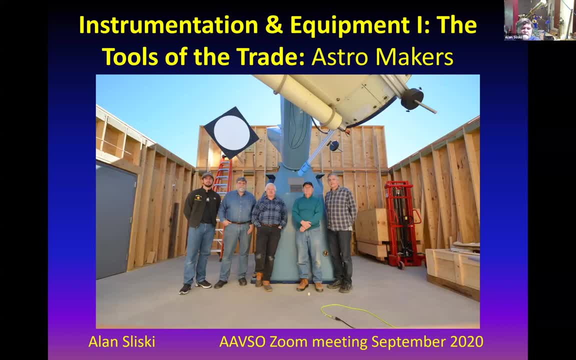 needs, And those are all valid. And there are people that want to buy a working solution and get on with their observing, And that's fine too. We have a very open system. So I'm going to talk about some of the gadgets I've been working on And I'm working with George. 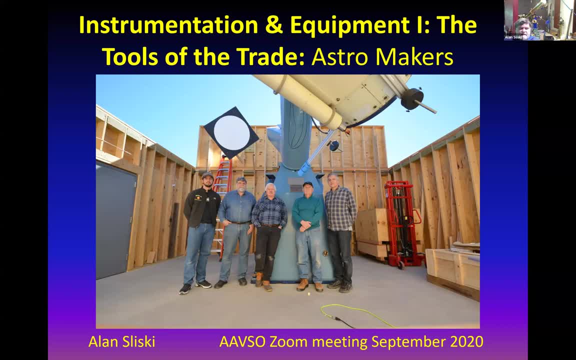 and Arnie to put these things into a format that other people can pick up and work with. So the picture you see is a large telescope I've been working on out in New Mexico. It's a 36-inch bowler and chivvins. that was at Princeton. It was given to a friend of mine And we built a new. 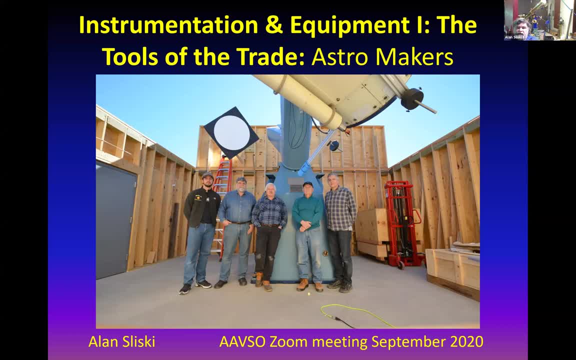 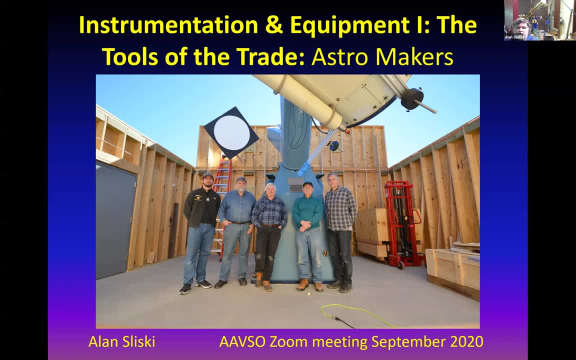 back together And it's almost ready for remote autonomous observing. You can see the telescope, But the thing on the wall, the white dot with the black surround, is an interesting combination of ideas that I've been working on for many years And Arnie Hendon has also been working on, So it's 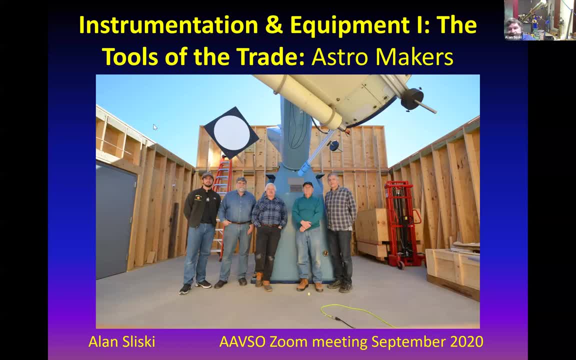 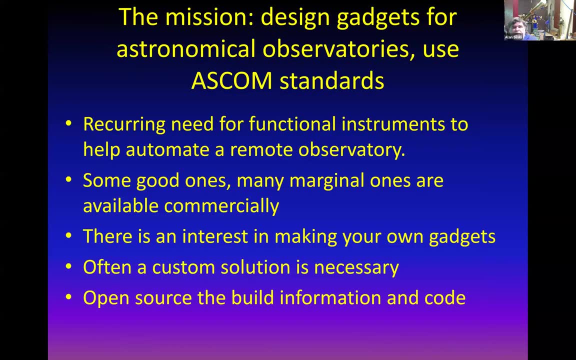 a combination of ideas that people have been working on And it's pretty interesting And I technologies that is ready for other people to to use. so the mission is to design gadgets for astronomical observatories and to use the existing ASCOM standards so that we can communicate with the world all the high. 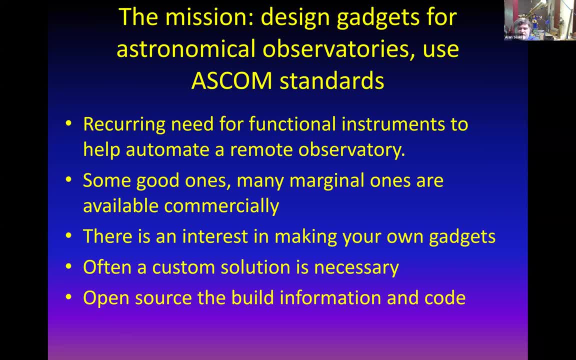 level applications, ACP for observatory automation and maximum and things like that. so all of these widgets have a common language. they speak a common language. there's a recurring need for these functional instruments to automate a remote observatory. you need weather information, you need a flat fielder, you 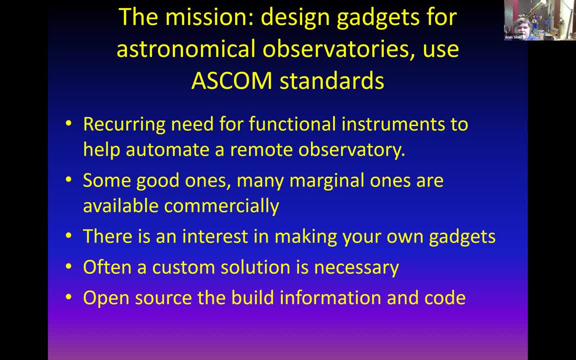 might need a focuser or a filter wheel. there are some good ones on the market. there are many marginal ones on the market and I get requests from people to build equipment that can't be bought. so to make a flat fielding system for a 36 inch telescope there, you can't. there's. 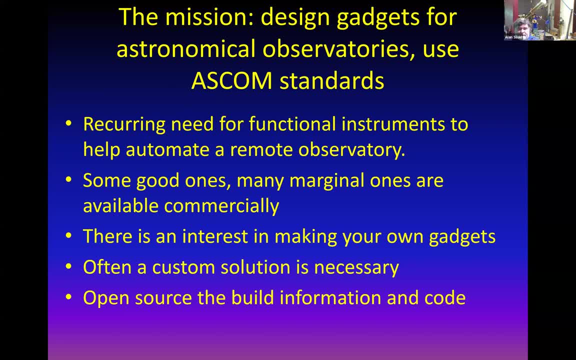 nothing you can just order, and so we're going to try to generalize that, to allow you all to make your own stuff, whether it's for 80 millimeter refractor or something much bigger, where sometimes a custom solution is necessary, and we're going to adopt the open source model so that we can. 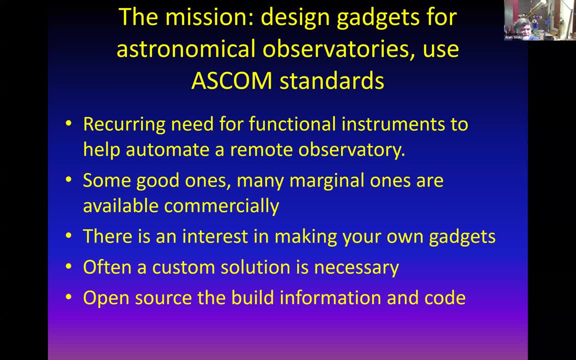 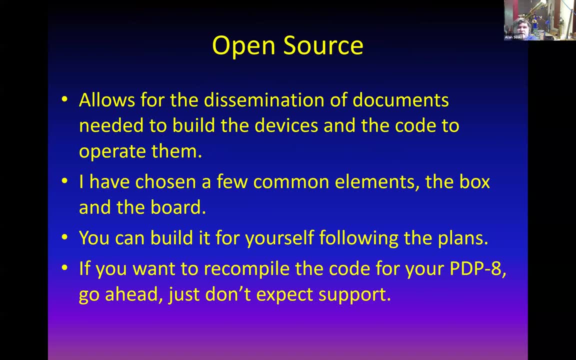 share with people this information in a way that they can pick it up and run with it. open source I I have an interest in the history of technology and the open source movement I'm going to say started in Massachusetts and the actual movement out in, far out in North America was on bursts of compressing. 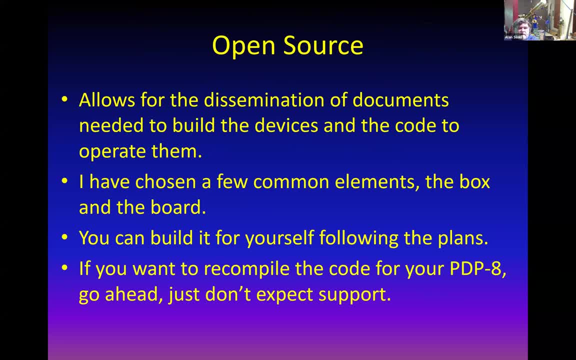 the rifle a while ago. actually it was around the mainね. This is a different call. this is a new, ever update on program coverage and my many big people have been with it since 1968. but people talk about 60 dollars today in the United States in the fields up. 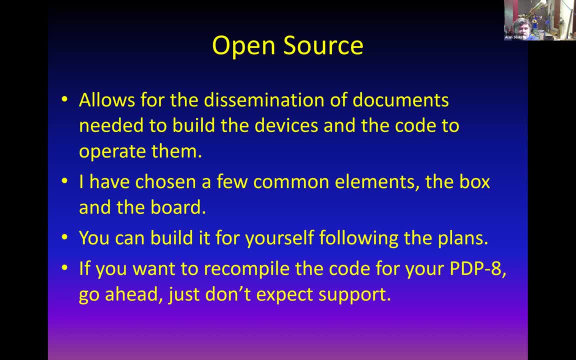 into the 80s, something that I haven't touched on either, but still, everybody said we can get involved in Navy Vet, but so we got to do that. I didn't do that at the moment and we got at the same time. I was there this last year, you know it was线 by a. 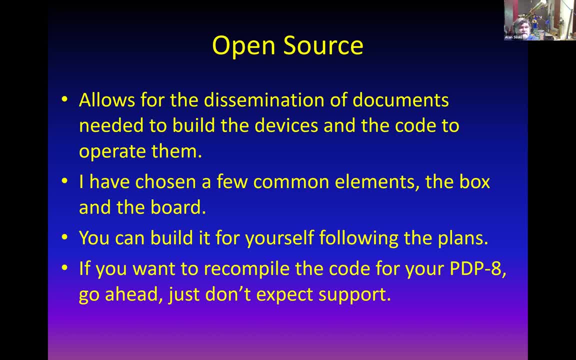 call the re framed rifle shooting�ess wayingt that's acted as combat, the first rifles with interchangeable parts, or was main winds of Vermont? the Springfield arsenal in Springfield, Massachusetts, played a big role when the the Arsenal contracted out parts to be out, parts to be made by local machine shops. part of the deal was you had to. 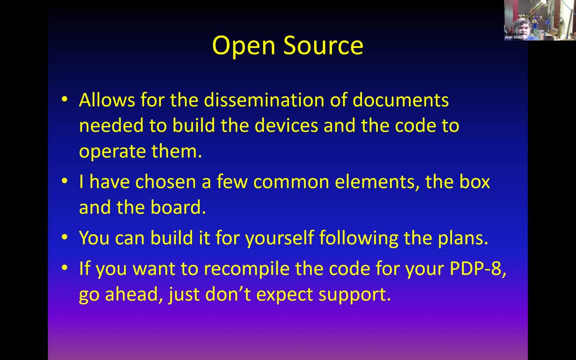 show the government inspectors how you made this stuff, And that's sort of- I believe sort of- one of the early examples of open source. The machinists used to travel from shop to shop and work for each other, and the ideas would spread. 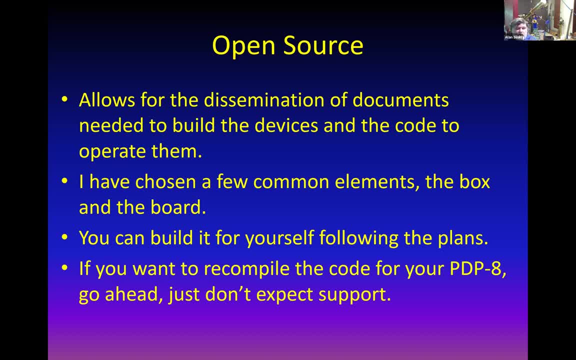 And their attitude was this open source thing where it's good to share knowledge, and if you built a very cool machine to make gun stocks or something, I could buy your machine and I could take it apart and say, oh, I can do that better. 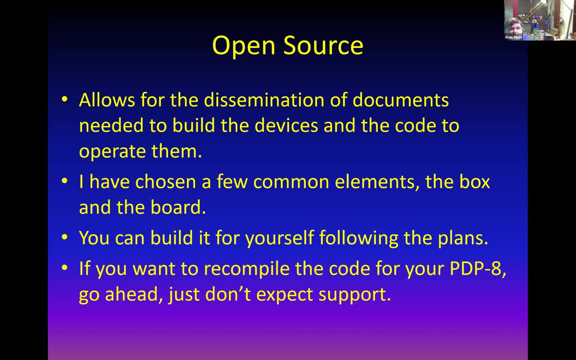 I can make a new machine and nobody would shoot me for that. So in that spirit- these astronomy gadgets- I've made the executive decision to choose a couple of common elements: the box and the board. So I finally found a very nice weatherproof plastic enclosure. 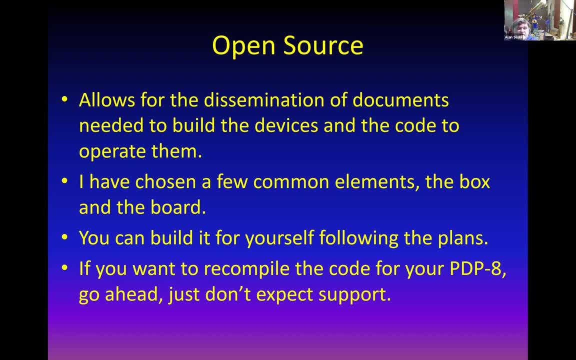 that'll hold an Arduino board. Now, if you want to design your own 3D printed enclosure, you're welcome to do that. If you want to recompile the code to run on your vintage PDP-8, you can do that too. 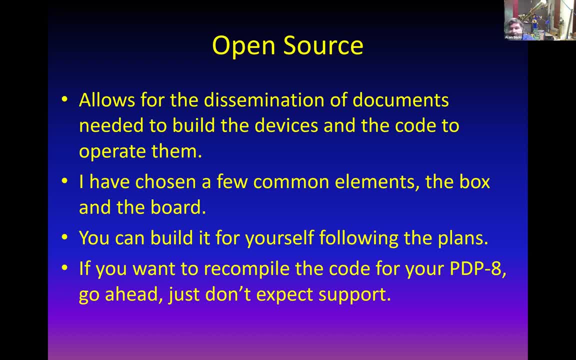 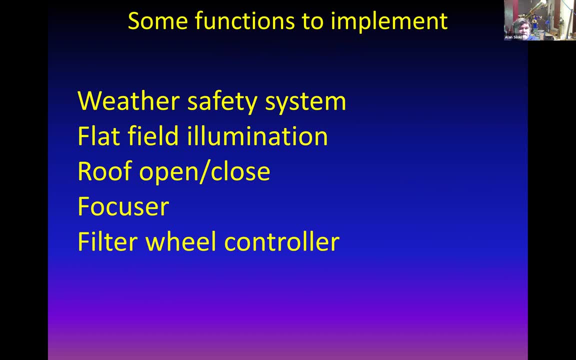 But I want to provide at least one working example. These are some of the functions we're looking at, whether it's a 3D printer, a 3D printer or a 3D printer Safety system. flat field illuminator. 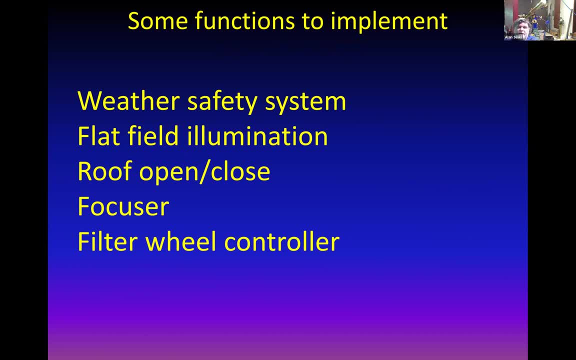 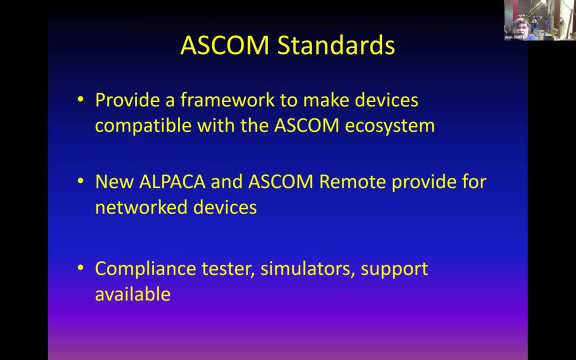 observatory roof open and close. A real dome controller is much more complicated- Maybe we'll get to that someday- Focuser and maybe a filter wheel controller, ASCOM standards- if you're not familiar with that. there's a wonderful ecosystem for common lanes. 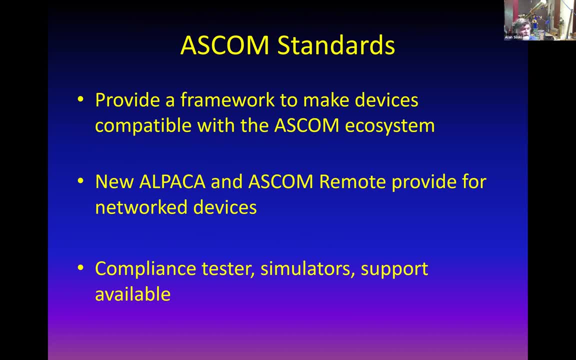 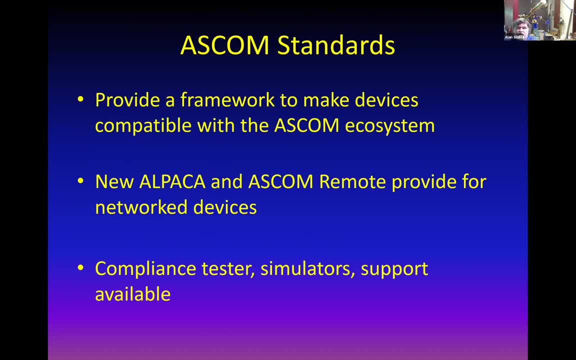 And it allows a common interface. There's a relatively new feature of that called ASCOM Remote, And they've branded this new thing. They call it Alpaca And what it is. it's a way to have network devices, The older model of having a device driver. 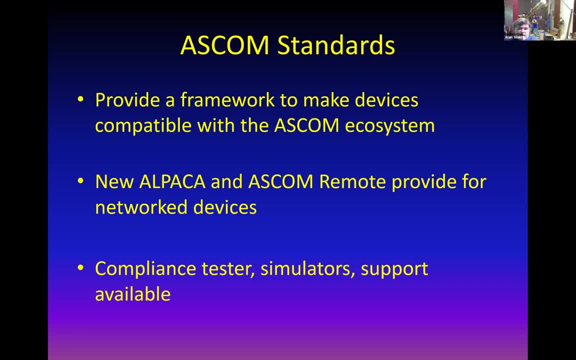 in the computer vanishes, And now the device that's on the network again speaks this common language for the device that it is. I'm very happy that they've made that move. I've been urging lots of people for years to go to ethernet. 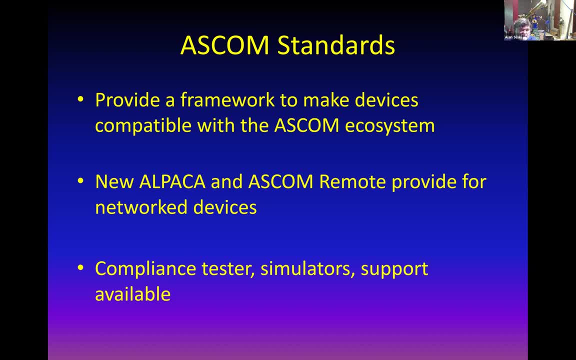 instead of USB or serial ports. even worse Part of it is that USB and serial ports go directly to your motherboard and astronomical observatories often are in places where they have a lot of lightning and that's a bad combination. And ASCOM also. there's a big infrastructure. 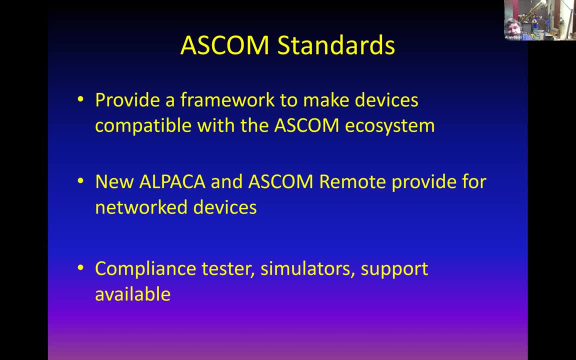 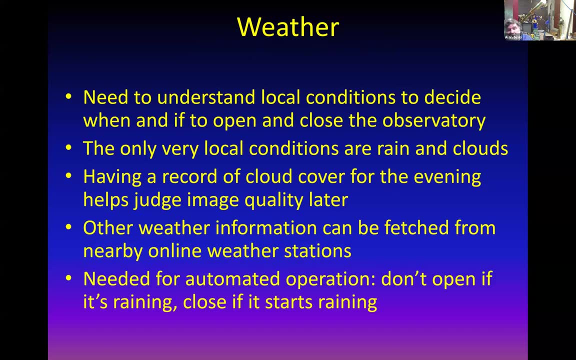 So if you develop something, there's compliance testers, simulators and there's a big ecosystem and network of support. The first gadget that I thought might be useful very generally is a weather. I'm calling it a weather safety system. You can call it other things. 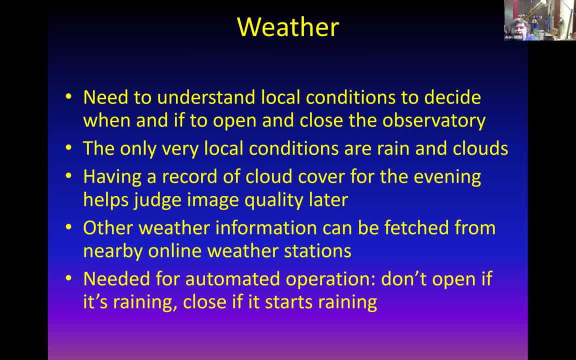 but you need to understand the local conditions to decide when and if to open and close an observatory remotely, even if it's just in your backyard or if it's across the world, And the only very local conditions that you'd need to know about are rain and clouds. 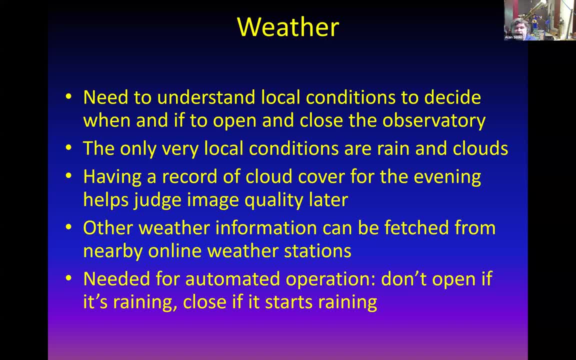 If you want to get the wind speed and the temperature, whatever, you can fetch that from nearby weather stations that people graciously connect to the internet, And having a record of cloud cover for the evening may help you check your image quality And the 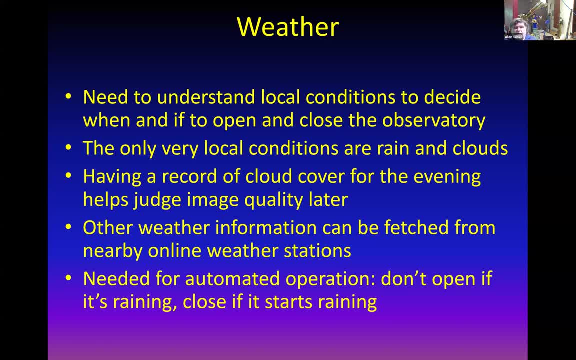 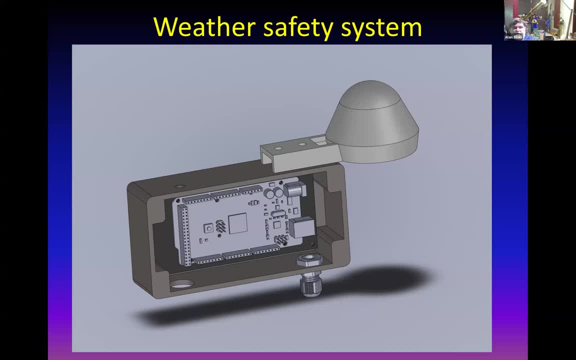 the rain sensors in the cloud sensors basically don't open if it's raining and closes if it starts raining. So here's the CAD model of a very simple gadget. It has an Arduino board and a rain sensor in a box. I've chosen for several reasons. 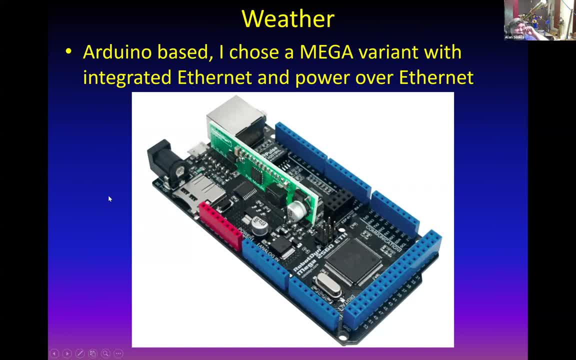 I'm not gonna get into a lot of detail, but in Arduino Mega it's a. Arduino is a very popular microcontroller for hobbyists and they're readily available. They're not- they're not- very expensive. This particular version has a ethernet integrated. 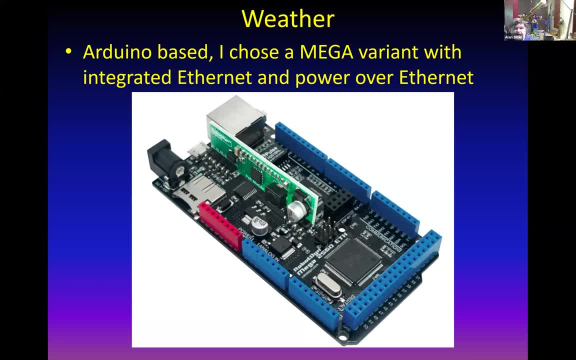 and, more importantly, power over ethernet. So you don't need a separate power connection to the box. You can run the standard power over ethernet. So you have one cable to the box. That's the power of the other part of the box. 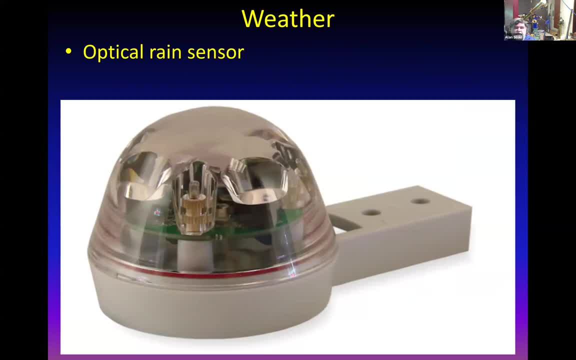 I found this very nice optical rain sensor. So the electronics is not actually out in the weather. You know there are a lot of conductive type rain sensors and they do work but they're actually exposed to the, to the elements. So somebody makes this little gadget. it's about $50. 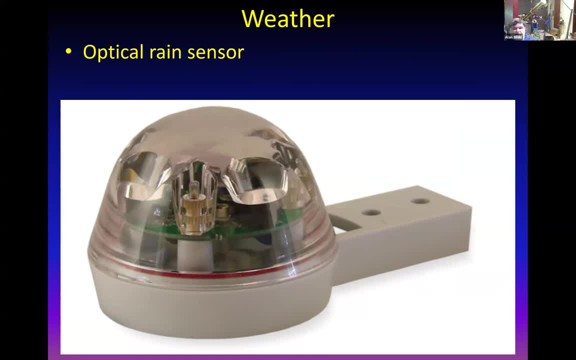 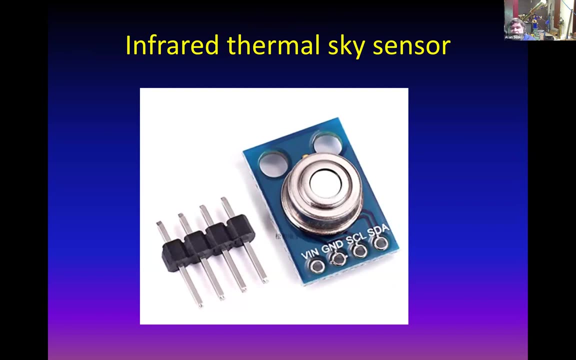 and it has a little heater in it and it has the electronics and it's. it uses the internal reflections in this acrylic dome to see whether there's raindrops on the surface. There's a infrared sensor that's sold to the Arduino community, the hobbyist community. 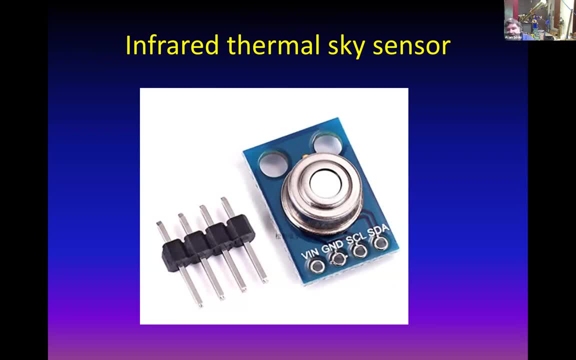 It's $3 or something. it's not very expensive. It looks at the sky and you can tell whether or not it's cloudy. If it's cloudy, the sky is warmer than if you're just staring out into deep space. It also has a ambient temperature sensor. 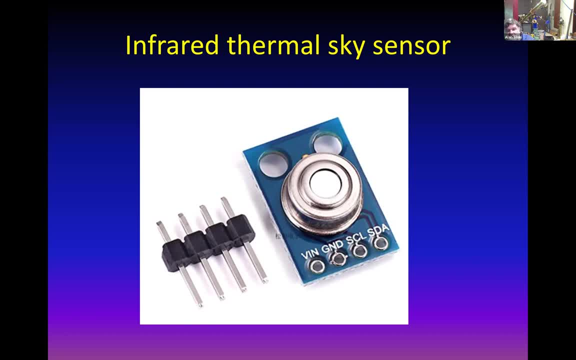 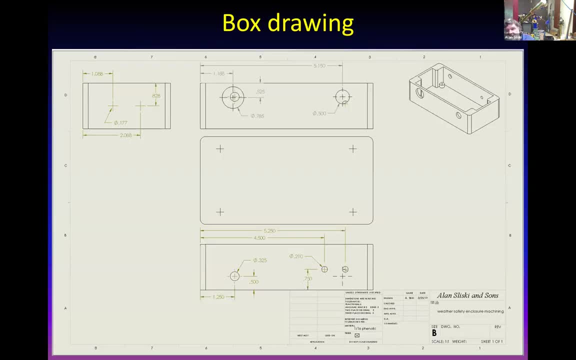 built in so that you can check the local condition And the code is readily available and it's easy to integrate. So I designed a box. This is part of what will be available, So you can buy that particular plastic box and you can follow these plans. 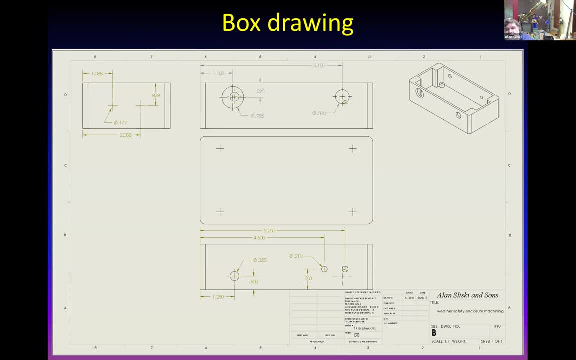 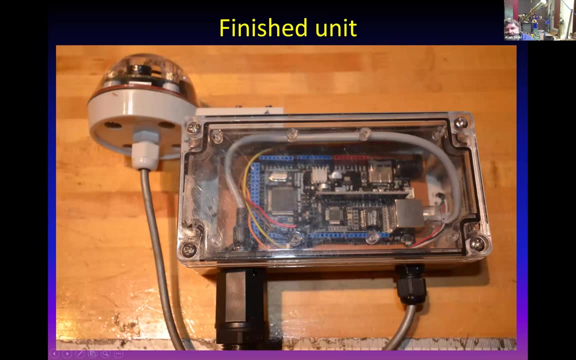 and drill the holes in the right place and be able to build the gadget. And here it is, together with the Arduino in the box. This thing on the left bottom is a waterproof ethernet feed through, So it allows you to get the ethernet cable in. 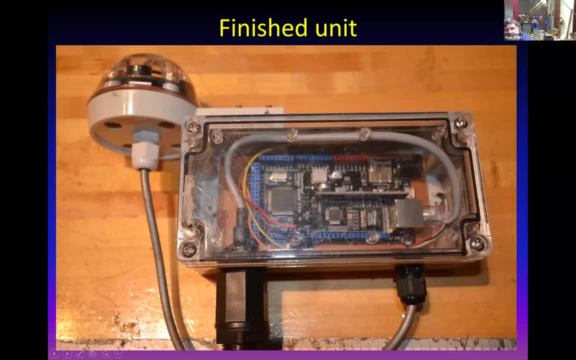 without getting the insides wet, And then the rain sensor cable comes around and talks to the Arduino. The details of this: we've built two or three of those so far and the documentation needs to be polished up. It's not if we have a couple of early adopters. 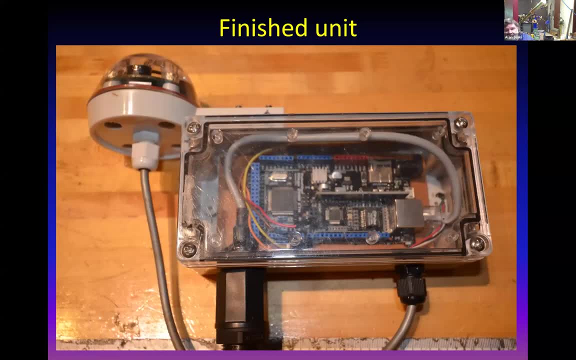 that aren't afraid of. this is not Heathkit that was mentioned before. in the 60s and 70s, people would make either simple things or the major project- you could assemble your own color TV, And they had tremendously detailed instruction manuals. 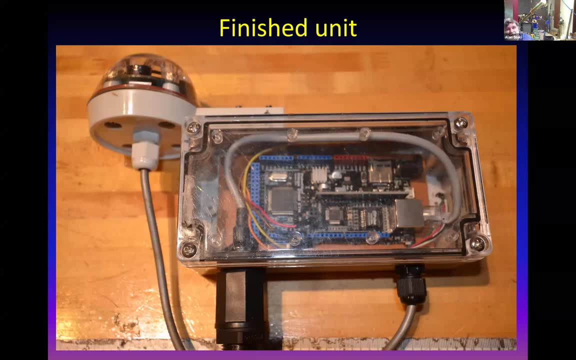 If you want an interesting example, go on eBay and buy an unbuilt Heathkit. They're getting pricey now, but anyway fantastically detailed. I don't intend to do that, So you have to have some skills and have a little bit of a sense of humor. 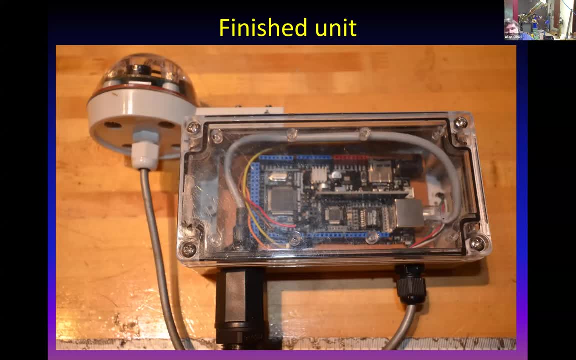 to take on a project like this, but it's doable, And what I want to do is provide an example- at least one example- where it all works, And then people can either build that and move on to the next thing or, if they want, to fiddle with it, 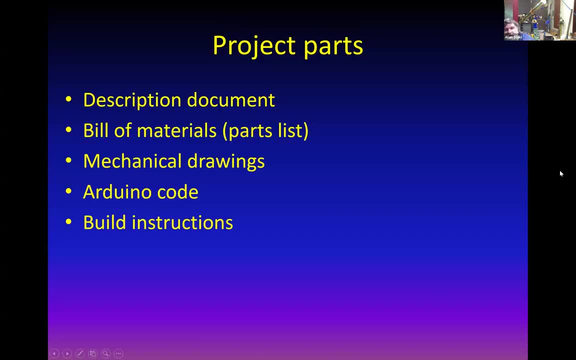 and add a ultraviolet Sensor. that's okay too. So what I expect will be the project will be a description of what's going on, a bill of materials, which is a parts list and where to get all the parts. mechanical drawings. like you saw, the box. 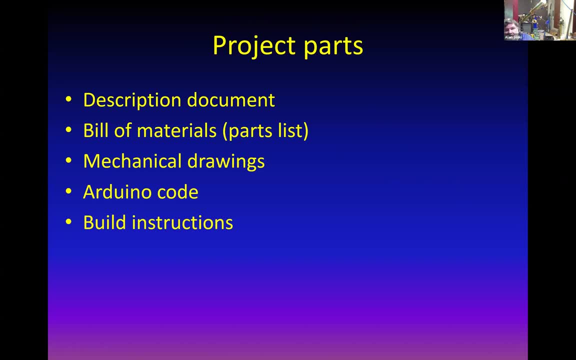 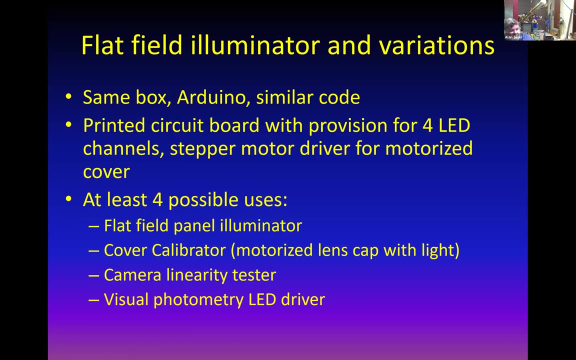 where to drill the holes, the Arduino code and some build instructions so that you have an idea how to put it together. So the that little plastic box. you need to tap the holes in the bottom of the box to accept screws to mount the Arduino. 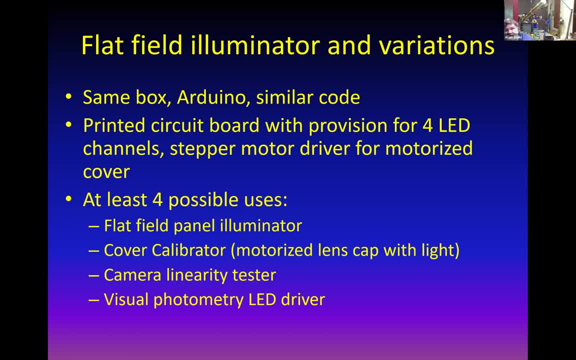 Not hard, but it's just a note. Flat field illuminator is the next thing. that's fairly far along. same box, same Arduino and much of the code will be the same, And I've designed a printed circuit board that can run up to four LED channels and has a step. 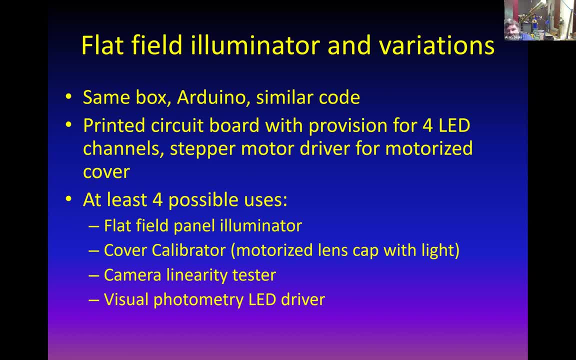 or motor driver if you want a motorized cover. So there is a new device type for ASCOM called the cover calibrator. It's a motorized lens cap with the flat field they're built in. there's a commercial product called the flip flat. 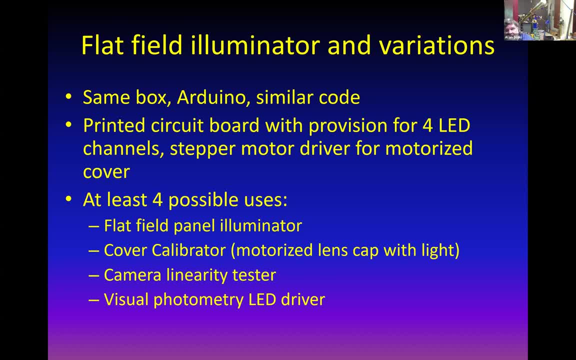 I don't know if they're making them anymore, but same idea. But it turns out there's. there are some other applications, So you can make a flat field illumination panel. I'll show you that in a minute, This color calibrator which would have the motorized lens cap. 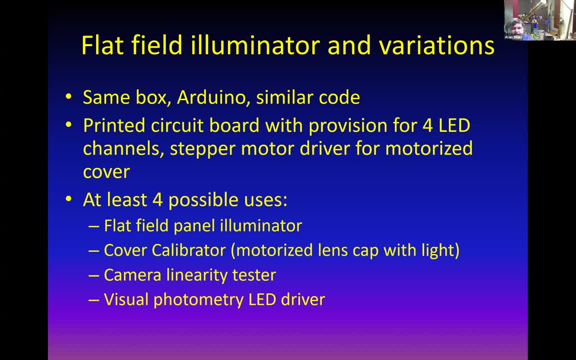 with the flat field they're built in. You can use the same stuff for testing camera linearity, because you have very precise control over the illumination levels. And then Arnie mentioned that there might be interest in a visual photometer And the hardware would be, you know, an eyepiece holder. 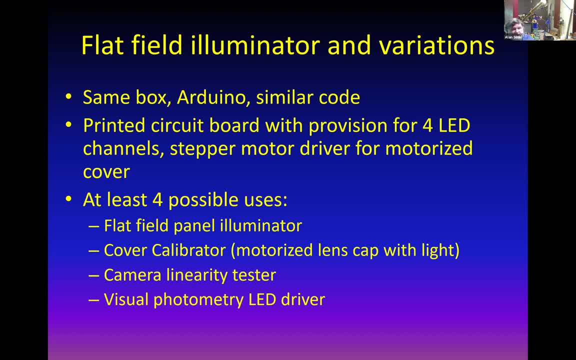 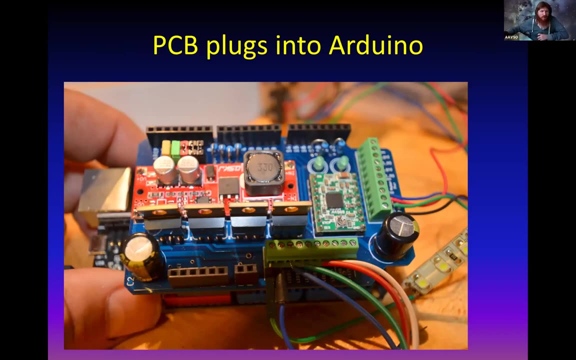 with a beam splitter of some source and optics to create an artificial star. But this circuit and everything could be used to drive the LED with a range of known brightnesses. So over time now, Alan, so you might want to wrap it up. 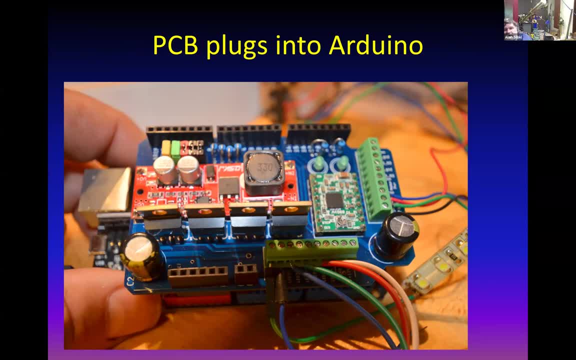 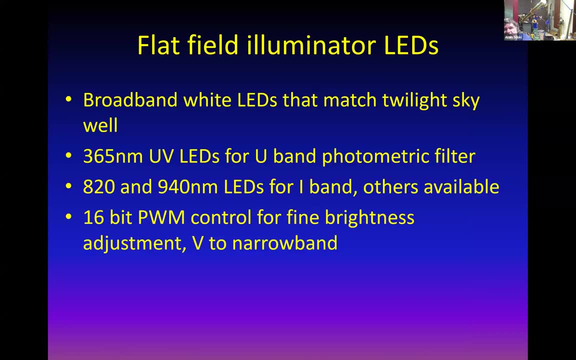 Yep, So this is the circuit board that drives the LEDs and the stepper motor. Okay, This is the flat. talking a little bit about the flat field illuminator, So this: I've discovered these broadband white LEDs that match the sky pretty well. 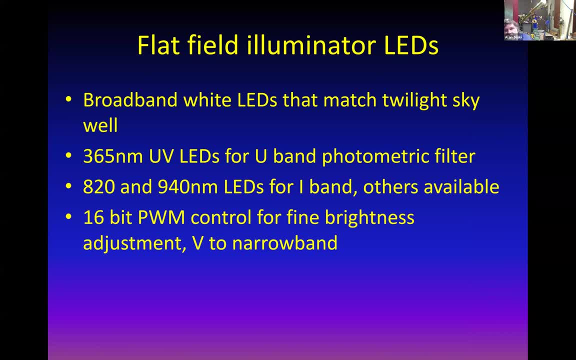 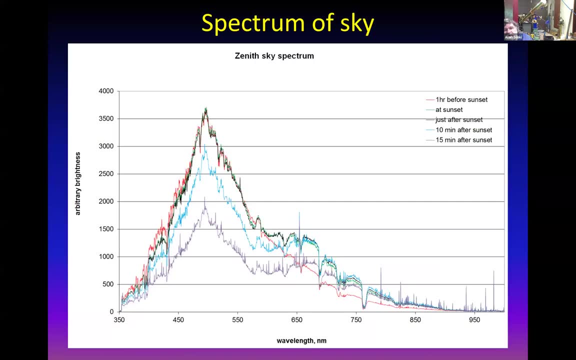 And you can also have UV and infrared LEDs and 16 bit pulse width modulated control. These are the filter transmissions I measure. This is the Zena sky spectrum on the same scale different times before and after sunset to compare to doing sky flats. 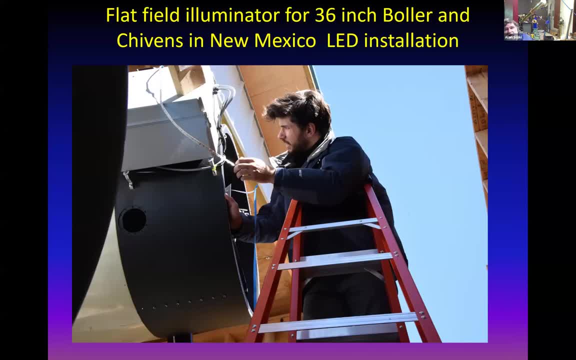 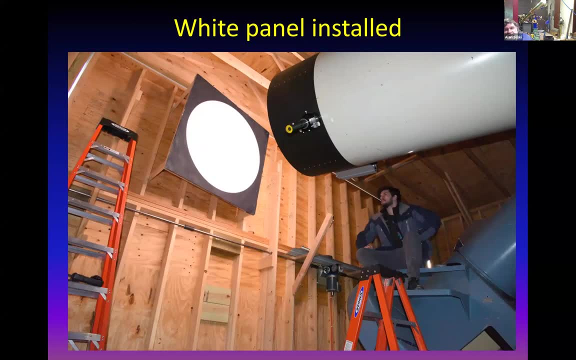 These are the white LED spectra. This is installing those white LEDs on the front of the 36 inch telescope. And that's the flat panel. That's a. it's a styrofoam panel which is very inexpensive, and styrofoam is very white. 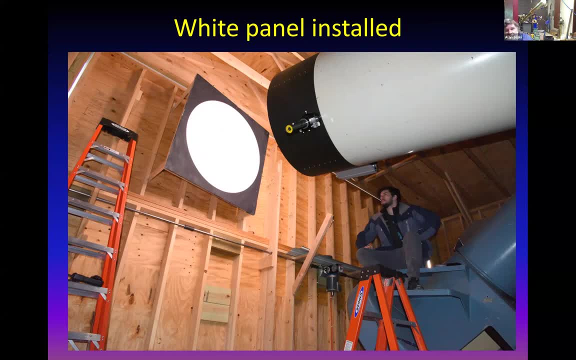 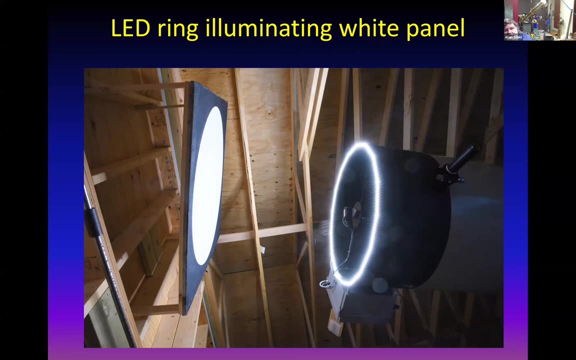 not because of the composition, but because of the structure. The foam creates this white like snow and you don't have to worry about the spectrum features. It makes a good flat field panel And it's illuminated by the ring. What we found is, if you put the this panel 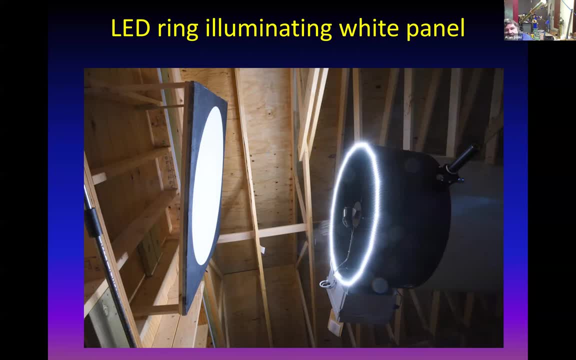 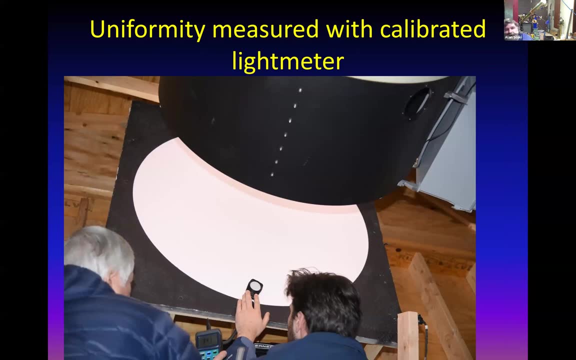 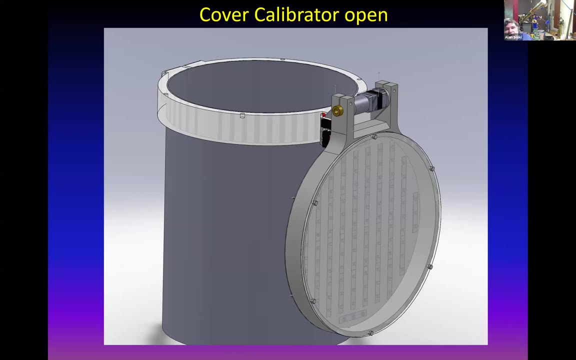 one radius away from the ring, you get extremely good uniformity. We measured the uniformity very carefully with a calibrated light meter And this is the cover of calibrator I'm working on. This is the CAD model. open and closed. You can see the LED array. 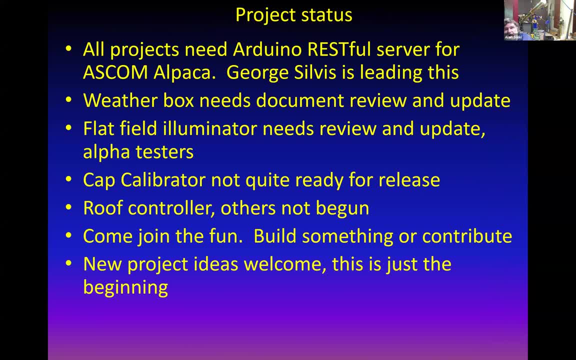 You can see the LED array inside the cover And here's the project status. There's some code which is kind of the major element left to be done. The weather box needs. I got to update the documentation. The flat field illuminator needs to be packaged up. 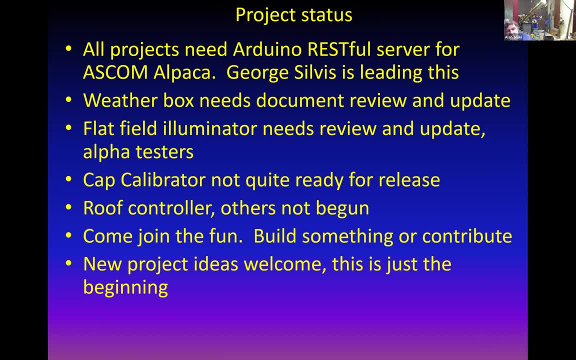 for people to test out. The cap calibrator is not quite ready for release Roof controllers, others not begun Anyway- and I encourage you guys to participate And there's an AVSO forum for this stuff. 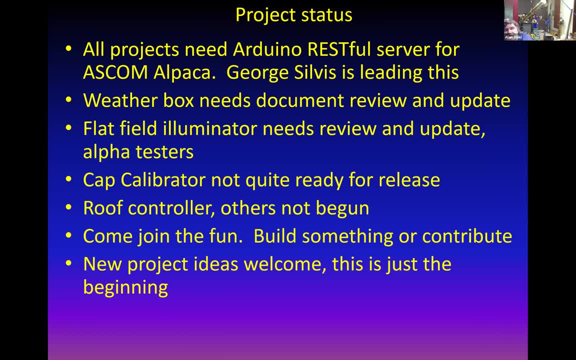 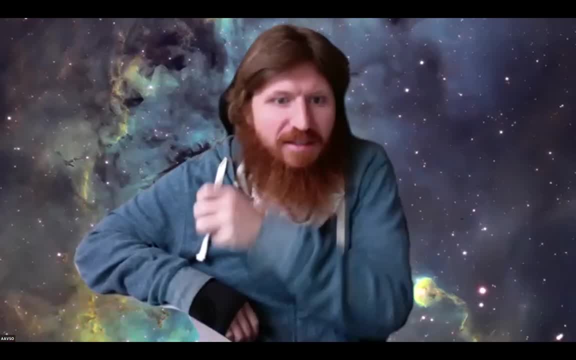 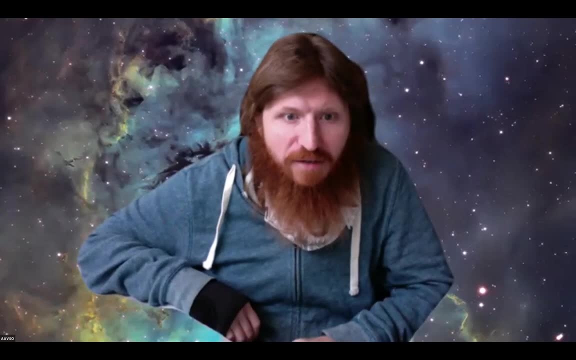 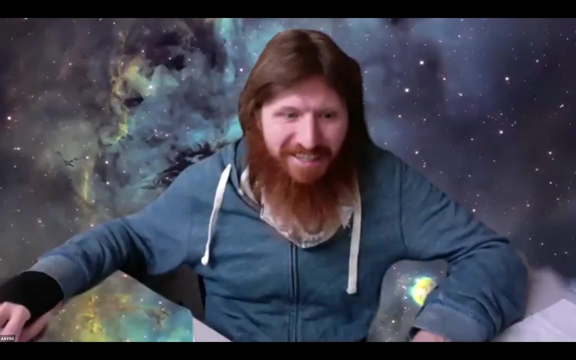 that's just getting organized. Thank you for your attention. Thanks, Alan. So let's try, Tim again. You've just muted yourself. I'm sorry, can you hear me now? Yes, now we can hear you, Perfect, Okay. yeah, I apologize for. 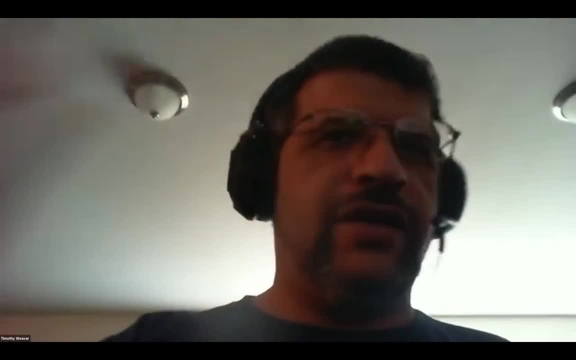 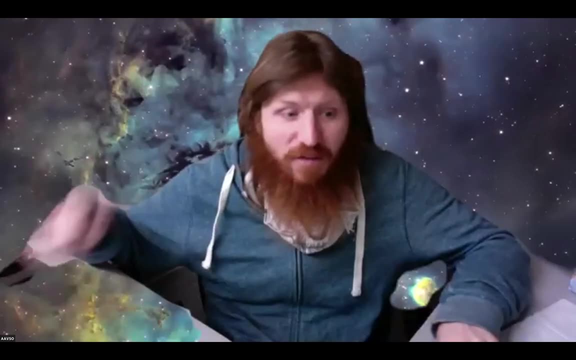 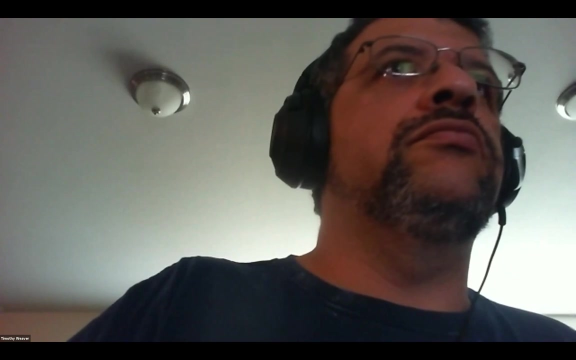 I tested this equipment out. when I first got it, I thought it was going to be work. I thought it was going to work out. So let's get started. Yeah, so, All right, let's get started with. 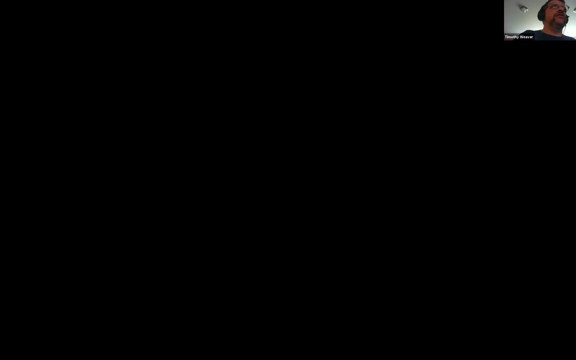 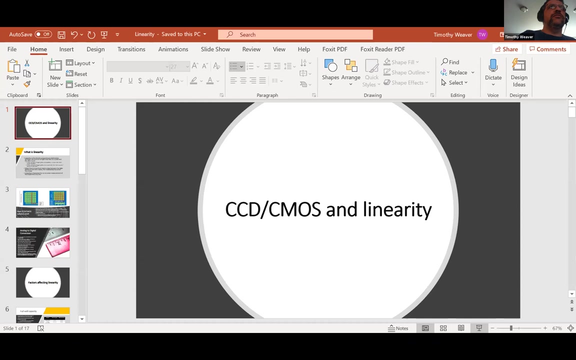 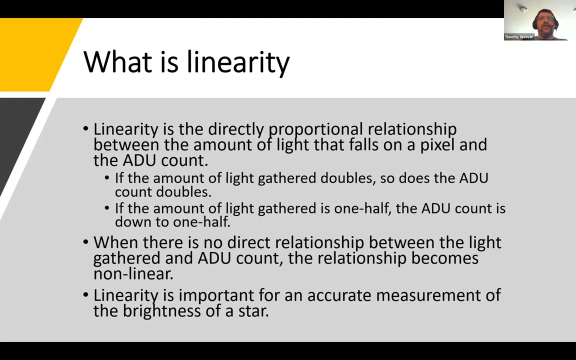 I'm jumping way ahead, There we go. So I'm jumping back in, Here we go. All right, CCD and CMOS and linearity. Now, linearity is very important for taking accurate measurements of stars. Linearity simply means that, if yeah, that the proportion. 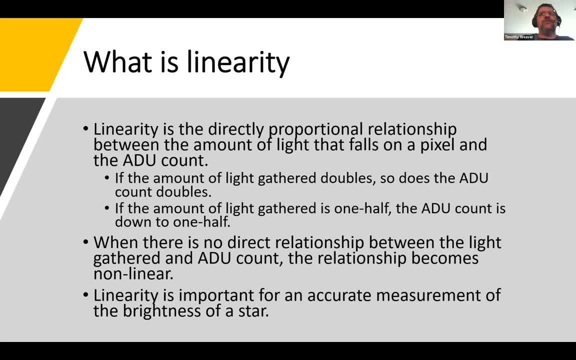 that the amount of light that you gather is proportional to your ADU count. If your ADU. If your. If your light or light is proportional to your ADU count. If your ADU. If your. 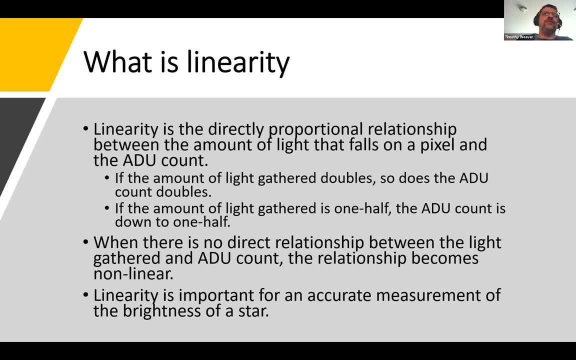 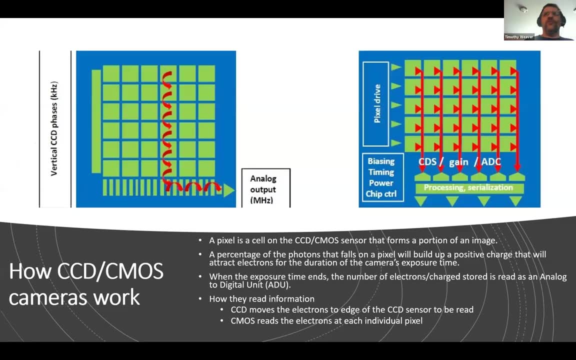 if the light you gather is double the is, if you double the amount of light you think you gather, you double your ADU count. When there's no direct relationship between the light gathered and ADU count, the relationship is nonlinear. All right, before we start on on linearity, I'm gonna talk a little bit. 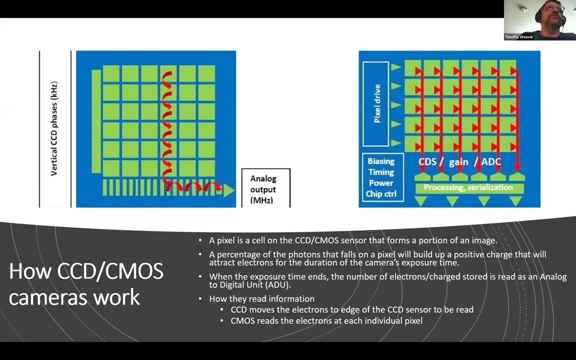 how CCD and CMOS cameras work. All right, if you've ever looked close up to your screen, of your, of your, if your television or your computer monitor knows, there's like little cells inside those cells are pixels. Well, just as your television has pixels, so does your camera, or at least your electronic. 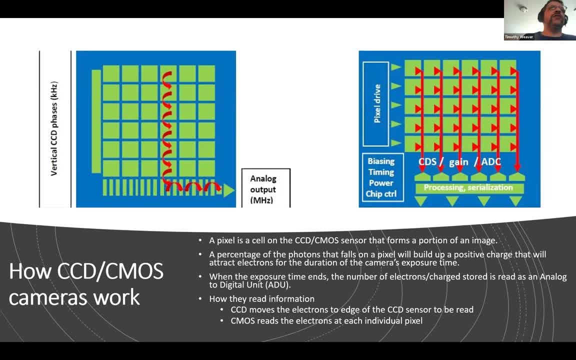 camera does. And what these cameras do is that, whenever they're, they're photosensitive semiconductors. basically, like a photon. a photon, a quantum of light, falls on a pixel, the, and a certain percent of them are absorbed into the, are absorbed into the semiconductor material. it really it loosens up an electron and the electrons. 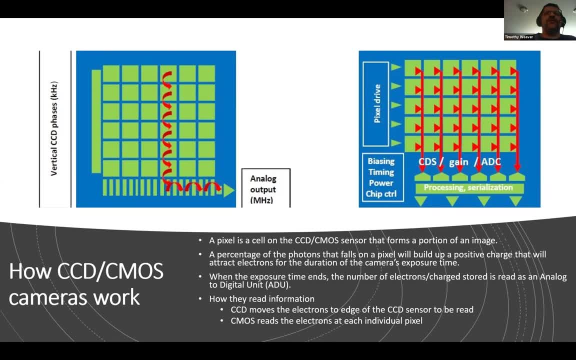 are gathered in in something is roughly a capacitor, and this happens during the entire exposure time. when the exposure time for the for the image is over, then all of those electrons are then shifted or moved to a amplifier, where they're measured and stored as an analog to digital unit, which is the adu, Now the 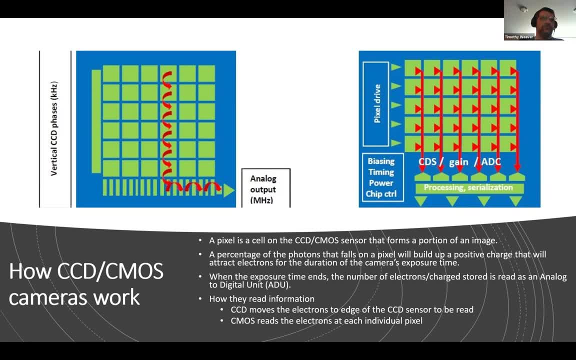 difference between CCD and CMOS is that CCD have had like one or two of these amplifiers, or a or a adu that measures the electrons or the analog output, Whereas each of those CMOS, each of them, have their own amplifiers and they measure them out. so you can match. so think of it as a CCD, as a series. it's. 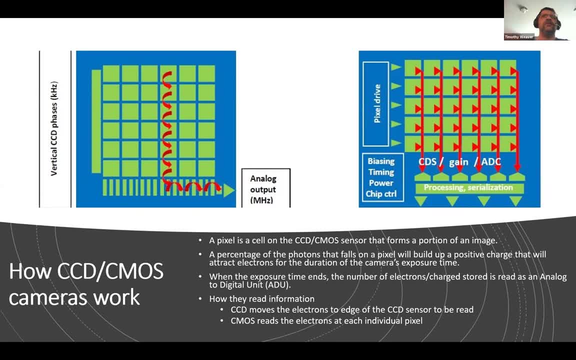 more like a series circuit, whereas the CMOS is more like a parallel, and you can guess which one probably is going to be faster than the other. and I have a little bit of it. I have an animation I can show you. I just got to stop sharing. 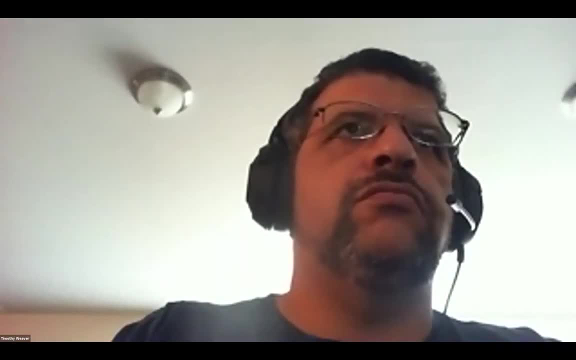 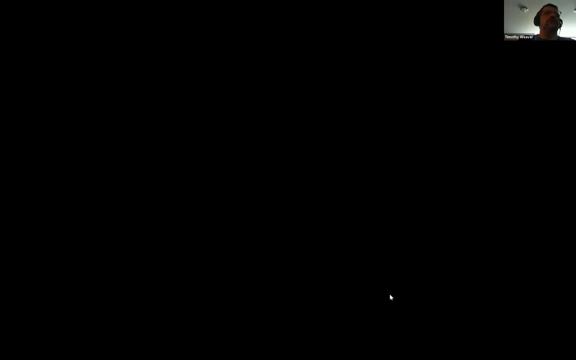 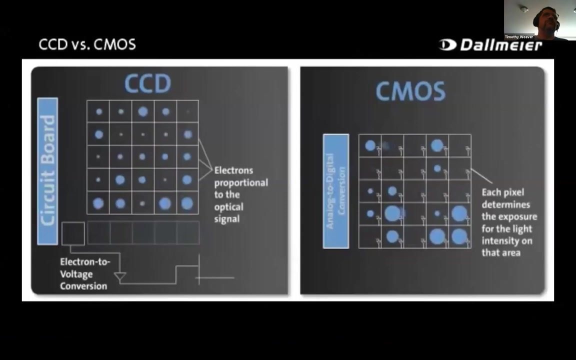 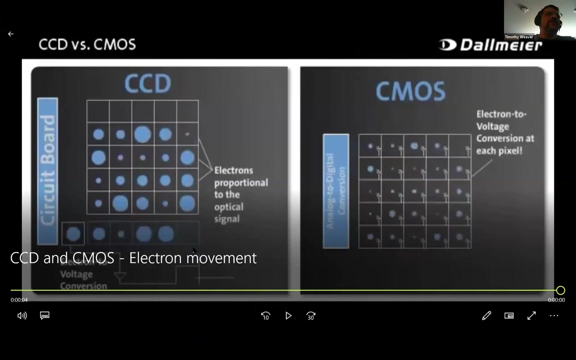 for a second. okay, can you see it? okay, as you can see the seat as. okay, it's real quick. I'm now. I tried to look for a longer video, but but basically the CMOS with the CCD, all of them collect and they measure them out, and then they measure them out, and then they measure. 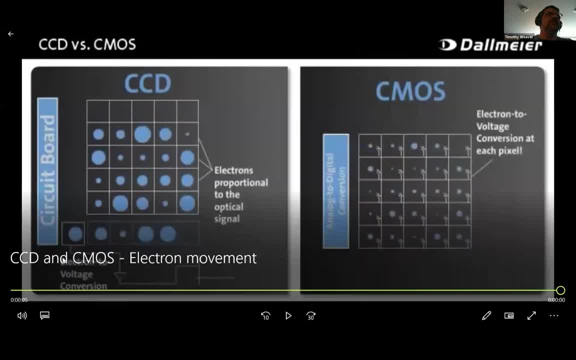 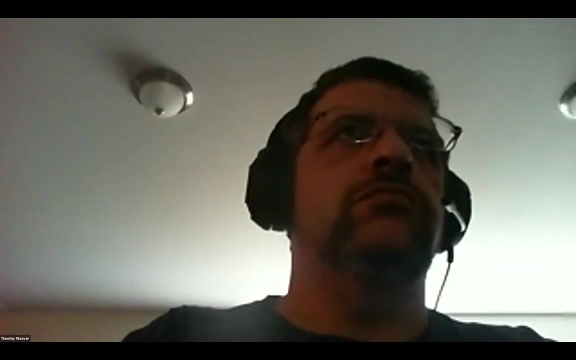 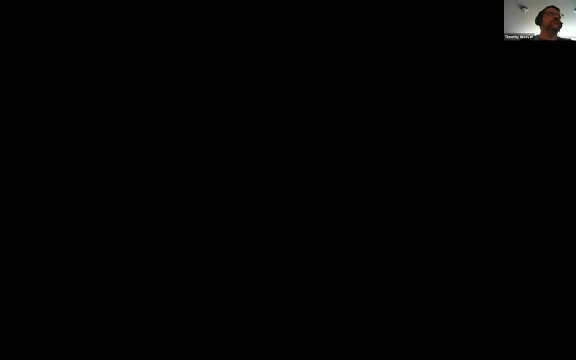 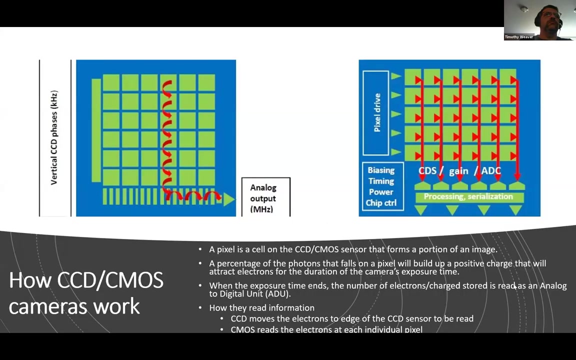 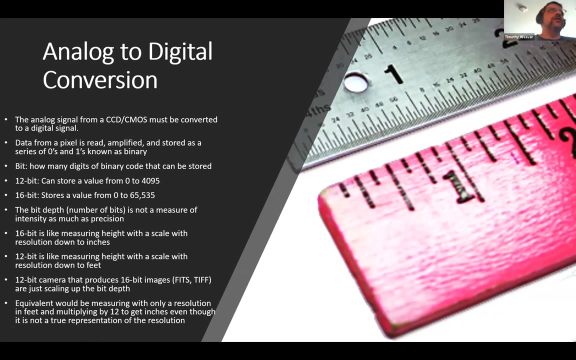 reach, reach. they read out one row at a time, right here, on the, on the electron to vultures: conversion, right there. whereas with the CMOS, they read out on each individual pixel, you, the CMOS, they read out on each individual pixel. okay, now with analog-digital conversion, okay, okay, the way, way, your information. 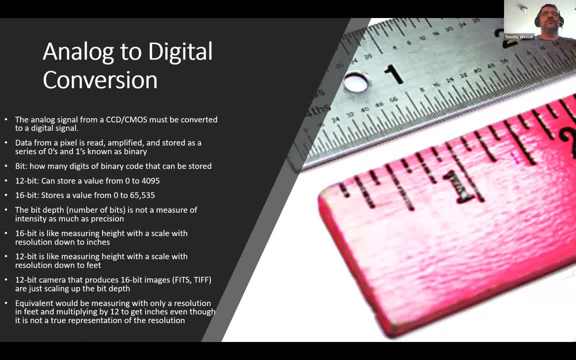 is stored. everything is stored is basically as zeros and ones, and the more resolution or the more brightness resolution that you get out of the your camera, it what. the amount depends on how many of those zeros and ones you have distorted information in. sometimes you have 12 bits, sometimes it would, or. 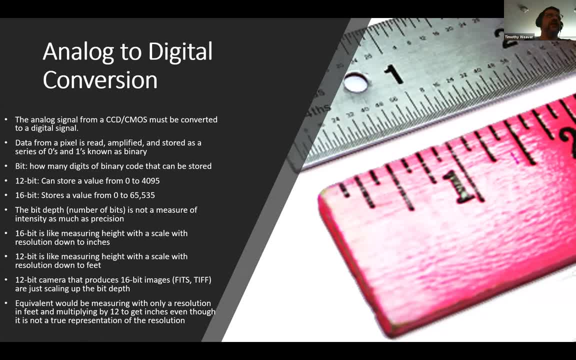 at least with this. with some, a lot of the CMOS cameras you have 12 bit and some of them are some of the. the DSLRs are 14 bit, but a lot of your CC, your astronomy CCDs, are 16 bit. so with a 12 bit you can store values from 0 to 4,000. 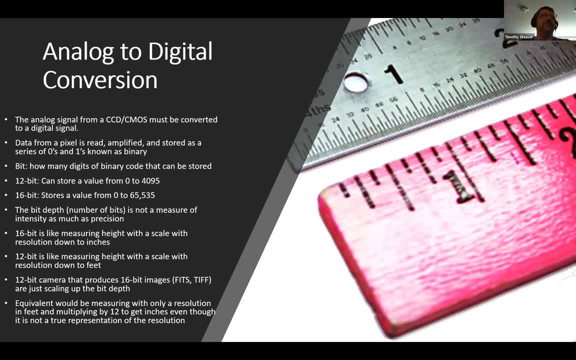 95 for 16 bit. you can store from 0 to 6, 65,530, 5. this is not a minute, it's not really a measurement of intensity, but it measures the you, the units between. there is more of a resolution. at best, the best analogy would be having a having, a having. 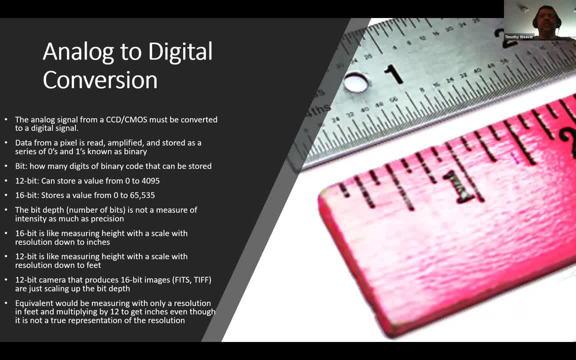 a meant something that measures in in Feet versus something that measures in in inches, Like if you had a measuring tape that only measures in feet. So if you measure somebody's height, you measure. okay. if they're five foot four, all you can measure them is at five feet. 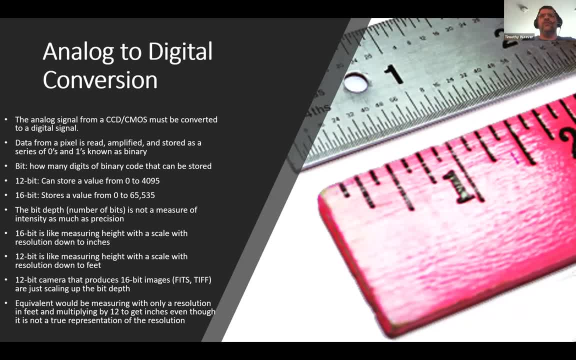 or six feet, So you can either round up or round down, or round to the nearest foot. You don't get a real, you don't really get a, you don't really get an accurate measure with them. On the other hand, if you have a measuring tape that you can measure in inches, you can get down to five, four. 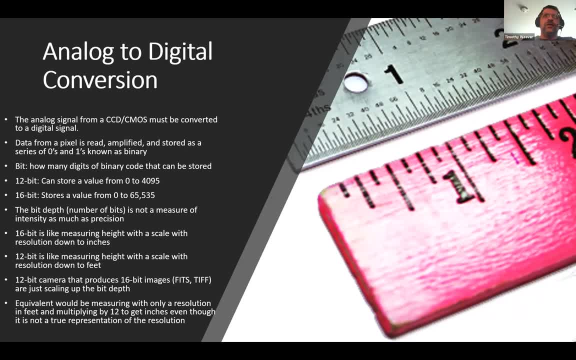 or five, seven or six, three, And your 12-bit would be the one would be the measuring tape that only measures in feet, Whereas the CCD, the 16-bit camera, would be the one that measures in inches. Now, whenever you submit your data to AABSO, it's all going to be in 16-bit. Now that? 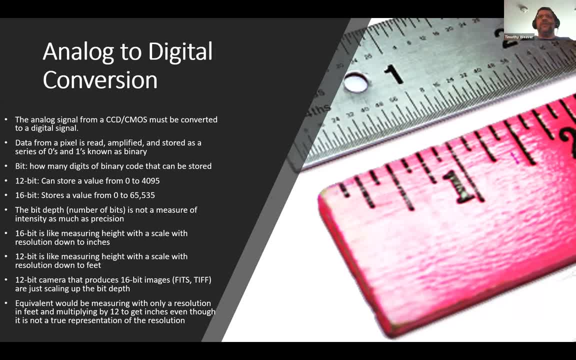 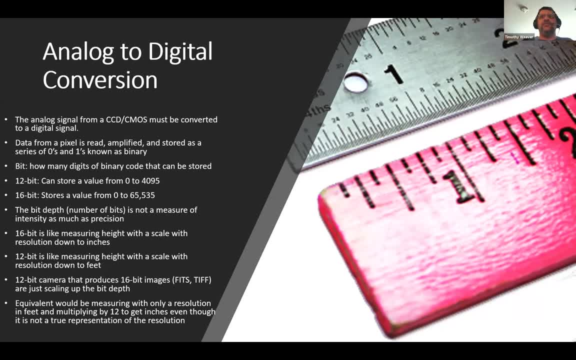 that value, that that 80, that analog digital unit by 16.. So you go from a 12-bit to 12-bit to 16-bit. but that's not really. it's not really that accurate. The equivalent would be to take: 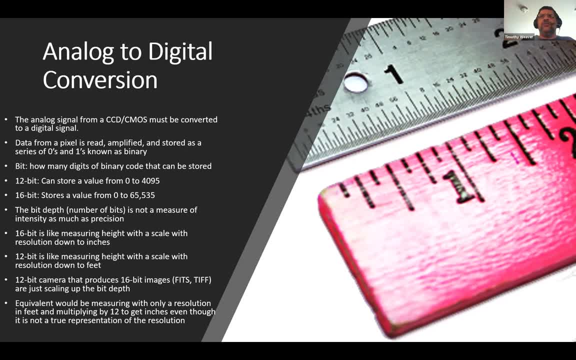 the. take the, the tape measure that measures only in feet, and then multiply by 12. You won't. you won't get any. it won't be any more accurate, But instead what you'll have is a bunch of people that's going to be measured in 60 inches and 72 inches and 48 inches. So all you've done. 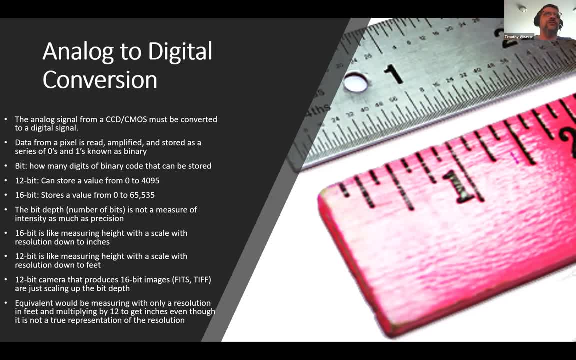 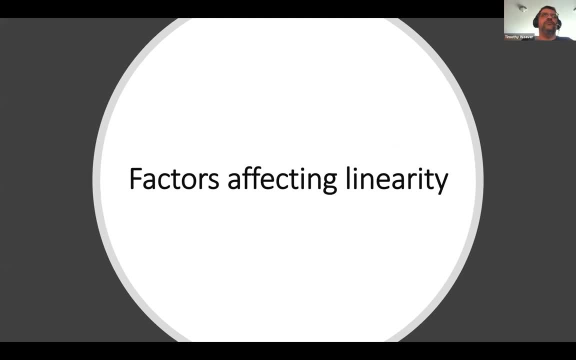 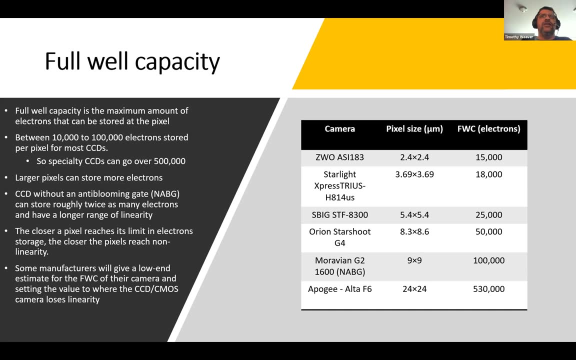 is: take the foot and multiply it by 12 to get it to get inches. Now here's some of the factors that affect lineality. All right, full well. capacity. This is the amount. this is the now, this is actual measure of intensity, or how much intensity you can measure. 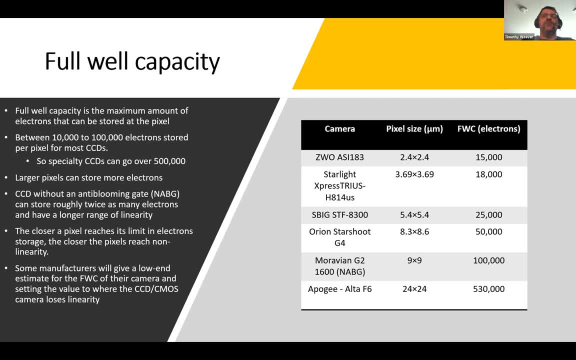 All right, whenever your your CCD camera, what it measures is electron. basically, The photons are just the is all right, it's supposed to be measuring photons, but, but when? but the? but your analog digital unit is measuring the electrons that that you, that you get from. 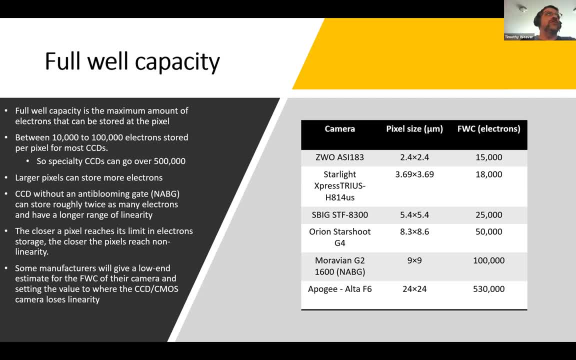 whenever the photons hit the pixel. So the high, so the larger the full well capacity, the more, the more photons you can store, I mean the more electrons you can store, And this is usually in proportion to the size of the pixel. Bigger pixels will hold more, hold more electrons. 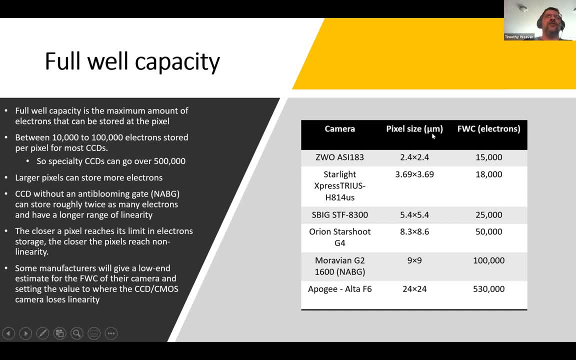 And here you see a chart showing a pixel size all measured in microns, or one one thousandths of a millimeter, to show how small they are. And it can go all the way up to 24 by 24 microns. 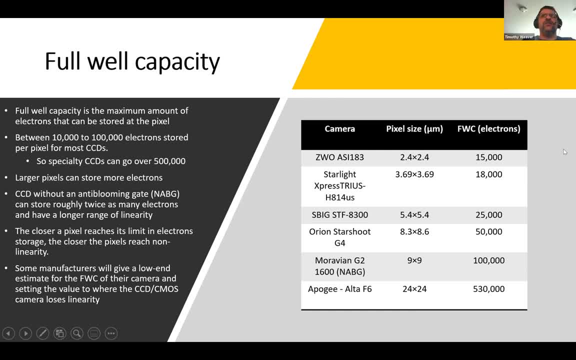 Now most of your, most of your regular CCD and CMOS cameras are going to be are going to measure in the range of 10,000 to 100,000 electrons for each of those pixels, Though there is the exception- the Apogee Alpha F6, that's an example of one that could hold up. 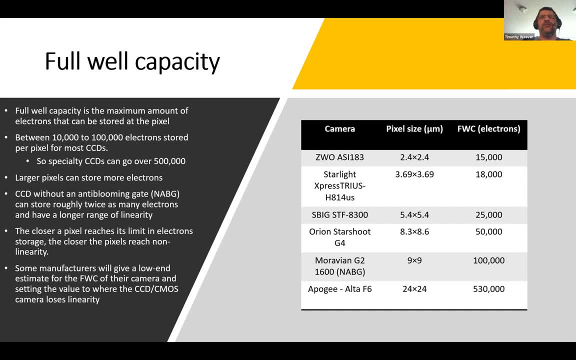 to like 500,000, but that's because the pixels are. you can actually hold at least. you can hold at least a dozen pixels in one of their pixels, from even one of the cameras for one of the larger pixels. Now CCDs have something known. now there are some CCD cameras that can hold twice as. 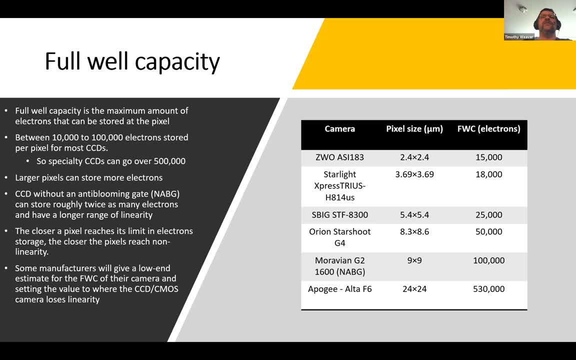 many pixels than a comparable camera. with the same, they can hold the same amount of electrons. they can store the same amount of electrons in their pixels as a comparable CCD camera. and the reason why is there is something called an anti-blooming gate. What happens is whenever 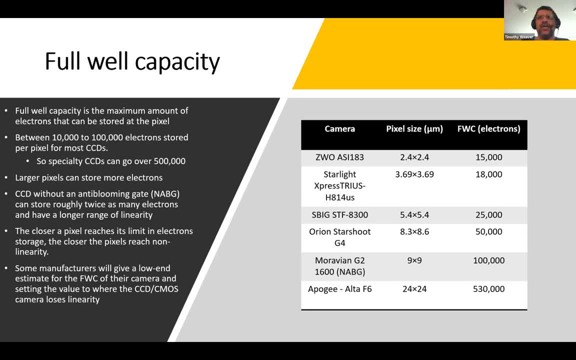 that pixel becomes saturated. if you don't have an anti-blooming gate, then the electrons will bleed over to the pixel next over. Now you may seem like, well, we don't want that one because it's going to just mess up. 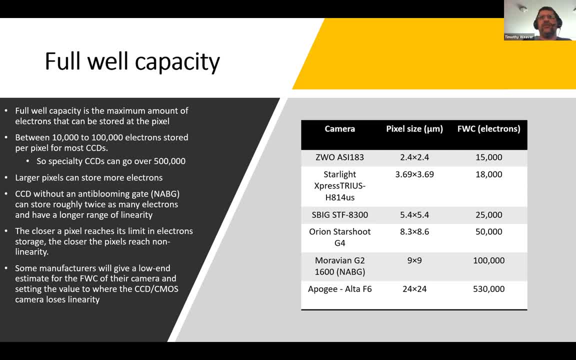 the image that we take. it's going to bleed over into that next star over. but the advantage to a CCD camera with a non-anti-blooming gate is it has greater lineality and it can store twice as many pixels. you just have to be careful not to oversaturate. 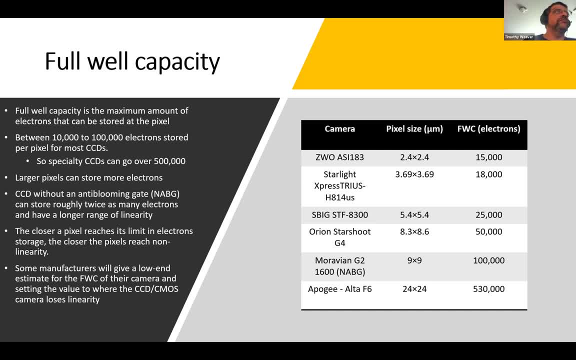 your pixel Now with some- now some- manufacturers, they will give you a low ball estimate on the full wealth capability of a camera. The reason why that is lineality. Their camera is linear up to a certain point and then everything becomes non-linear. So what they do is they give you the full wealth. 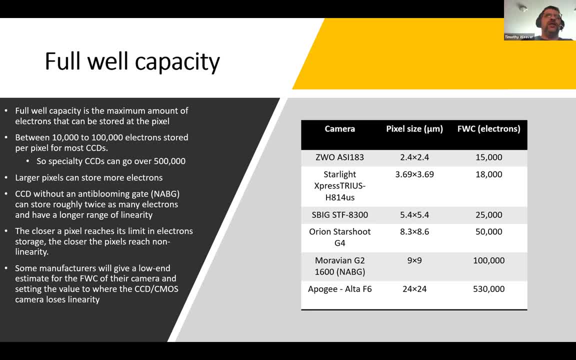 the camera can actually hold the full wealth, but the camera can't hold the full wealth. more pixels but it, but then, but then the relationship, but then it would start being a non-linear Quantum efficiency. This is just the. 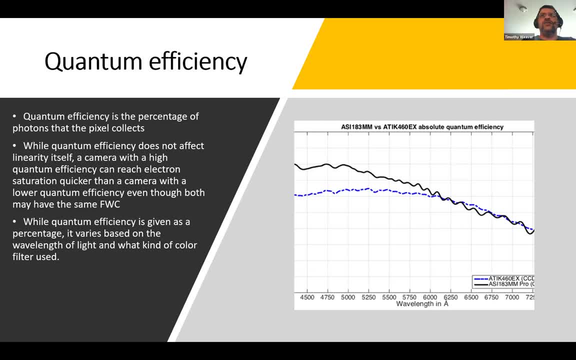 this is how efficient your, your, your CCD camera, can absorb photons. You, you have a certain percentage of your photons that will actually be absorbed by the CCD camera, And others they're not going to be. they're not going to read on there. 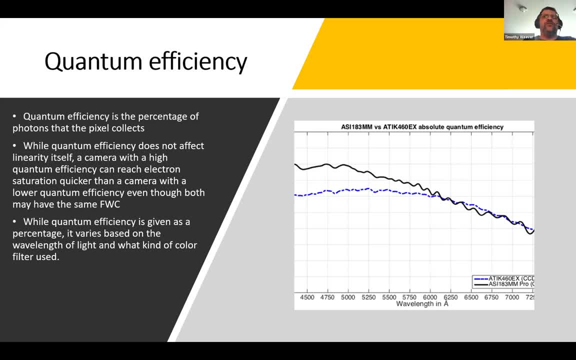 Now you'll get a certain number, Now you get a plain, flat number for it, Like like one of mine, the, the ones that I'm going to show you later, which I did the lineality test on. they give an 80% quantum efficiency, but that's it. But that 80% really is for one wavelength of photon. I mean one wavelength of light. 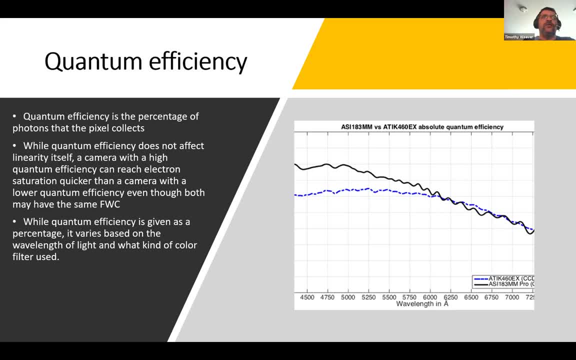 Over other wavelengths. it's not as efficient, But typically it'd probably be more accurate if they were to integrate the, The quantum efficiency, across the entire wavelength. At least it is to me. It will be a more accurate measurement, but they don't do it that way, So you have to be careful with that. 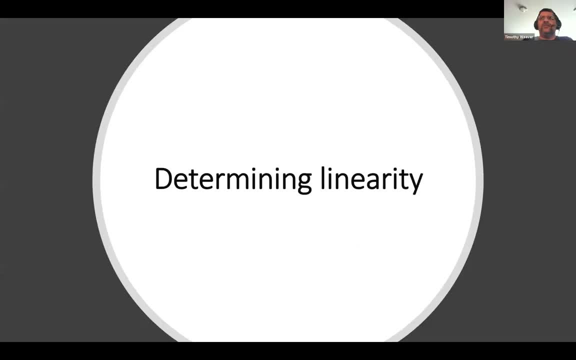 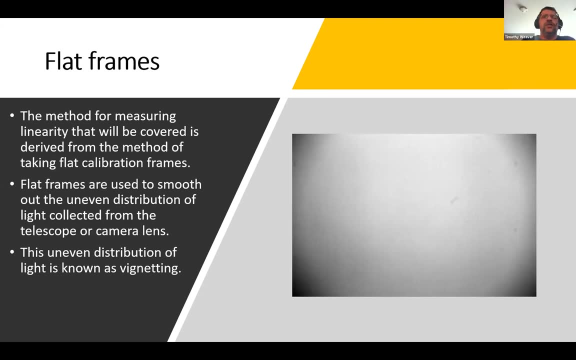 All right, determining lineality. Okay, I I took a pretty much a bare-bone approach to that, And what I did was the same thing you do with taking flat frames. The speaker before me was talking about taking flat frames. Flat frames are a very complex thing to do. 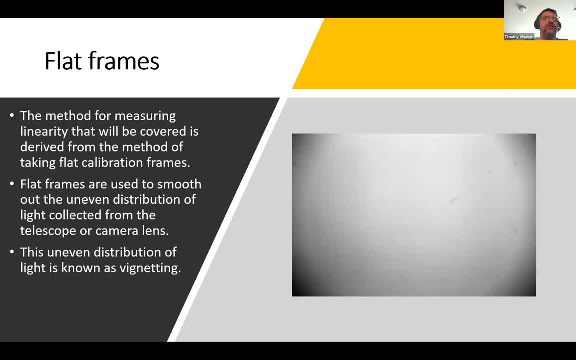 taking flat frames. Flat frames is just a way of dealing with the uneven collection of light in a telescope, mirror or lens. So if you can see this picture right here, the light is not evenly distributed and there is some variation in the light, particularly in the corners. The corners look real. 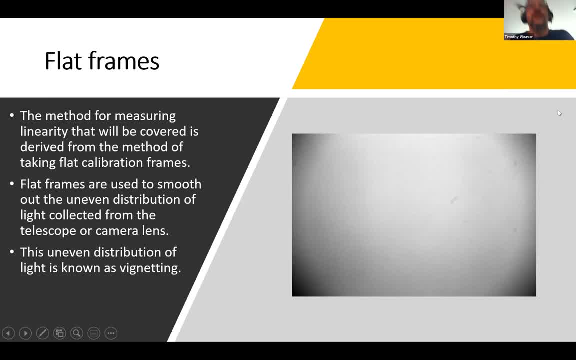 dark, That is known as the netting, And to correct for that you take flat frames And the flat frame will calibrate your images to correct for that uneven distribution of the light. It's also good for detecting dust particles, also for calibrating for dust. 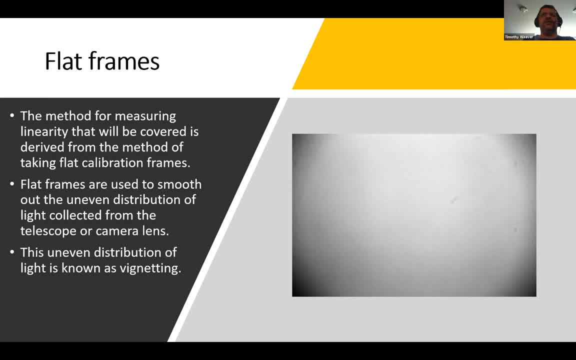 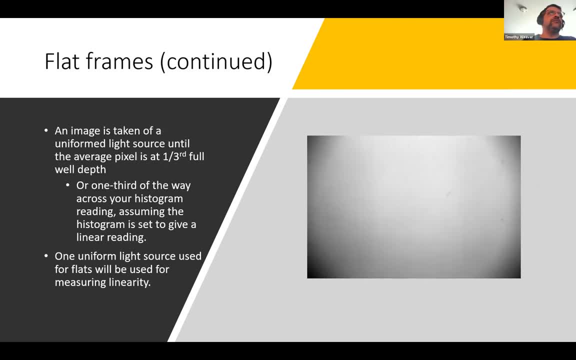 particles that would wind up on your CCD sensor or on the lens. The ones that are in the background are the filters, and you can see that that's the ones that are being calibrated. Okay, so what you do is you usewhat I use is a light box or a flat box, and 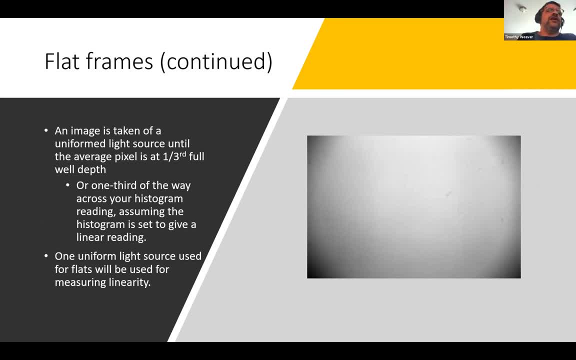 what I do is I take the image until it averages at 1-third full well depth. So whenever the image averages out at about 0.1 mm, it really is 1-1.2 mm, because this is an exact same image. So it's not going to be that black and white, but it's going to give you the same point of view. 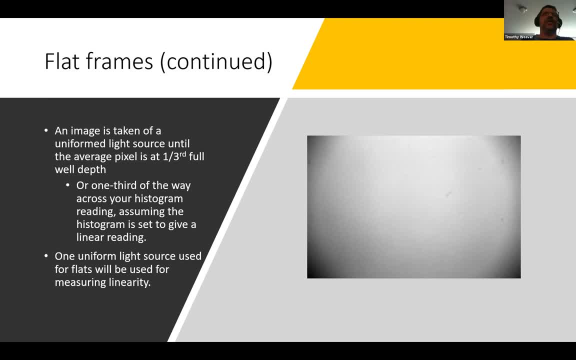 I take the image until it averages at at 1-3 mm, So it's going to give you the same point of view. one-third of the, I guess, the ADU count I'm then, and then then that's, that would be them, that would be the amount of exposure I would. I would, uh, I would have. 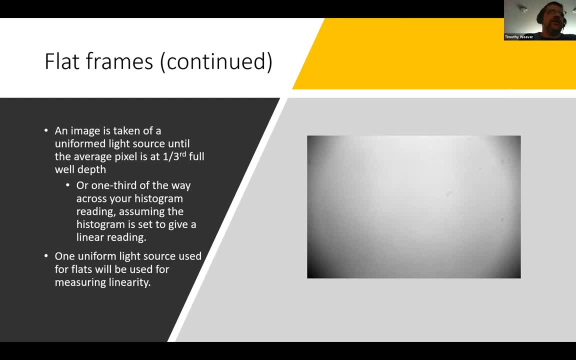 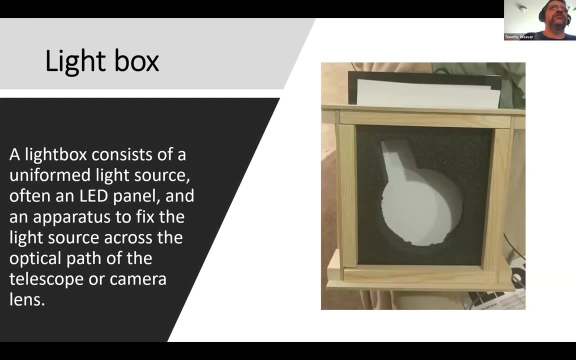 for that picture, for that image, and then I would average out all the, then would average out the all the flat range, because I would. I would take about like 15 of them, and this is two minutes left. okay, this is my light box right here. okay, this is a home, this is something I made at home and all I would do is since: 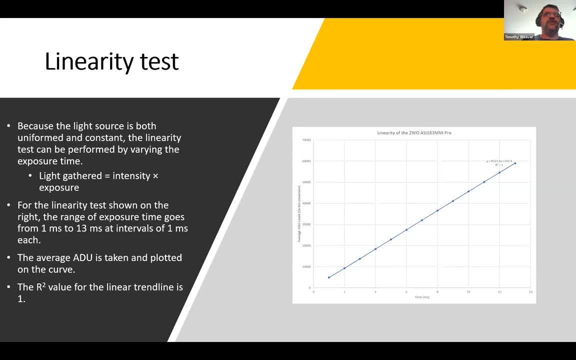 I have a uniform source of light. all I have to do is vary the exposure time, and this is for a ZWO ASI 183 monochrome camera. the time is in measured in milliseconds and I measured out the average ADU count after it's been convert, converged with: 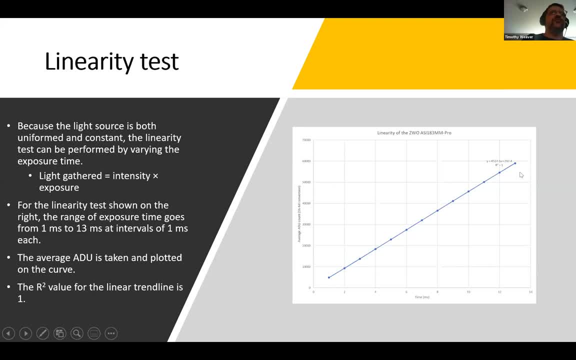 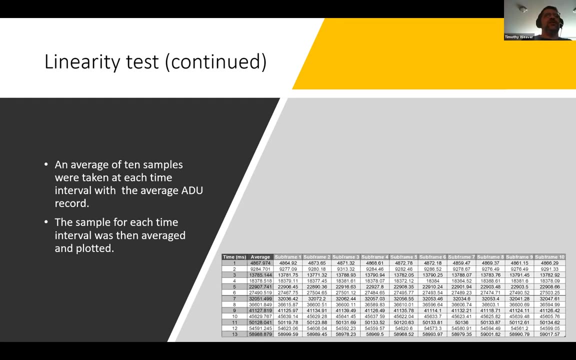 16-bit image and you see it's a pretty much a straight line, right? and I didn't just take one image I took at. I took ten exposures. I mean I took ten images and each at a interval of one millisecond in exposure. so I took, took a set of ten at. 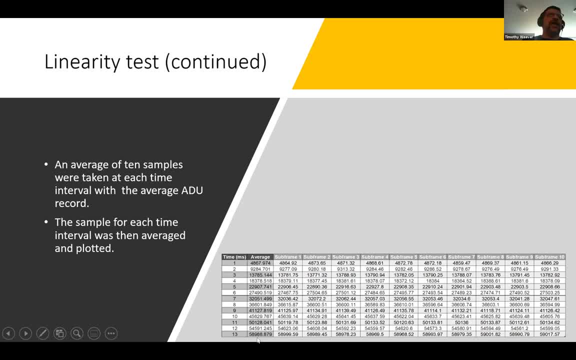 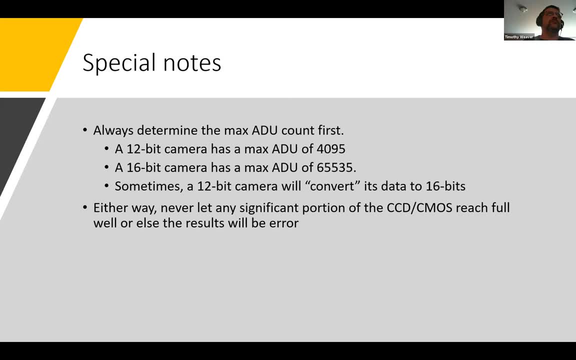 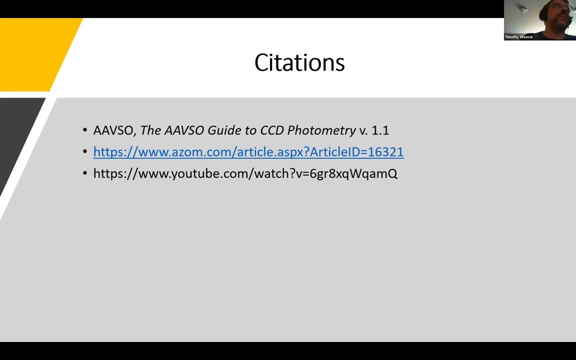 one millisecond, a set of ten at two milliseconds, so on averaged them out and I plotted them on there on the graph, all right, and here's my site. here's some. here's some my sources, that I've some my sources that I use for this, for the presentation. 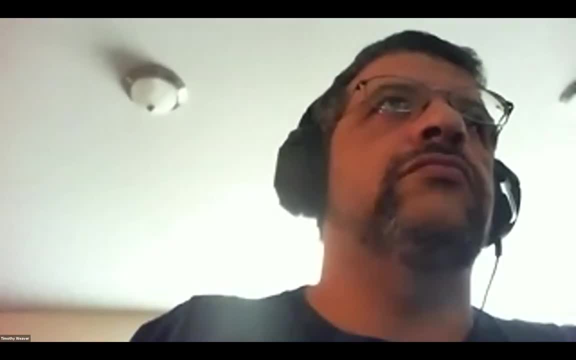 alright, because I'm, as I'm, ready to go. John, that's what we came to do. then chose myいや. I want to provide if you'd go ahead and see if you can find my father's wireless 812 controller. you know, don't be correct. 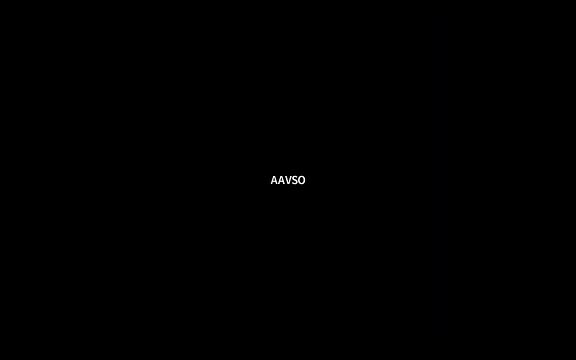 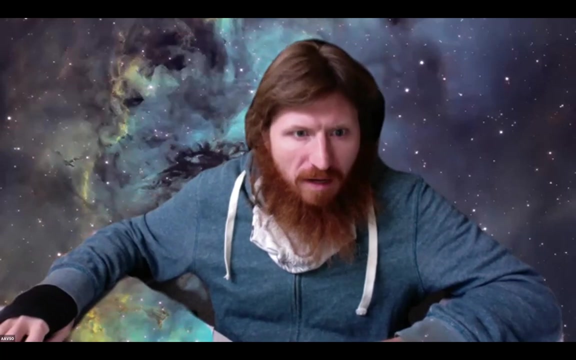 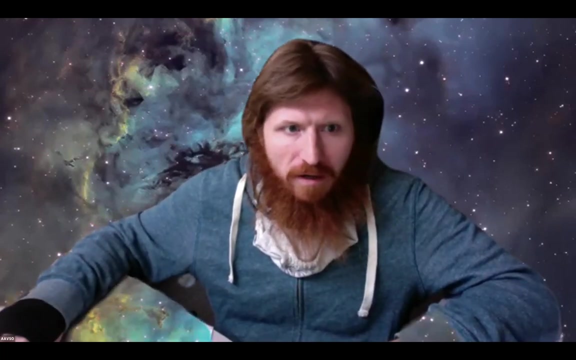 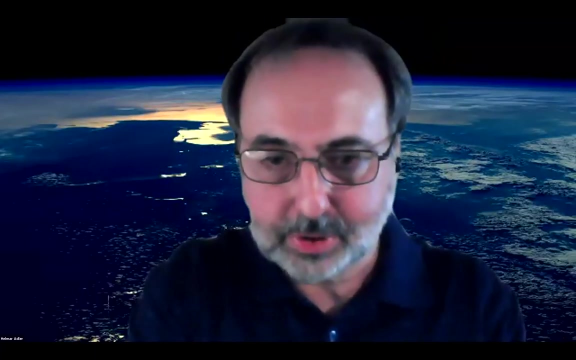 all right, I'm done, unless you got any questions. yeah thanks. so next up, we actually have a final addition to the Astro makers section, which is Helmar, in which is inside Helmar and the last thing I wanted to want to 것 explaining the Thanks, Bert. Hello everybody, Let me share the screen. 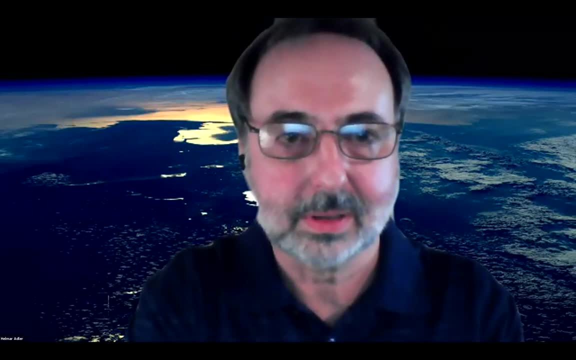 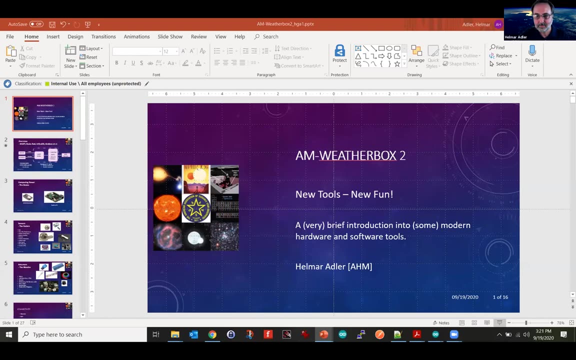 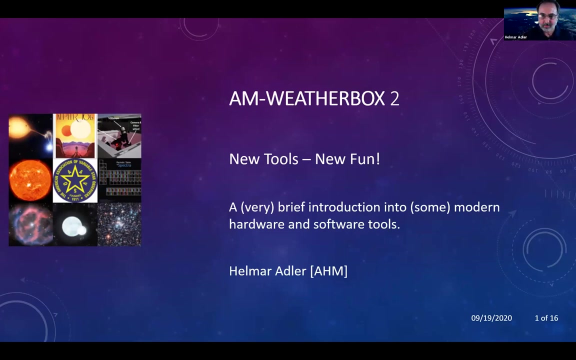 Can you see the screen? Okay, I would like actually to follow up on what Alan gave before his talk, before I was asked to talk a little bit about what I'm doing, We have independently worked on what we sometimes call the weather box. 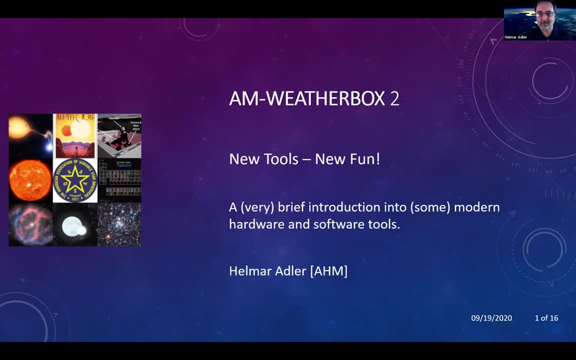 So, again, that is a safety gadget to make sure that our telescopes are not getting rained on Or that we can take images which are not obstructed by clouds, for example. So I was for a long time. I was thinking about: what is it what I should be talking about? 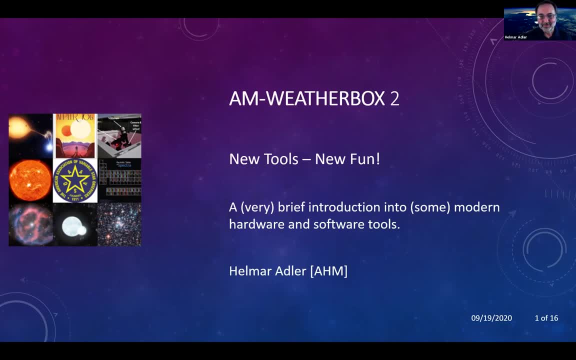 I don't want to duplicate what other people have done already, So I call this new tools, new fun. We are in the at an age right now where the Internet of Things is exploding. There are a lot of open source Software solutions around which we should be utilizing. 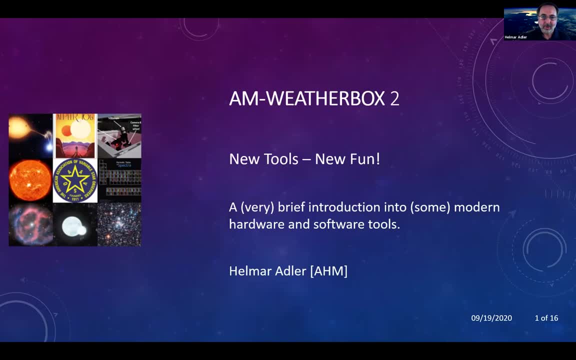 There was a lot of hardware developed which we could be using. It's getting cheaper and cheaper and more powerful. So what I would like to give you is a very brief introduction to some of the possibilities we have in regard to hardware and software tools. 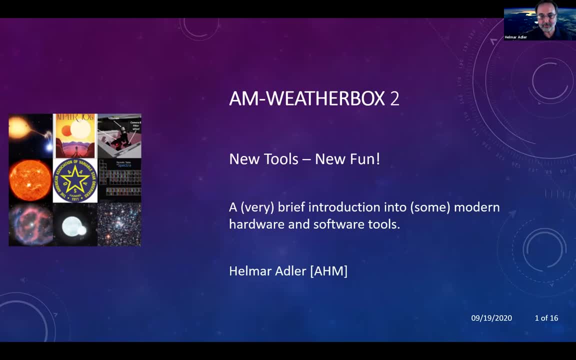 I have been a member of the AAVSO. I found out Today for 10 years. in two days, I have my own observatory in the backyard and I know what the problems are. I'm, at the same time, one of the operators of the telescope network which the AAVSO. 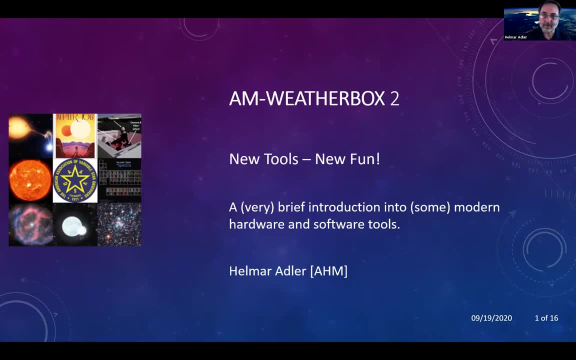 is running, and I can feel how difficult it is sometimes to really control telescopes remotely, Where you don't the backyard to change things around or make sure things are not happening, but you solely depend on the remote functionality of your equipment. So let 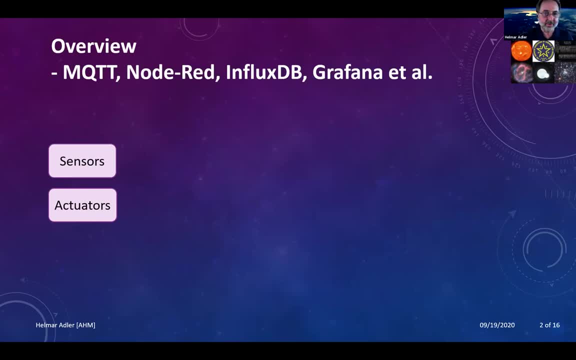 me start, and I apologize for these animations here, but I thought it might be one time when PowerPoint presentations with animations might be useful. So let's think about what we want to achieve in a system which we want to automate and remotely control. There are several use cases. if you want, Think about you. 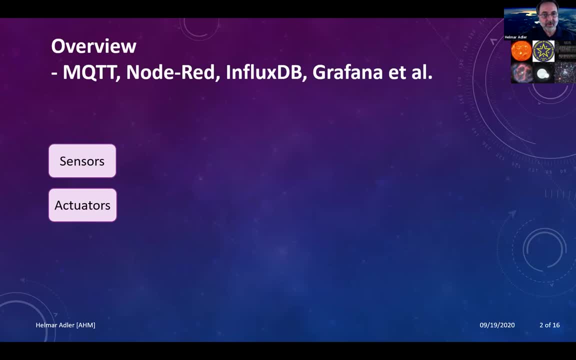 have an observatory which gets hot in summer. You want to switch on a fan- very simple. You have sensors there, you have a thermometer and at some point you reach a threshold and you want to use, use a fan to cool down things. So we have sensors, we have actuators and somehow they 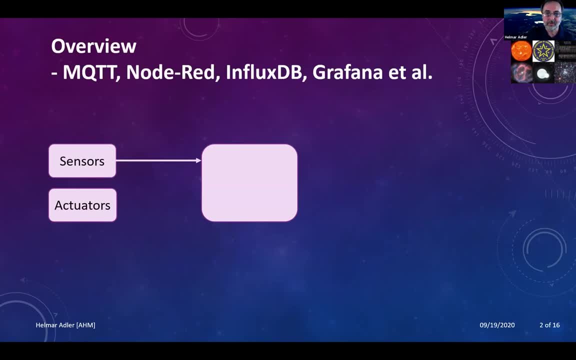 need to communicate with one another And you will have a unit which takes all these data measurements and distributes them to the actuators. Keep in mind again: we could use cloud sensors, we could use relays as actuators- all sorts of things can happen. 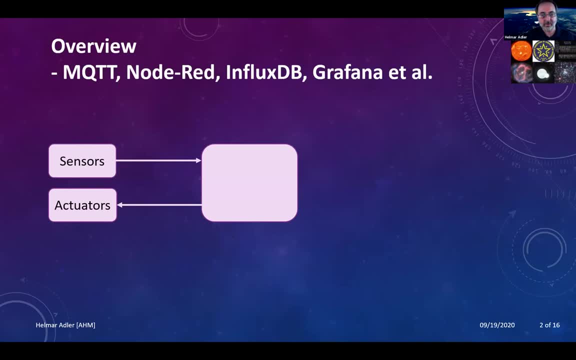 and is very interesting to do in the background. What I have been using lately is something what is called a network protocol, which is called MQTT Long word. it's messaging queuing, telemetry transport. It is actually a very nice publish and subscribe network model that. 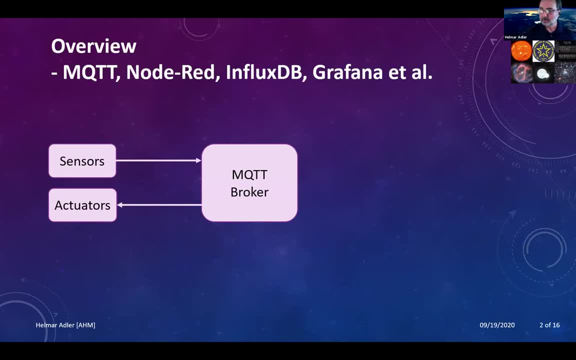 makes it possible. That allows. That allows small devices like Arduinos to talk to one another in an easy way, without too much overhead. It has a very small footprint as what code is concerned. So in the MQTT talk, you call something: what the sensors are sending out, you're publishing. 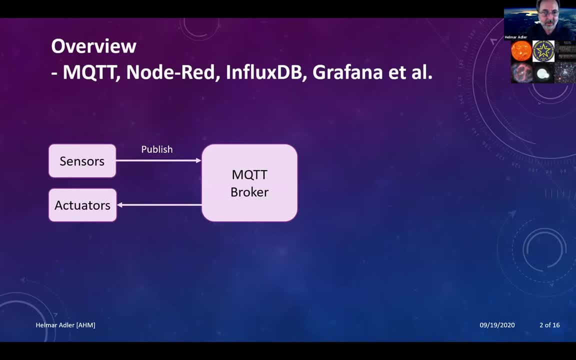 you're publishing a topic And then you have other embedded controllers, for example, who can, Who can sign, subscribe to those topics, And all that is distributed by these MQTT brokers, which is another item in this little network. But then, if you have all these data, you might. 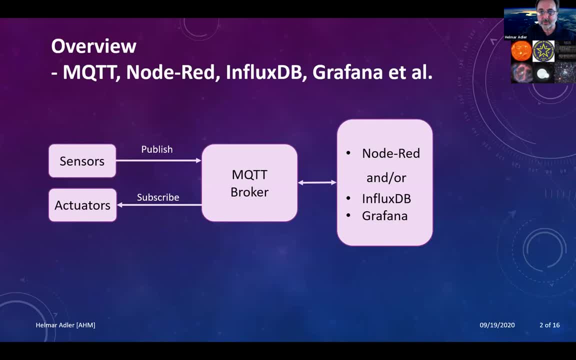 like to put them into a database, And there are lots of tools around. They're all open source. There is InfluxDB- has become pretty well known lately- and Grafana InfluxDB, as the name says, is a database. 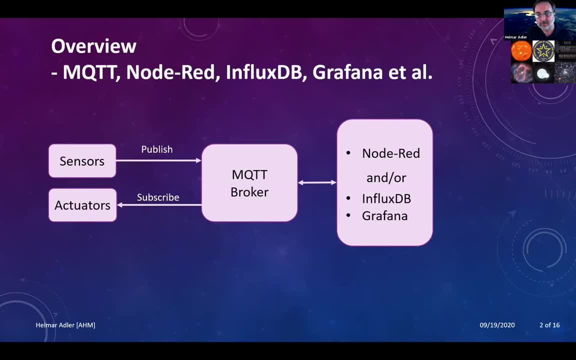 Grafana is a visualization tool which allows you to send out alarms and alerts at the same time, And I have been using for prototyping something what's called Node-RED, And I would like to show you a little bit about this one later on. 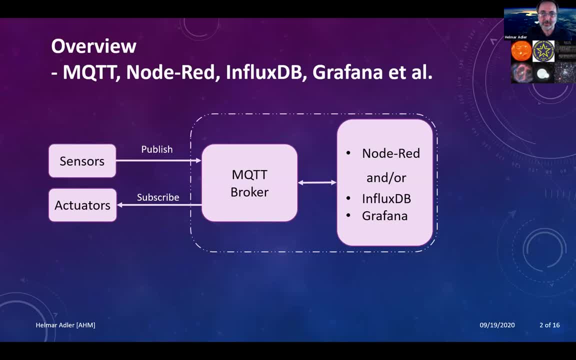 All these MQTT broker pieces of software- Node-RED, InfluxDB and Grafana- they all fit onto a Raspberry Pi. I'm not sure if we have mentioned the Raspberry Pi before Arduino's Raspberry Pis. they work very well together. 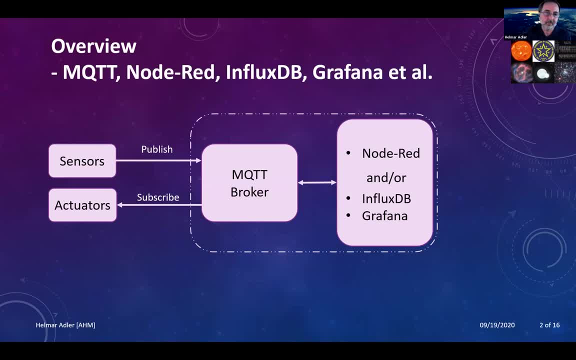 Relatively low cost. The embedded controllers I would like to introduce to you are even less expensive than the Arduino's, And they have Wi-Fi capabilities, So at some point we even want to utilize web services. For example, we could go and find: 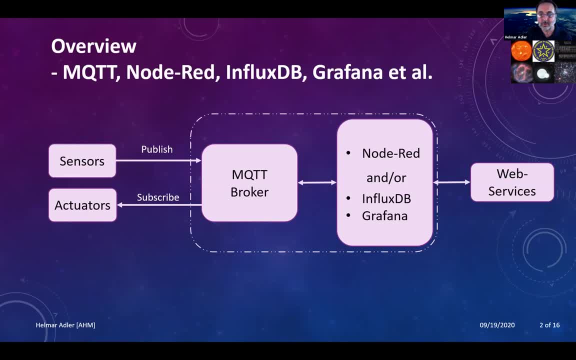 whether reports, whether forecasts, which we could utilize, or we want to send out emails, SMS messages. All this is possible literally on your desktop or in your backyard. The controllers: embedded controllers for sensors and actuators controls, as I mentioned before. I would like to introduce you to some. 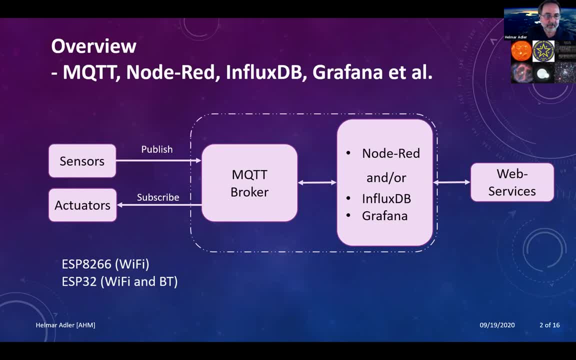 which are made by a Chinese company called Expressiv. They are ESP8266,, very well known in the hacker community, And they provide Wi-Fi connectivity, and the ESP32,, which is sort of the follow-up of that smaller device And that has actually Wi-Fi and Bluetooth and is a dual-core model. They're very inexpensive. The ESP8266 you can get for about two to three dollars, The ESP332 maybe double the price And you can get whole lots of 10, for example, if you are a little patient from China. Alibaba is a very good source for those. 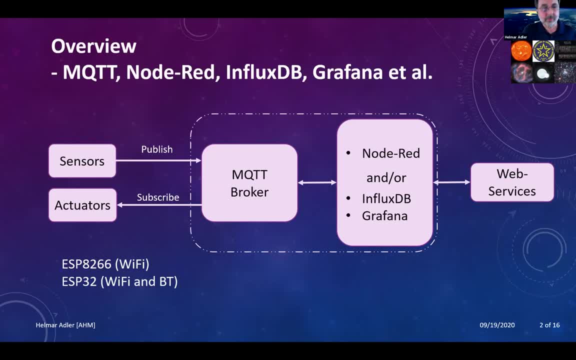 And you get 10 for about 20 dollars, which I saw yesterday, And if there is a ridiculously low price you can distribute them into in your backyard or somewhere else in the observatory And you can make a little Wi-Fi network. 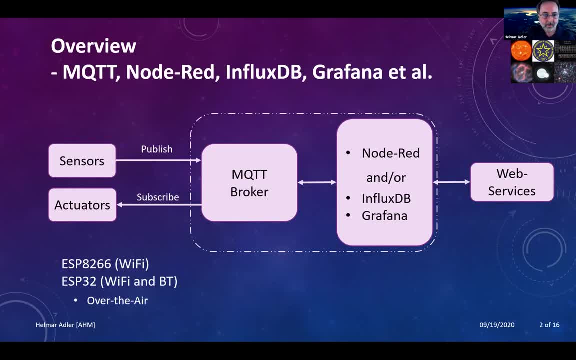 So I would like to introduce you to them. I would like to show you a few things, what you can do with them. Very important here is over-the-air programming, So instead of having a USB connection or an Ethernet connection, something like this, you can do everything wirelessly. 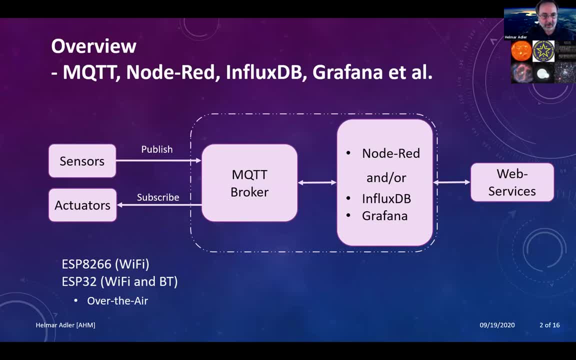 So your new firmware which you're developing, you can distribute over the air. If you have one of these little devices at a place which you cannot get to easily, maybe under your roof or in a very, very small space, you can distribute it over the air. 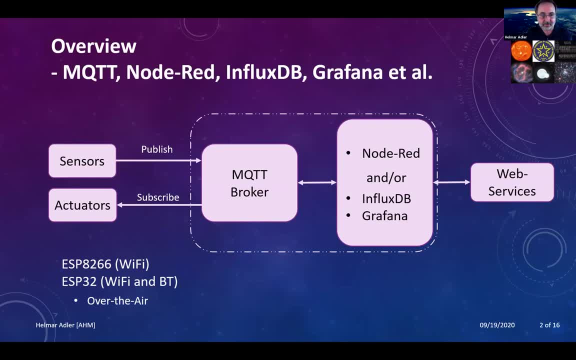 In a very far corner in your observatory. Those are devices to get and over the air will help you just to update the firmware. I mentioned already the Raspberry Pis. They have Wi-Fi capabilities And instead of like in the olden days where you use all sorts of software. 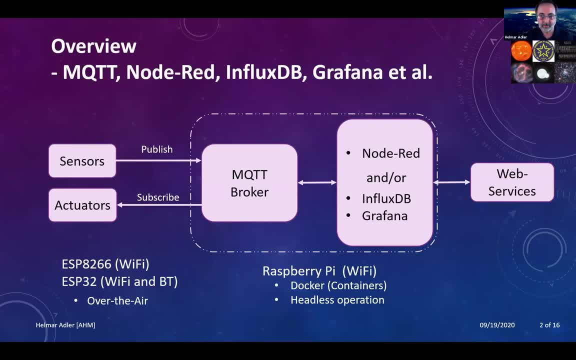 which you have to download first to your Raspberry Pi manually. we use now container solutions, And one is, for example, NET. You can look this up on the web. There are people who are already doing a lot of things for you. 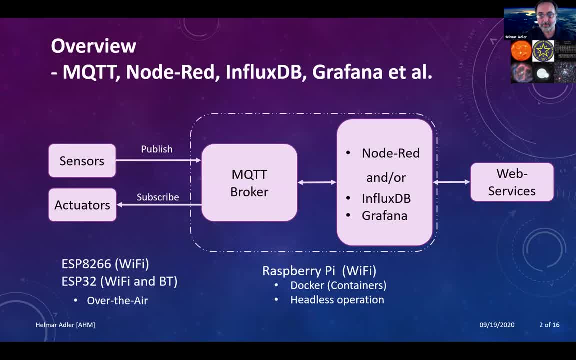 You can download those containers which contain all these software packages already. It's very useful if you want to work fast and if you want to update those packages- And they come with maybe 20 different pieces of software. You don't need to do that manually anymore. 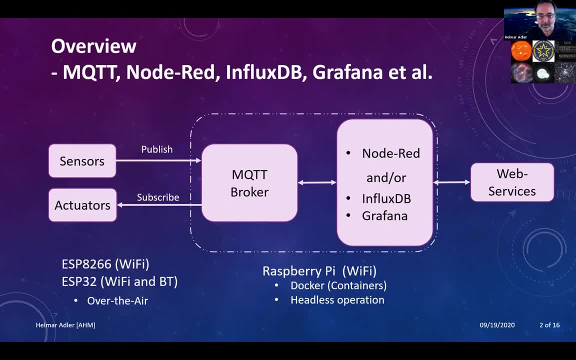 Important too is you can run the Raspberry Pi Without connecting a monitor or a keyboard to it. in what is called headless operation. You use a web browser, you hook up, log on to this, and then you can use the keyboard on your laptop, for example, and operate your Raspberry Pi. 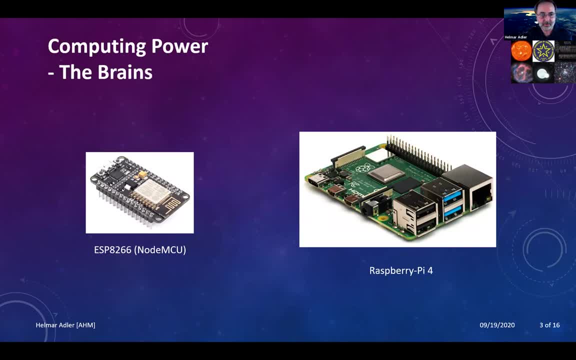 Here are two pictures. On the left is the ESP8266.. You see it's pretty small And the silverish thing there In the bigger chip is what makes the heart of that development kit what it actually is. Those kits are very useful because they typically provide USB connection. 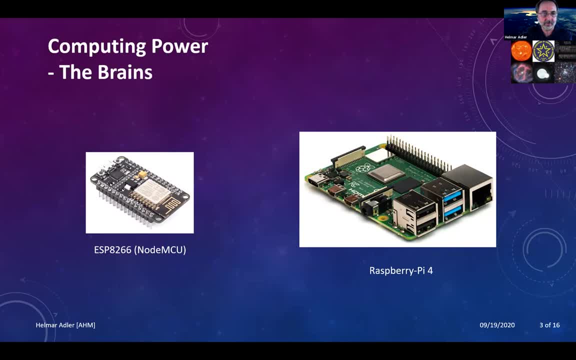 which is the first time you program these. It's very important and it supplies power as well. Raspberry Pi 4 is now the version 4 on the right side. They provide USB connectivity, Ethernet connections, They have monitor connections, et cetera, et cetera. 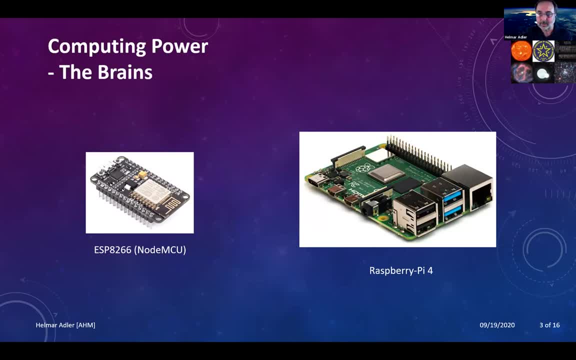 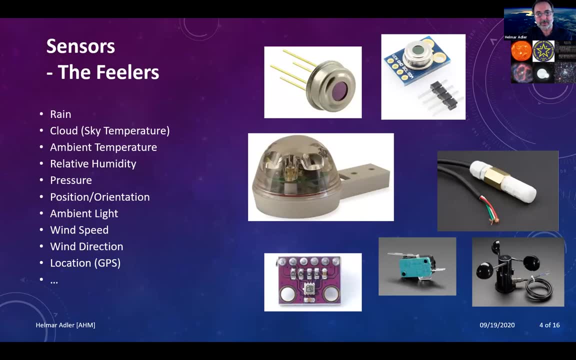 Very powerful. these days You actually can build your own little PC if you wanted to. Here is something I don't want to repeat what Alan has already shown: The sensors- I call them here the feelers. There are lots of possibilities. We can look for rain. 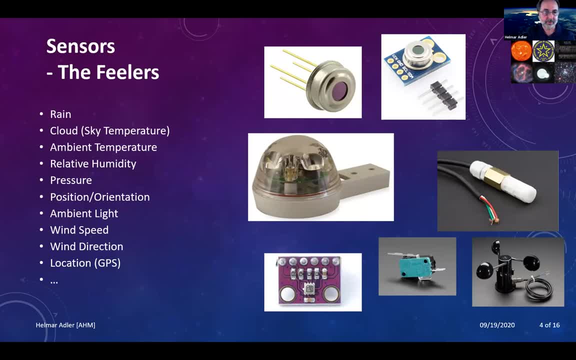 We can look for clouds We can look for. if you are interested in the weather for relative humidity and pressure, You can think about positions and orientations of the telescope itself. Sometimes, as a safety precaution, we don't want to run with our instrument into some obstacles. 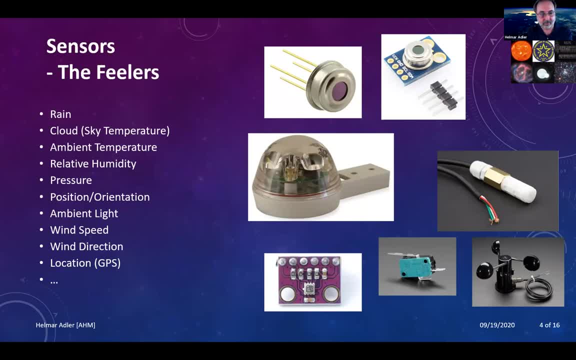 We can look for the ambient light and we can if we have a setup where we have to, where we move around with our mount, we can put a GPS unit on, And all of these are our sensors which we can use in our environment. 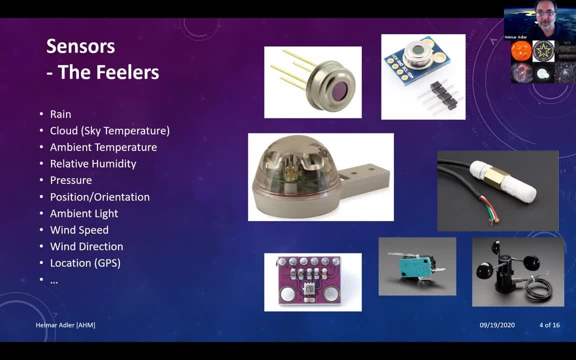 If your picture see on top is again is the infrared sensor To look at the clouds working at 10 microns. The rain sensor- I had used the same rain sensor as Alan showed before. Then there are very good temperature and relative humidity sensors around. 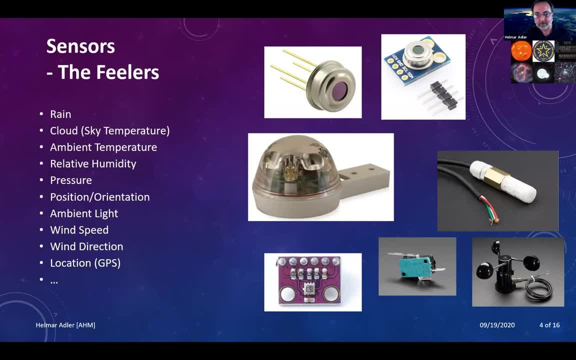 which are already enclosed, which is quite important, Because if you put your instruments into the elements, it's a very different story if you do something on a breadboard Or if you put them out into the weather conditions. Here in the northeast we have pretty hot and humid summers and very cool winters. 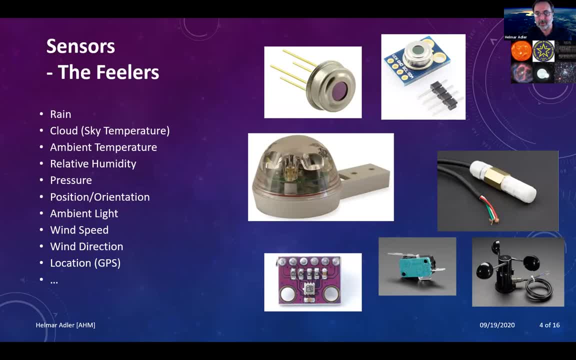 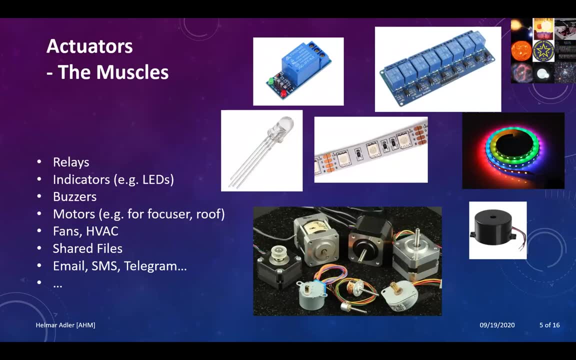 The instruments have to be protected quite well, So it's good if you can find those already assembled. You have about two minutes. Okay, Here are some actuators: the muscles relays. We can drive those. We can use LEDs as indicators or maybe for our. 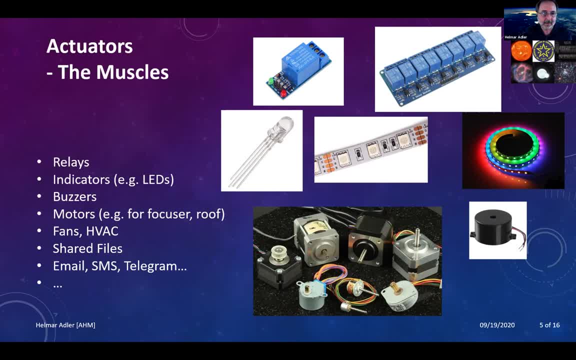 flat panel illumination. We can use fans or we can use, for example, motors. Here is a little one. If you look on the bottom of this picture, there are a couple of stepper motors And you can build your own focusing devices with those to do autofocus on your telescope. 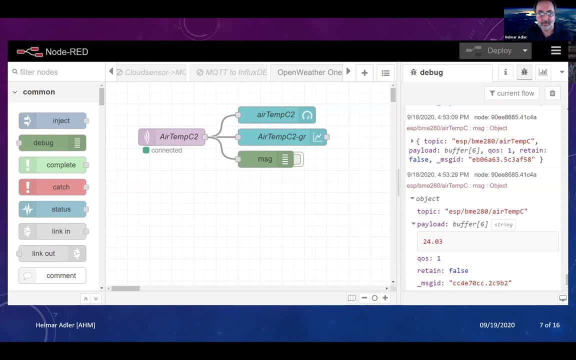 I will just show you a little, a few pictures of Node-RED. Node-RED is an environment Which is what is called a flow-based development. It's a low-code development tool as well. You don't write now single lines of codes. 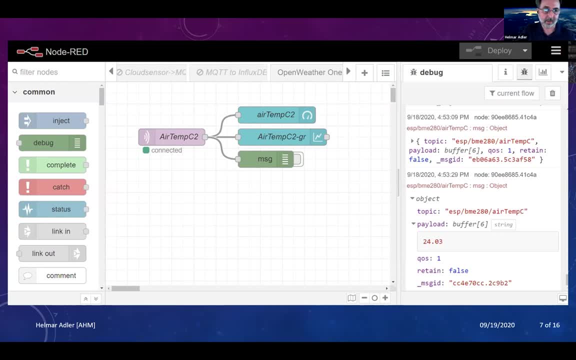 But you use, for example, these rectangular nodes And you have to define, if you double-click on those, what these nodes are supposed to do. There is what you see here: The air temperatures You see is actually an MQTT input node. 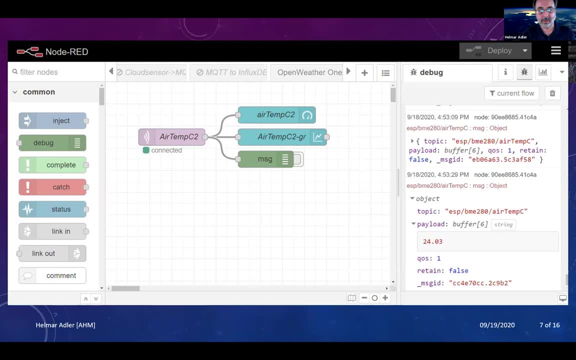 And it takes the data And you can connect now other gauges, graphs, icons to that node And it provides the message. And if you look here at the left side, you see what one of those messages is. Here is ESP. 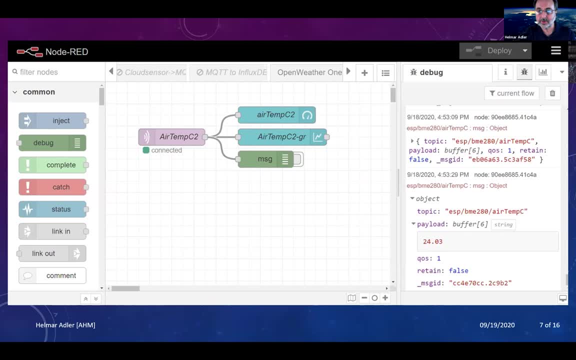 BME280 is the type of a sensor I use. It's the Bosch sensor Which provides environment Or mental temperature, humidity and pressure values, And it provides this is what MQTT uses as a topic And it gives that message. 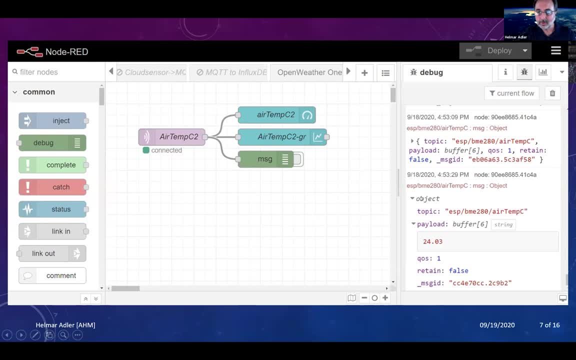 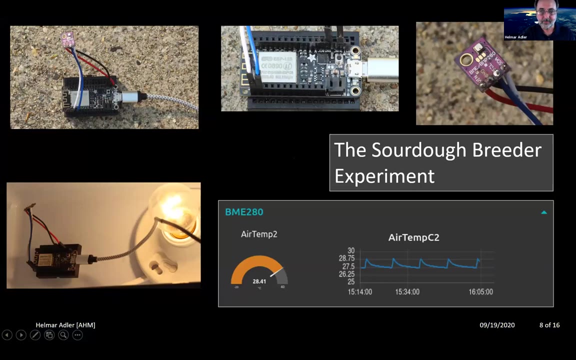 And if you open these different objects here and the payloads here, you see actually a temperature And this is the message which will be given through these wires to the gauges Or the graphs Here. briefly, I did something with the top left. 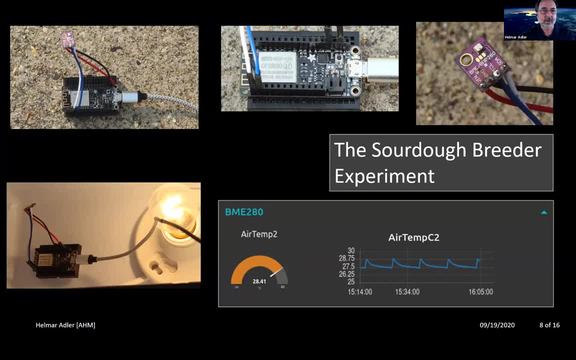 You see here an ESP8266 with the environmental sensor And I call this the sourdough breeder experiment. Like everybody else, I was baking more than usual during the COVID-19 phase And my sourdough didn't develop too well. 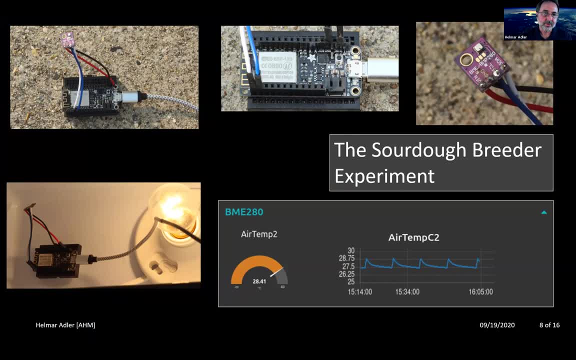 So I used one of these nodes, These little ESP8266 plus the sensor nodes, And put them into an icebox, Put a light source in there. It's an incandescent lamp Which can be switched on and off. Now I can regulate my temperature. 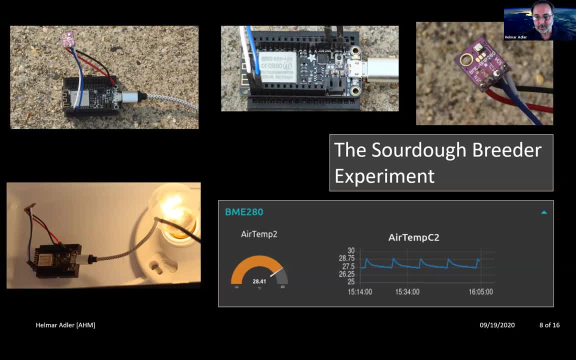 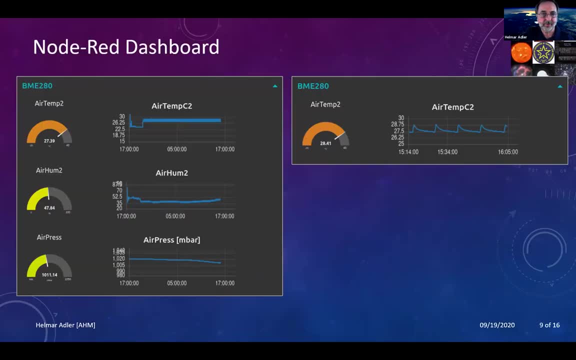 And you see on the bottom one of those regulated temperature curves, And I elevated the temperature And now my sourdough is actually working much better than before. Now here's something that's a little more special, A little more serious. Here is where you can see a display of the air temperature, the air humidity and the air pressure. 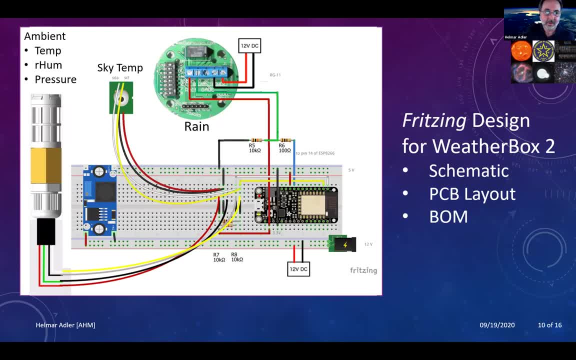 Coming back to the weather box and the sensors for cloud, rain, etc. Here is something that I wanted to show to you What we can use. It's a fritzing design. Fritzing is a piece of software which allows you to make these drawings. 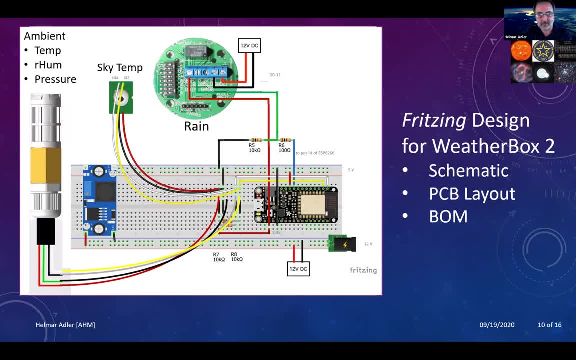 It's very helpful. It's very helpful if you use breadboards, for example, and you want to wire things together. Sometimes it's easier just to make these drawings first, because, before you start to sort it, That piece of software allows you to make these schematics. 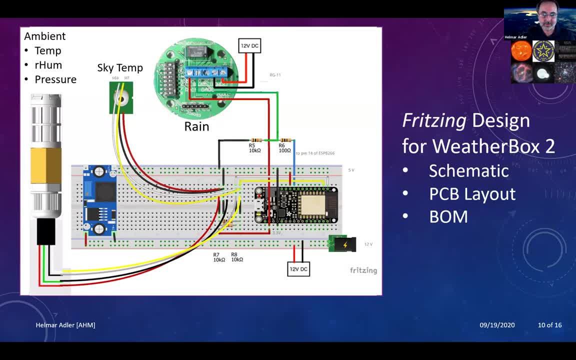 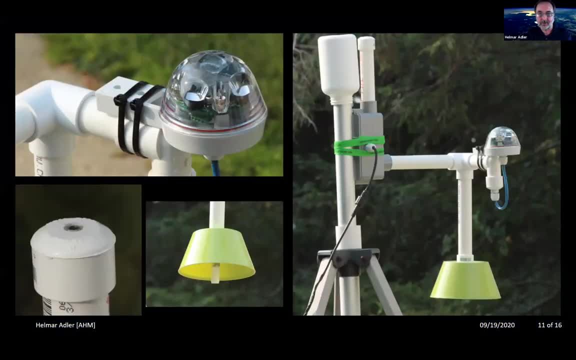 It actually provides PCB layouts without routers And it provides a BOM, Very useful if you want to share things later on. Here are a couple of pictures of what I have in my backyard. Here is a very different footprint than what Alan had before for his weather box. 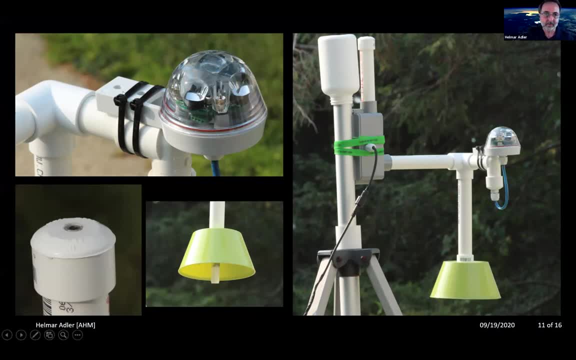 And you can see here the rain sensor, of course. Here is the tip of the infrared sensor which is looking towards the sky. Here is my temperature and humidity pressure. No, it's a temperature and humidity sensor And I made an experiment. 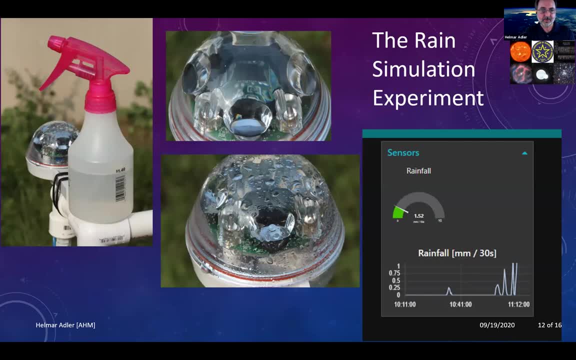 The rain sensor, The rain simulation experiment. So I borrowed a spritz bottle here from my wife And, because we don't get rain right now, for about two weeks spritzed some water onto the rain sensor And you can see on the right side, if you get the software correct, that I have certain rainfall simulated during the period of 30 seconds where I update now the values. 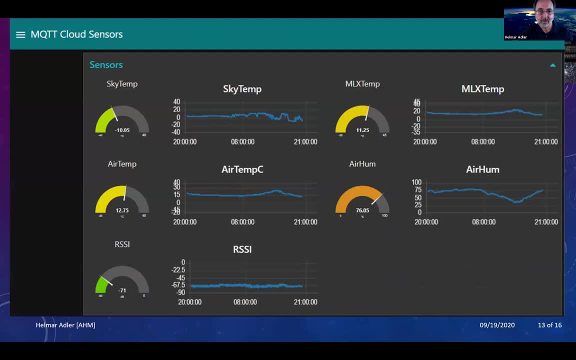 So this is very useful. So if you look for rain, Here is now the, So you might want to wrap it up pretty soon. Okay, I will. It's just last, almost the last slide. Here's the sky temperature displayed. Then I have the air temperature, the ambient temperature and the ambient humidity. 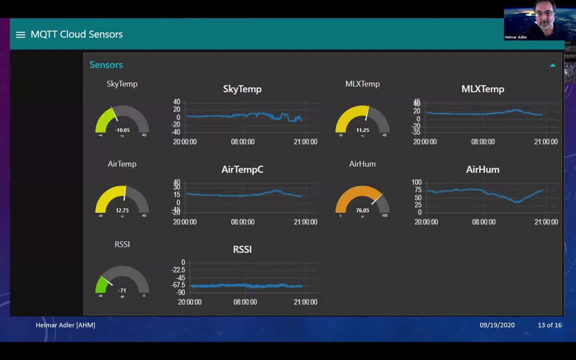 And then I call something here the MLX temperature, which is the temperature sensor which is built onto that infrared little sensor module, Since the module gives you the temperature of the PCB And for me it was interesting to see how close that temperature is to the air temperature which was measured independently. 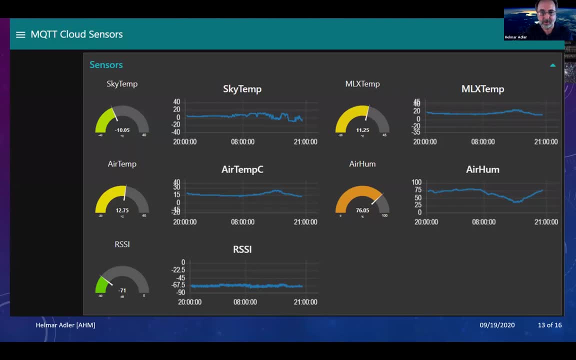 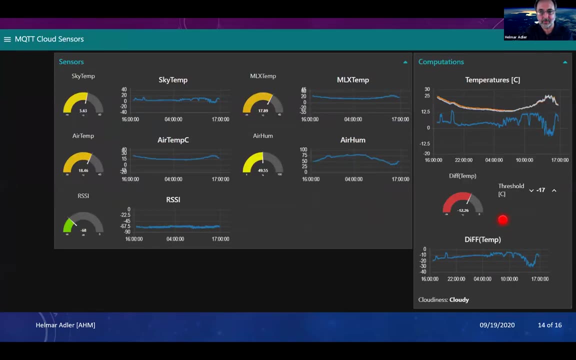 And I can just report they are very pretty close together. It's about a two degree difference, which doesn't make a lot of difference if you want to connect, to compare now the sky temperature to the ambient temperature, because that is what we are interested in. 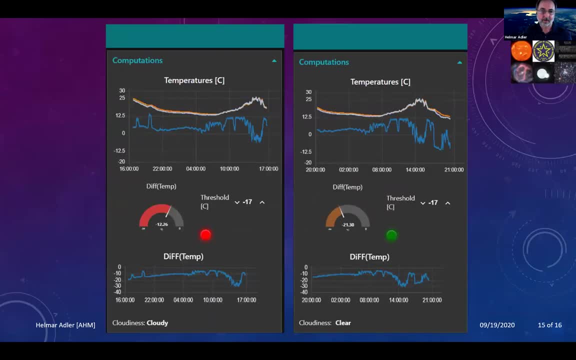 So this is what I do with what I call computations, And here's where it becomes interesting. On the top I have all the temperature, the three different temperatures which are measuring. displayed in blue On the top is the sky temperature. On the bottom area I have the difference temperature between the ambient temperatures and the sky. 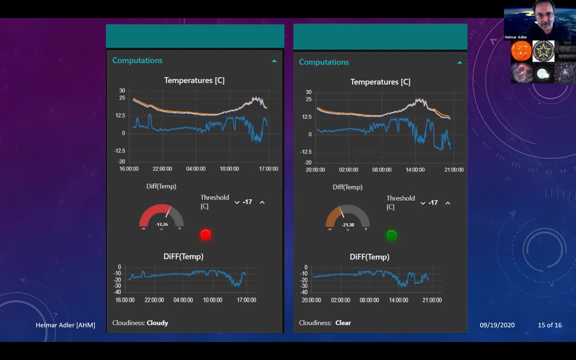 And that is where I can put thresholds on now to determine, Let's say, I have a temperature difference Of 17 degrees Celsius. This gives me an indication of if there are clouds or not. Now, if I put a little LED, everything in software in red and in green here, if the conditions are fine for clear sky, it's green. 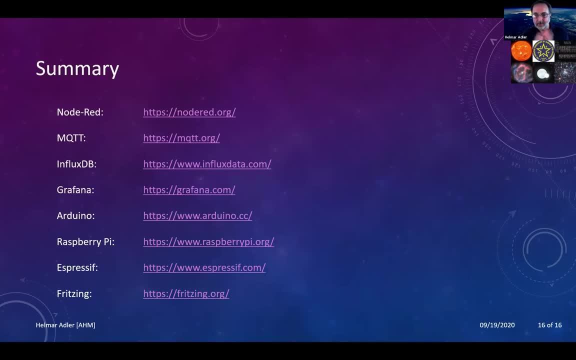 And if it's red, then it's cloudy. So this is what I wanted to show to you: There are lots of tools around which we can utilize for free, As amateurs, as more people who want to be a little more serious about automation. 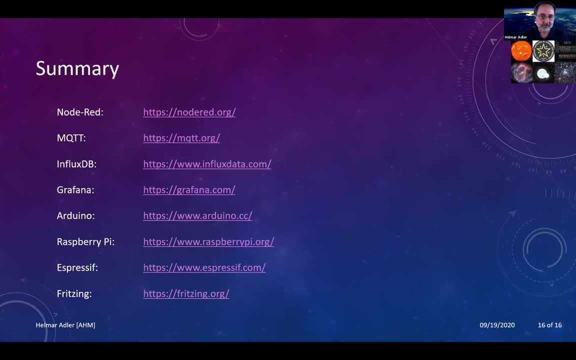 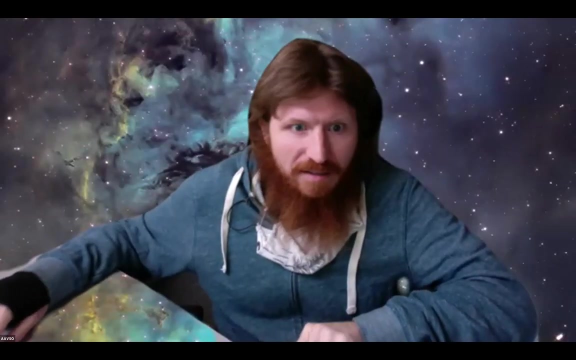 And I have a whole slew of lists, a list here of links which can be used, And I think we can make those available later on. Thank you very much. Thanks, Almar Tom. why don't we move on to you? and? 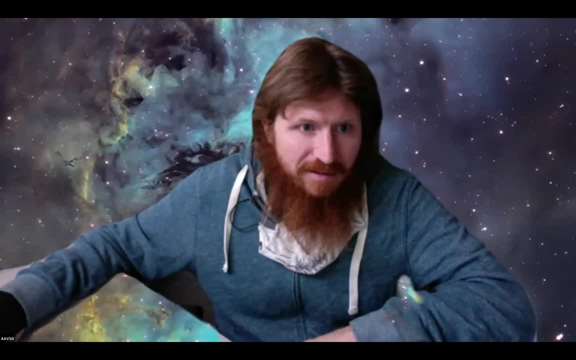 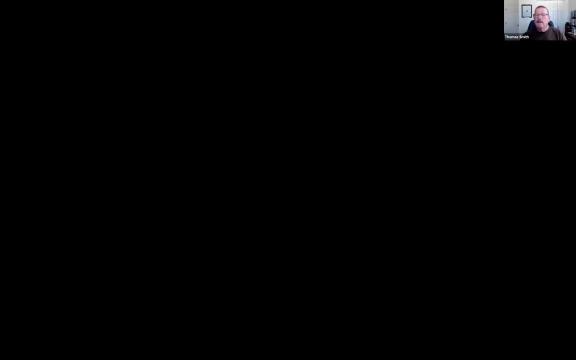 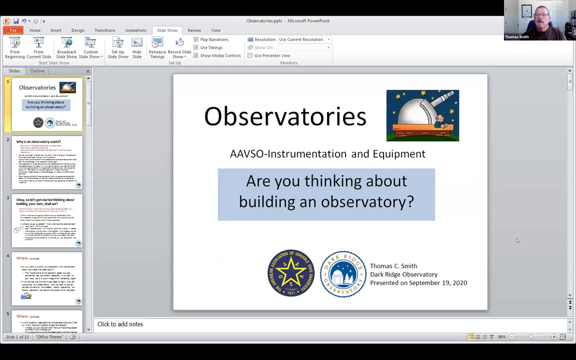 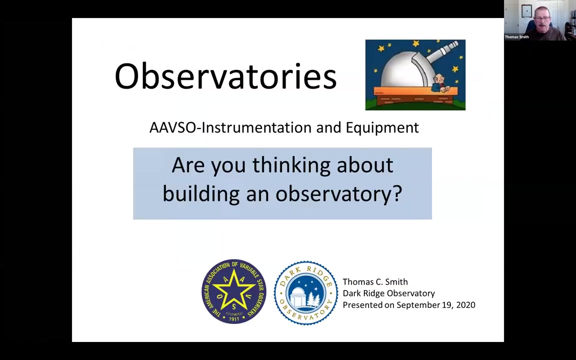 observatories. It sounds good. Let me go ahead and share my screen real quick so everybody can see it Looks like we have a little bit of latency here on the controls. Here we go. Everybody see that. okay, I mean hope you can. 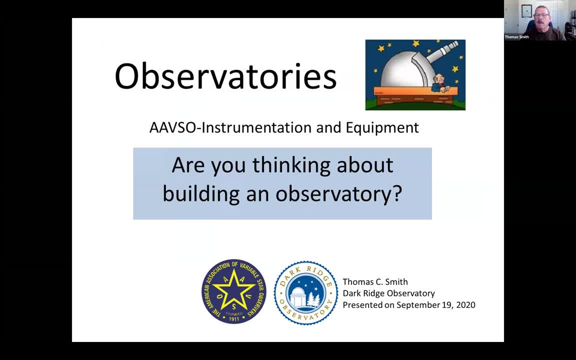 Hope you can hear me fine. My name is Tom Smith and I operate the Darkridge Observatory. Darkridge Observatory was one of the components that developed the APAS database. I put together all the hardware and ran the systems, But my observatory- 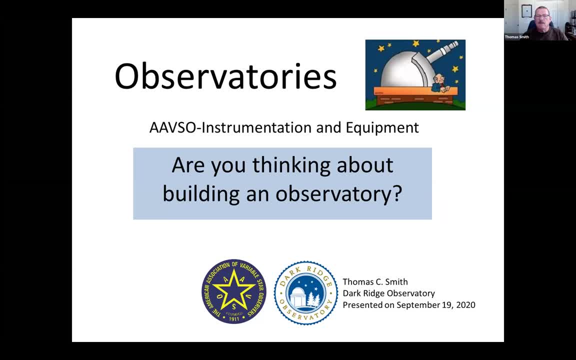 is in the Sacramento Mountains in the central south of New Mexico. I'm in an elevation of a little over 7,000 feet And that nice Princeton telescope you saw at the first screen that Alan showed that's about eight miles away from me. 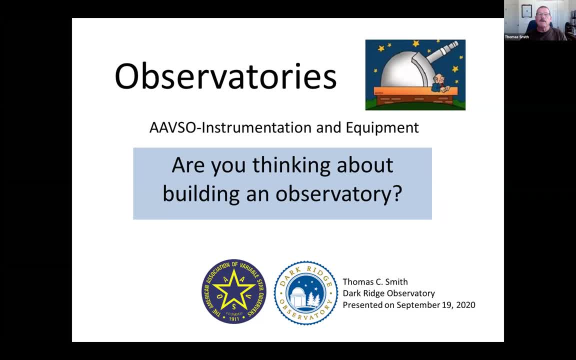 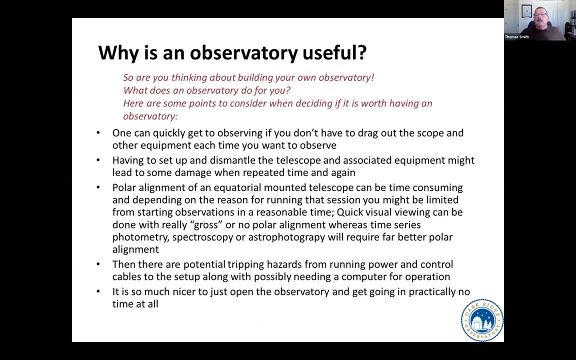 as a bird flies And it's a real nice area. Good seeing that type of stuff most of the time. We're in the middle of monsoons now, but it's going away. So observatories- Hmm, Why would you want to have an observatory? 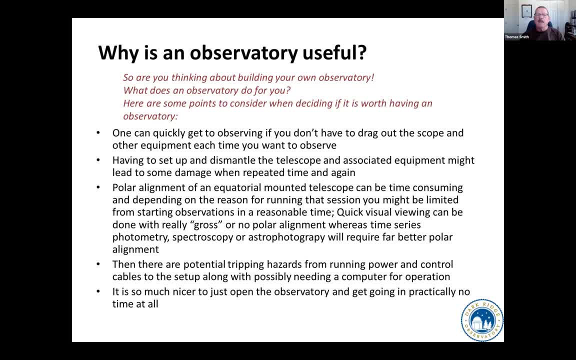 Well, observatories can do an awful lot for you, And I'm going to truncate a lot of this so that we can get through it quite quickly because we're running out of time. One of the things about observatories is you've got instant access. 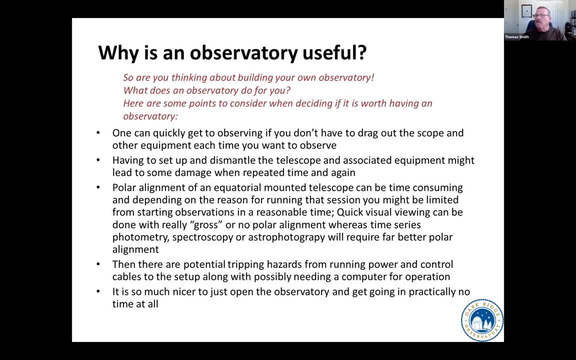 to a scope or equipment that you can put on the sky. Oftentimes, when you drag stuff out and put it back away, you can damage equipment, so you need to be concerned about that. And then there's always once you get the equipment out and set up. 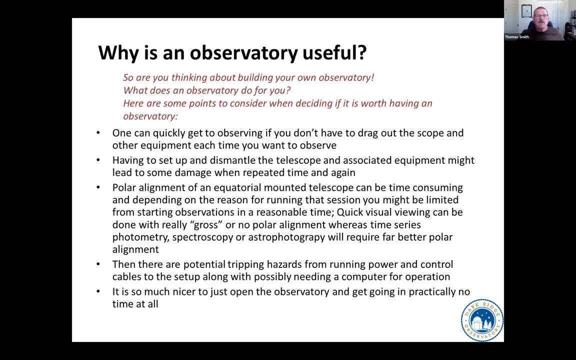 you have to do alignments, polar alignments, so that you can take either astrophotography or do science- photometry, spectroscopy- in a much better fashion. And then there's also polar alignment if you're just going to go out and do some visual looking. 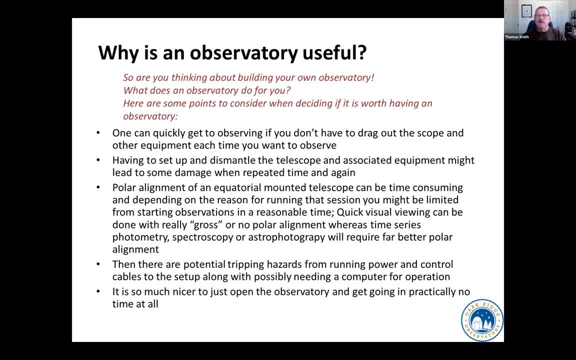 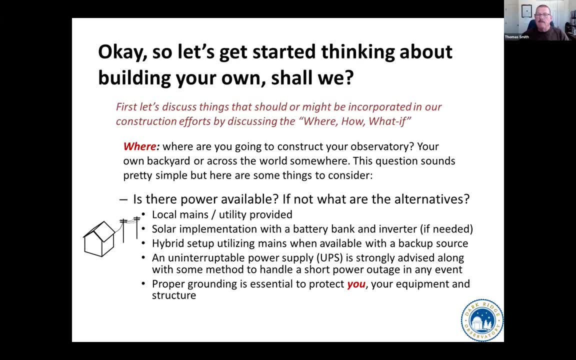 or that type of stuff. So having an observatory of a kind makes it much easier. You just jump out and you're on the sky. It's quite nice. So here's a couple of items here. Now I'm not going to go into great detail. 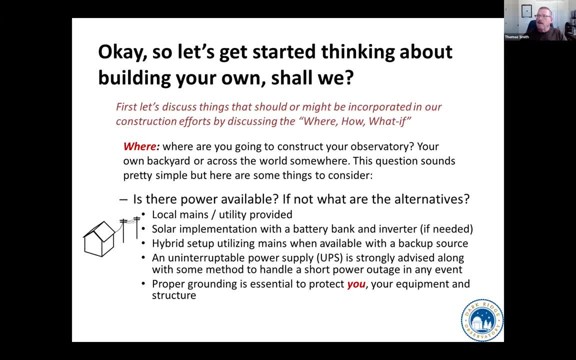 on a lot of these. I've got a full series of YouTube videos that I'm sharing with the AUVSO that go over soup to nuts, basically for building a remote and a robotic observatory system, And that will be shareable for you. 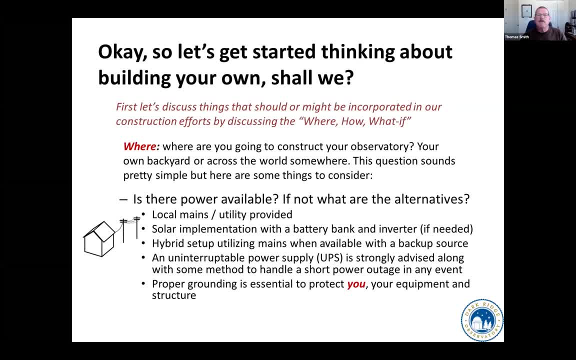 But basically, here's some of the things that you need to consider: The where, the how and the what ifs. The what ifs are really, really key here. If you're going to have an observatory, you've got to know where it's going to be located. 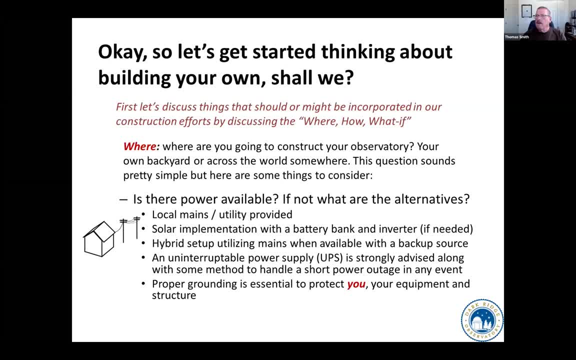 I mean you will. It's either going to be close to your home, in your backyard, or it's going to be located some remote distance, And each of those have both their strengths and also their issues to deal with Challenges. We won't call them issues. 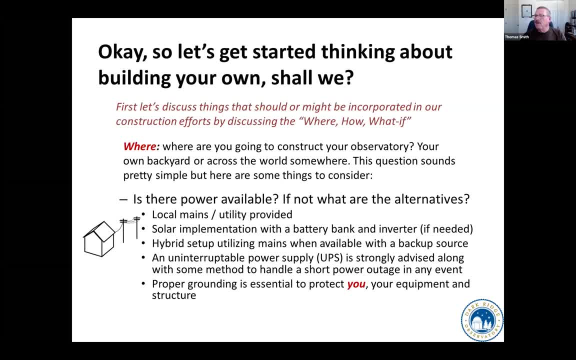 We'll call them challenges, Because you can have a lot of fun with a remote observatory too, And a remote observatory in your backyard isn't that far away from being a robotic observatory 10,000 miles away. So you know, it's just a matter of. 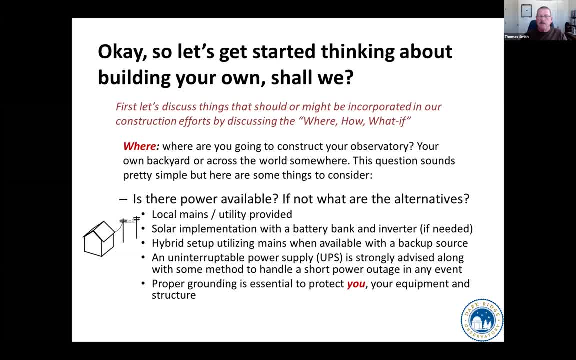 looking at a few things differently. One of the things you need to make sure you've got for our equipment anyway is you need to make sure there's power available. Many ways to do that. You can have the mains system or a backup system. 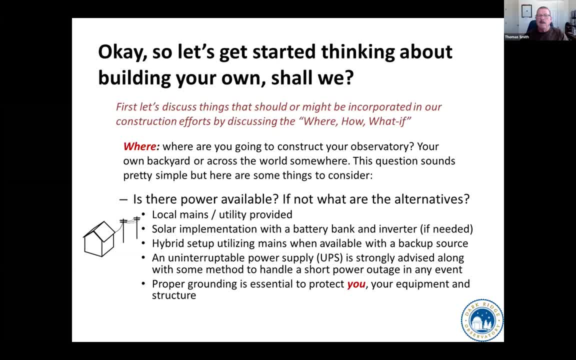 battery if you want a solar implementation, which is really nice to have, And also the hybrid model allows you to utilize both those. One thing that's very important, at least in my opinion, is an uninterruptible power supply- UPS. 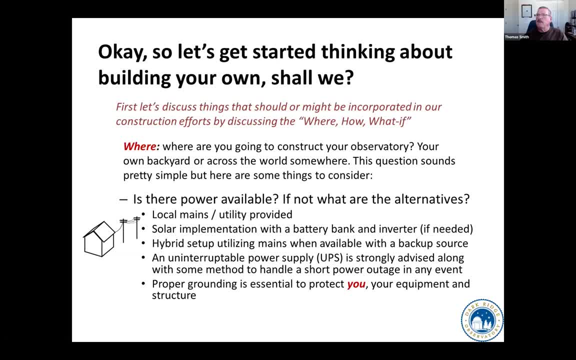 This will give you a little bit of chance to handle some of those short duration outages where you can take the actions you need to to put your observatory and equipment in a safe condition, assuming you can, Grounding obviously very important throughout. 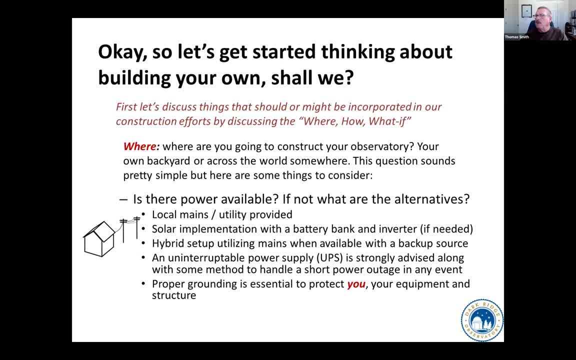 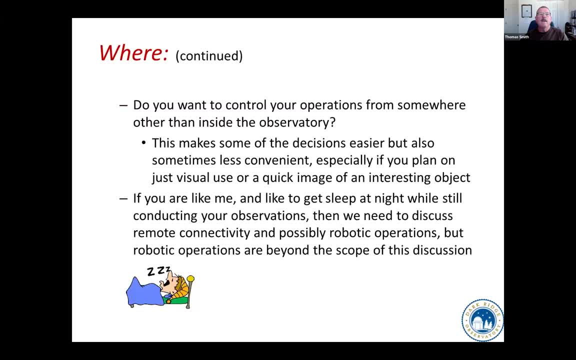 That's for your safety as well as the equipment's. I want to highlight your safety here. We're dealing with mains power in many cases, so it's important to realize what you can and can't do there. So control of the observatory, that's very, very important. 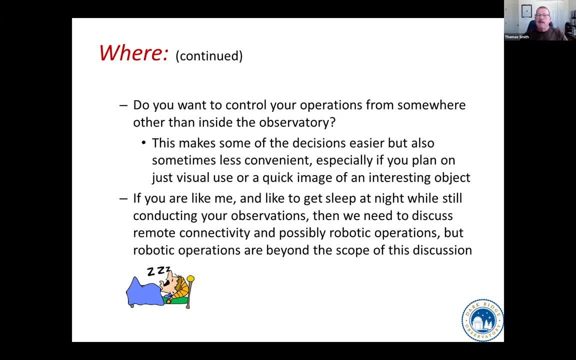 And the equipment in it. You've got to make a few decisions about how you're going to do this. If you're not going to have a remotely robotic observatory, or even a remotely operated observatory, it's great. You can just get your observatory opened up. 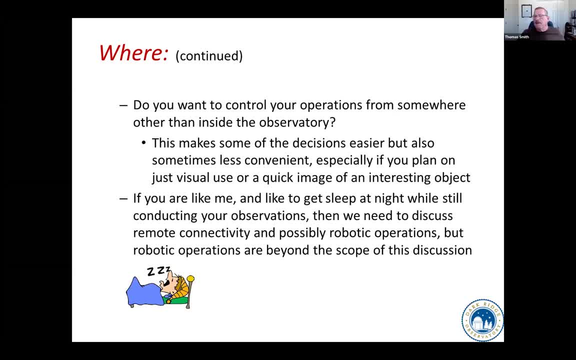 get out and start taking your pictures, do what you want to do there, take your science data, But I like to sleep. as it shows you in the bottom drawing, I do operate everything as much as possible in a robotic mode, And that's after you've shaken it out. 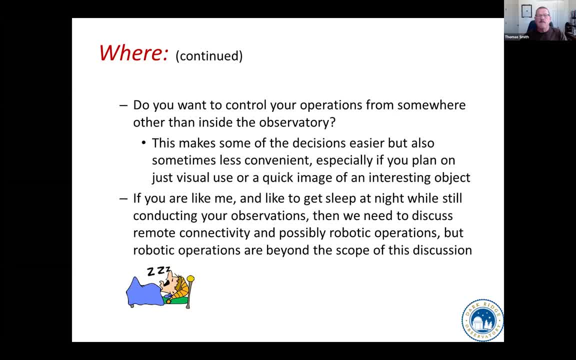 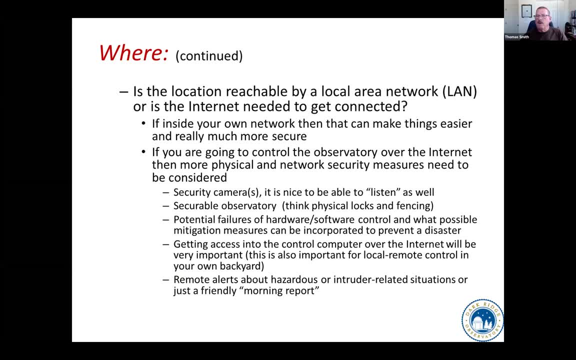 in a remote operation. So can you reach this telescope and equipment. That's important to be able to do that. If it's in your backyard, it's great. You've got probably your local aerial network, your LAN, that you can handle. 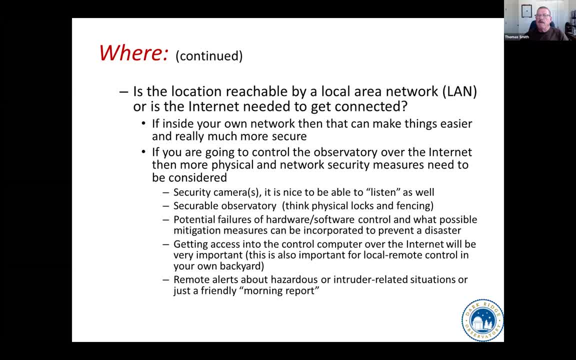 But if you're going to send it across the internet and deal with that type of stuff, you need to have a little bit more thought about security and your physical components, where they're going to be located, how they're going to operate. I've got a couple of items here listed. 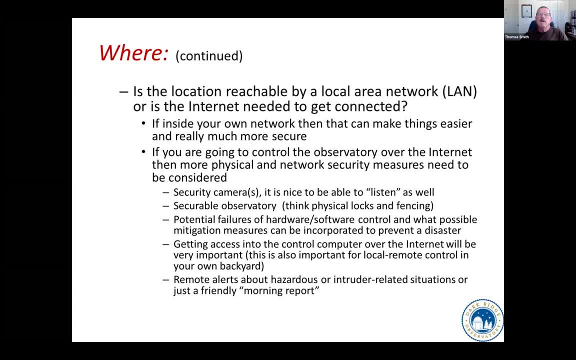 Security cameras are really, really important in my opinion. It's a two-way audio, So you can hear your equipment move. you can hear what it's doing, those bleeps and beeps As well. it makes it quite convenient. 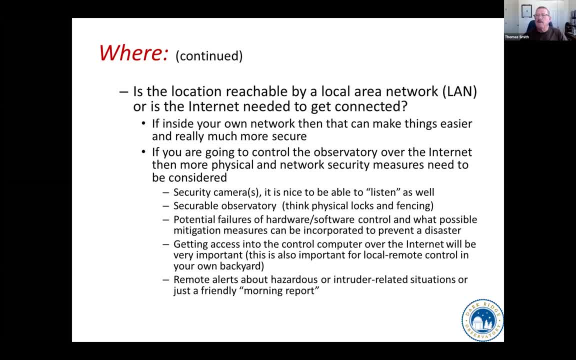 if you need to do some adjustments, You can have a second person out there working on your equipment and your audio can go back to them through a camera or another mechanism- another way to do that- But audio is very important too. Certainly not as big as 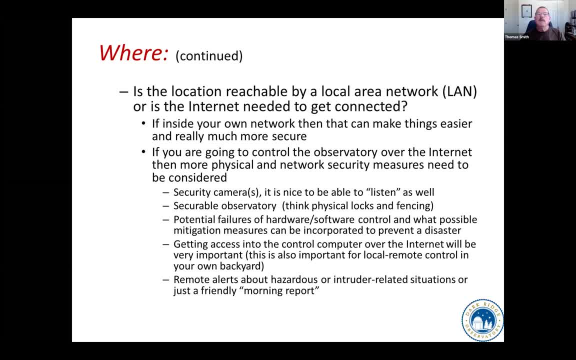 having visual indication of what's going on, but it can help a lot. You've got to think about locks and fencing if you're going to be remote. That's really important. Potential failures with hardware: We'll talk more about this when we talk about what-ifs. 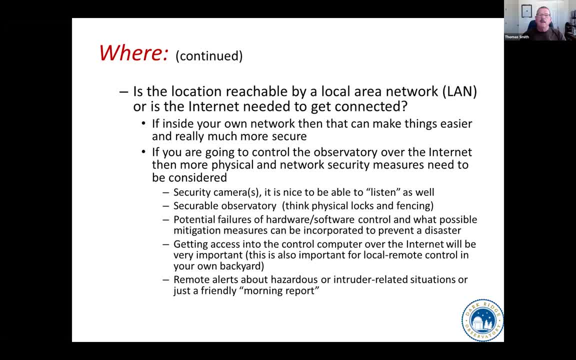 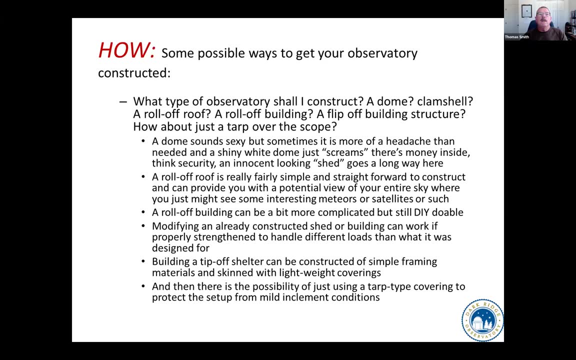 so let's just skip on a little bit here. Getting access to your computer over the internet is important, but you need to take some more of these controls, or think about what you would do in those instances where things go wrong. How are you going to do this? 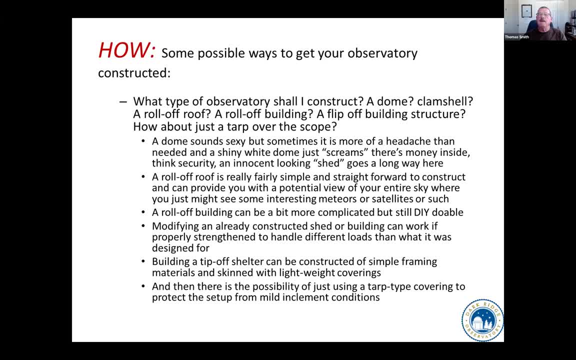 Don't get scared off. First off, an observatory can be anything you want it to be. It's just a real nice way to go out and get busy on the sky without having to waste additional time trying to set up. But here's the things you can think about. 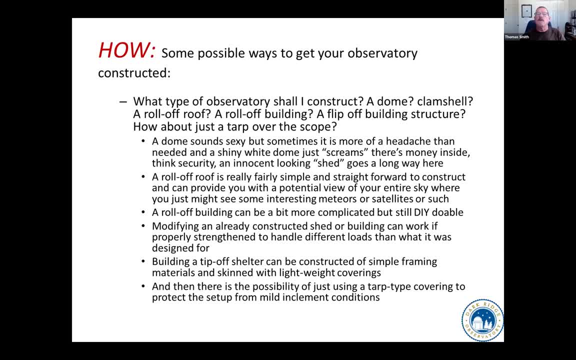 A dome, a clamshell, a roll-off roof- which is common- A roll-off building, which is common too, A flip-off structure? or how about, just as Richard Berry said at the beginning, a tarp over your scope? 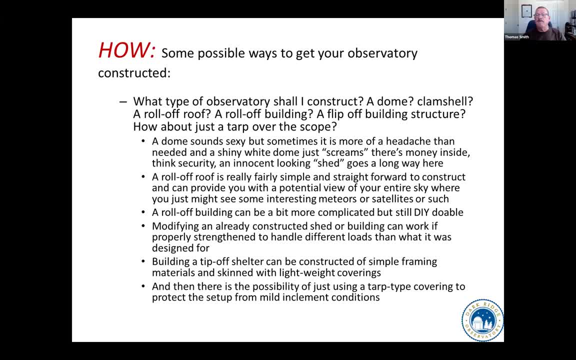 That is an observatory. It means you can get out there on it. provided you don't have extreme weather conditions, then that's totally acceptable. Of course, it's nice to be able to go out and either sit down in a place and enjoy it in an enclosed environment. 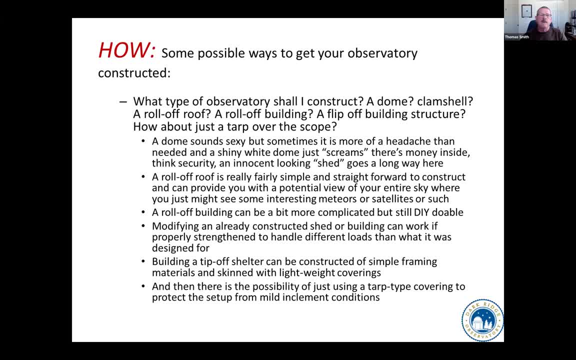 or remotely operate from the comfort of your own house. So here's some notes on those. One of the things that really is important is that very first top part where it says a dome sounds sexy, but sometimes it's more of a headache than needed. 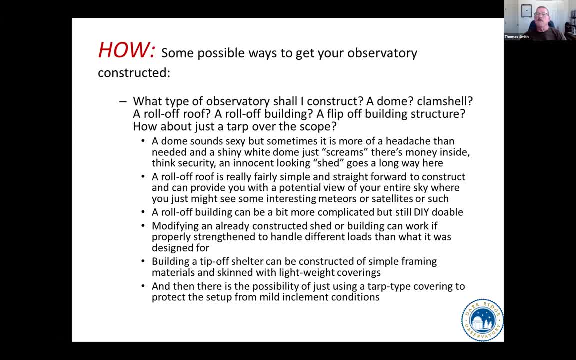 And it's very true. When you go up and down the road here where I live, you can see observatory domes all over the mountains, speckling the mountains And they're just a real security risk. I mean, you know, it just says to people. 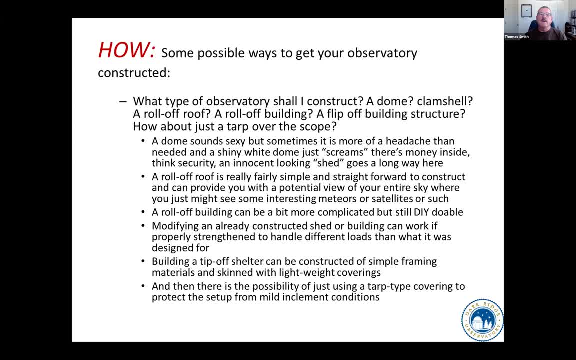 you've got a great amount of equipment and money tied up there, probably, But it doesn't have to be that way. In fact, my observatories are all roll-off looking sheds. You wouldn't even know that there was an observatory there when I was a kid. 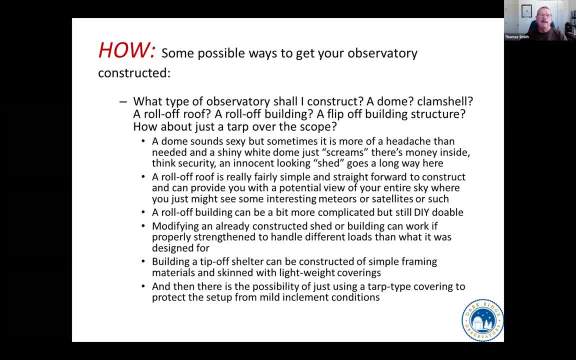 So, anyway, you can build an observatory out of about anything If you're going to modify some kind of a structure that is pre-built. I've seen quite a few people use, for example, those Rubbermaid storage sheds, and they'll modify them. 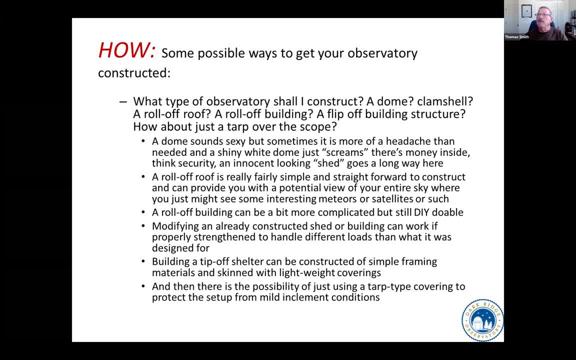 to be like a roll-off building, which is great. They work good- But you do have to take into account that they were designed for a particular structure and a structural load, So you need to beef that up a little bit when you do that. 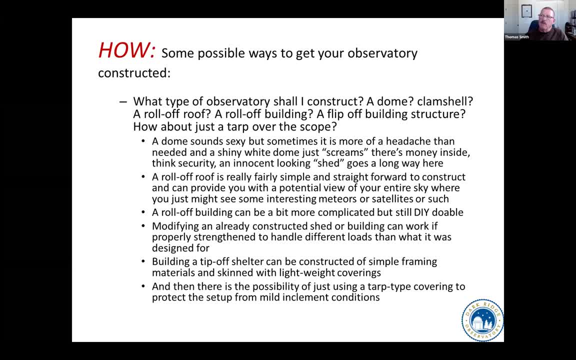 Builders are pretty easy. You can go out and just tip your observatory roof off yourself, if it's a small one, and get to observing. But you need to then be able to go out and close it, And unless it's motorized, 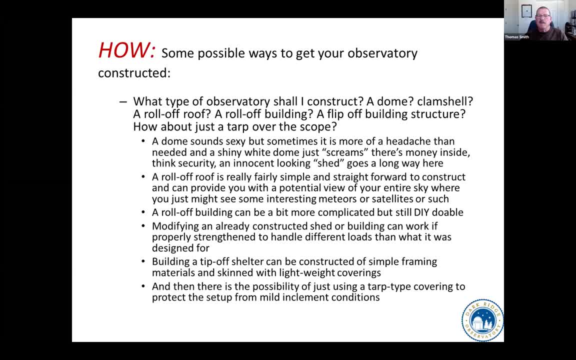 then you're going to have to go out and close it if you get inclement weather coming in. And these weather stations that are being developed, they're quite easy to build. There's really not a lot to them, but they're key. 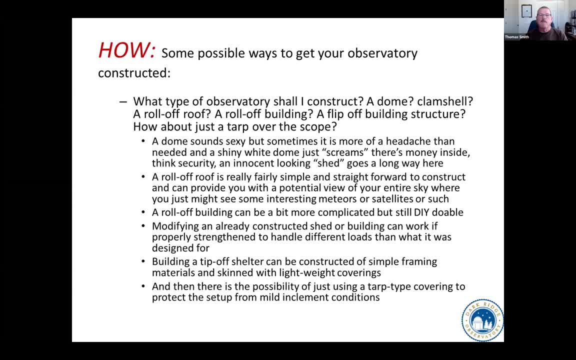 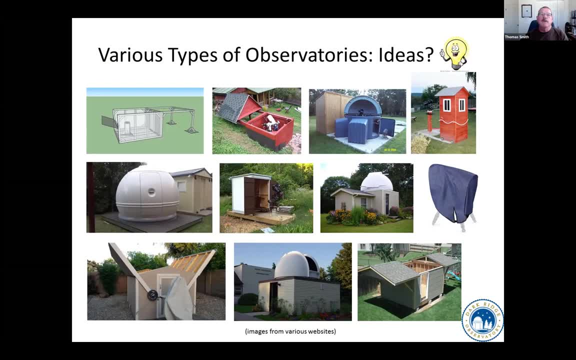 They're key to know that your equipment's going to be safe for it and for robotic operations. Here's a couple of different kinds of observatories. just some pictures that show you different things: The classic roll-off on the upper left and that one has a south dropping wall. 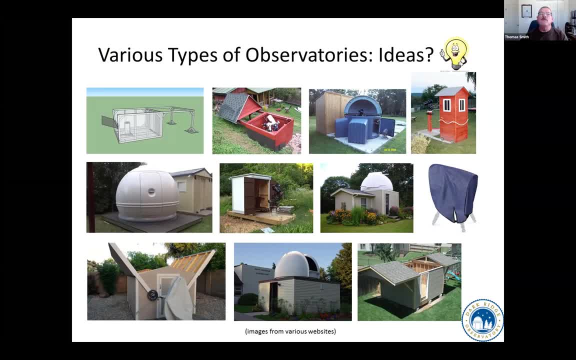 so you can go farther down to the south if you want to. You can see there's complex observatories, there's very simple observatories. You can do whatever you want, Make it as fun and interesting as you need to for your particular science projects. 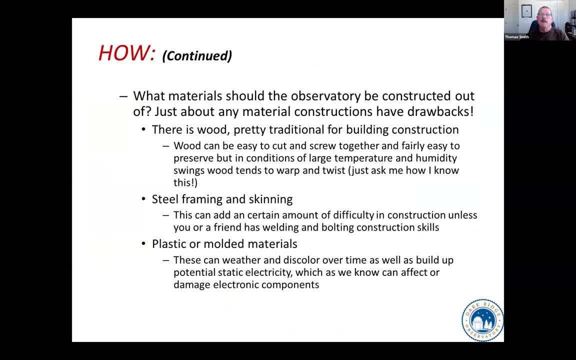 So how are you going to get it built? Who's going to do it? Are you going to do it? I mean, I love doing DIY stuff myself. I build everything out here myself: The hardware, the software, the building structures. 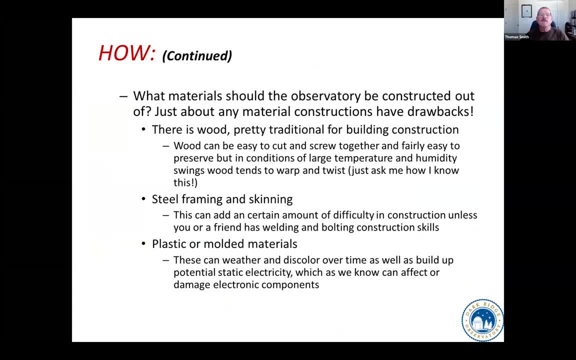 the infrastructure, all of that type of stuff. But there's a couple of things to think about. What are you going to make it out of? Well, wood is pretty classic. I mean, it's traditional. People build observatories out of wood. 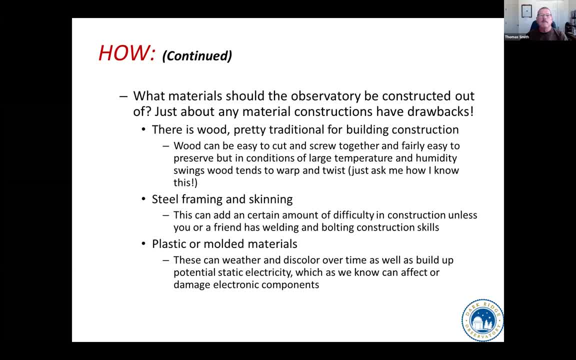 and you saw a real nice wooden structure in Dave Middlebent's location. You can see that construction is very common. However, in my location here I get a lot of high temperature changes and humidity swings and that wood tends to warp. 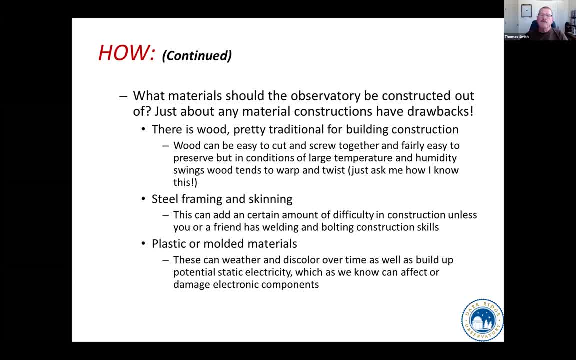 even if you've got it preserved pretty good. You can construct an observatory out of just a simple steel frame if you've got the capabilities to do welding or bolting if you need to. And then there's those plastic bolted structures that work really good. 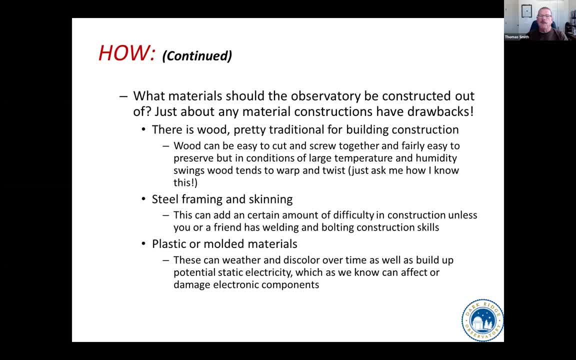 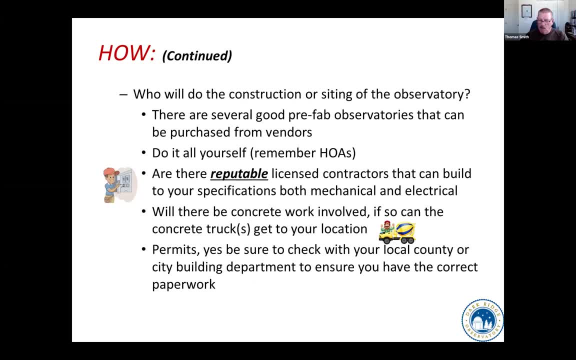 They sometimes discolor over a period of time, but with the UV, especially up here at 7,000 feet, some of that plastic component can be damaged quite a bit. One thing I want to back up and talk about real quick is that we said grounding earlier. 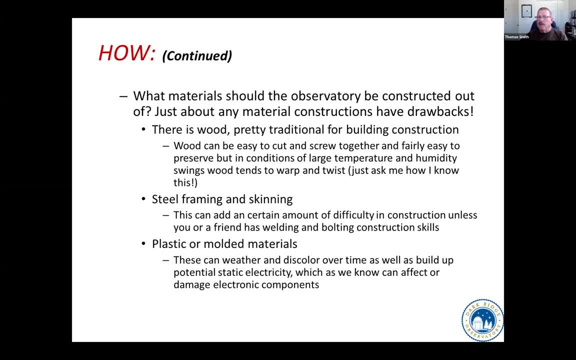 Down at the bottom of those plastic or molded type observatories. often they can build up a static charge. So if you modify one to use it, make sure you take into account your grounding. Your equipment will like you better. So here's what you've got to worry about. 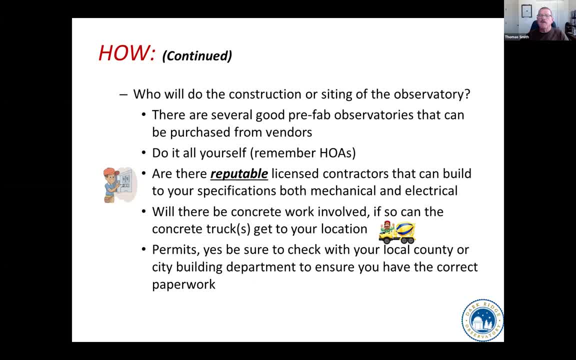 Who's going to do it? Remember, you've got oftentimes an HOA. I don't have them here- My nearest neighbor's over a mile away- But if you do have somebody do it for you, Are they reputable and licensed? 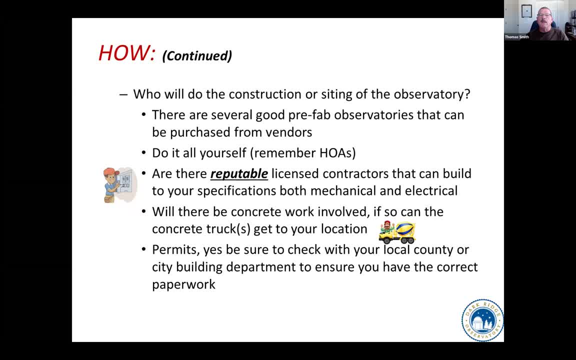 You need to make sure they are, to make sure you get the best quality and what you really want to have in your observatory. If you're going to build poor concrete, you need to make sure your trucks can get there. My driveway's a half mile long. 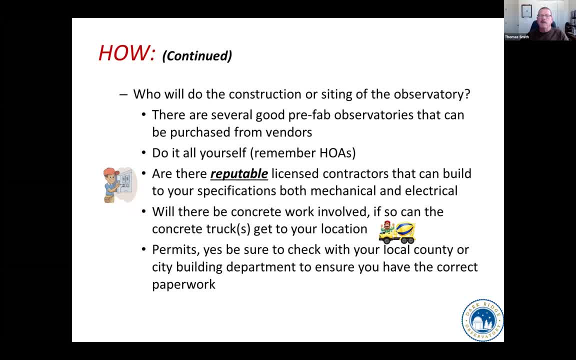 and it's got a hairpin switchback in it, yet I still am able to get concrete trucks up. But you need to think about that. And permits: yes, you need to check with your local building permitting department to make sure you're in compliance with that. 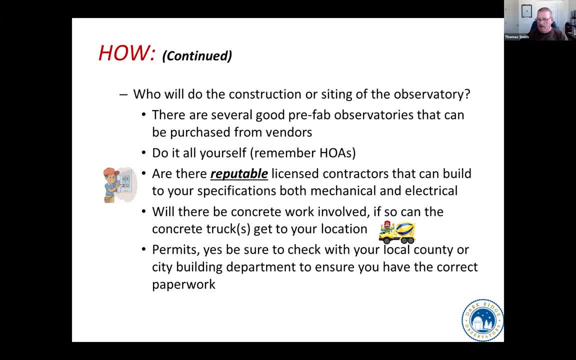 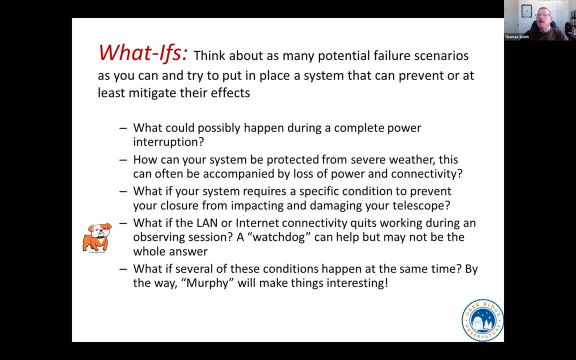 if you're going to build an observatory, especially if it has mains power to it and that type of stuff. Here's what's really kind of important, The what ifs. You've got to sit down and you've got to think about what possibly could go wrong. 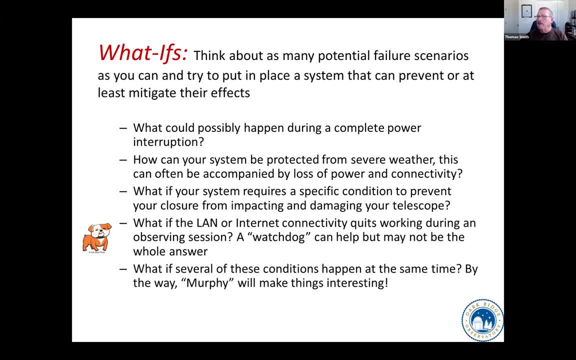 with your observatory, start thinking about stuff that could cause equipment damage or just plain loss of connectivity, for example. How are you going to protect your equipment in loss of power or connectivity? How are you going to take care of that? Oftentimes, 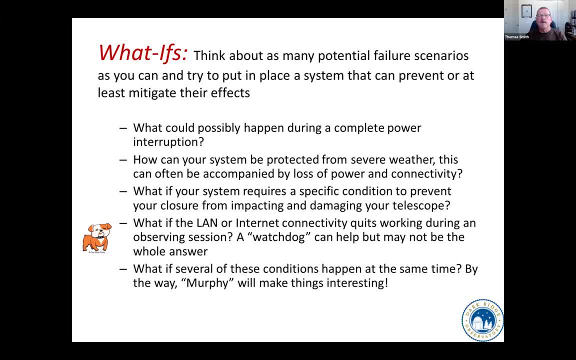 folks set up a watchdog type internet service or a local network service that sort of pings your main system to make sure that you have connectivity back and forth And if not over a period of time, it can oftentimes reboot your router or whatever your other issues are. 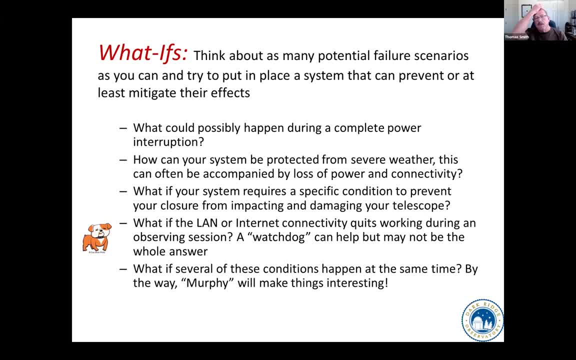 with your particular connectivity, And so yeah, Murphy's going to get in your way. That's a fact. You're going to have problems, Even if you sit down and take copious notes. you're going to miss some things, And that's all part of the fun too. 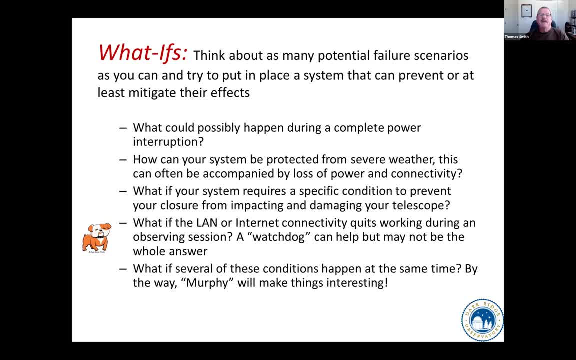 is learning what you didn't know, because you won't know what you don't know. Anyway, those are the kinds of things you need to take a look at: Loss of power and multiple things happening all at one time, If you know somebody in the area. 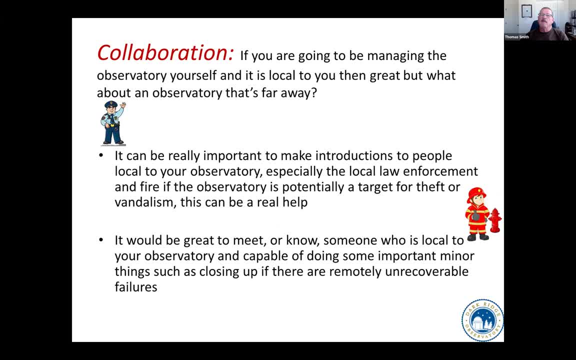 it's great. It helps a lot. You can collaborate with them in a lot of ways. If it's a remote observatory, especially if it's an area where it's susceptible to vandalism or theft or damage, it's a good idea to meet your local. 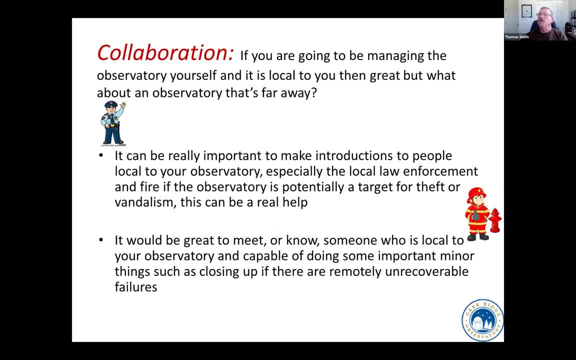 law enforcement and your fire folks. Take them up to your observatory, Show them what you got, Let them see how interesting astronomy can be, And just stay in touch with them And if you know somebody in the area that's got skills, that can help you out. 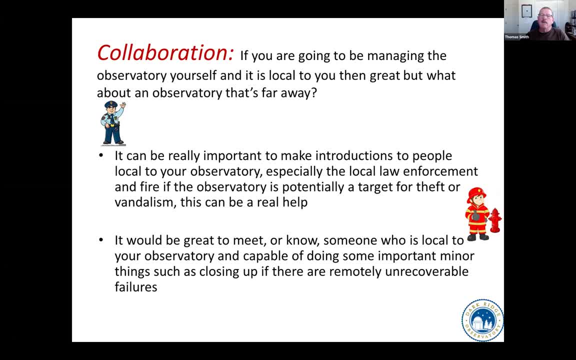 on a remote system. meet them, Talk to them, Get involved with them, Even if it's just they go out and just close your roofs or something if you need to In a big weather storm, when you've lost power and your internet connectivity. 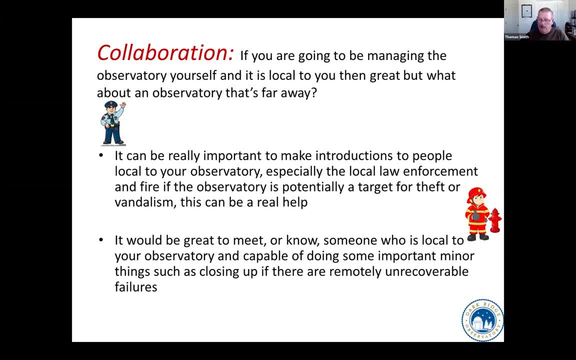 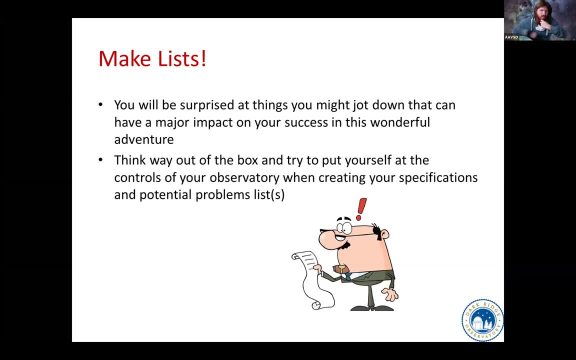 oftentimes someone can get out there and just close it up and make it safe enough until you can repair it. So that's a good idea. Two minutes, Tim, Go ahead. Two minutes, Okay. so here's that list thing. Make a detailed list. 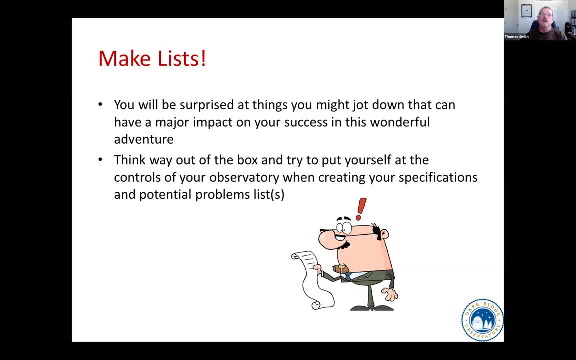 Sit down and think about things that can go wrong and then write down what you think you might be able to do to mitigate those things. And definitely think way out of the box, because you never know what's going to happen Again. there's a lot more, much more details. 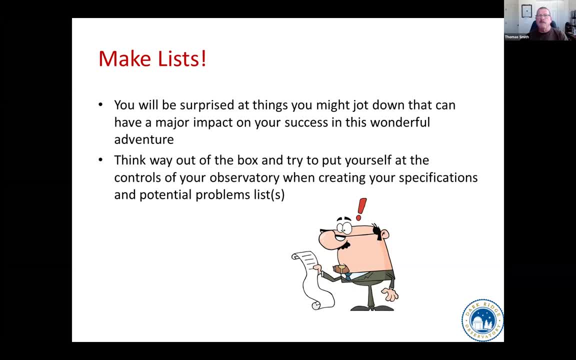 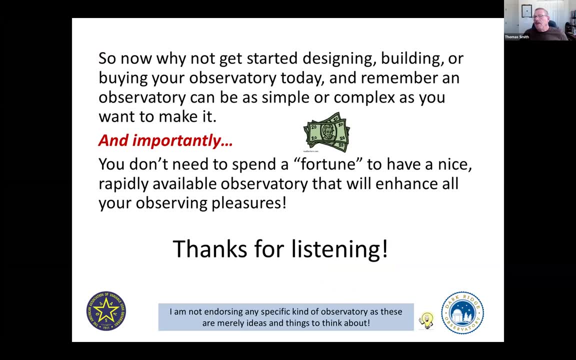 I've got about a 10 or 12 series of videos set up on YouTube. Those will be available through the AVSO also. But with that I want to say so now get out there and start building it And remember you don't have to spend a ton of money. 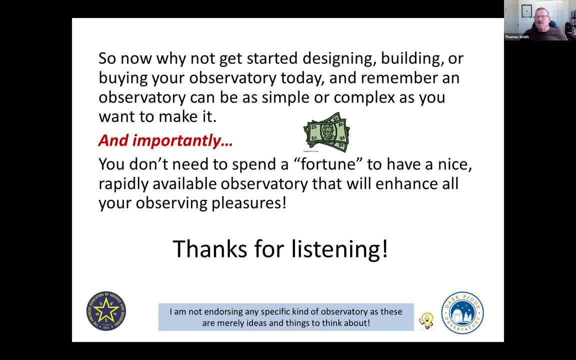 It doesn't have to be anything really fancy. It can be as simple or as complex as you wish to make it, And remember things always grow, So get out there and enjoy it. Have a good time. Pleasurable observation settings. Thanks you guys for listening. I appreciate it. 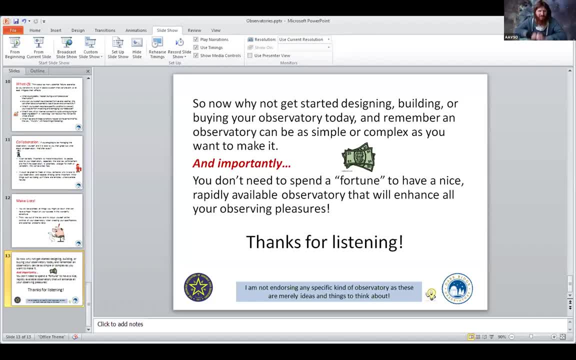 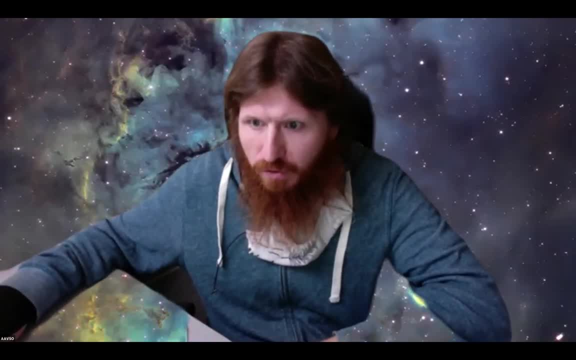 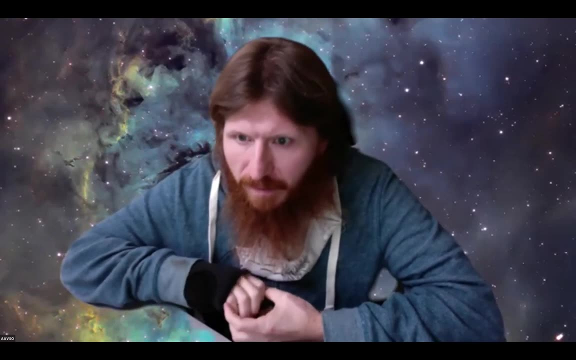 That's it. Thanks very much, Tom, And thanks again to all of our speakers this session. We have a few minutes, so why don't we just jump straight into Q&A? So the first question that we have is Molly and, I guess, Phil. 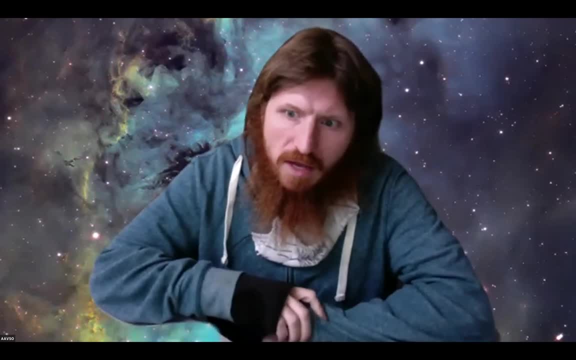 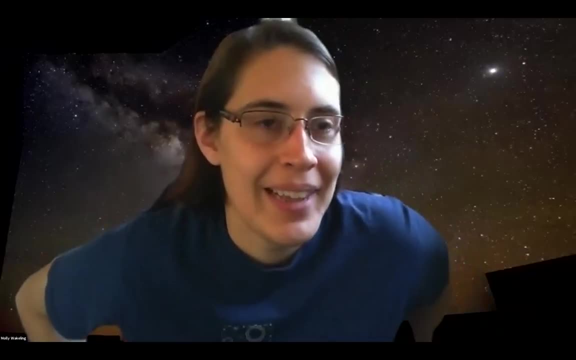 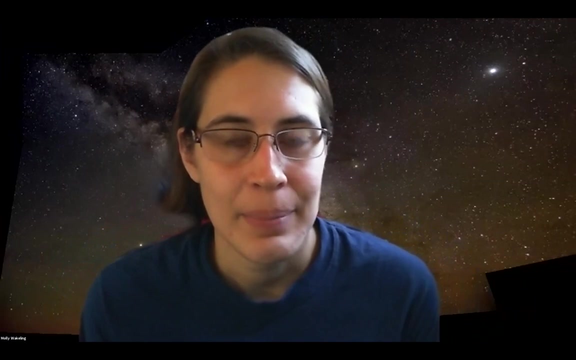 wants to weigh in on it as well. When do you use check stars and when do you only use comp stars? So not going to lie, I've not figured out how to use check stars in VFOTE. I couldn't really find much on them in the manual. So I just use comp stars and I delete ones where the magnitude that was measured is too far from the actual known magnitude of that star. I just take those out so that it doesn't make an anomalous measurement. So yeah, I'm still kind of new at this. 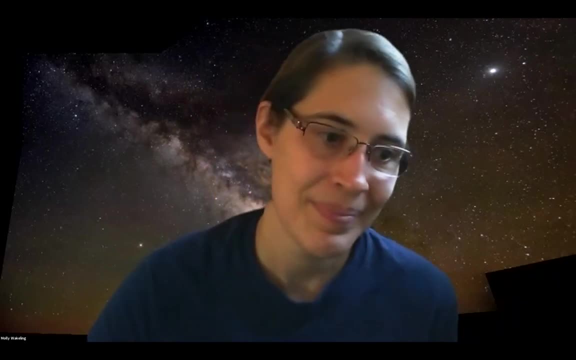 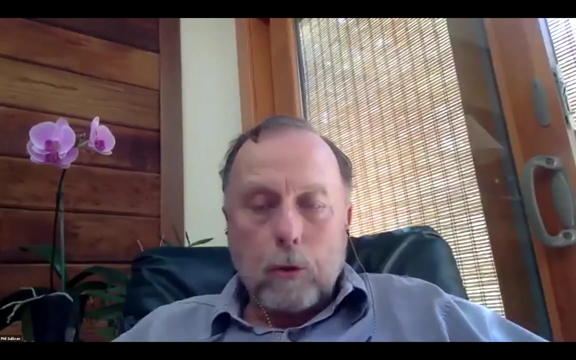 So yeah, I don't know, I've not used check stars. Well, I take that If you're using only a single comp star, you should always use a check star. The check chart allows you to make sure that the comp star isn't. 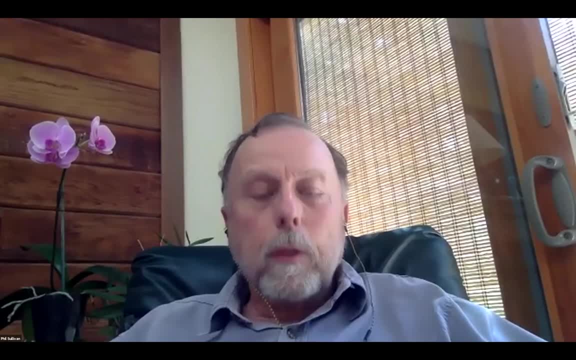 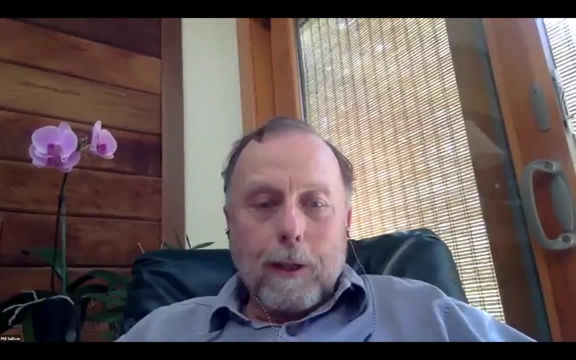 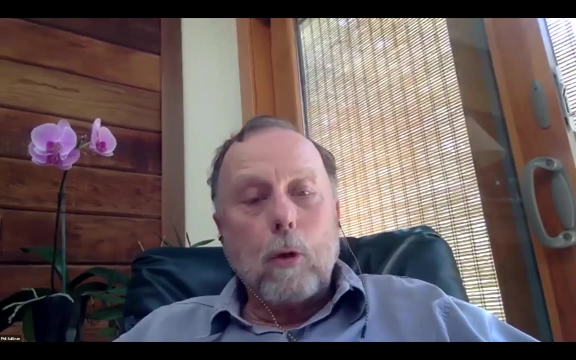 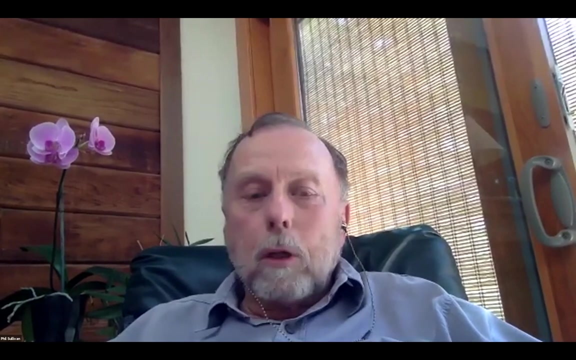 varying or that the atmosphere isn't varying. So a single comp star is. you just have to use a check star. It also allows you to give a measure of uncertainty if you're doing a series. But yes, you've got to use a check star if you're. 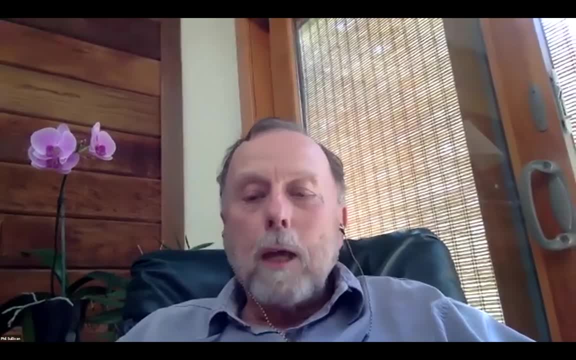 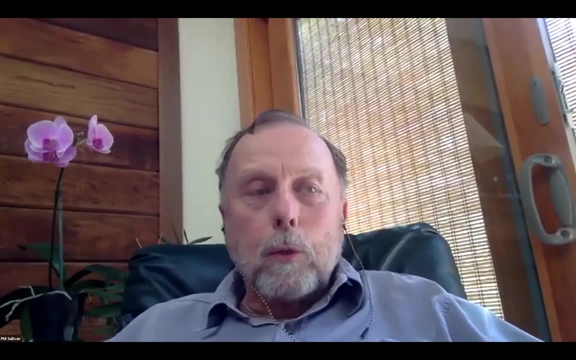 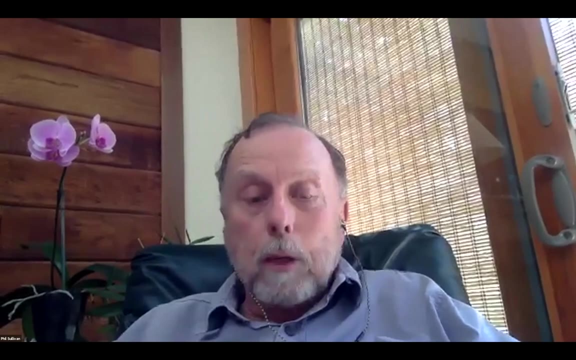 using only a single comp. You can do that in VFOTE. You can specify any of the stars in the AAVSO comp series by just clicking on it. It brings up a box in VFOTE and you can change that star to a check star. 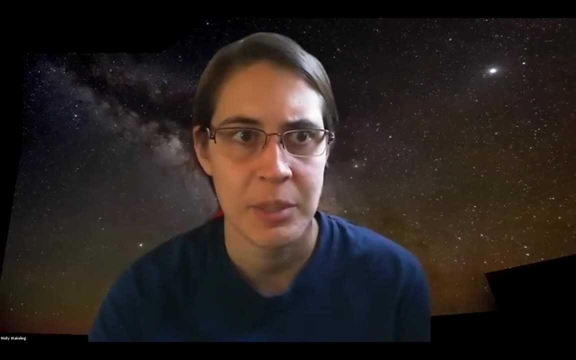 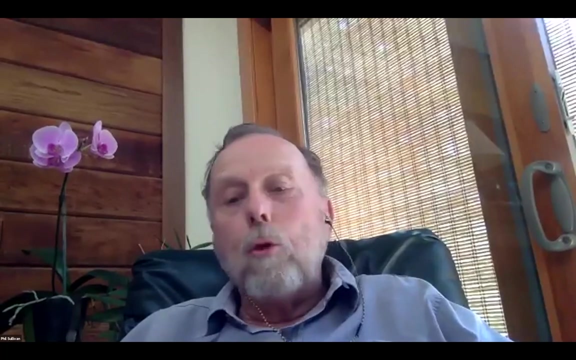 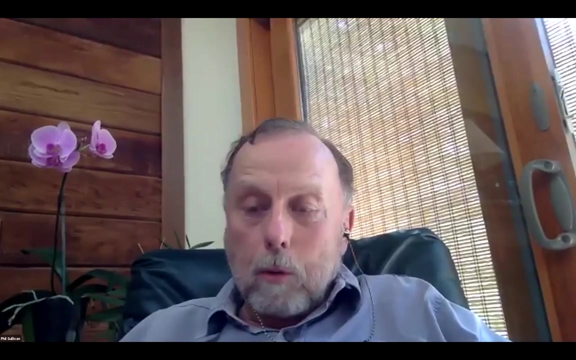 Try it. What's the difference between a check star and a comp star? A comp star, well you know, is a star up against which you are measuring the variable. A check star is not used in the analysis of the variables magnitude. 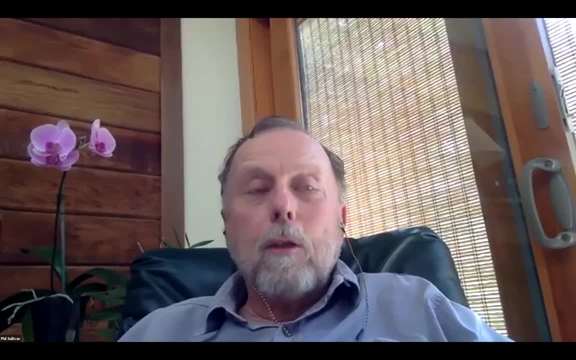 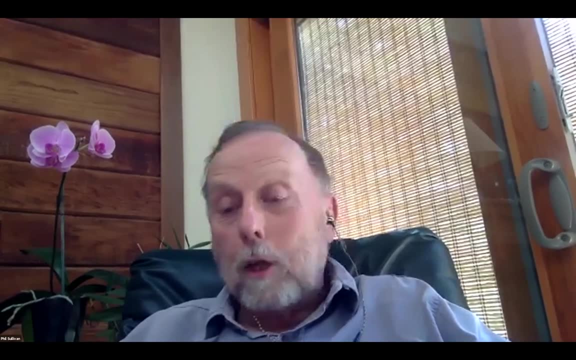 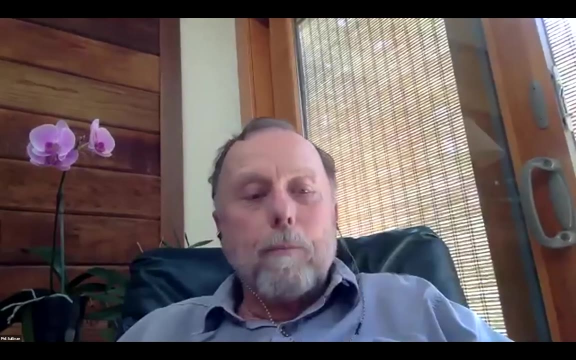 It's used as a way of making sure that nothing else is varying in the sequence If you're using an ensemble. So it's like a comp star for the comp star, Sort of. yeah, You can use the measurement of the comp star versus the check. 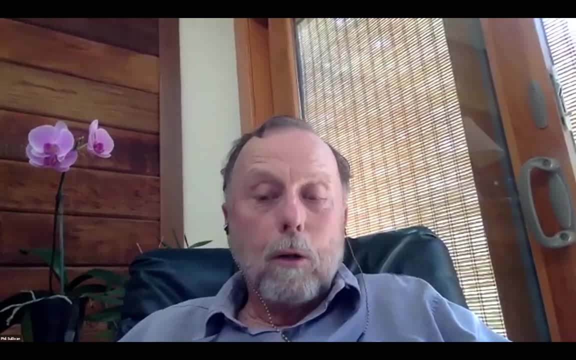 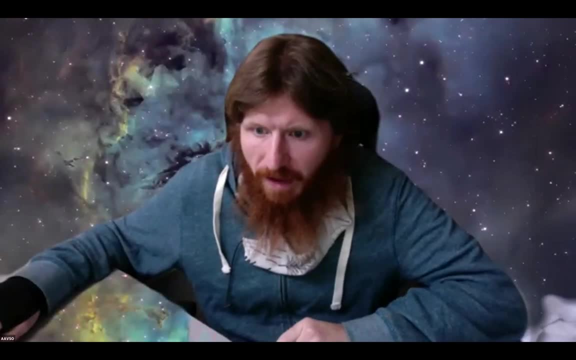 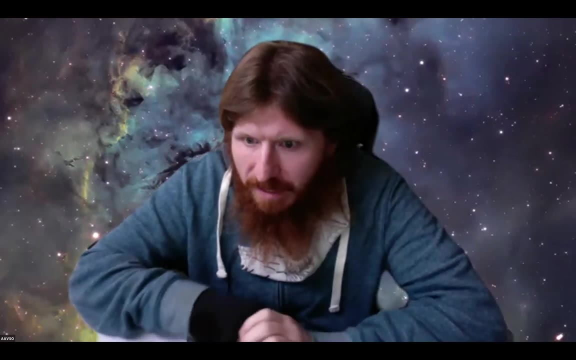 star, just to make sure that all your comp stars are behaving. I'll try that out on my next submission. We have a DSR DSLR related question. This one says: if you're using a DSLR camera and you don't have any photometric 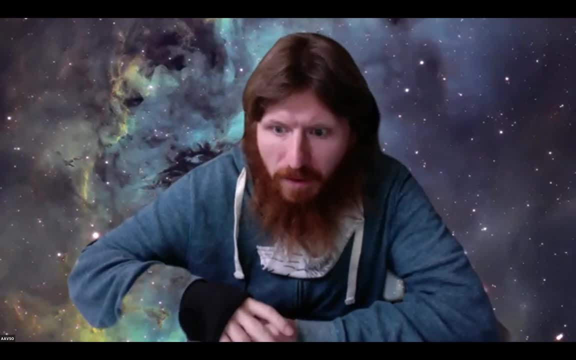 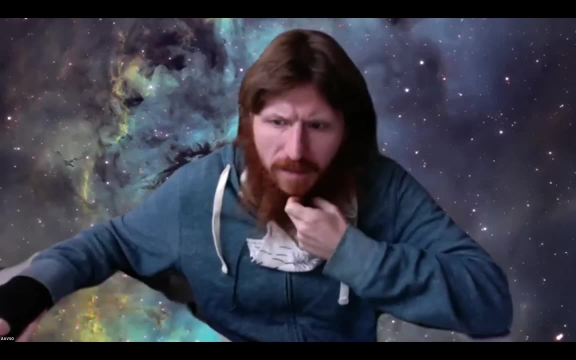 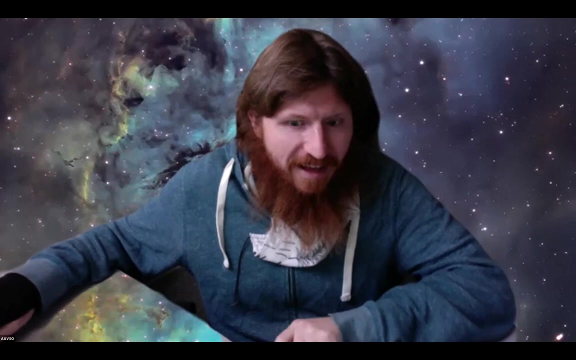 filters. what channel is the best for variable star slash exoplanet photometry? They actually suggest is R the best channel, And I'm pretty sure the answer to that is no, But I believe the best channel is G. George, I think you. 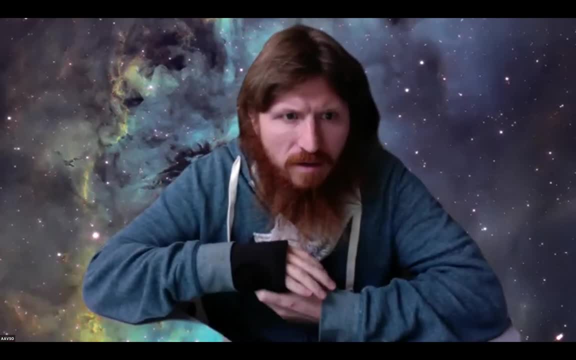 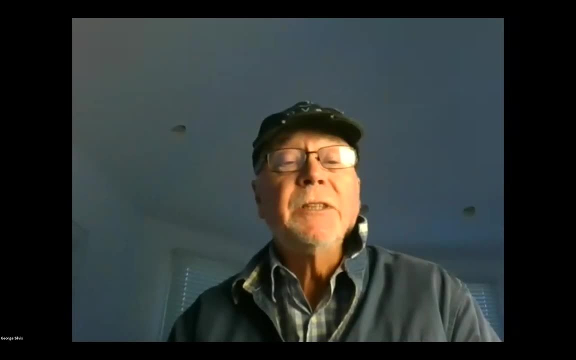 would be good to answer this or, Richard, I could step in. You definitely want to use the TG channel from a DSLR. It has the closest match to the Johnson's V. Red is way too wide. It's very problematic to use that. 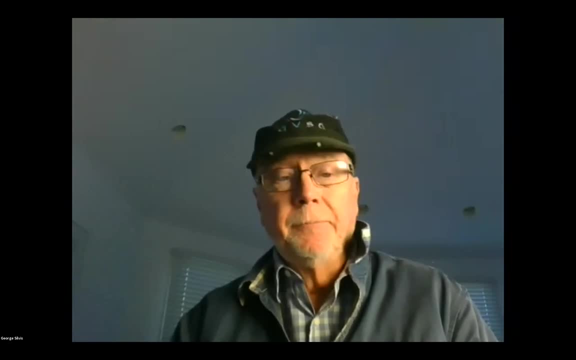 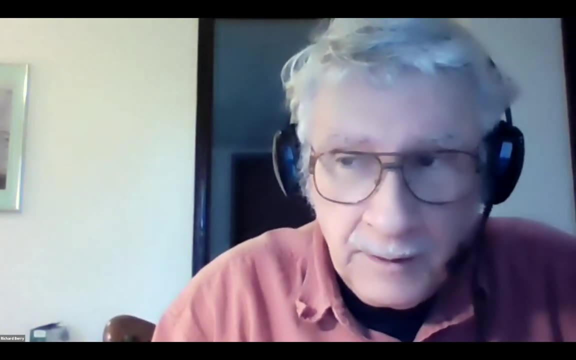 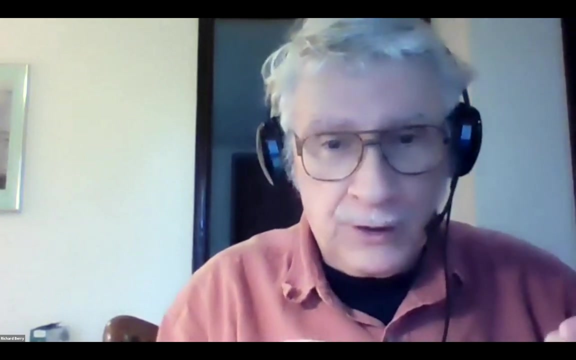 So G is the best. Yeah, and I've been doing some experimentation using Bayer filters and some standard cameras binned 2x2, which basically puts together the R, G, G and B filters, And I'll be reporting on that. 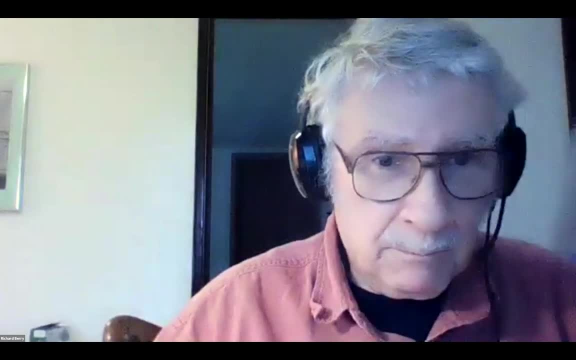 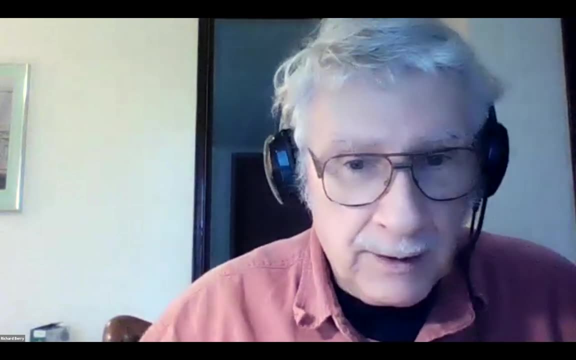 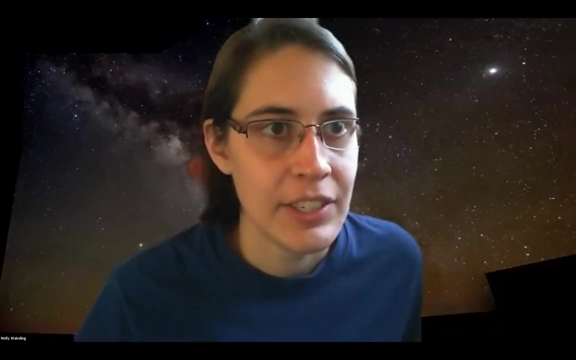 briefly next week at the CMOS, But basically, if you bin Bayer material, you get something that's quite close to TG. I want to add real quick that Barbara Harris, who's a prolific AAVSO observer, she uses a DSLR and she's going to be giving a presentation. 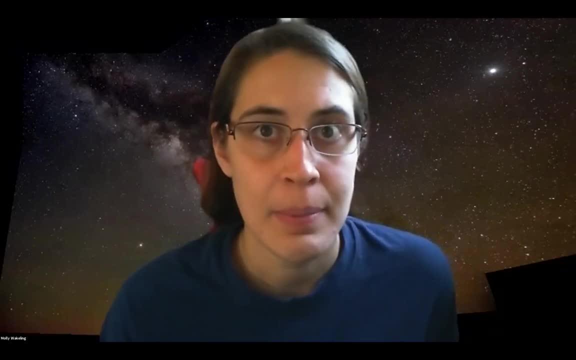 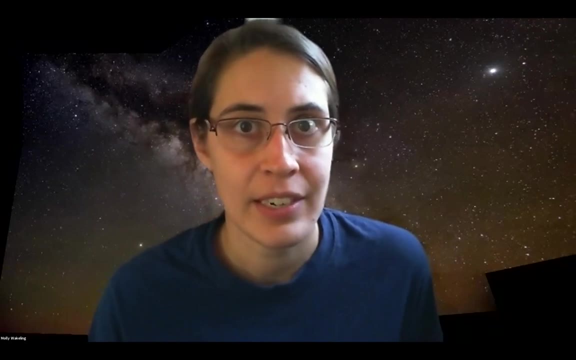 on the Astra Imaging Channel on October 18th about how to do photometry and how to do variable star observing with a DSLR. So for folks who have DSLRs, tune into the Astra Imaging Channel at 9.30pm Eastern. 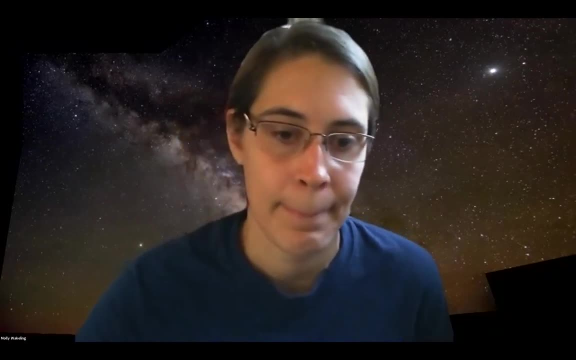 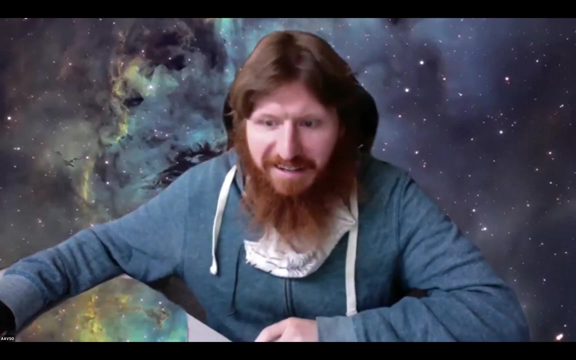 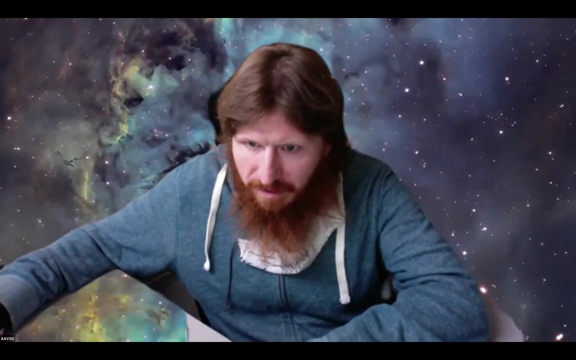 time on October 18th to see Barbara's talk about how to do it. Our next question is for Tom. Actually, let's that one seems a little bit more tongue in cheek, so maybe we should go to that one. that's a little bit more serious for now. 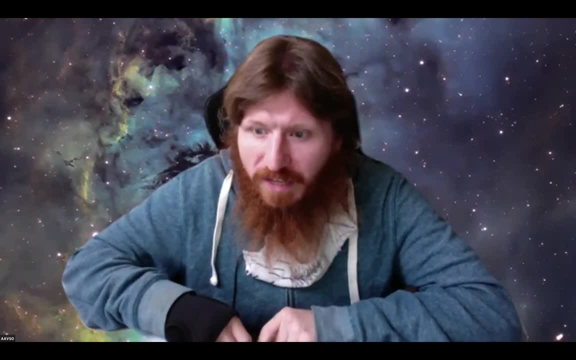 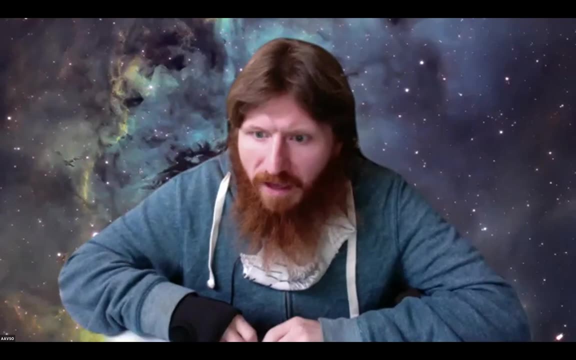 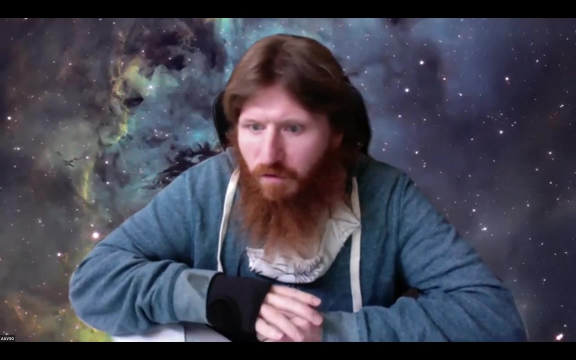 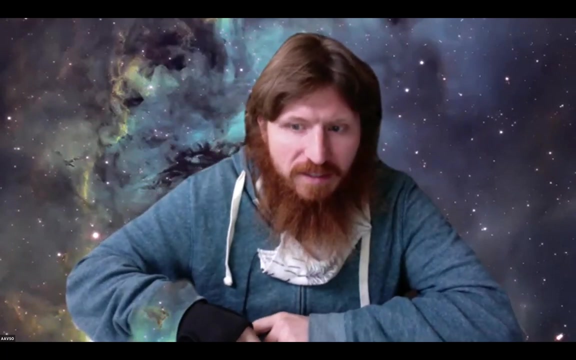 What is the? so someone has a question about flat field illumination. They say that they have not an electroluminescent panel for flat field imaging, but that their uniform illumination is still bigger than 1%. Is it possible to use it even if it's above 1%? 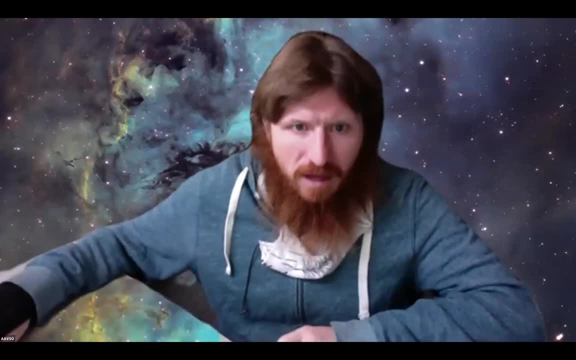 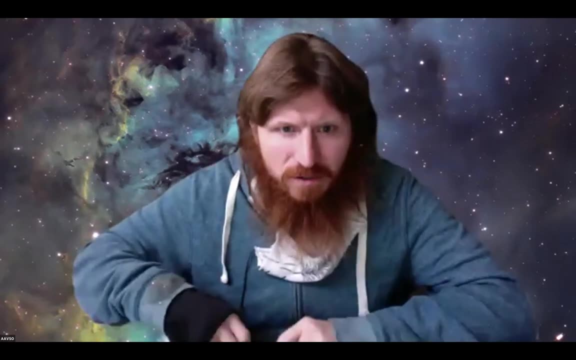 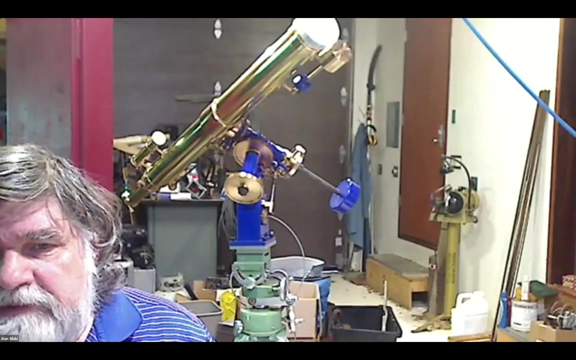 or do they need to find something else? And this is probably a question for one of the makers, Alan, I think you're muted, Alan. Yeah, so you're going to all flat panels. have some limitation on the uniformity, and I think 1% is actually. 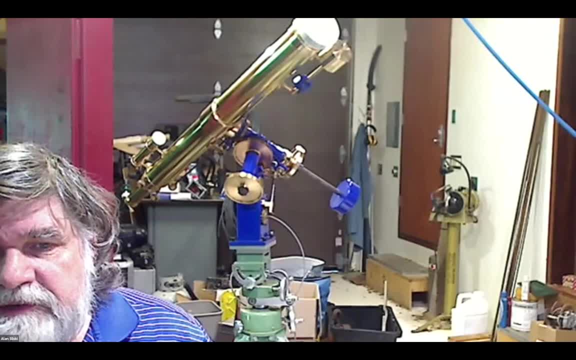 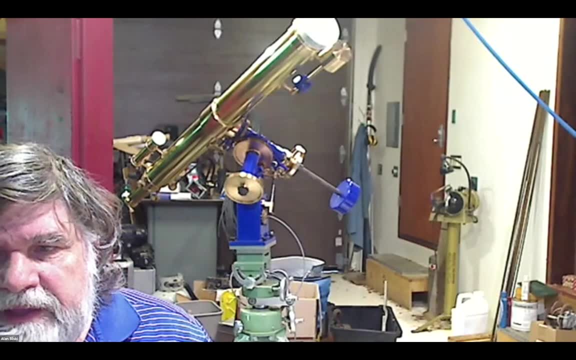 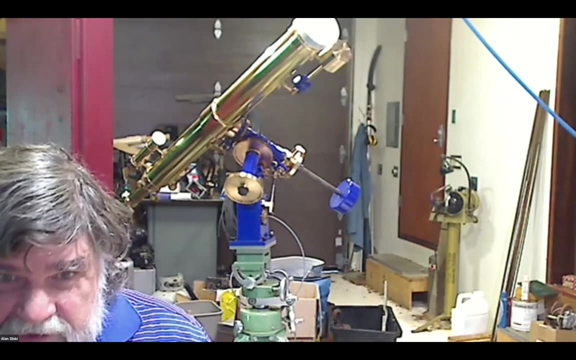 pretty reasonable. Some of the photometrists may have some there are. there may be techniques for you know, improving upon that, but I think 1% is pretty good and if it's 10% it's much more difficult. but Gary Walker, who's somewhere online. 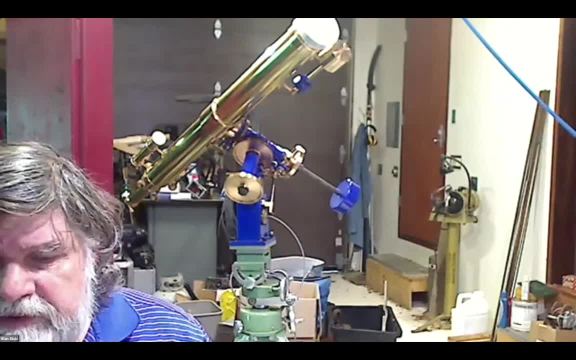 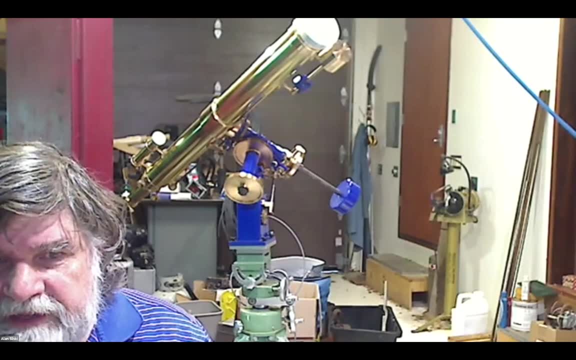 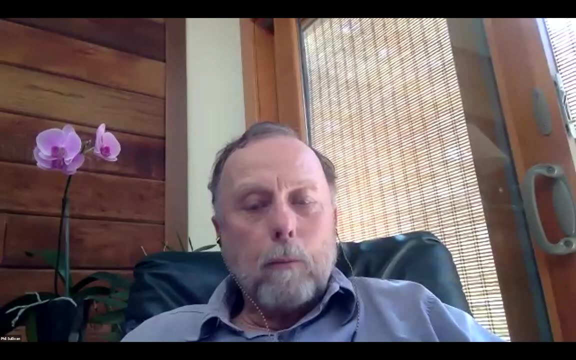 or some of the other more experienced photometrists that do flat fields, either with panels or twilight flats, might be able to add more detail. I agree, Alan. I think 1% is pretty good. I don't know if you're going to find a flat. 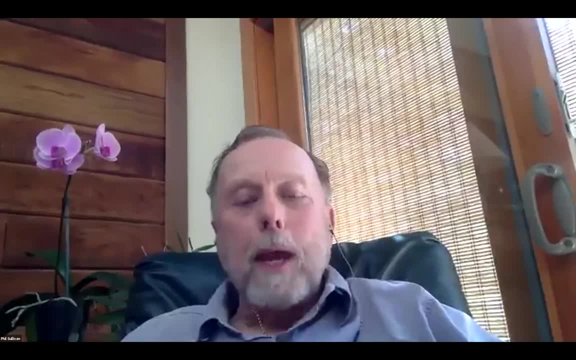 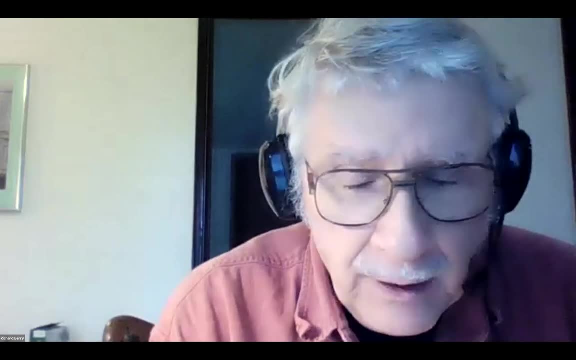 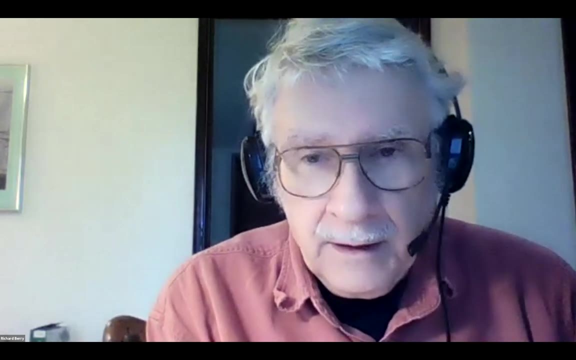 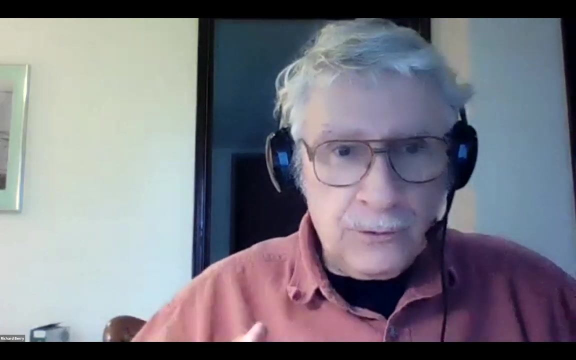 electroluminescent panel that gives you better than 1%. Yeah, and depending on the geometry of the situation, you can put a diffuser of some kind close up to the optical system on the DSLR so as to diffuse the image of the already 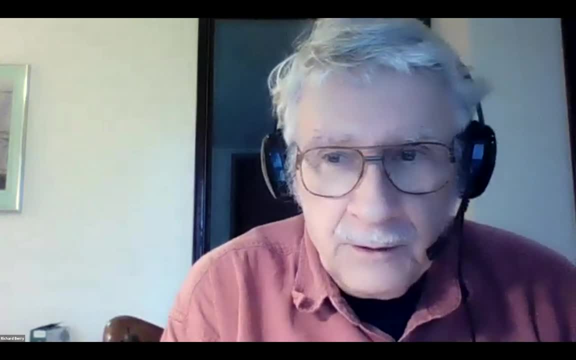 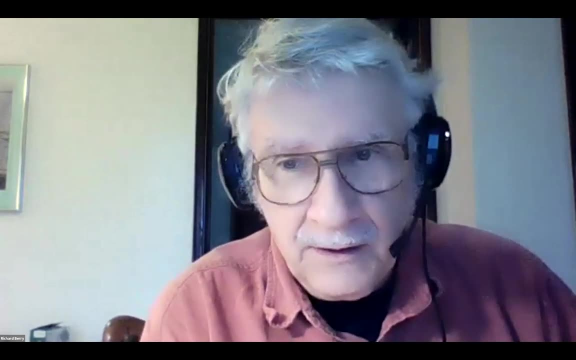 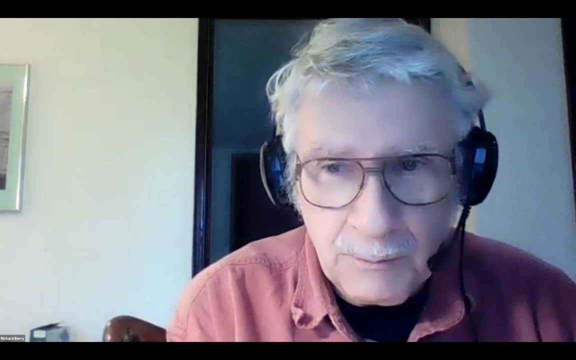 diffused source. There's a fair amount of this is going to depend on the focal length of the lens and the DSLR and so forth, but on the whole I wouldn't say that 1% is not bad Okay. So this question really is. 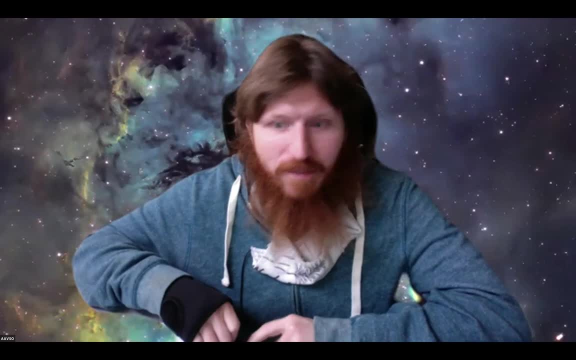 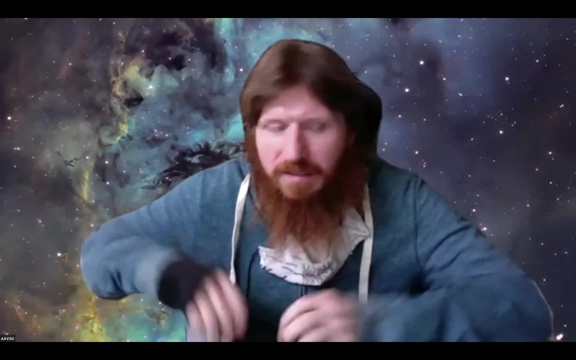 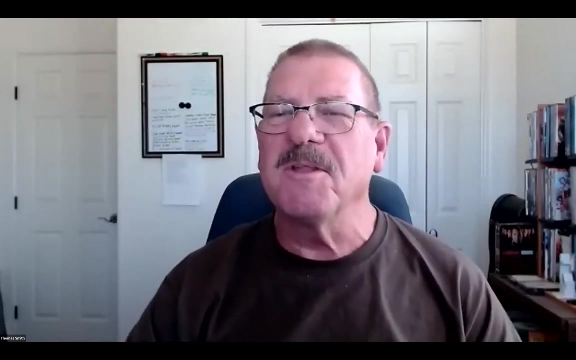 for Tom, I have a feeling that you're going to have to ballpark this quite a bit, but the question is: approximately how much would it cost to build a slide roof observatory that's 10 feet by 10 feet? I just typed an answer in there for the person that asked. 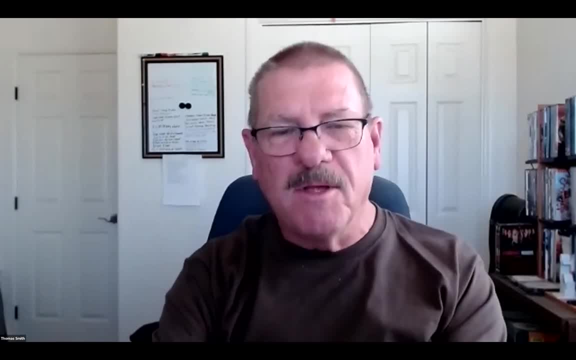 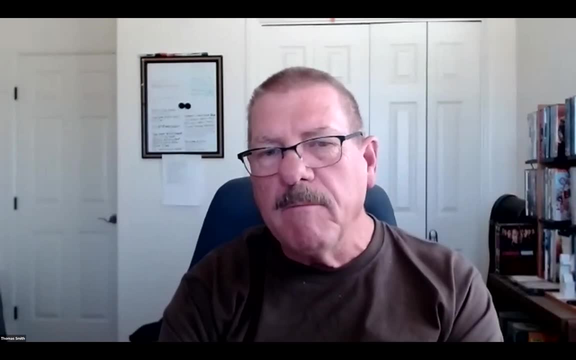 but that's okay. Let me give you my answer. Like Arnie Hendon always says, it depends- and it really does depend- on what you want to do with that 10 foot. I was able to construct a couple of small 8 foot by 8 foot observatories. in my quote unquote- backyard quarter mile away from me over there for under around $500 for the structure and it really only took a little while to do that. The hardest and long- not the hardest but the longest- part of that was building the pier I had to dig. 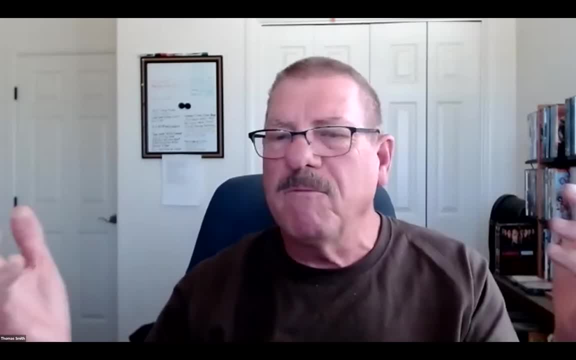 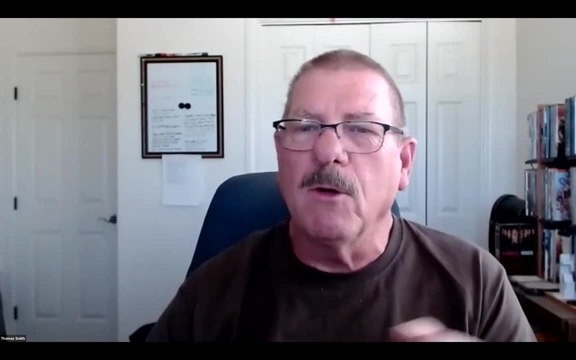 and I have nothing but rocks up here. So it can go anywhere, from you know $400 or $500 up to you know it's astronomical in prices. You can go anywhere you want and I don't mean to be tongue in cheek with that. 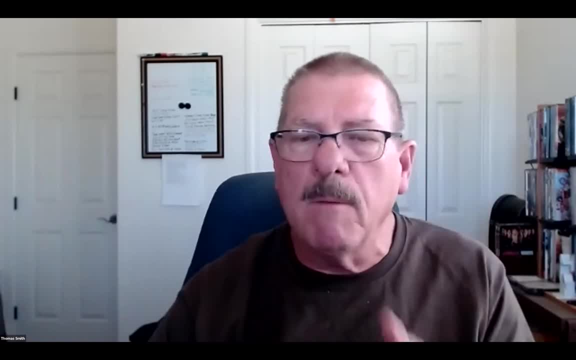 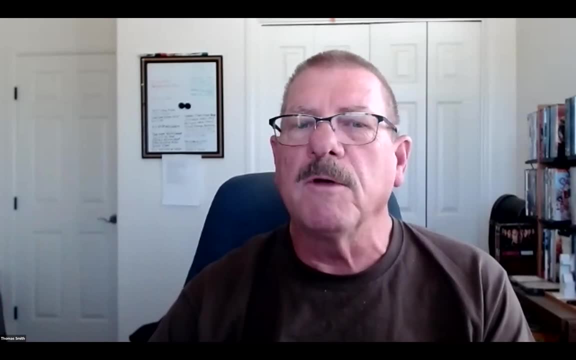 but it's absolutely true. If you want to make this thing totally robotic, automatic, don't touch things- fully integrated, you can spend upwards of $10,000, $12,000 on just your observatory itself. but you don't have to do that. You can put. 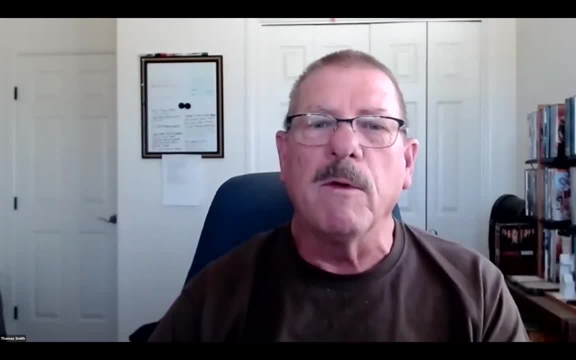 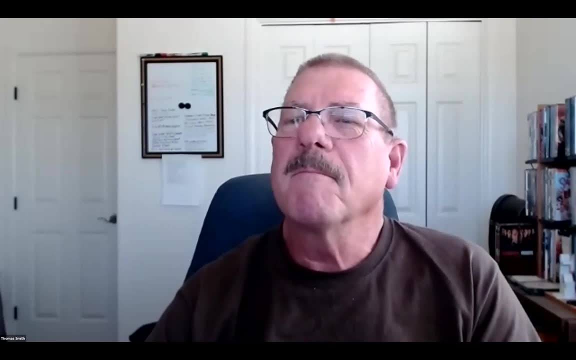 yourself a harbor freight tarp over the top of your telescope to start with, if you want Go from there. See if you enjoyed doing that kind of science work in your backyard. Hope that answered Cool Thanks. So this next question is probably going to. 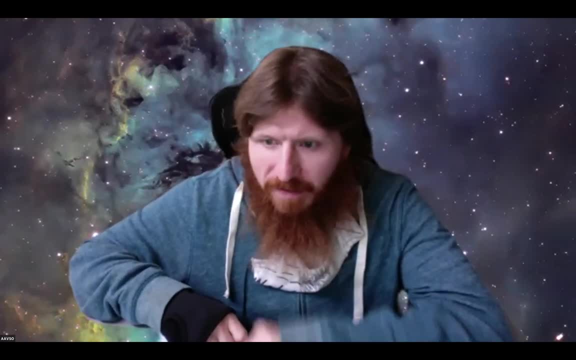 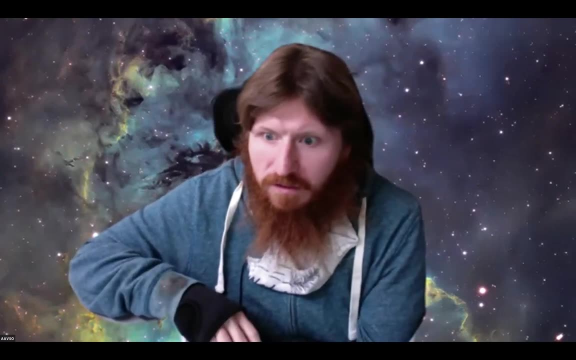 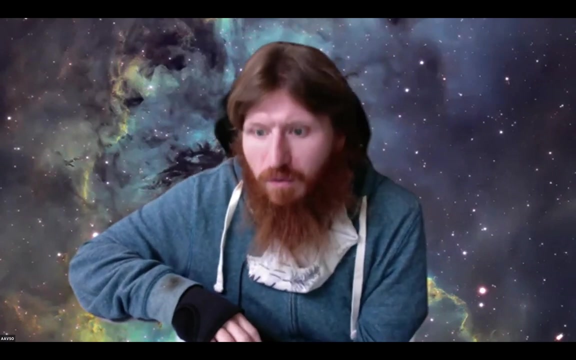 be a little bit of a debate, but I think it's worth asking. It says the various Johnson Cousins filters look very much like the response of many color CMOS cameras. Why not use a color CMOS camera and then select a given channel to correspond with either BG? 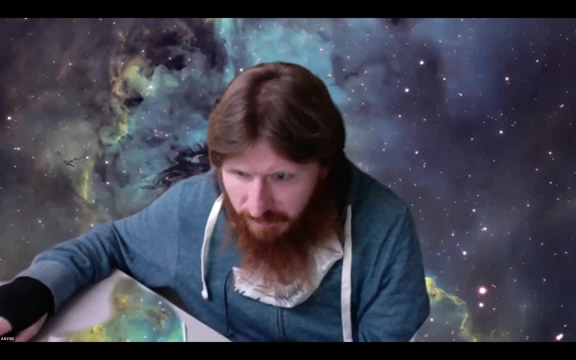 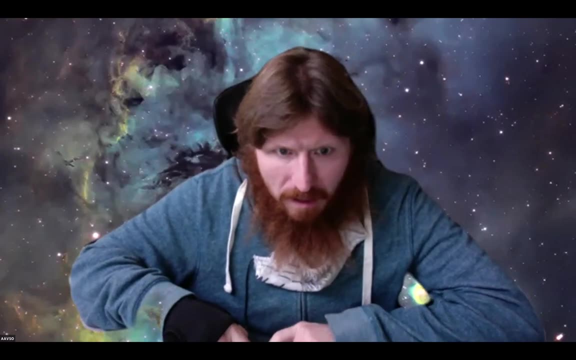 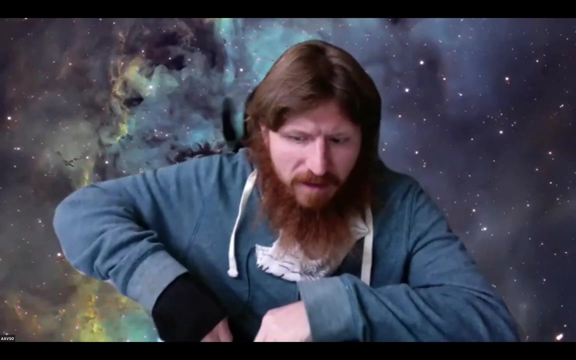 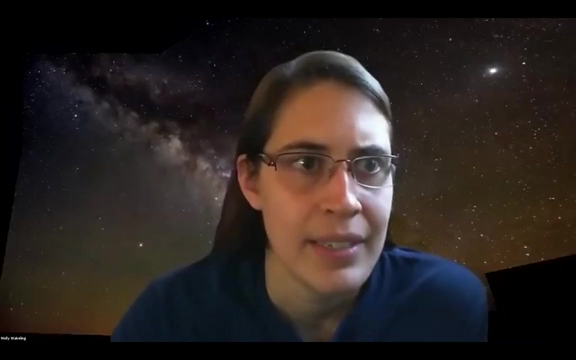 or R And then those will be reported as the various colors. So there are a couple of reasons to or not to do that. I think we'll be talking about this a little bit next week. Richard Well, these like the photometric filters and Sloan. 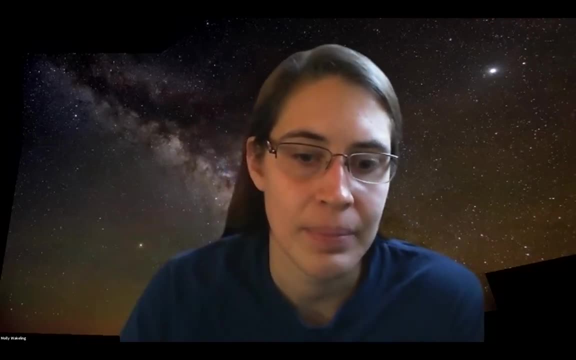 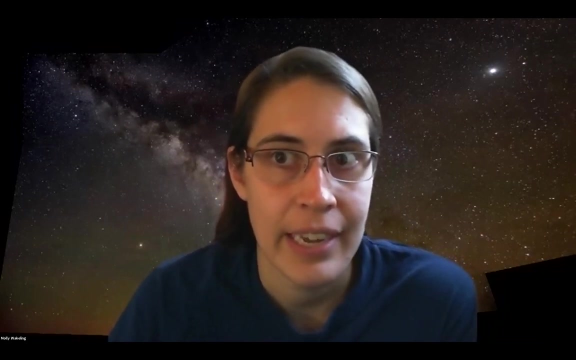 and whatnot. they have a standard wave band, whereas the color filters on a CMOS camera, or any color camera, are not standard and they cover a different part of the spectrum than the photometric filters, So you could be getting more of a different 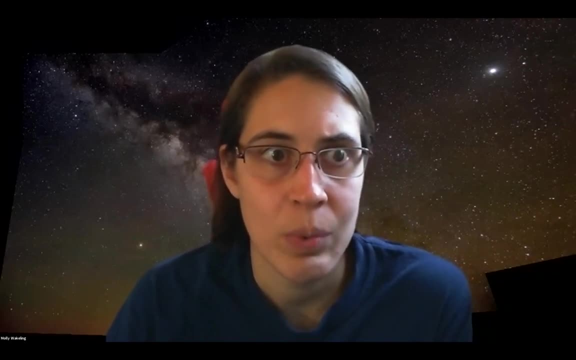 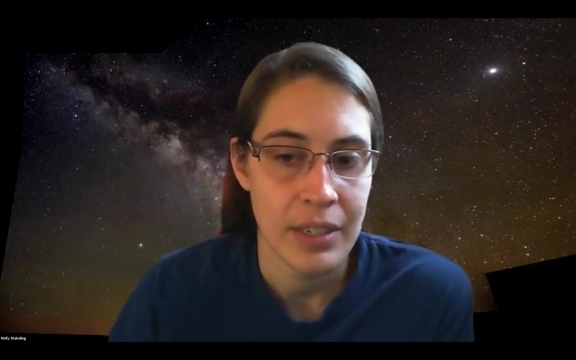 wavelength of light in that filter than the standard. So when you go and report that the magnitude of the star is this in V band, that's going to be slightly different if you use the G filter off of your DSLR or a G filter on a monochrome. 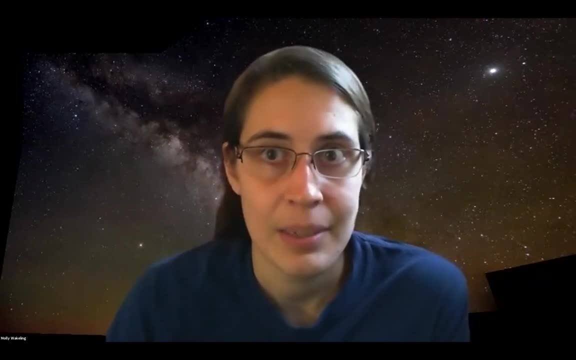 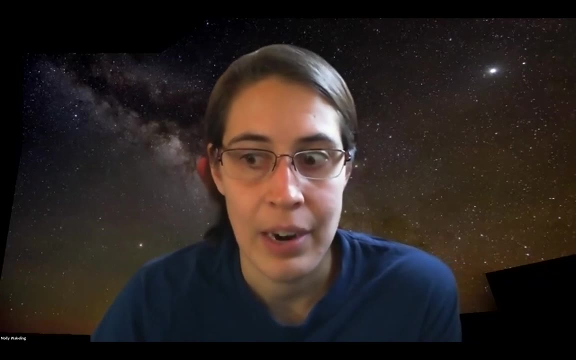 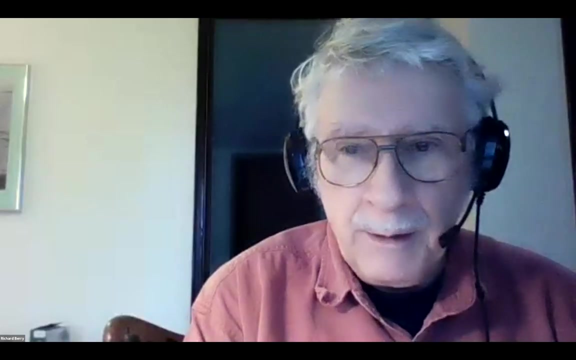 camera. They're not the same. I mean, they look similar, but they cover different parts of the spectrum, and the photometric filters are a standard that is known. That way, the measurements can be compared to each other more reliably. Yeah, the problems. 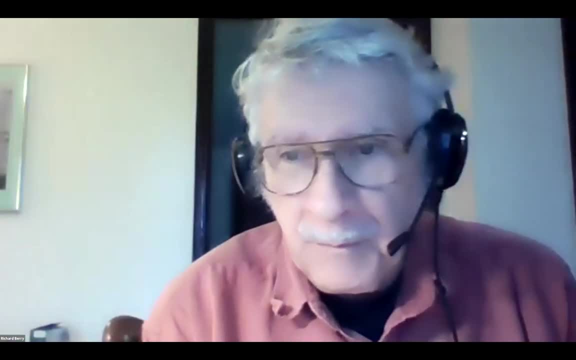 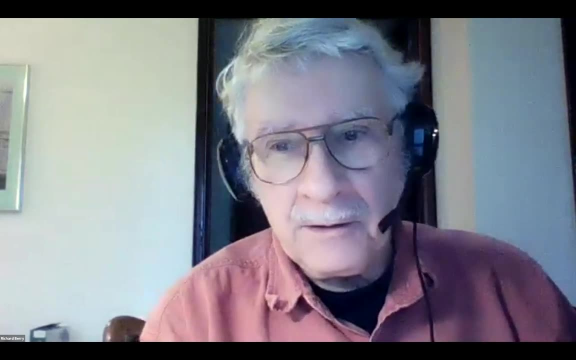 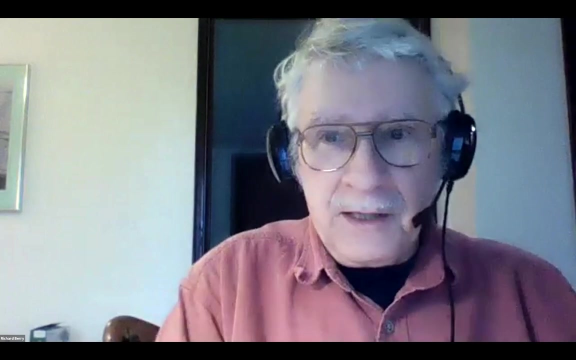 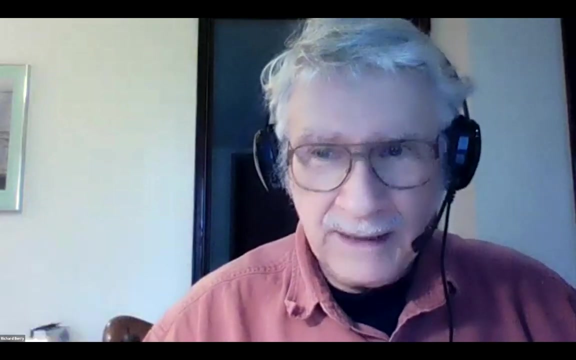 really seem to come with red stars, because, first of all, the color filters on the Bayer systems vary from maker to maker. What they do is they say, well, we'll just put on a stable dye that won't decay, And then we'll use software. 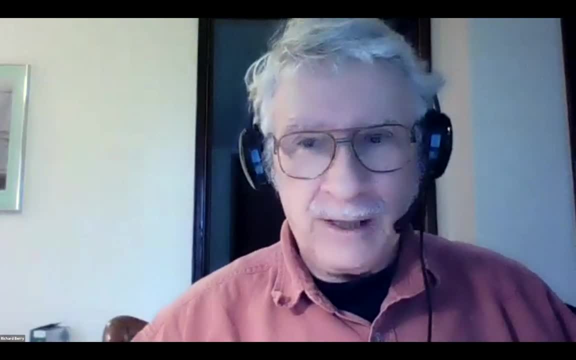 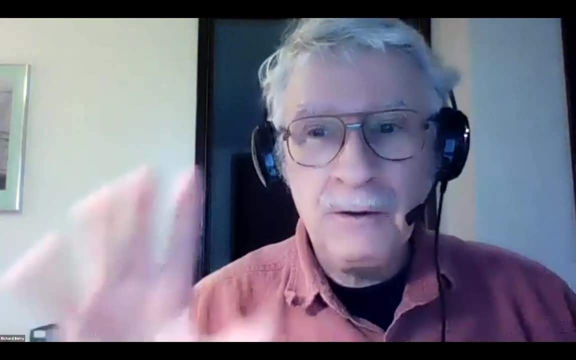 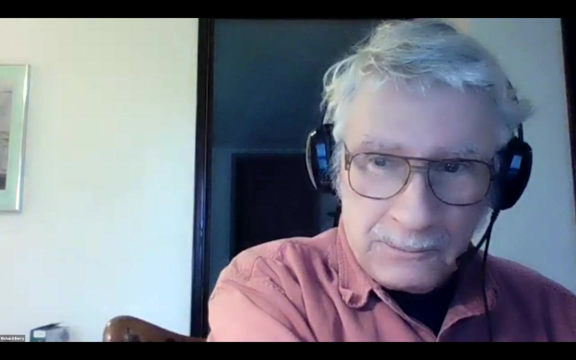 to transform the colors so that human flesh looks like human flesh and trees look like trees and the sky is blue. You could do that if you wanted to spend your life figuring out how to transform stars into standard magnitudes. Or you can say: well, 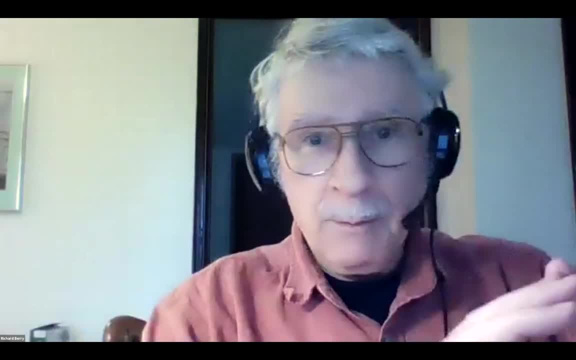 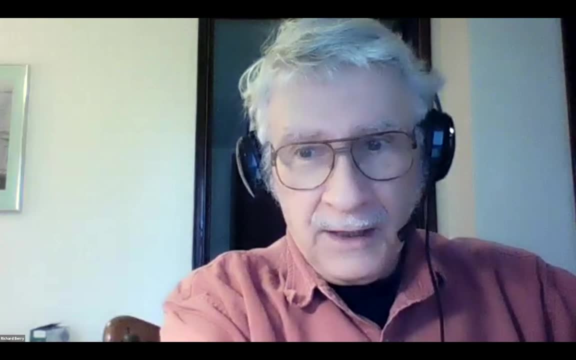 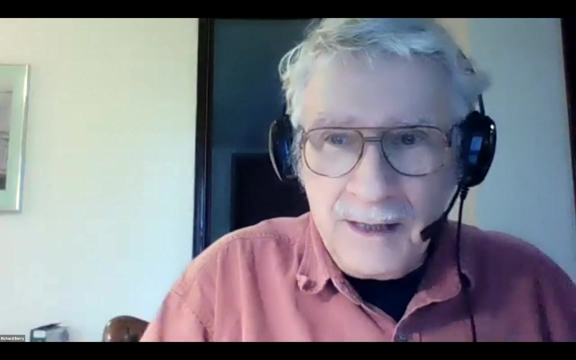 and this is what I've been experimenting with- is to cram them all together, figure out how bad the deviations are and then work on stars that are not red, And this takes us back to what Phil was saying: Yeah, you can use. 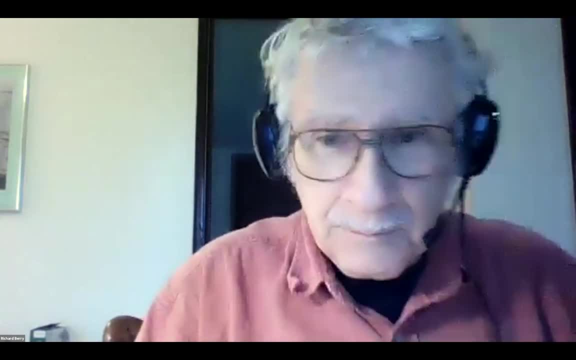 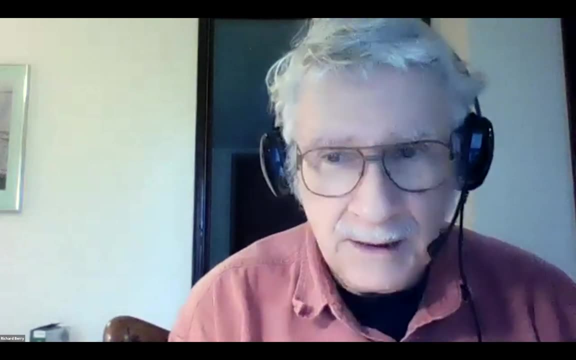 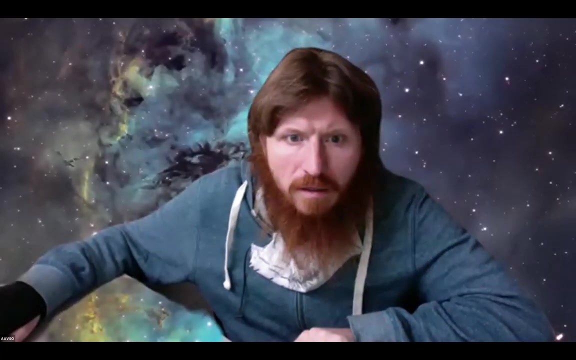 a green filter and it's a reasonable approximation of V and it can be transformed pretty easily into V. Tim, did you want to say something? Yes, I do. I think with the issue with the DSLRs, don't they use an infrared? 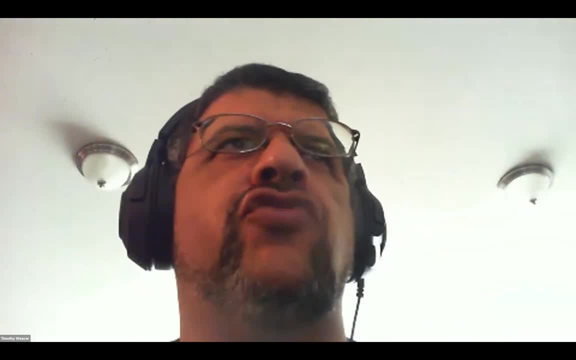 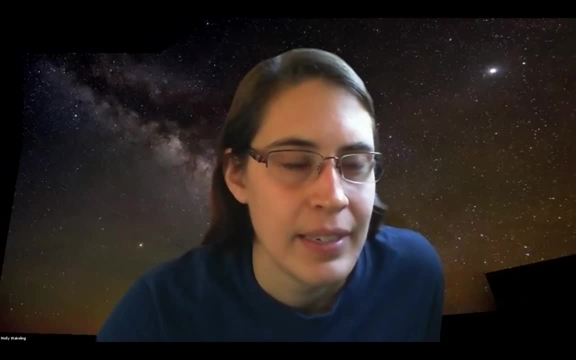 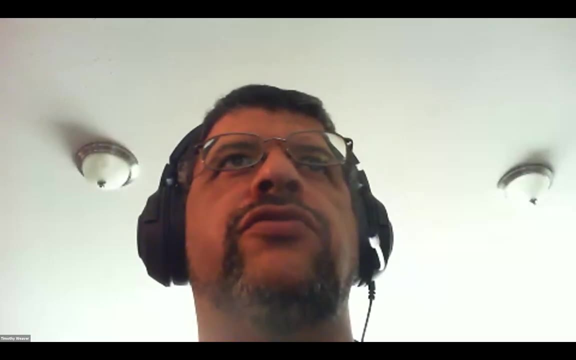 filter that wouldn't. that may or may not be in an astronomy CMOS camera. Is that correct? They have a spectrum filter that cuts out a lot of the red spectrum and all the IR and UV. Yeah, the DSLR ones do. 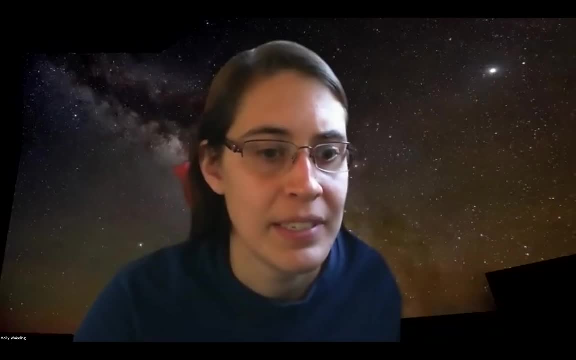 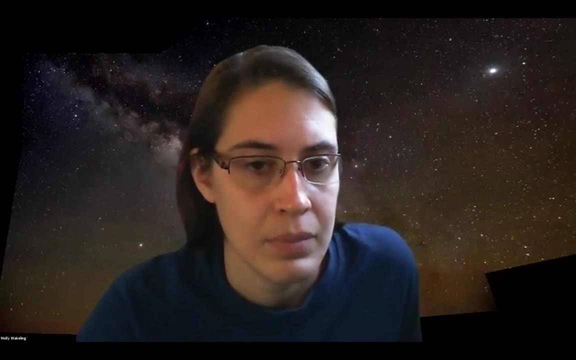 I know that. but what about the astronomy CMOS? Oh yeah, a lot of astronomy CCD cameras don't have the UV IR cut filter and you have to put one in your optics train, And the problem is you don't know whether it has that. 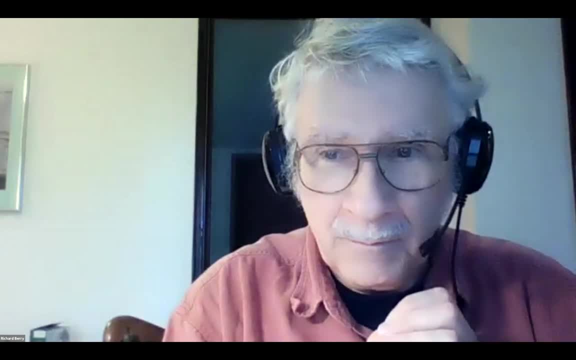 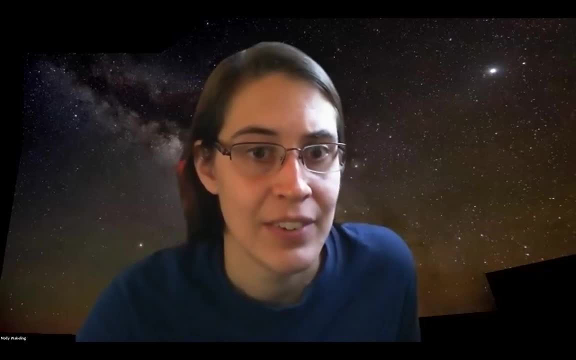 filter either. Usually you do, because you need to put one in your train if it doesn't have one. and it'll be pretty obvious if you're using a refractor, for example, and you get these bloats around the stars- Big bloated, yes. 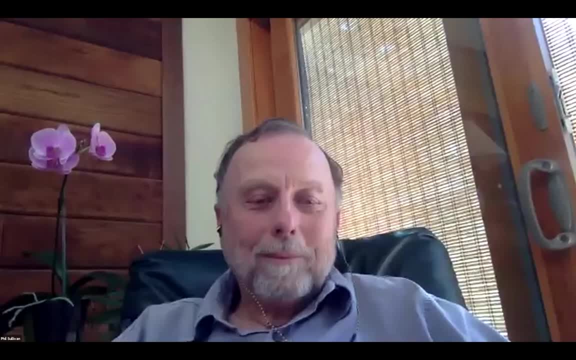 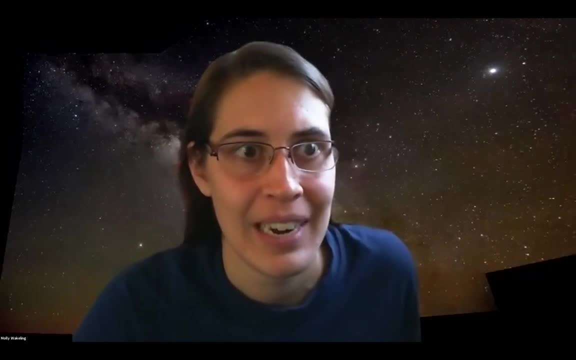 In a refractor, you will know right. Yes, I think that's published usually with the description of the camera, or, if not, the people on forums will tell you whether it has one built in or not. So it's really the variability. 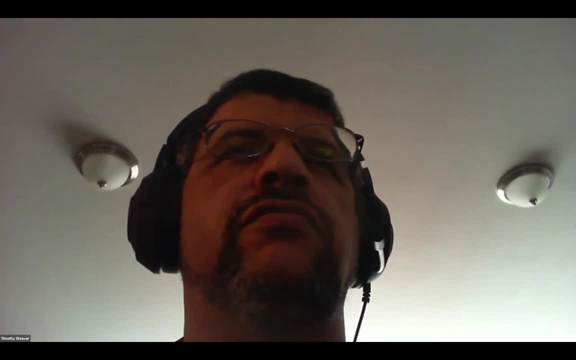 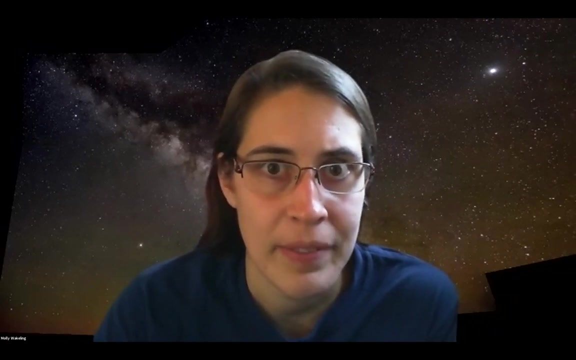 among color CMOS. that's the issue, But they go all over. it's all over the place when it comes to what color channels. what colors make it through what channel. Yeah, now I understand that there are ways to transform those, but I think you have. 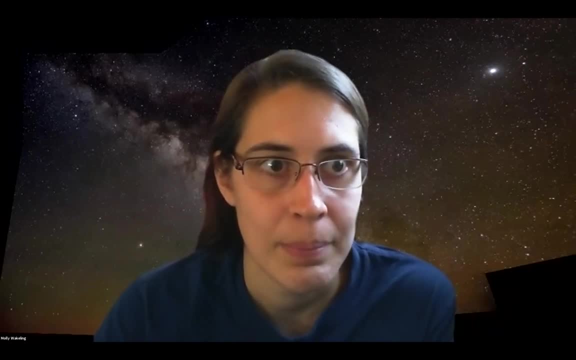 to do some measurements. I don't really know what all is involved. I'm hoping Barbara covers some of that in her talk, Because I know people do do DSLR photometry. You just have to either transform it or submit it, not as. 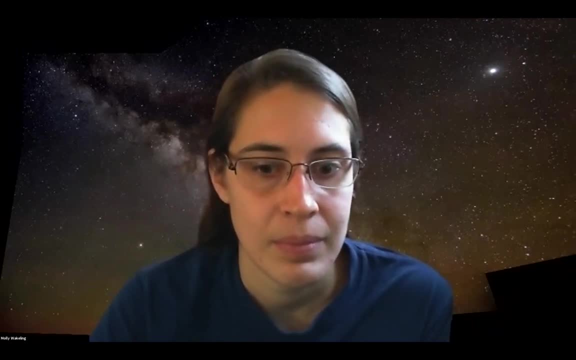 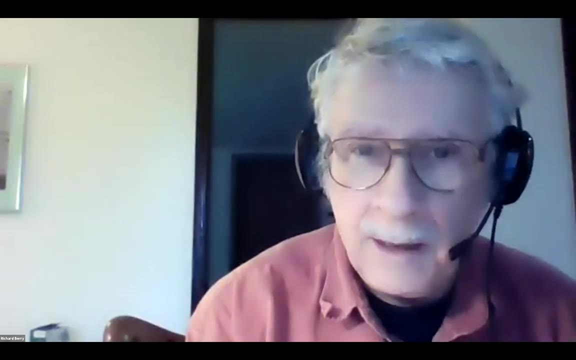 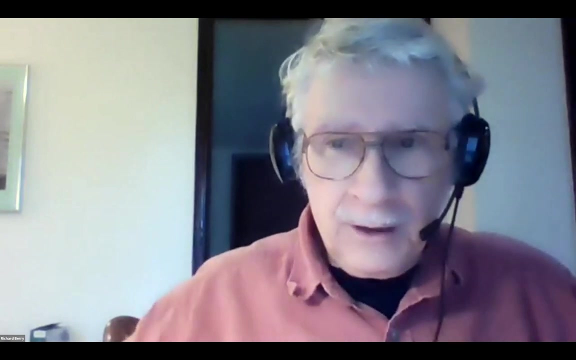 you can't say that it's V, because it's not. Not that you can't do photometry with a DSLR, but you have to do some extra stuff. Yeah, I mean, it would not be too difficult to work up a standard protocol for take a. 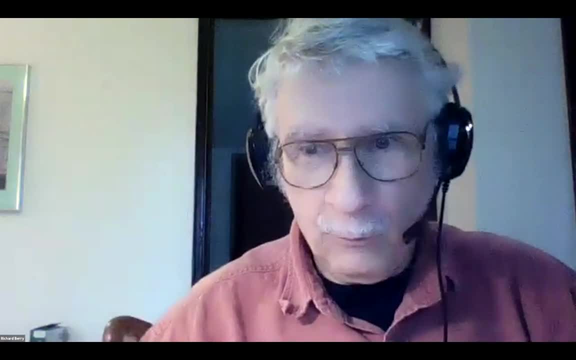 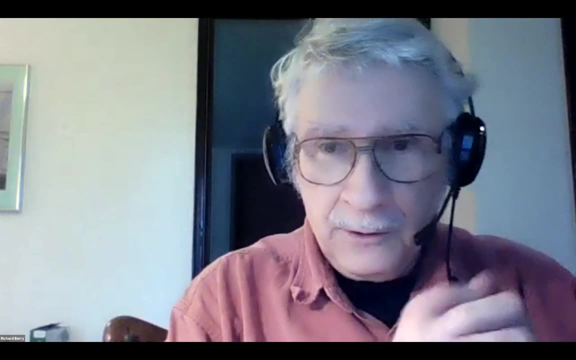 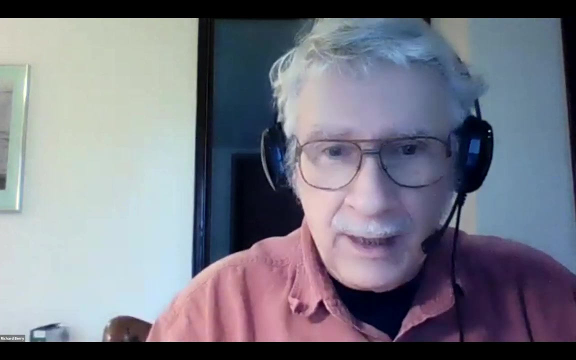 picture of this area, which has a wide variety of stars, especially a lot of extra red stars. Do the photometry with whatever camera you have and then determine whether or not you can do good photometry and what is the best way to do that. 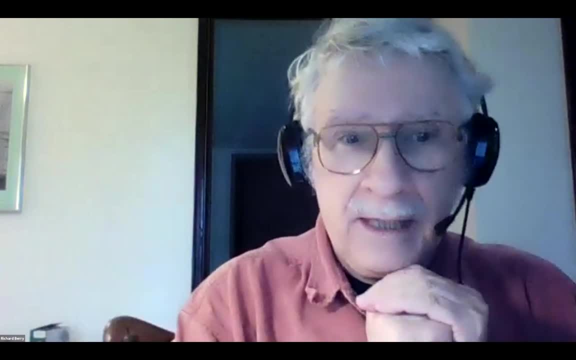 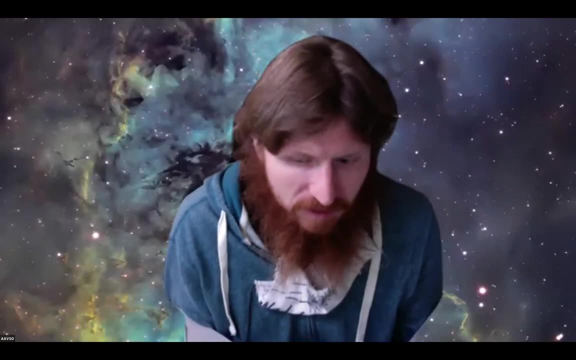 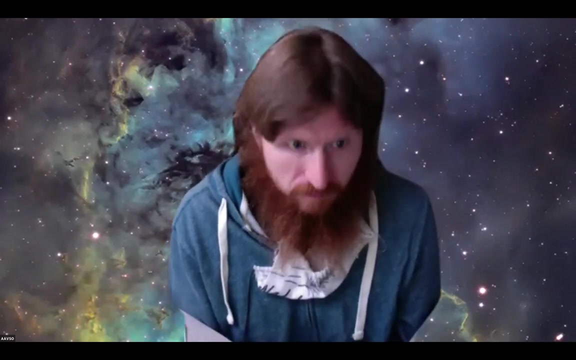 In other words, take a completely wild animal and try to tame it. One issue that I see with DSLR is that if you just want to take your own photometry and compare it to your own other photometry, that you do, it's likely fine. 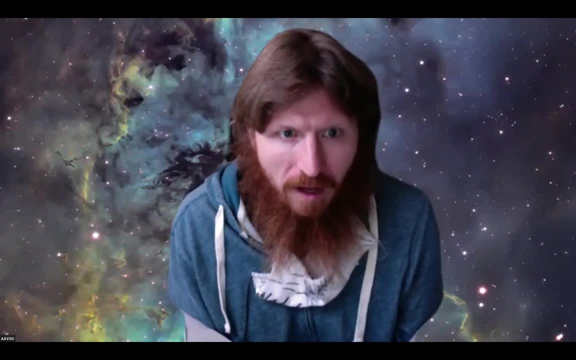 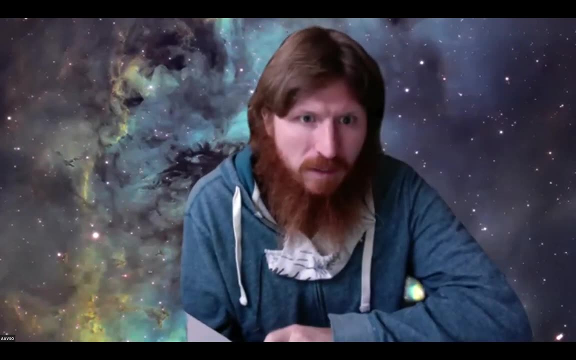 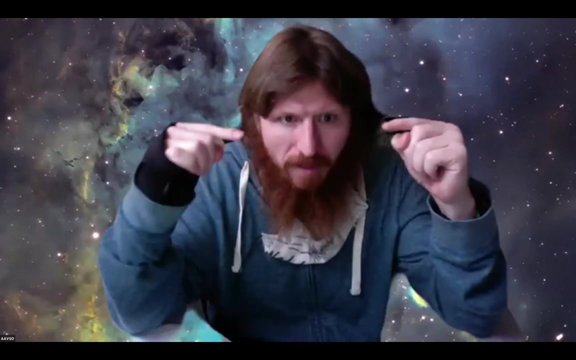 You can probably get good results, especially because you can, you know, do differential photometry and not necessarily care about standardizing it, so to speak. But if you want to submit it with respect to other people, then you really need to care about exactly. 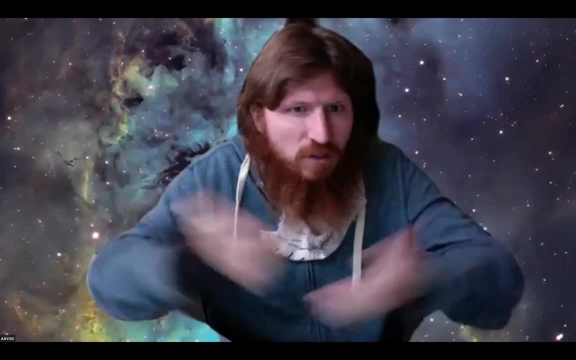 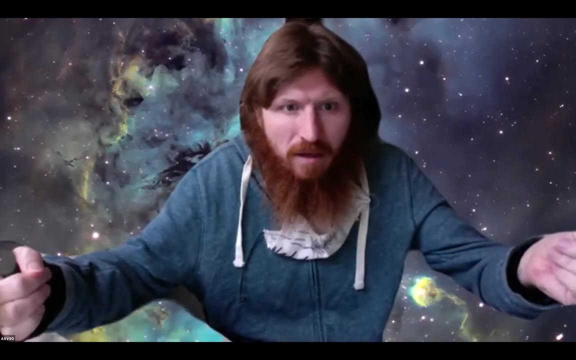 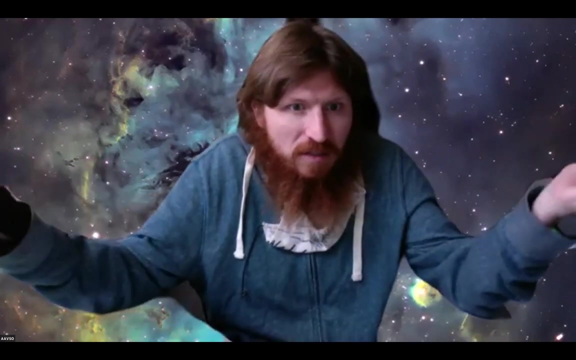 what that value is. And one thing that's just never been clear to me is that, from camera to camera, how close is TG, TR and TB? You are using one DSLR versus another. Are the response curves the same for each of those different types of pixels? 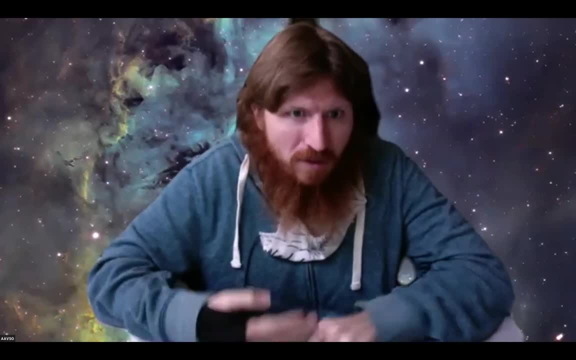 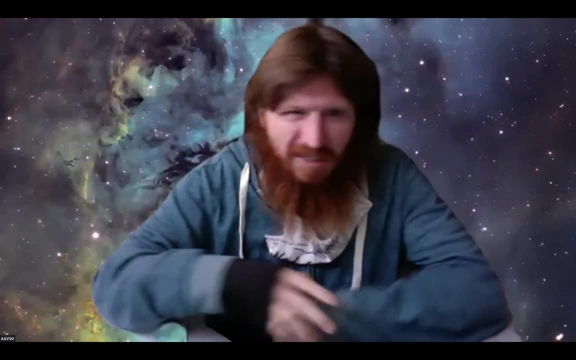 And that's something that I've never gotten a good answer to And that, even if they're close, it could cause some problems when you try to compare from observer to observer, which is one thing to worry about with DSLR. But 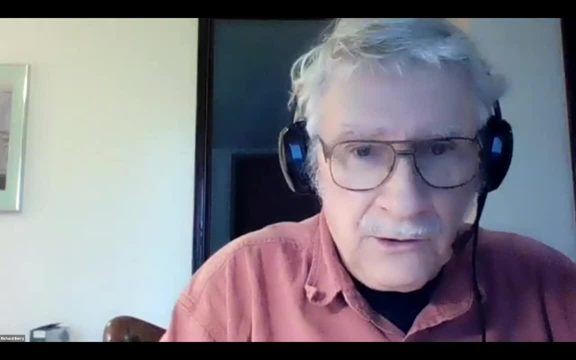 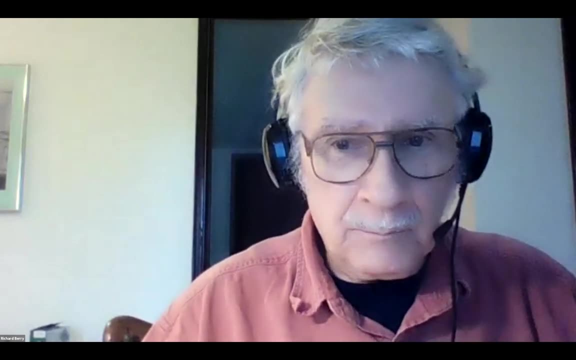 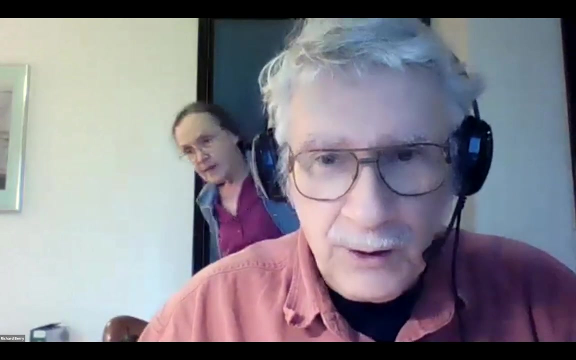 it just kind of depends a little bit. Exactly the same problems or exactly the same arguments. with one-shot color cameras, You, they, the company that manufactures the chip is not trying to do astronomy. They're trying to make pretty pictures of one kind or another. 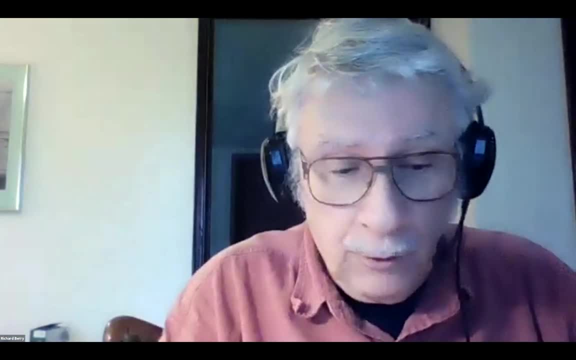 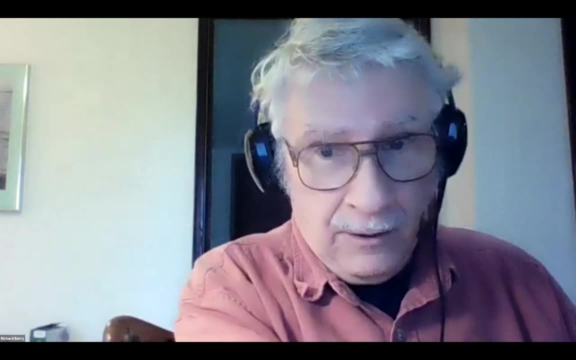 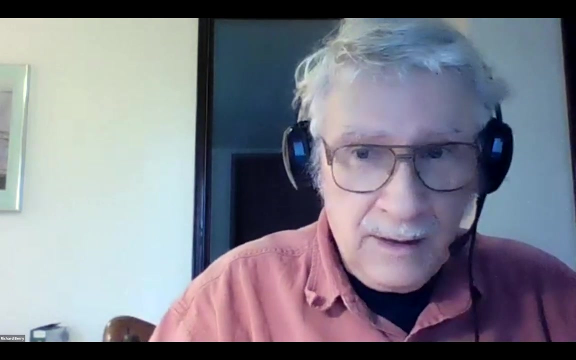 And basically we're only coming up to a time when- because, as CCDs get harder to find, we're now coming up to finding that these inexpensive Bayer cameras- and inexpensive well, basically, DSLRs too- are inexpensive Bayer cameras. how to use those optimally? 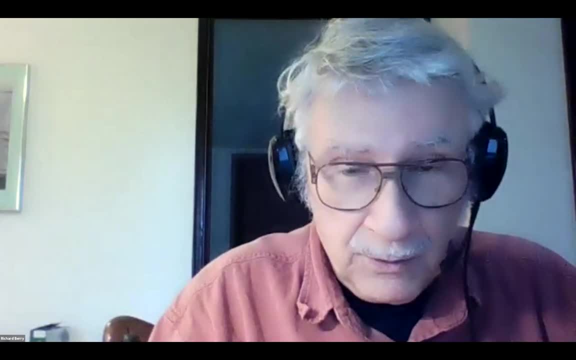 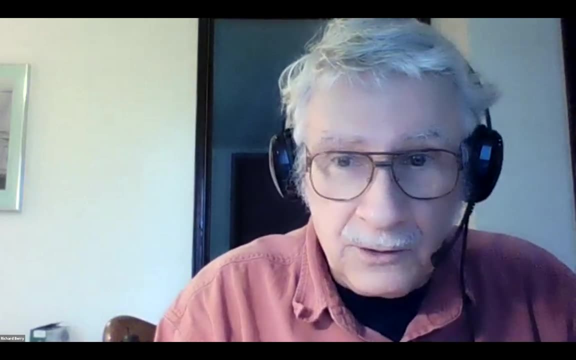 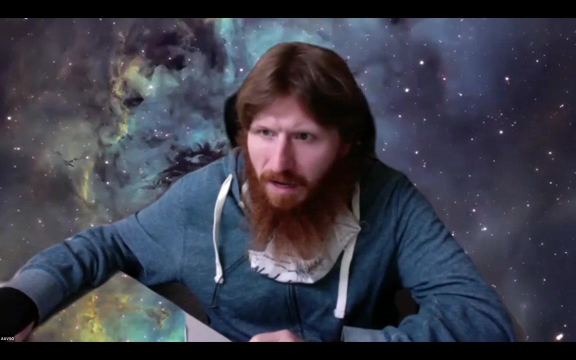 And the answer is, as sort of indicated is: we really don't know the best way to use these things yet There is experimental work to be done. Okay, and with that I we didn't get to quite all of the questions, but we did do quite.